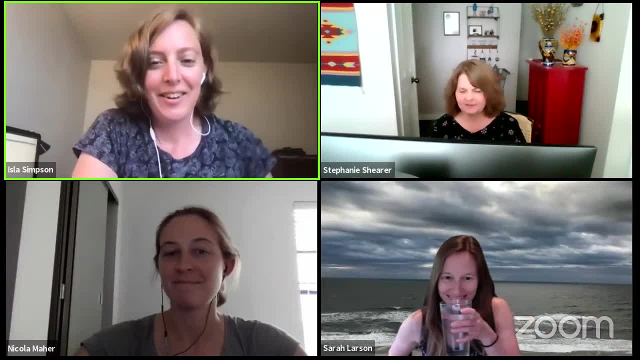 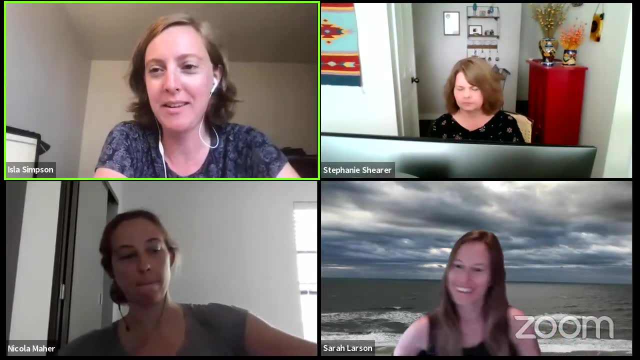 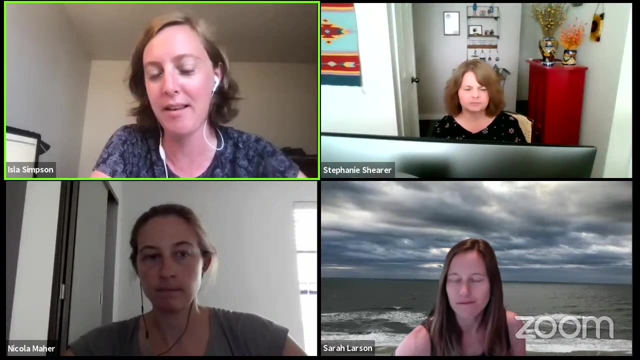 three for me. All right, let's get started. It's one o'clock and I didn't leave any time for logistics, So welcome to the Climate Variability and Change Working Group meeting. So we have a lot of excellent talks lined up this afternoon. This is being streamed live on YouTube. I 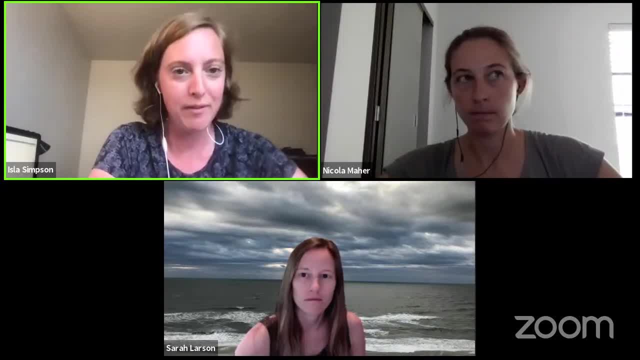 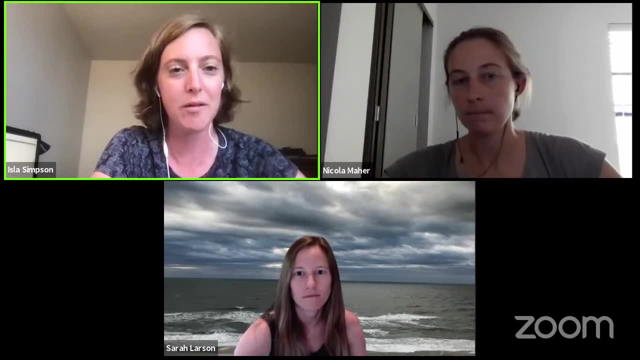 hope you're all doing well And also the chat will be saved, and that includes any private chats you might make. They're downloaded as well when you do that. So for the speakers you have a 10-minute slot, leaving two minutes for questions. We'll give you a warning at 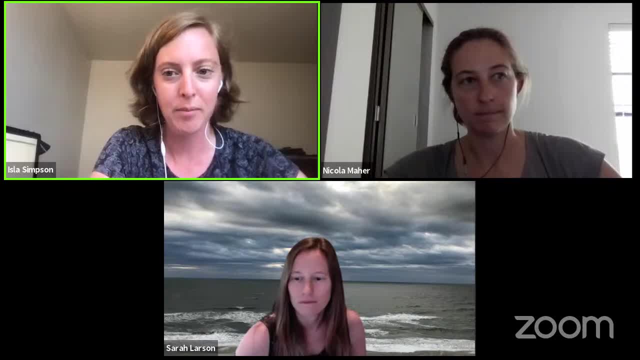 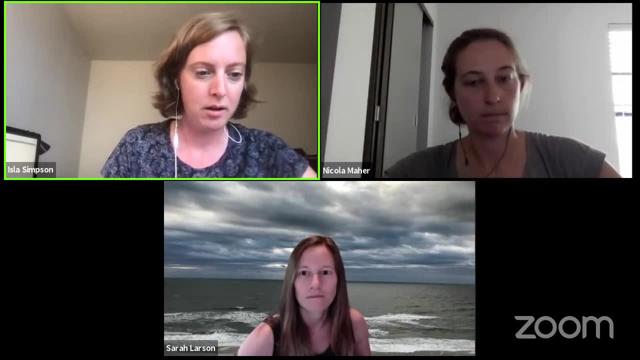 eight minutes and then we'll stop you at 10.. So Aishu is going to chair the first session. Aishu, Okay, Now let's start the meeting. As I said, I'm going to start the presentation. I'm going. 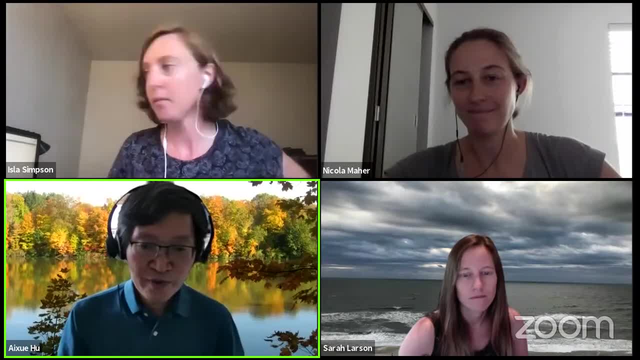 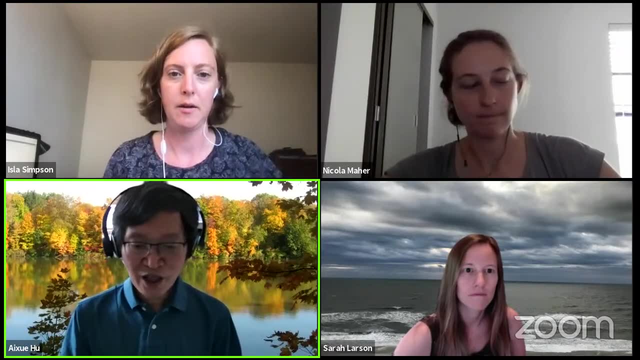 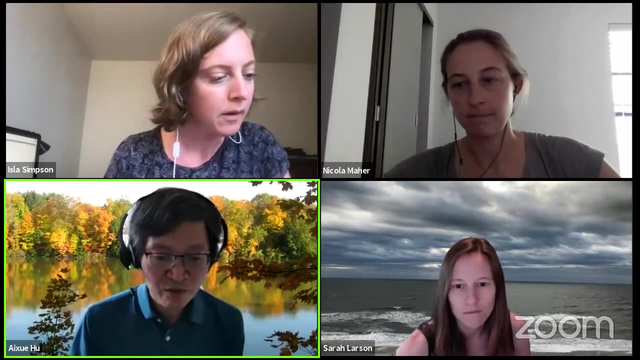 to start the presentation. As I said, the meeting, the talk will be 10 minutes and with two minutes of questions. I will give you an eight-minute warning And before we start, I would like also take this opportunity to thank Jiri and Emil for his long leadership role in this working group. 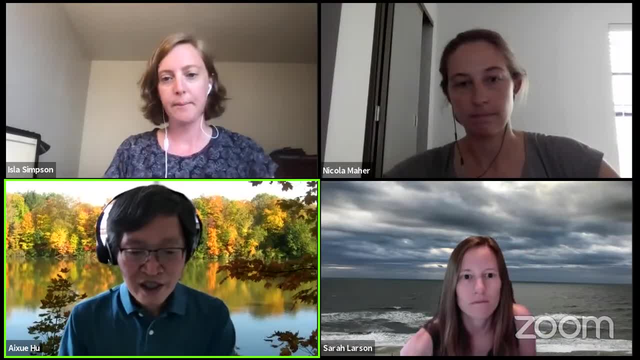 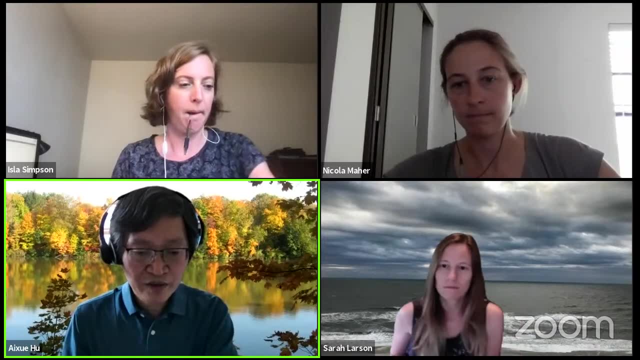 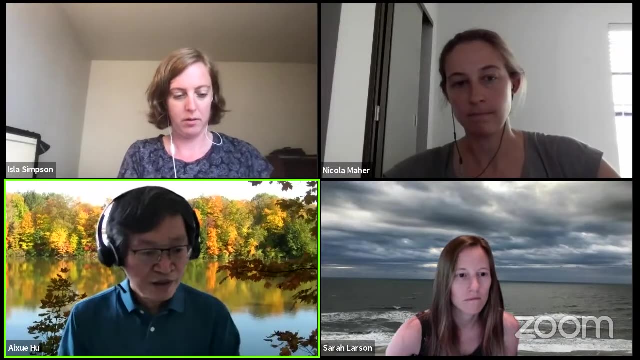 and congratulate him for winning the CSM Disengagement Achievement Award, And also I would like to thank Xiangping Xie and Pierre Collector for their service for this group, And they stepped down in the screen and welcome Sarah and Larson to join the CBC Working Group. 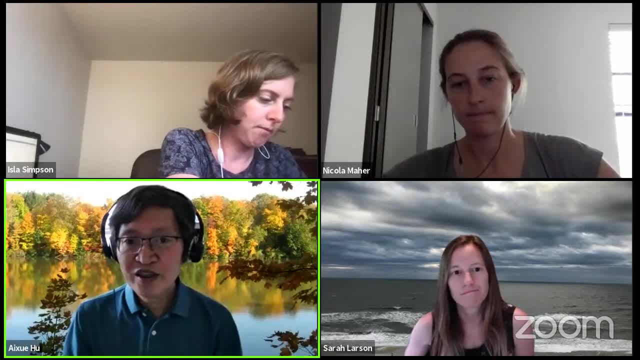 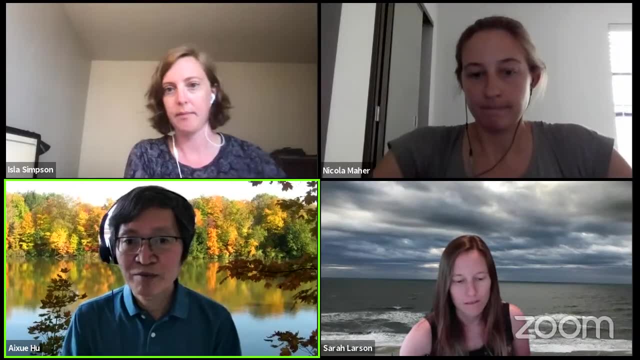 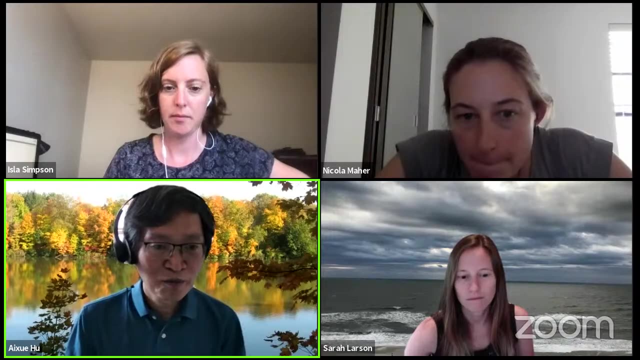 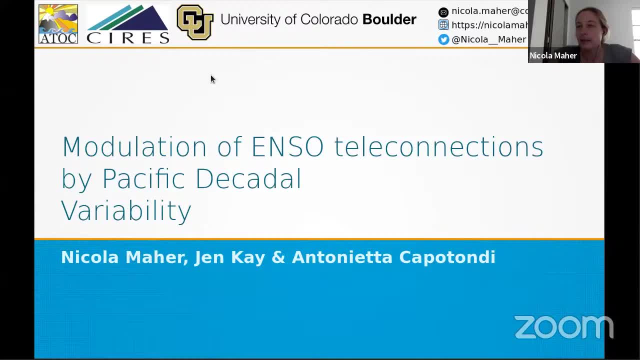 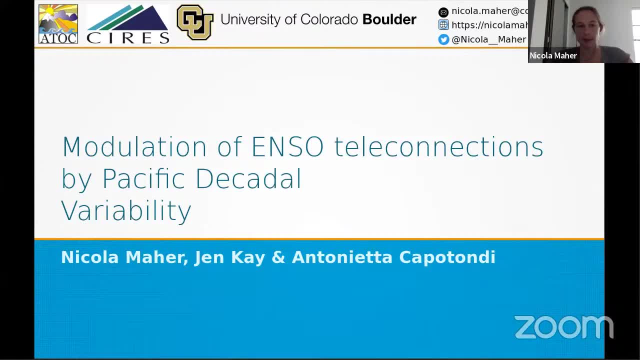 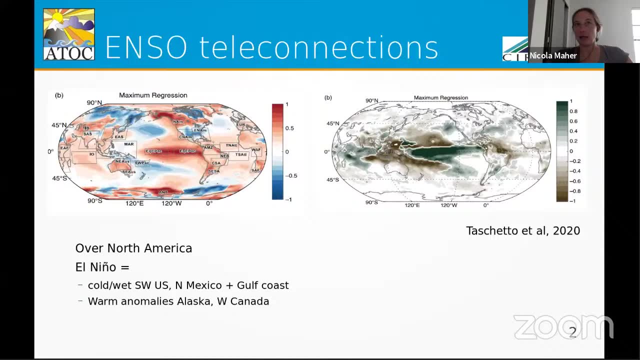 can modulate ENSO teleconnections over North America, And this is work I'm doing with Jen Kay and Antoinette Capitondi. Okay, so in the figure here you can see ENSO teleconnections And this is the maximum regression of temperature change and energy. And then the next slide. 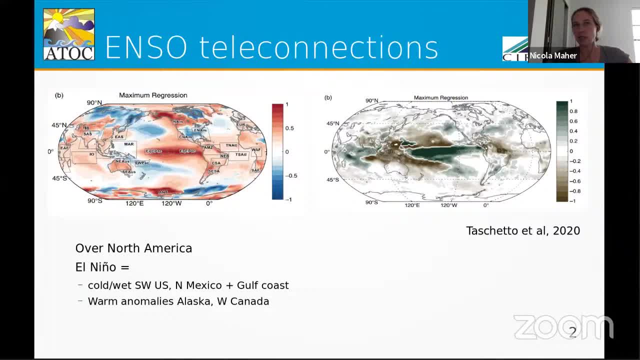 I have MUSICS of temperature on the left and precipitation on the right onto the ENSO index from Tashedo et al 2020.. And you can see that ENSO has global teleconnections and over North America, El Ninos tend to cause cold. 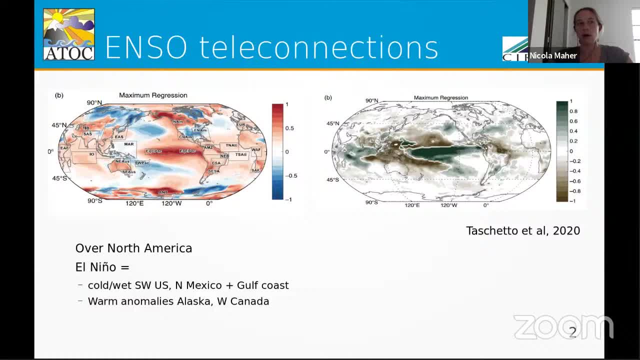 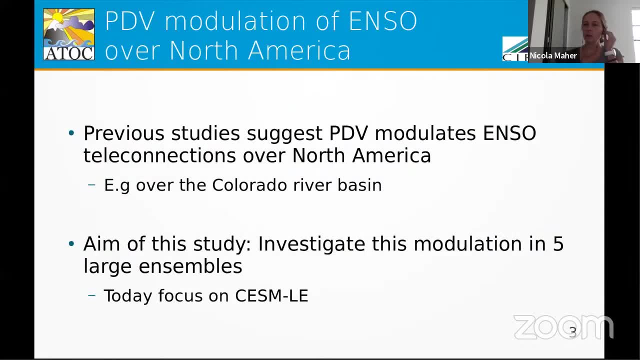 wet conditions over the southwest US, north of Mexico and the Gulf Coast, and warm anomalies over Alaska and western Canada. Okay, So previous work has suggested that the PDV can modulate ENSO teleconnections over North America and there's been a lot of local studies. 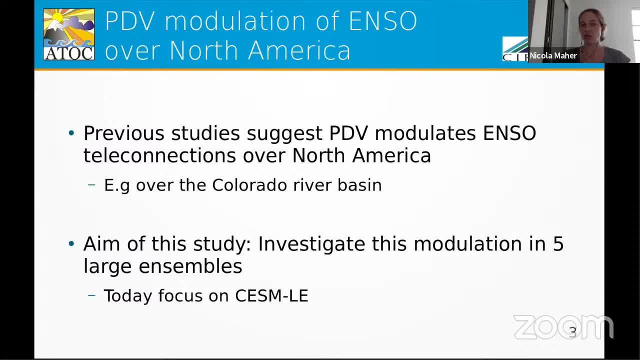 including one that suggests that the PDV can change ENSO teleconnections over the Colorado River Basin by changing their spatial imprint, and then this can actually change the sign of what you see. So the aim of my study is to investigate this modulation in five large ensembles. 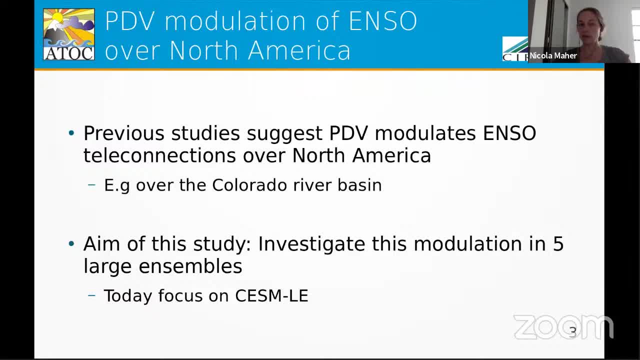 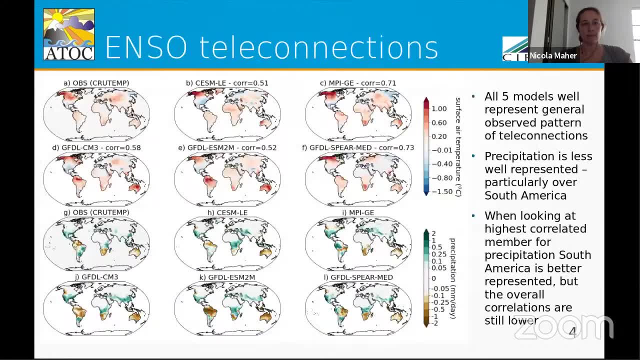 And we're using large ensembles because we have lots and lots of events that we can composite over and we can use them to study the changes in the environment And truly tease out the role of each of these modes of variability. Okay, So the first question we want to ask is: 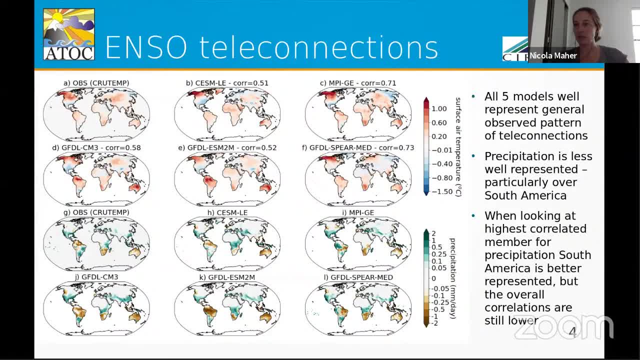 can the models actually represent ENSO teleconnections? So the figure you see here on the top in red and blue shows temperature teleconnections and in the bottom in green and brown, shows precipitation teleconnections. The observations are in the top left And I'm showing the ensemble member. 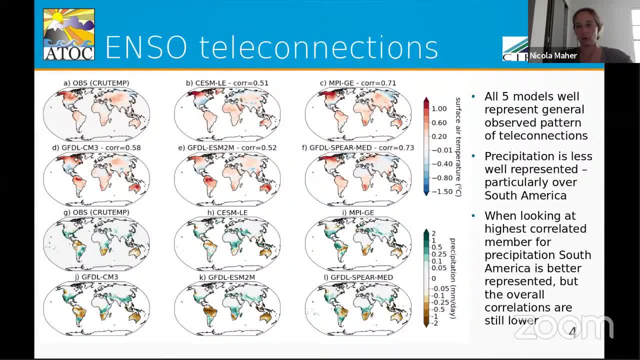 for each large ensemble that is modulated by the most highly correlated observations. You can see that the temperature patterns in observations are generally well represented in all of the models, as are the precipitation patterns. However, the precipitation patterns are kind of a little bit less well represented over South America. 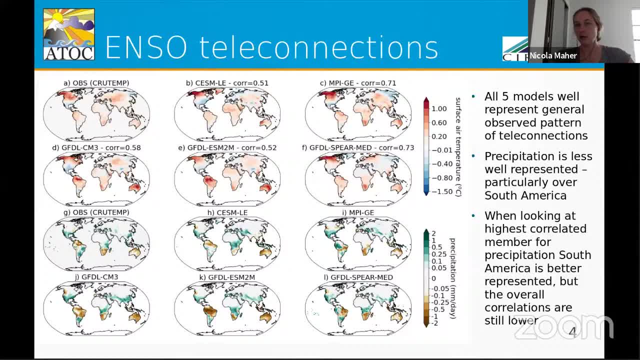 I'll note that if we do the same thing, where we use the highest correlated member for precipitation instead of temperature, this bias over South America looks a lot better, but the overall correlations are still lower for precipitation than temperature. Okay, The second question you might want. 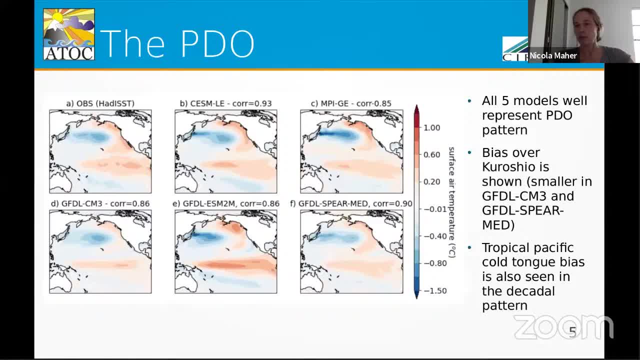 to ask is: can the models actually represent Pacific decadal variability? And today I'm going to use the PDO index or the Pacific Decadal Oscillation. And this figure is very similar to the previous one. We have observations in the top left and the highest correlated ensemble member for each model. 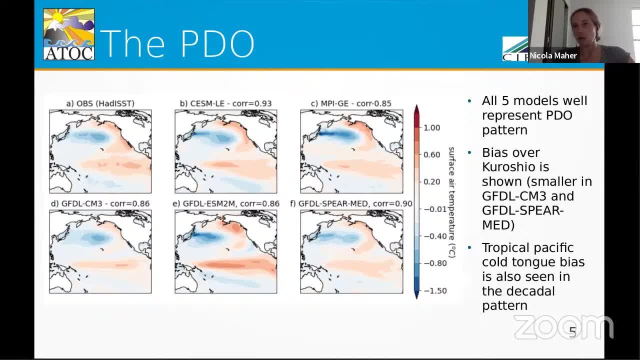 You can see again, the overall pattern is well represented in all models but we do see some biases, particularly in some of the models, including CSM over the Curratio region, And we do see this tropical Pacific cold tongue bias. that's. 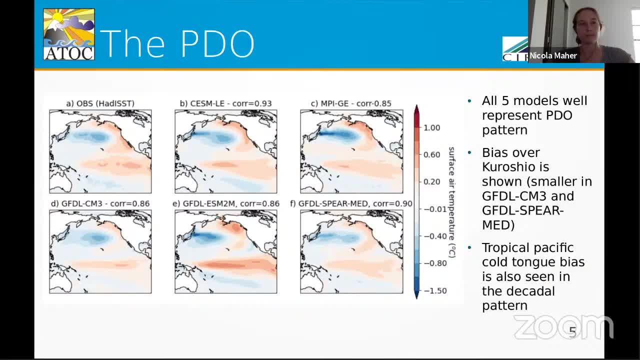 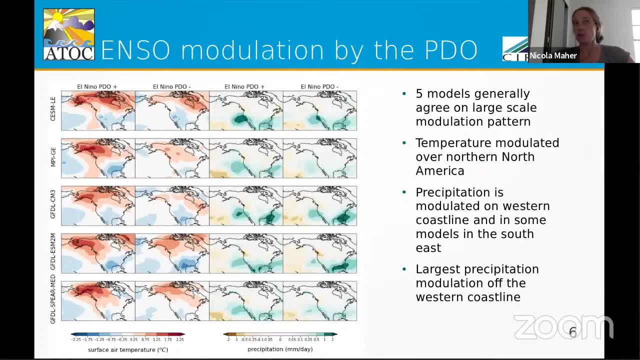 in the interannual ENSO signal as well in this decadal pattern. Okay, So let's jump straight into some results and try and answer the question: is our ENSO teleconnections modulated by the PDO over North America In the figure you can see here? 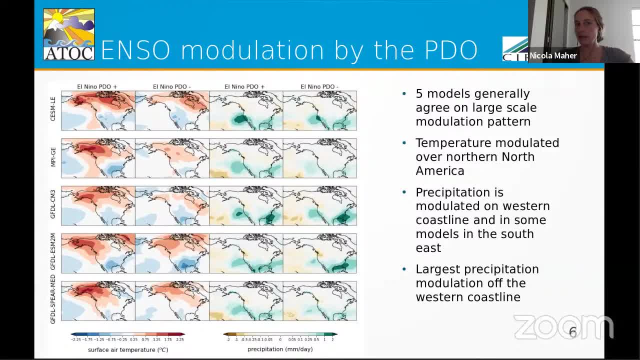 each row is a different large ensemble with CSM large ensemble in the top row And I show again red and blue for temperature and green and brown for precipitation. The left row of each set of columns is El Nino's, when the PDO is in a positive phase, and the right row is 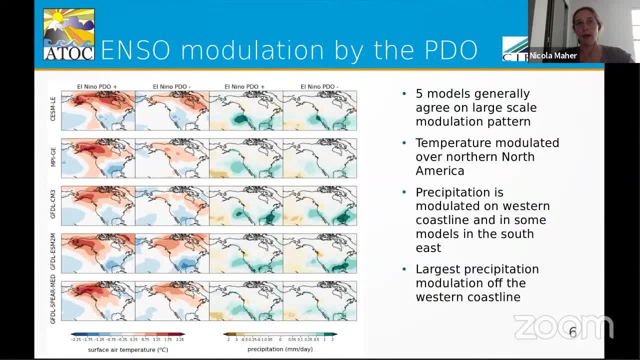 when El Nino, when the PDO is in a negative phase. So we can see a few things here. First, the models generally agree on the large-scale patterns. although there are definitely some local differences, The temperature patterns are very similar, They're very similar. 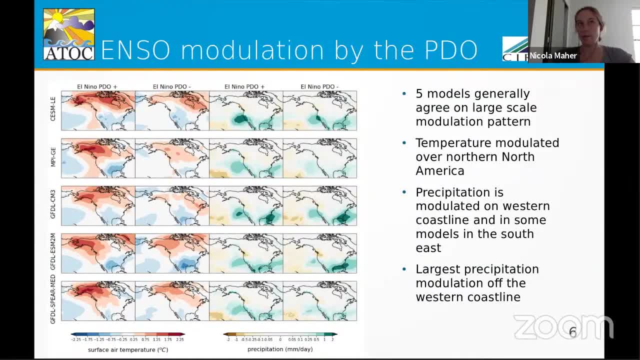 The temperature pattern is most strongly modulated over Northern North America by the PDO. Precipitation is most strongly modulated over the Western coastline by the PDO And we do in some models see something happening off the Eastern coastline as well And we say the largest precipitation modulation is 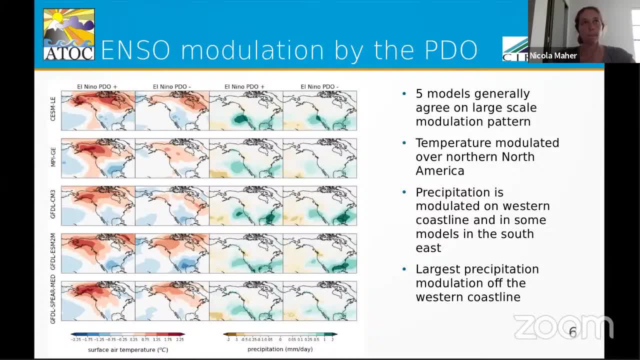 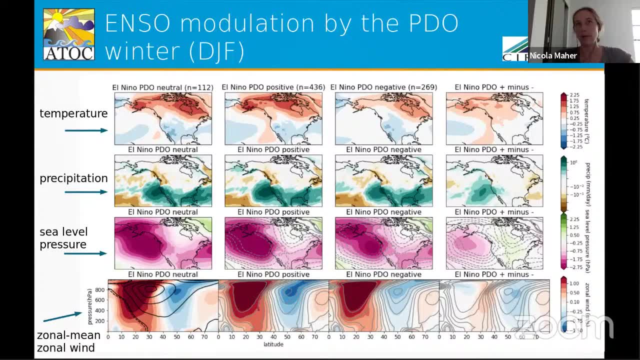 actually generally offshore. Okay, So now I'm going to use the CSM large ensemble to really delve into what we're seeing and why we're seeing it. And so this is the winter DJF response, and again you'll see temperature and precipitation. 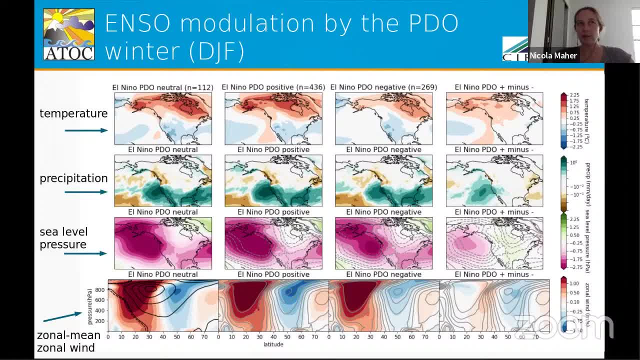 in the top two rows Here. on the far left we have El Nino's when the PDO is neutral. The second column is El Nino when the PDO is positive, The third column is El Nino when the PDO is negative And on the far right we have the El Nino's. 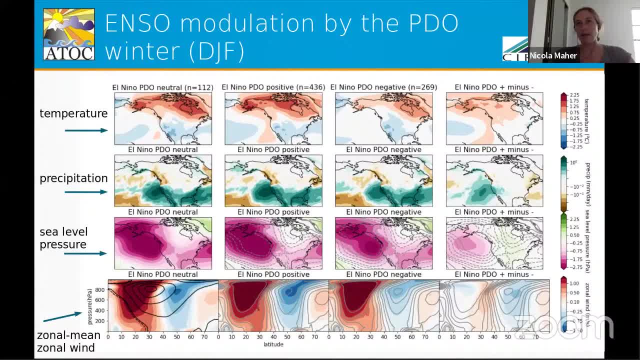 when the PDO is positive, minus the negative. Okay, And so you can see those patterns I've already described for temperature and precipitation in the top two rows. The third row, so the pink and green, is the sea level pressure anomalies, And you can see this basically. 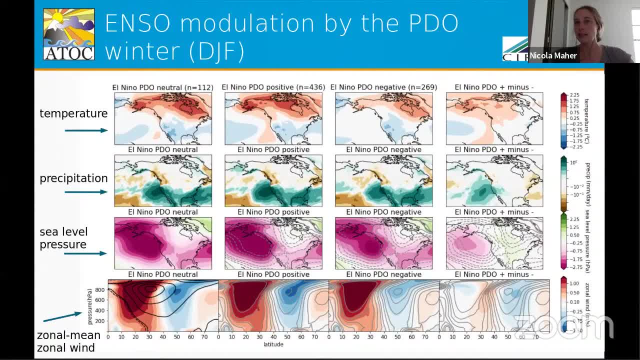 this big pink blob is the Aleutian low, And what you can see here is when the PDO is positive, the Aleutian low is strengthened and moved a little bit to the west as compared to when the PDO is negative. We also see a small increase in the high pressure. 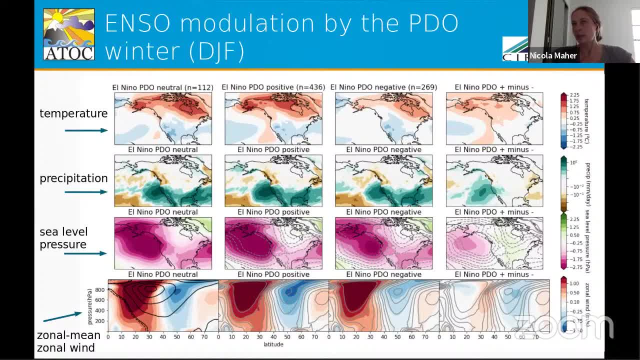 over the American continent And this could be what's causing, you know, the temperature anomalies we see in the top row, as we're bringing more warm air from the south, where it's warmer, up into the northern latitudes, And this kind of small high pressure anomaly. 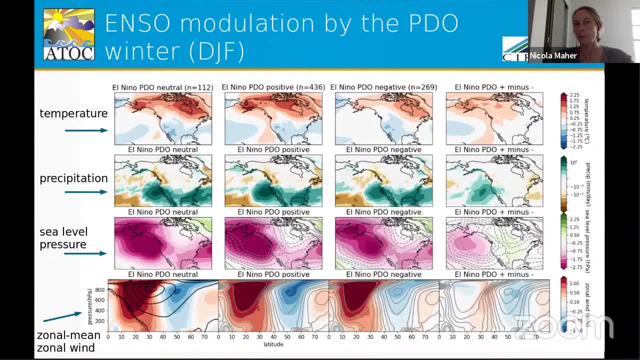 over the continent could also be causing less cold pressure events to happen over the northern north US. In the bottom row we have the zonal mean zonal wind, And I'll direct your attention to the bottom left panel first. Here the black contours are the mean state. 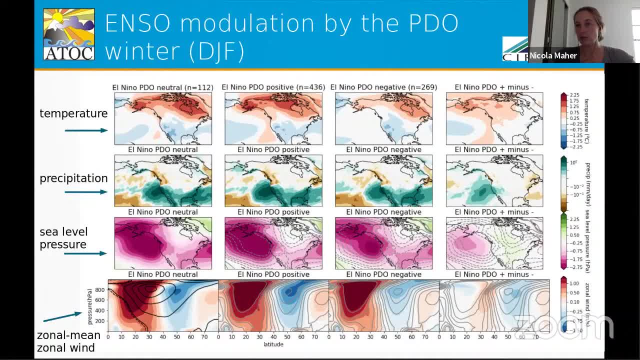 And the color is the mean state, And the colors are the anomalies for El Nino events when the PDO is neutral. And so you can see that the mean state, the winds that kind of, or the jet that comes onto the coastline of North America. 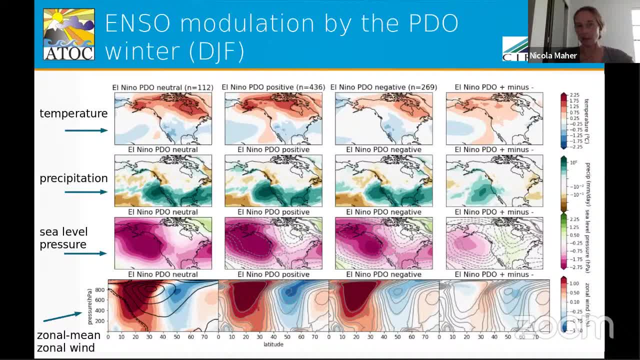 is strengthened and shifted south when you have an El Nino event. If you then look at the far bottom right panel, you can see when the PDO is positive. we have a small strengthening of the jet around 30 degrees north, And this could be what's causing these precipitation anomalies. 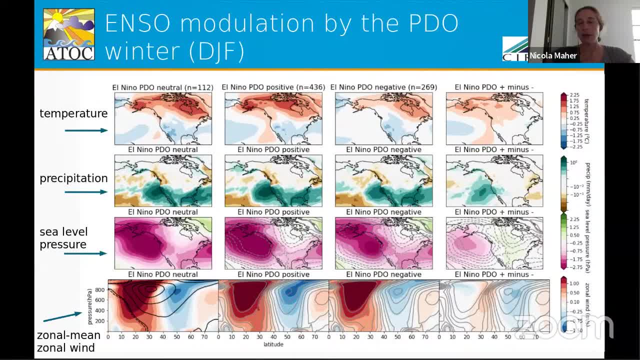 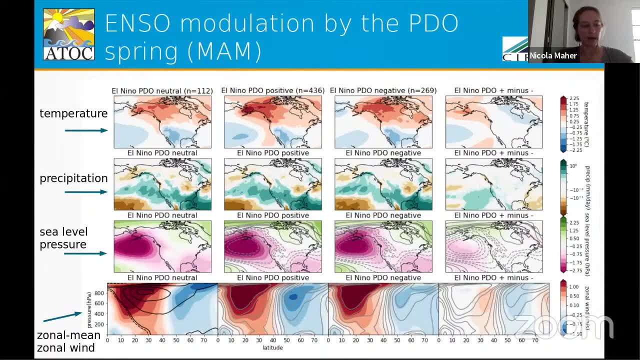 in the second row. OK, So the next question we can ask is: does this modulation continue into the spring? And I'm showing exactly the same figure here, but now for March, April, May, And you can see particularly if you. 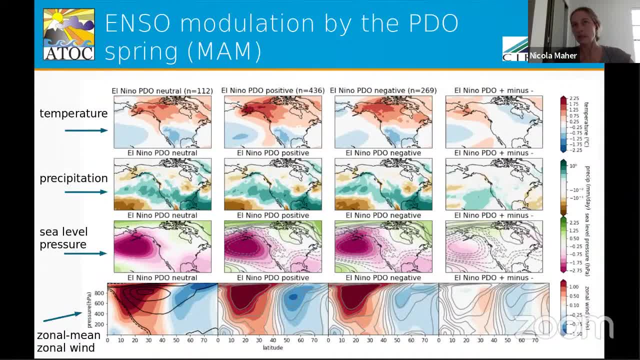 focus on the panels to the right, that there is some persistence into this season, but it's a lot weaker. I will note that if you use a different model- the GFDL, SPM, MED model- you see a stronger persistence into spring. 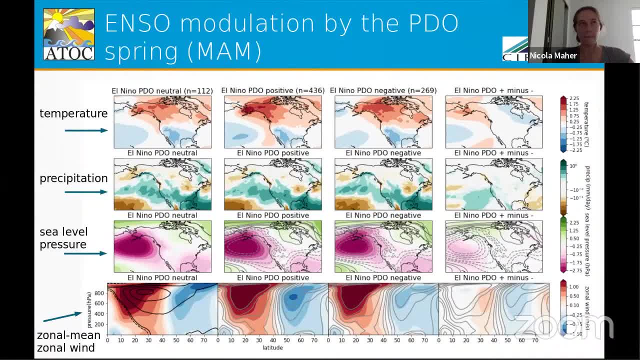 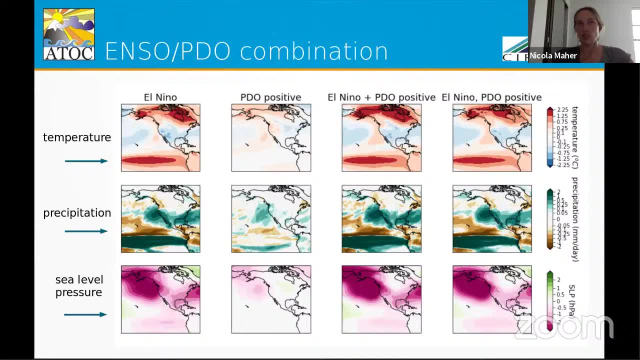 than you do with the CSM Large Ensemble. OK, So what's going on here? Is this some kind of superposition of modes, or are we just seeing a linear combination of ENSO and the PDO? So here again I show temperature precipitation. 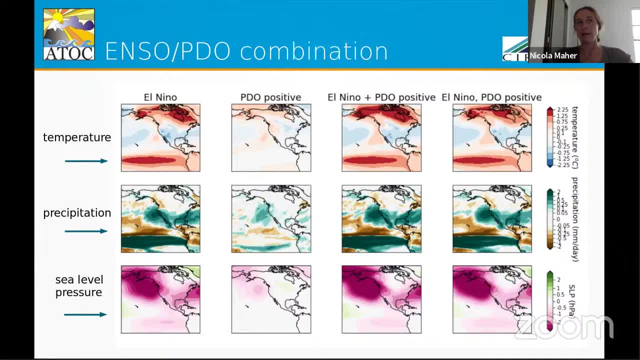 and sea level pressure. On the far left we show El Nino composites when the PDO is neutral And in the second column it showed PDO composites- positive composites- when ENSO is neutral And you can see that the PDO effect is. 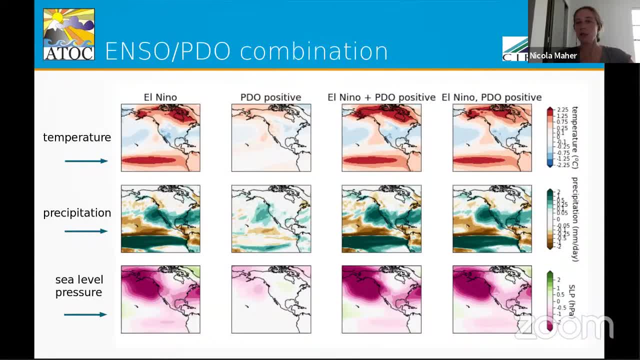 much less strong than El Nino And it's really cool to use Large Ensembles here because we can really separate out the two modes. In the third column we just show addition of the first two columns. So this is El Nino plus the PDO positive. 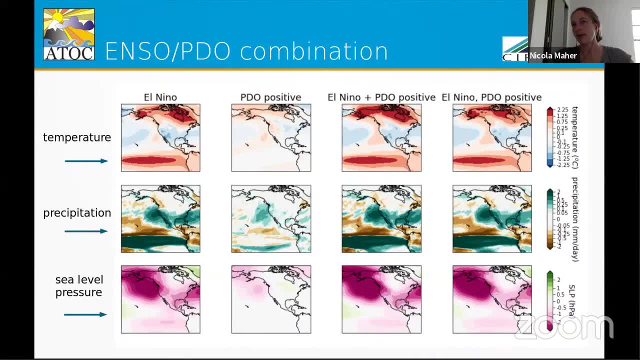 And in the last column I show the co-occurring events And if you compare those last two columns, you can really see that most of what we're seeing is just a simple addition of the El Nino when the PDO is neutral and the PDO positive. 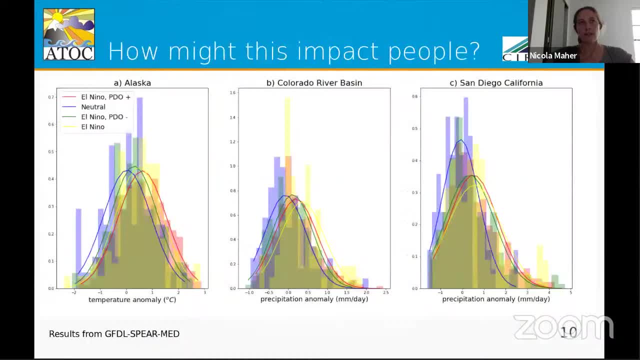 So we can see that the PDO is neutral when El Nino is neutral. OK, So how might this impact people? So, instead of showing composites here, I'm showing regions And you're looking at the whole distribution of all of the events within the ensemble. 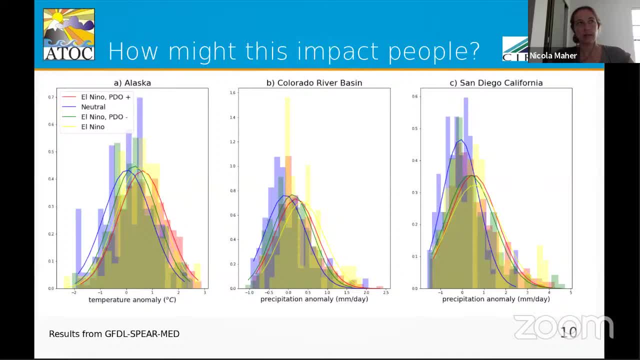 On the far left I show Alaska for temperature And here you can see the probability density function for: blue when we have neutral, neutral thanks. yellow when there's El Nino. Green when El Nino is co-occurring with a PDO negative. 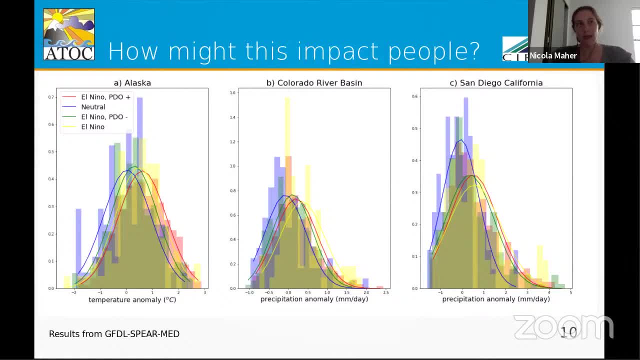 and red when El Nino is occurring with a PDO positive. And you can see here that, compared to the neutral, neutral distribution, the temperatures over Alaska are a little bit warmer when you have an El Nino, And then that effect is slightly larger. 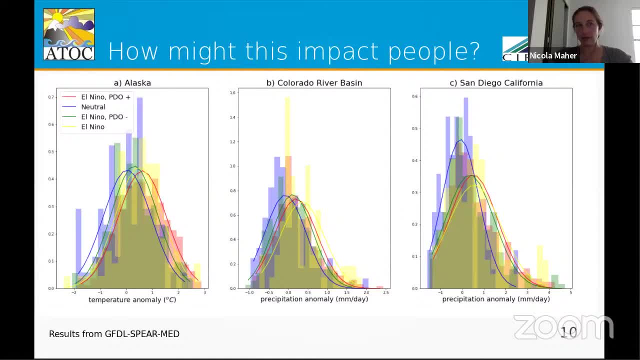 when the PDO is positive and slightly less large when the PDO is negative. However, you can see that the majority of events are all over the place And you could, for any individual event, you could observe a whole bunch of things, And this is just to show you that. 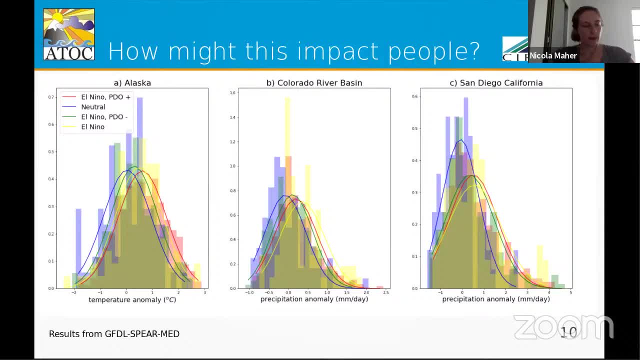 OK, And this is really kind of like a mean effect. The middle column shows the same thing for the Colorado River Basin And this is precipitation anomalies now, And here you can see that not much is going on. There is potentially a small effect of El Ninos. 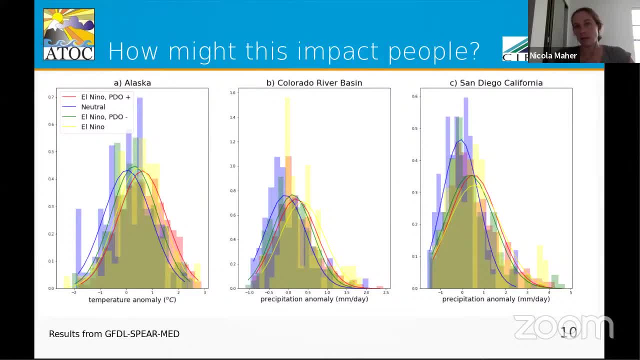 compared to the neutral phase. But the PDO doesn't really seem to be having much of an effect. And finally, if you look at the San Diego, California again, precipitation on the far right, you can see that the strong effect of that precipitation. 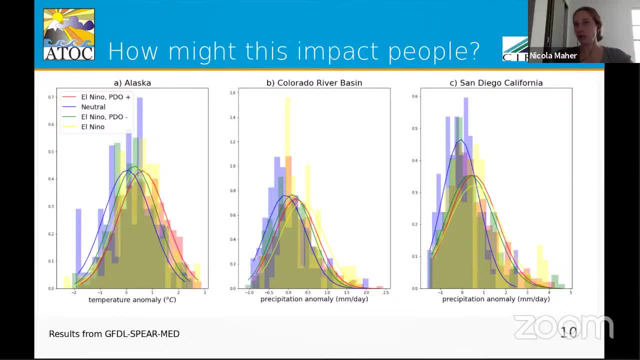 is pretty low And you can see that the distribution is definitely changed by an El Nino event. But you can also see that if there is an effect of the PDO it's pretty low by that clustering of the green, red and yellow. 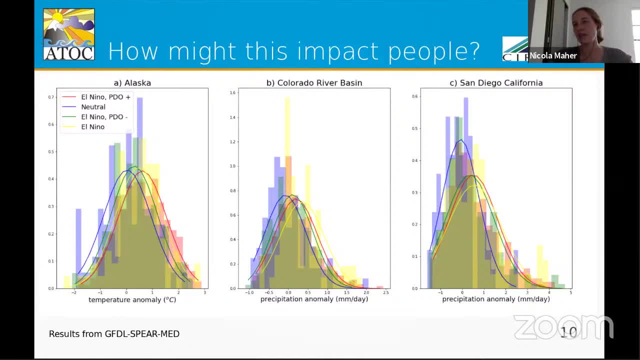 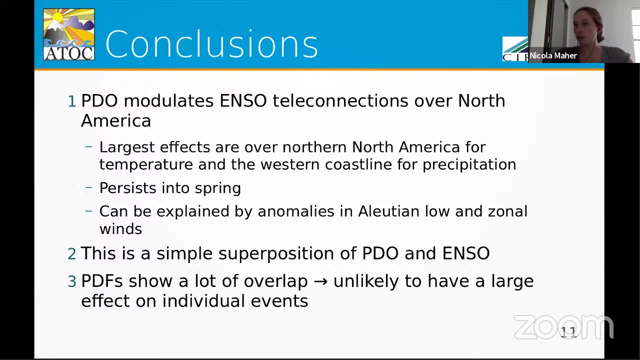 OK, So what have we found? We've found that the PDO does modulate ENSO teleconnections over North America And the largest effects are for temperature over Northern North America and precipitation on the Western coastline. We've found that the PDO does modulate ENSO teleconnections over North America. 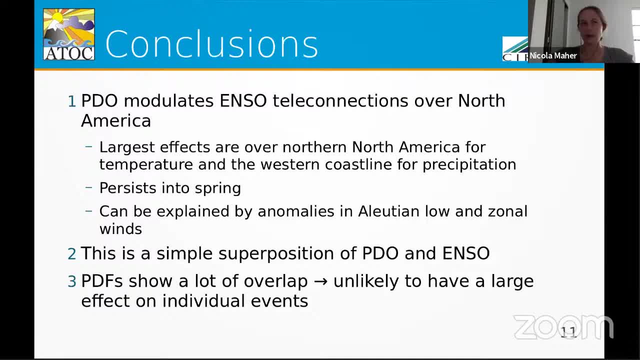 So we find some persistence into spring, but this is somewhat model-dependent by how strong this is, And most of what we're seeing can be explained by anomalies in the Aleutian Low and the zonal mean and zonal winds. This effect is really also just a simple superposition of the PDO and ENSO in the models. 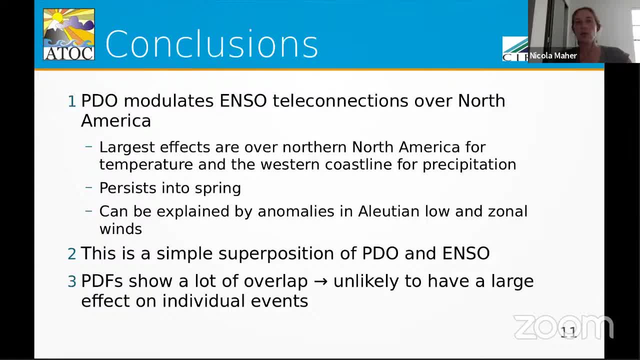 And finally, if we look at the probability density functions, they show a lot of overlap. And so if you were looking at an individual event and saying, hey, we know the PDO is in this phase and we have an El Nino, that's unlikely to be able to predict the effect. 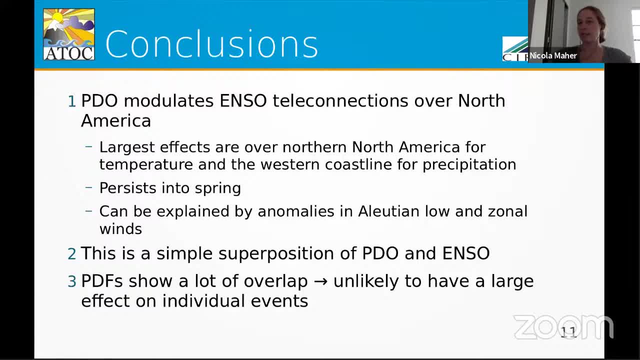 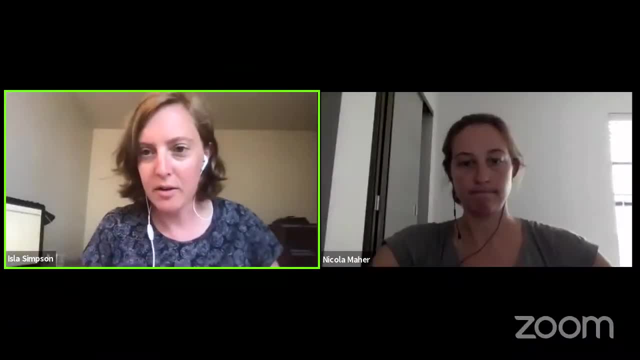 So we've found that the PDO does modulate ENSO teleconnections over North America and the Zonal means likely to be able to predict exactly what we're going to see in any given year, Thanks. Thank you, Bethany. You can either type the questions in the chat. 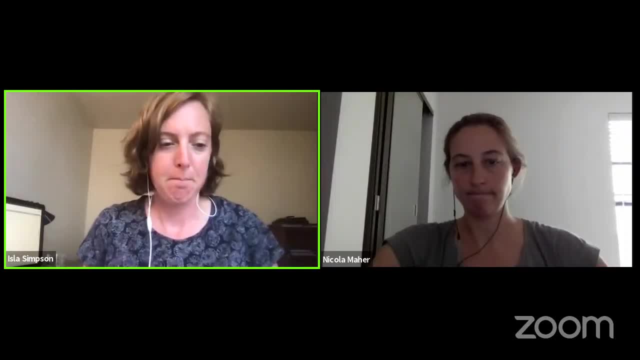 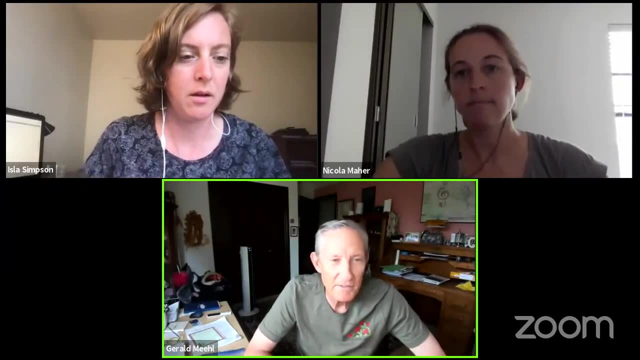 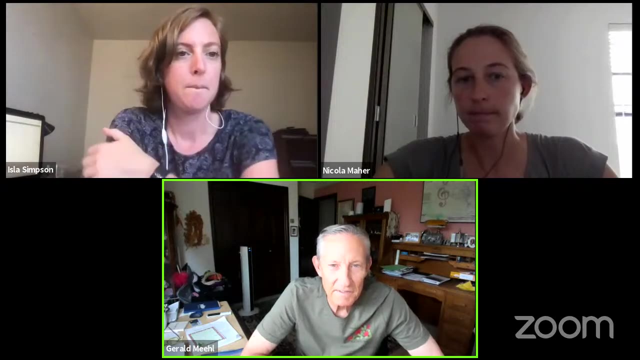 or raise your hands, Gary. Yeah, thanks, Technically that was very interesting. I'm curious: do the amplitudes of El Ninos enter into this at all, relative to the phase of the PDO? Yeah, so we haven't actually looked into that. 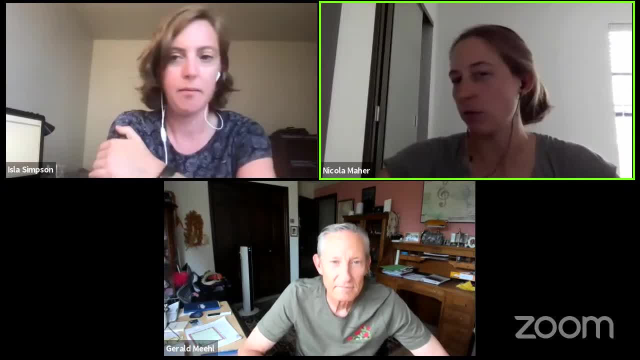 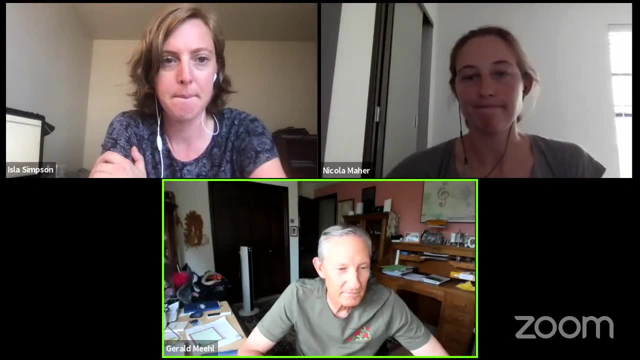 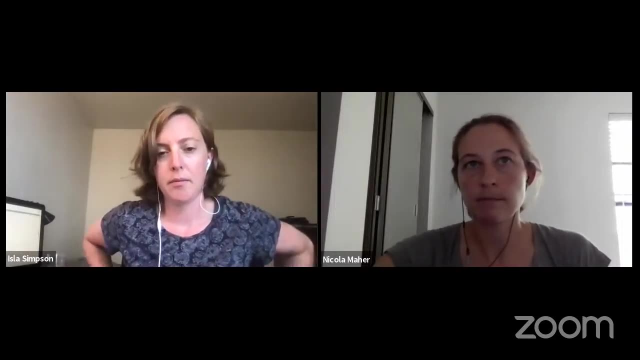 It's really just clustering of everything at this point, So we could kind of separate into multiple amplitudes. But yeah, I haven't looked at that. OK, thanks, Any other questions? No, OK, now let me move to the next slide. 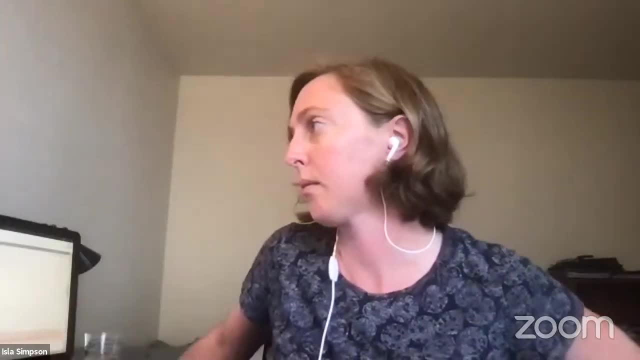 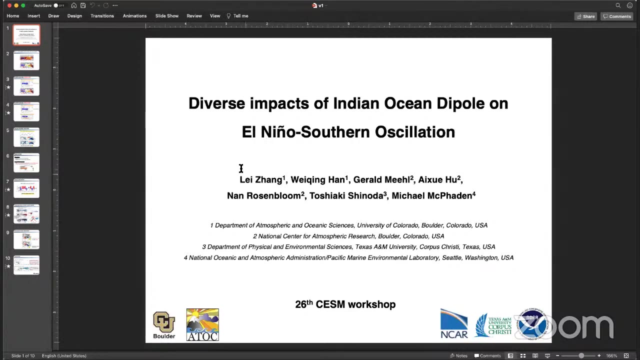 Next slide is given by Dr Lei Zhang. He will talk about Indian-Ocean dipole and ELISO. OK, Lei, go ahead. OK, thanks, Ashu. Can you see my slide and my cursor? Yes, OK, good. 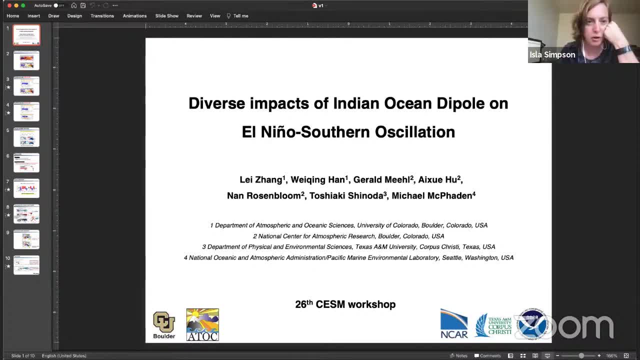 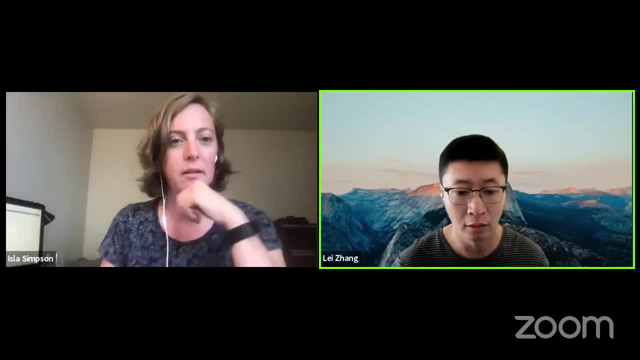 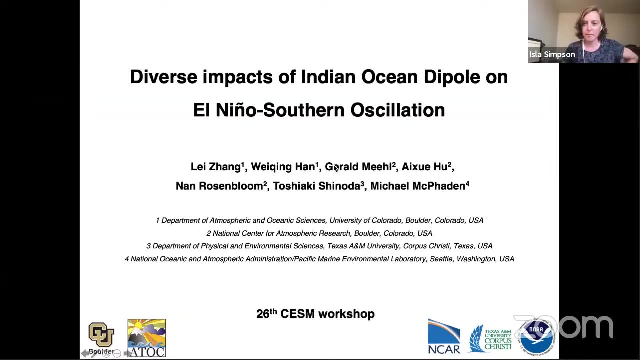 It's not full screen. Hello, Hello, Hello, Hello. I don't know if you want to view the slideshow or Oh, it is already full screen. Maybe I can try it again. How about now? That's better OK. 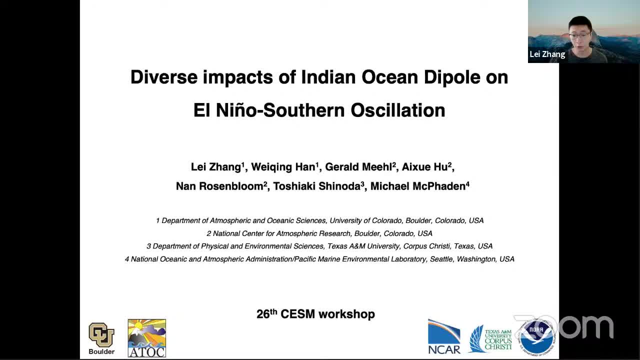 So hello everyone. My name is Lei Zhang and I am a research associate working at the University of Colorado, Boulder. Here are the collaborators of this work. In this study, we analyzed the impact of Indian-Ocean dive dipole on El Nino's southern oscillation. 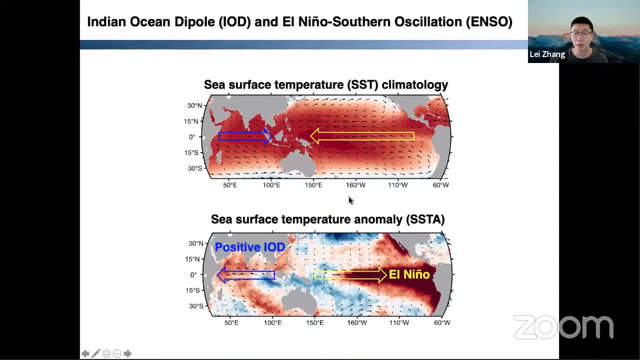 So IOD and ENSO are the two dominant inter-annual climate modes in the tropical Indo-Pacific region. Climatologically, the sea surface temperature is highest in the Indo-Pacific warm pool region, which drives large-scale winds converging toward here. 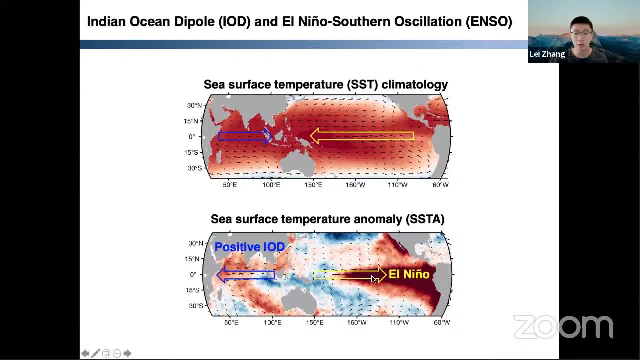 But during El Nino, the Pacific water escalation is weakened, accompanied by subspense anomalies over the maritime continent. Similarly, during positive Indian-Ocean dipole, there are weakened Indian-Ocean water circulation, as well as dry anomalies in this region. 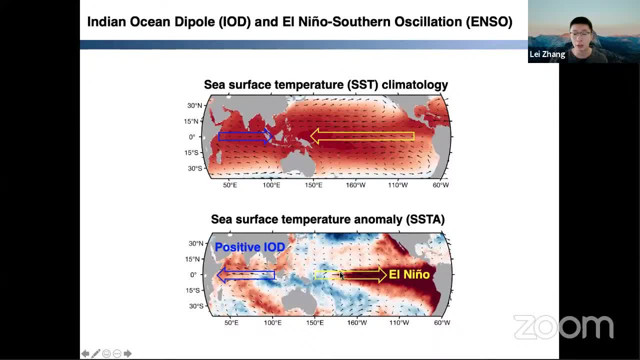 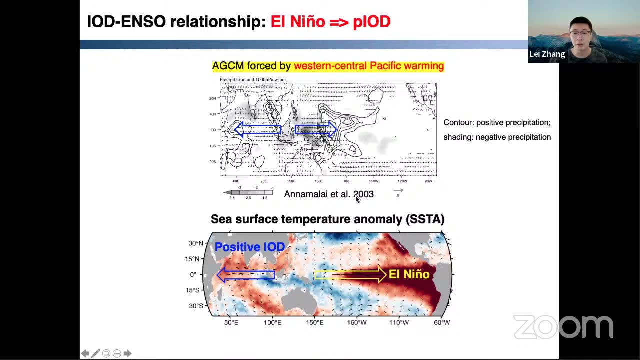 So the positive IOD and El Nino are associated with similar rainfall and circulation anomalies And naturally, people have found that these two can closely interact with each other. For example, a study by Anamela et al in 2003 found that when they forced an atmospheric model which of 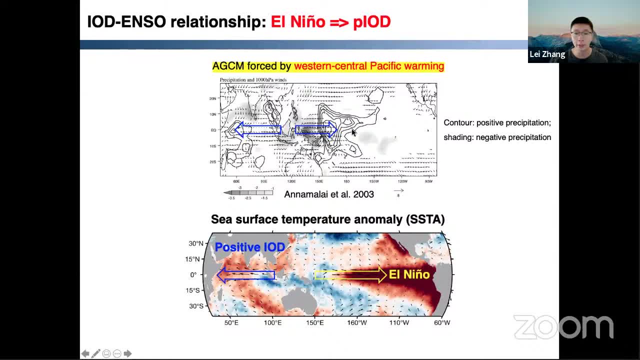 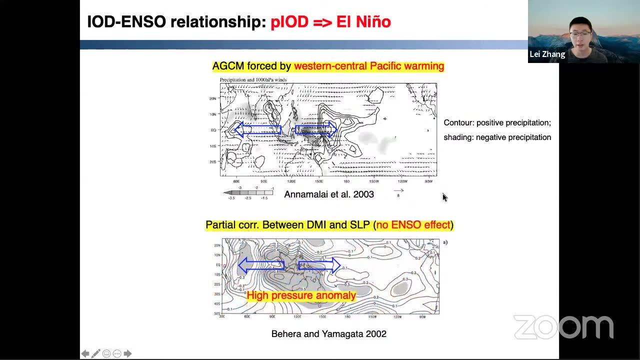 course, is the most effective model. with central and western Pacific warming, they find easterly wind anomalies over the tropical Indian Ocean. So this result suggests that El Nino can contribute to development of positive Indian-Ocean dipole. On the other hand, Bahaira and Yamagata in 2002. 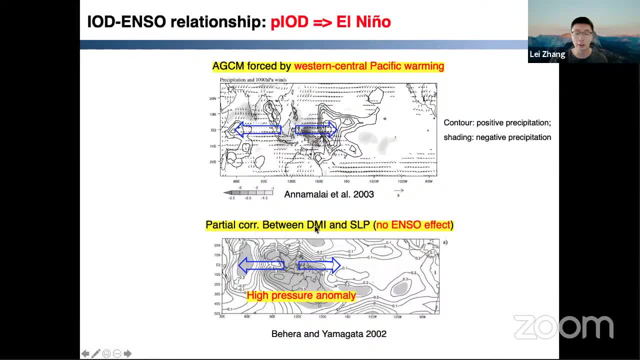 found that a partial correlation analysis between the dipole mode index and sea level pressure, with ENSO effect removed, shows higher sea level pressure. This drives westerly wind anomalies over the tropical Pacific, So this result suggests that in turn positive IOD can contribute. 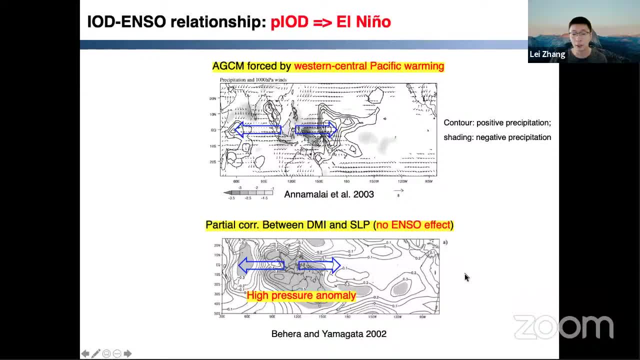 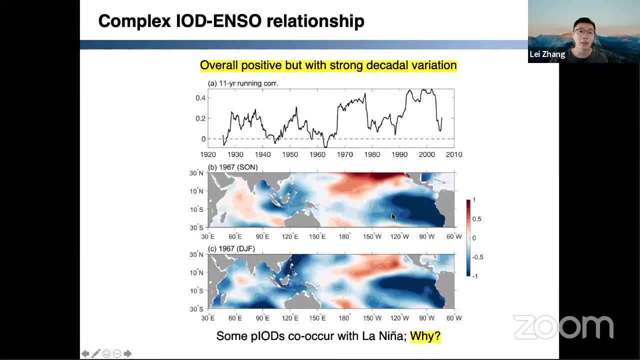 to the development of El Nino. So clearly positive. IOD and El Nino can interact and amplify each other. However, if you look at the observations, the relationship between IOD and ENSO is a little bit more complex. So you can see that the relationship between IOD and ENSO is a little bit more complex. 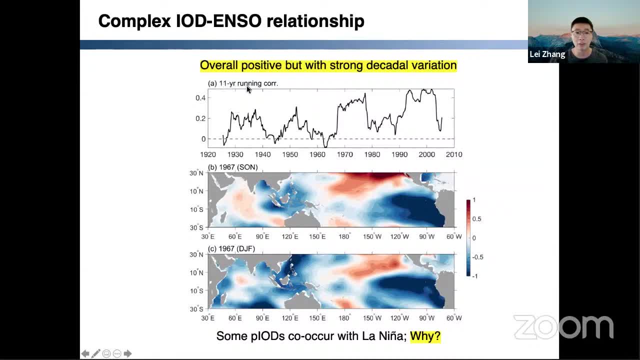 However, if you look at the observations, the relationship between IOD and ENSO is a little bit more complex, complicated than that. If you look at the 11 year running correlation between the two modes, you can clearly see this very strong decadal variation in the correlation, Although it is. 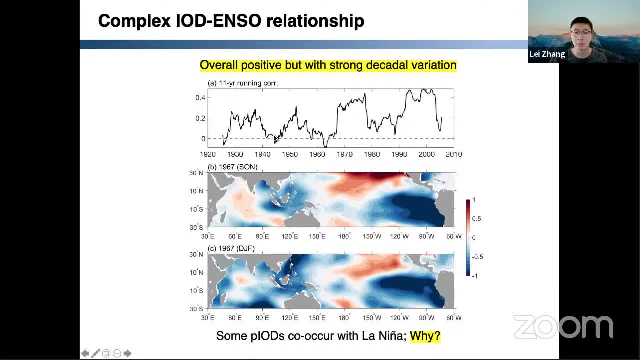 overall positive. during some decades the correlation between the two is very weak and even become negative. And if you look at climate models, models tend to show similar decadal variations. For example, in 1967, the observations show that a positive Indian ocean dive hole 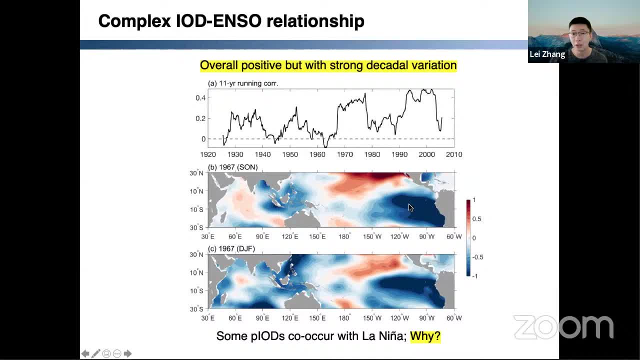 actually co-occurs with La Nina instead of El Nino. So this suggests that the relationship between IOD and ENSO is very complicated and we have not fully understood it yet, especially why some positive IODs co-occur with La Nina. In this study we focus on investigating. 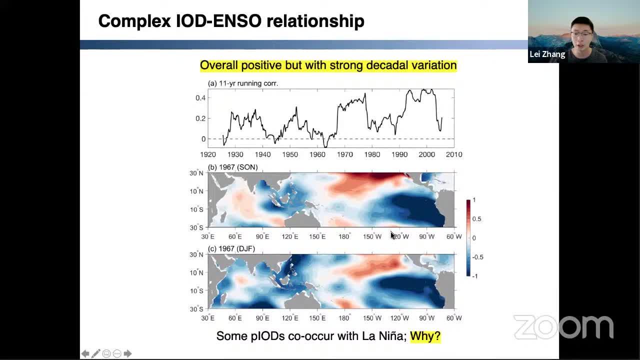 the correlation between the two modes of correlation between the two modes of correlation, impact of IOD on ENSO and hopefully our results will help us to better understand why events such as 1967 occur. So, to achieve our research goal, we analyzed observational data. 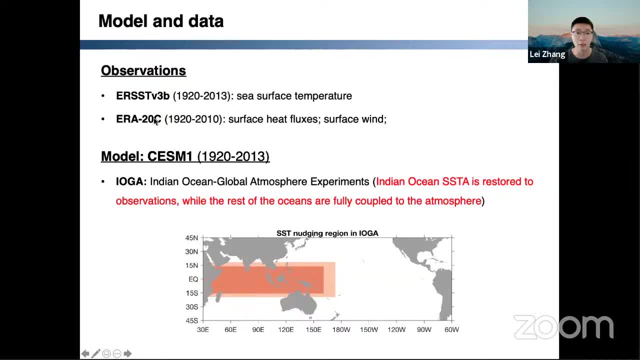 including ER-SST version 3b and ER-A20c reanalysis. In addition to that, we also performed and analyzed the so-called Indian ocean pacemaker experiments, in which we have restored Indian ocean sea surface temperature to observed values. Meanwhile, we leave the oceans fully. 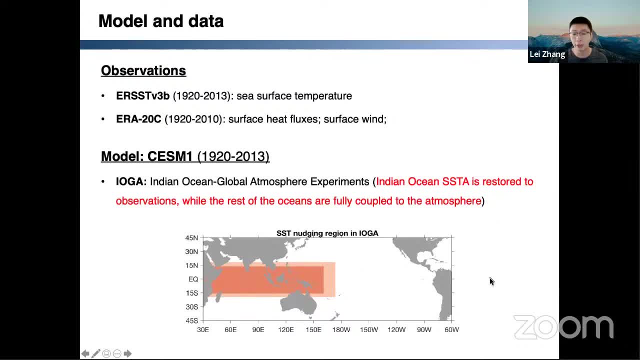 coupled to the atmosphere elsewhere, So we have 10 ensemble members. by slightly perturbing the initial conditions and ensemble averaged results, isolate the impact of the Indian ocean sea surface temperature anomalies on global climate variability, using which, in this study, we analyze the impact of IOD on ENSO. 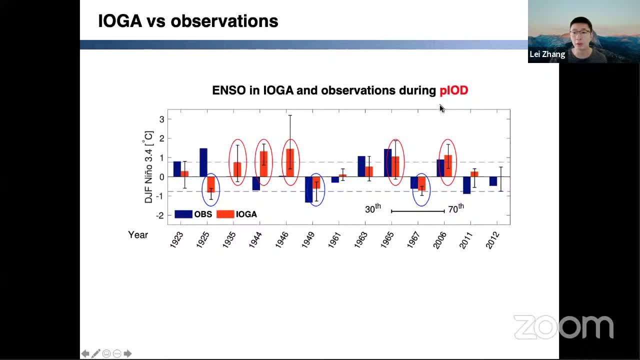 So first we selected all the observed positive IOD events, which is the x-axis, and we analyzed the DGF mean NINU 3.4 index during those years and compare observed values, which is blue, with the NINU 3.4 in the model, which is red. We find this result very interesting because 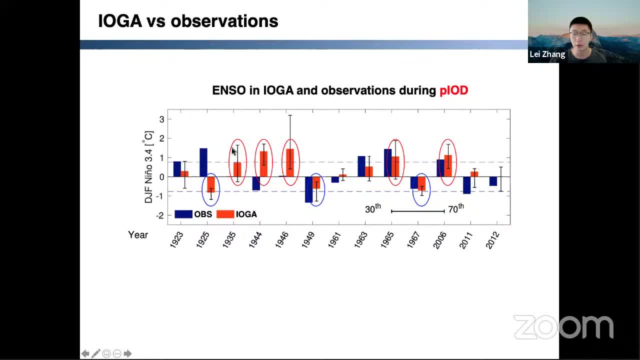 although the positive IOD tends to cause or contribute to L-NINU, because these red bars are positive, we do note that in some years, such as these three events in the model, there are L-NINU instead of L-NINU. In other words, positive IOD, indeed, can cause. 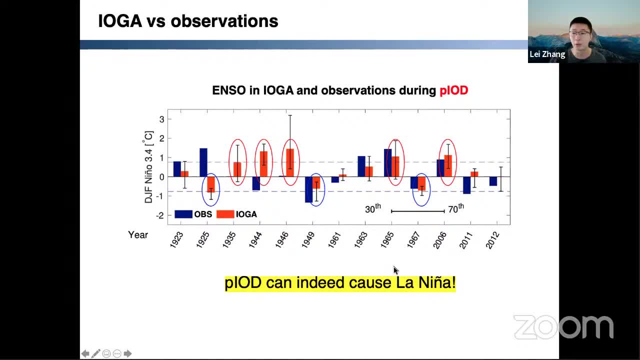 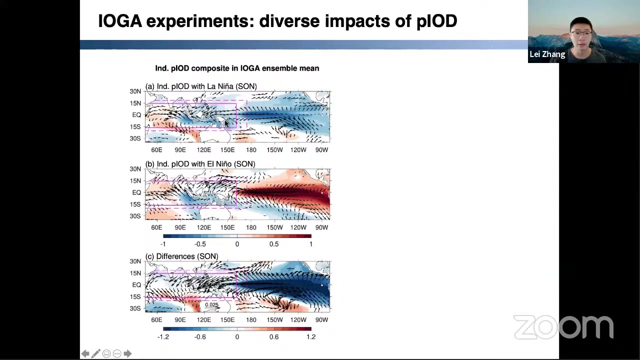 L-NINU. We find this result very intriguing and we want to understand why the positive IOD effect can be different between those two categories. So to answer this question, we performed composite analysis of these five years and these three years separately, and here is the result In the top panel. this shows the SST anomaly and the surface wind anomaly. 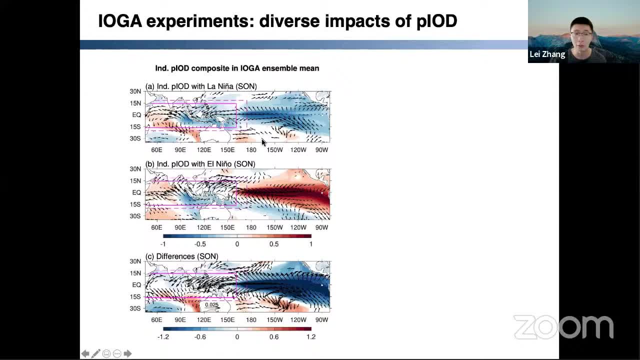 during positive IOD that causes L-NINU in the model, and the middle panel shows positive IOD that causes L-NINU, and the bottom panel shows the differences between them. We find that the largest differences for the positive IOD are located at the warm pole, For instance. 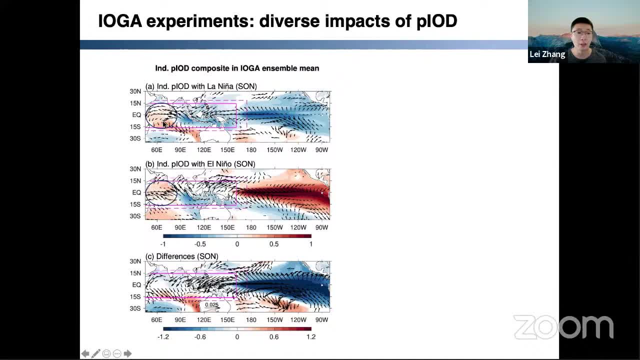 during this category, this positive IOD event, we find the largest warming located at the so-called Summer Calais Ridge region, while during this kind of positive IOD event, the largest warming is located at the Northwestern Tropical Indian Ocean. The difference between the two is even. 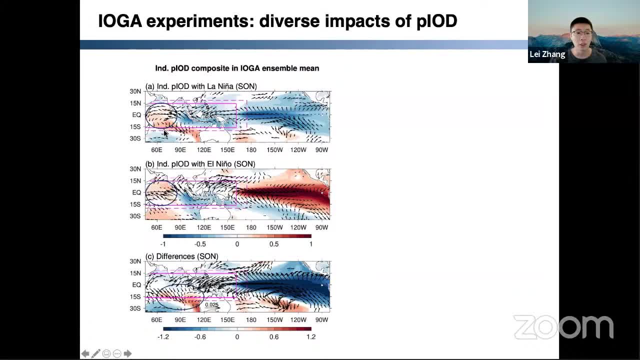 clearer if you look at the bottom panel. So the Summer Calais Ridge warming drives large-scale northerly wind anomalies, Together with easterly wind anomalies in the tropics due to the anomalous zonal SST gradient. this kind of positive IOD drives large-scale. 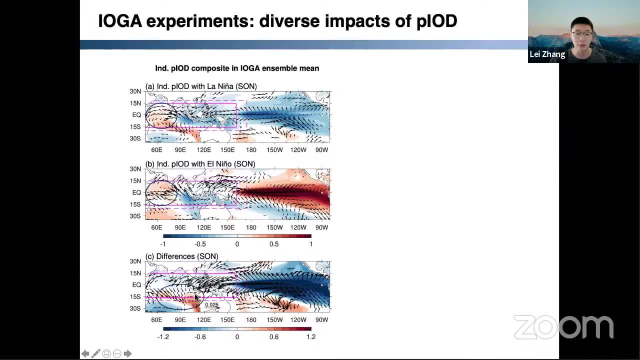 anticyclonic wind anomaly which extends to the Southeast Indian Ocean and causes northerly wind anomaly in this region. Because the background wind in this region is southerly, this wind weakens the background wind and causes SST warming of the west coast. 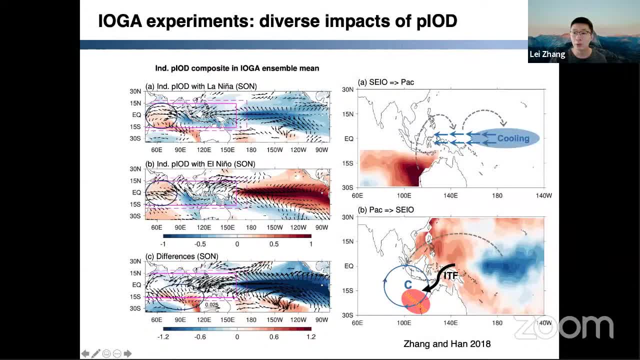 In one of our recent studies, we find that the Southeast Indian Ocean warming and the Central Pacific cooling are closely connected to each other and they can amplify each other through inter-base interactions. The Southeast Indian Ocean warming can enhance Pacific trade winds and cause cooling. Pacific cooling can contribute to Southeast Indian Ocean warming. 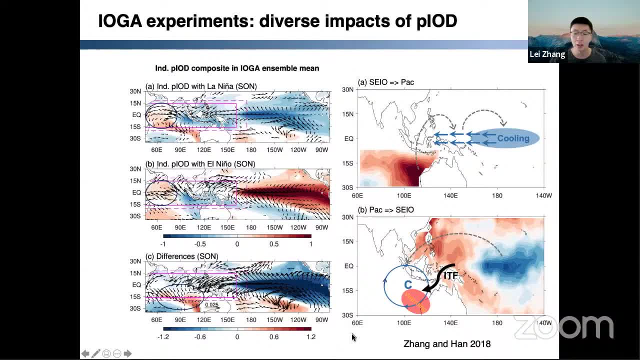 through both oceanic and atmospheric teleconnections. So these results together suggest that during this kind of positive IOD, with Summer Calais Ridge warming, it can cause Southeast Indian Ocean warming, which then, through inter-base interaction, causes Pacific cooling and therefore causes La Nina in the pacemaker experiment. 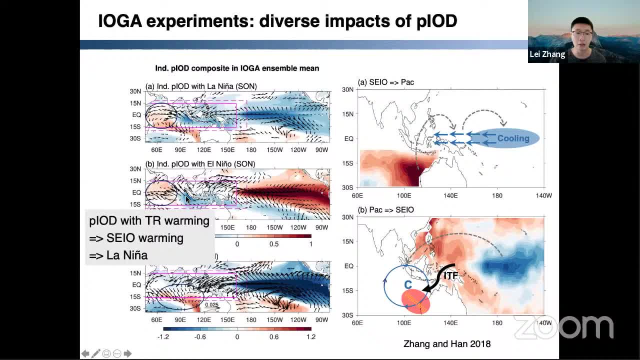 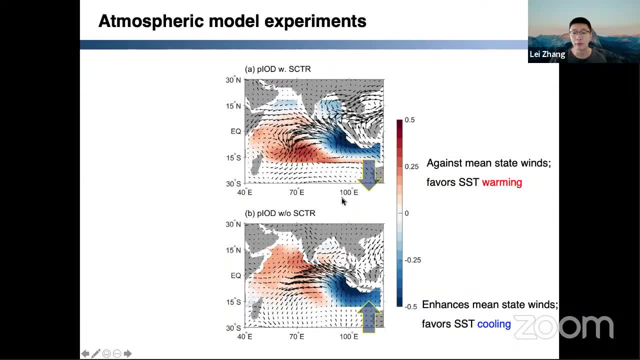 But during this kind of positive IOD, because it cannot cause Southeast Indian Ocean warming, it actually favors El Nino. To further prove our hypothesis, we performed additional atmospheric model experiments, which is forced using the two different positive IOD: SST anomaly patterns. 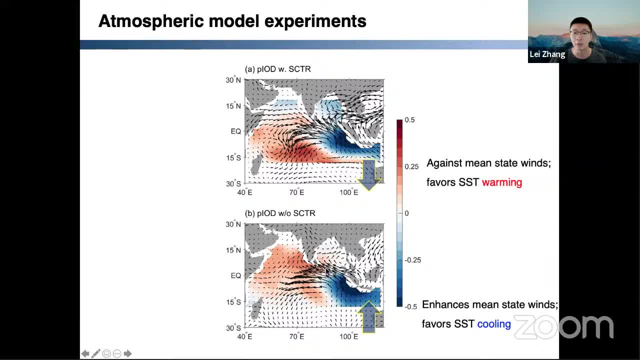 And these winds are the response to the two different SST anomaly patterns, one with Summer Calais Ridge warming and one without. Clearly, during this kind of positive IOD, the IOD can cause northerly wind anomalies here in this region. Again, it is against the mean state winds. 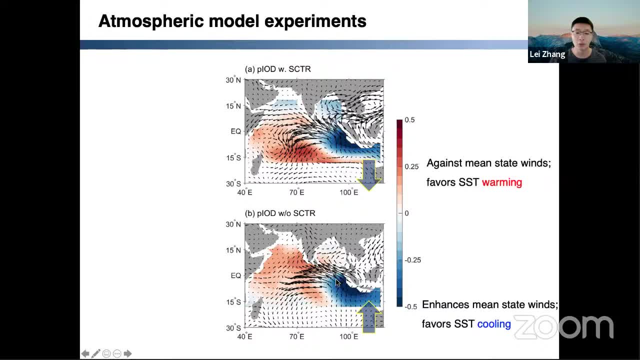 and therefore it favors El Nino. To further prove our hypothesis, we performed additional atmospheric IOD with Summer Calais Ridge warming on the Pacific Ocean with the same SST warning, but during this, But during this kind of positive IOD event- it actually causes northerly wind anomalies. 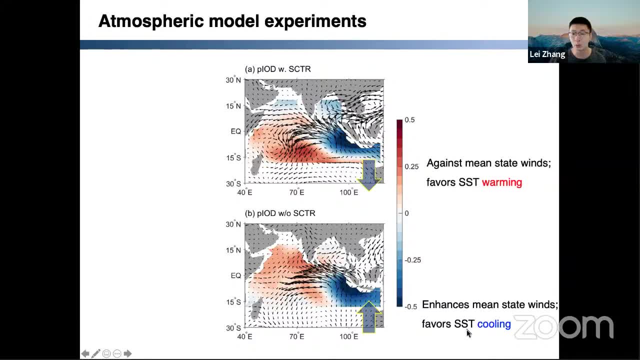 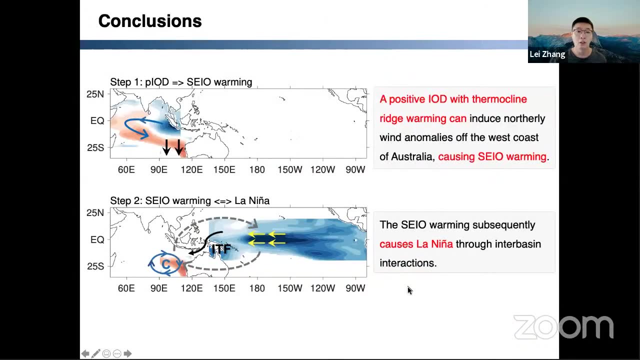 which enhances background winds and favors SST cooling. Because of this kind of different response in the Southeast Indian Ocean to the positive IOD forcing, this favors La Nina and this favors El Nino. So, to sum up, we finally found that the two of these predictions both 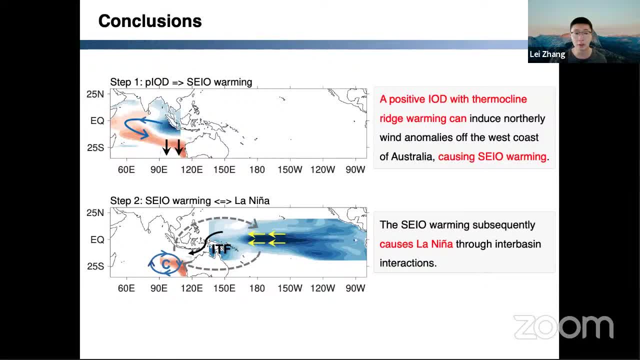 in the Pacific Ocean and the Pacific Ocean are very similar in their properties, But in the We find that a positive IOD not only contributes to El Niño but it can also contribute to La Niña under some circumstances. In particular, we find that a positive IOD with some kind of heat warming can induce northerly wind anomalies off the west coast of Australia, causing southeast Indian Ocean warming. 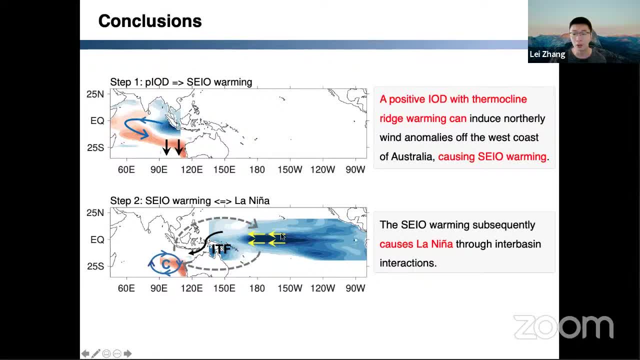 And this warming can further cause Pacific cooling or La Niña through interbasin interactions. This result actually explains why events such as 1967, when a positive IOD co-occurs La Niña- happened in the past, And our results also suggest that future studies that focus on IOD-enso relationship should take into consideration the detailed SST anomaly pattern of the IOD. 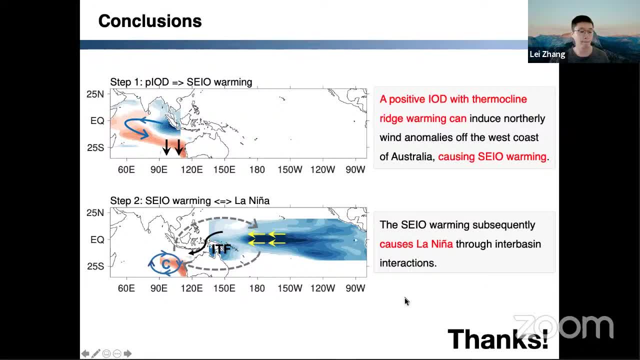 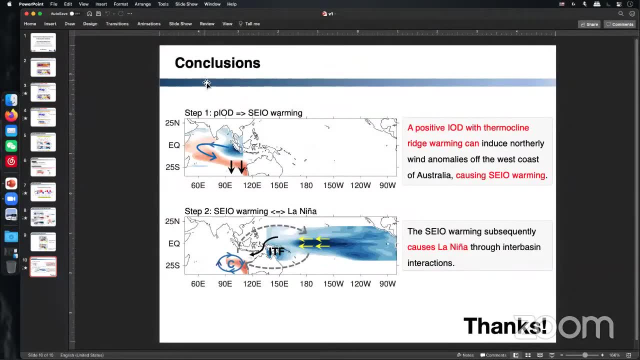 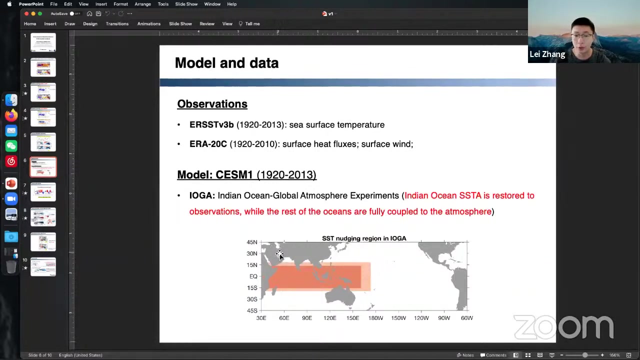 That is all. Thanks for your attention. Thank you Questions. I was just wondering: in your pacemaker experiments did you have all other forcings evolving And did you kind of take that into account somehow? Yeah, So in the pacemaker experiment we used a historical forcing plus RCP 8.5 for 1920 to 2005 and 2006 to 2019.. 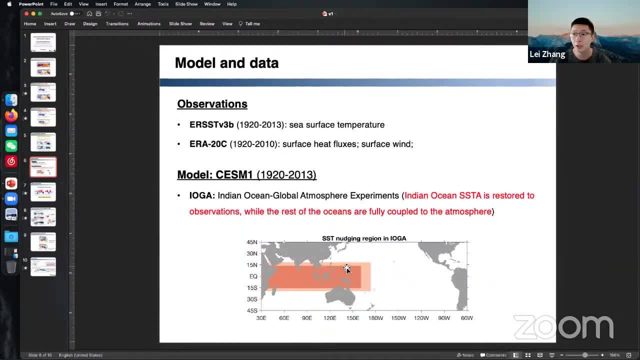 We removed a linear trend in our results. We also tried to remove the regression Okay And we also tried to remove the regression to the global mean surface temperature, And both gave us very similar results. So we think that external forcing may not play a major role here. 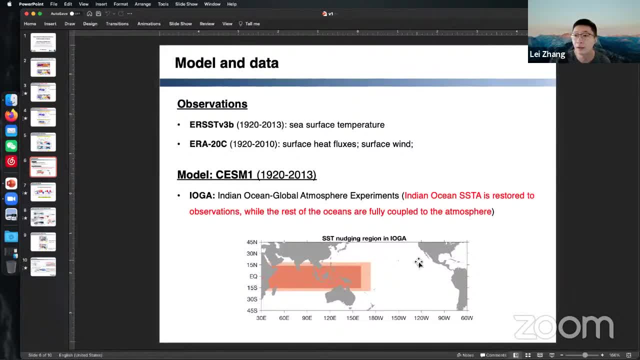 Thanks, Lei. This was a very nice study. So one question I have. So you have taken a very Western, Pacific centric view on this. Did you also look in those specific years when you had the La Niña in conjunction with IOD? 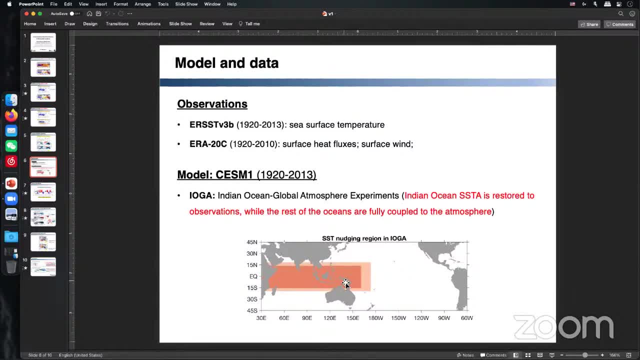 Positive IOD. Did you also look at the state of the tropical Pacific and other possible extratropical influences on the Pacific itself? Okay, Yeah, So I guess the question is because we include a part of the Western Pacific perhaps in the model, this can influence the ENSO. 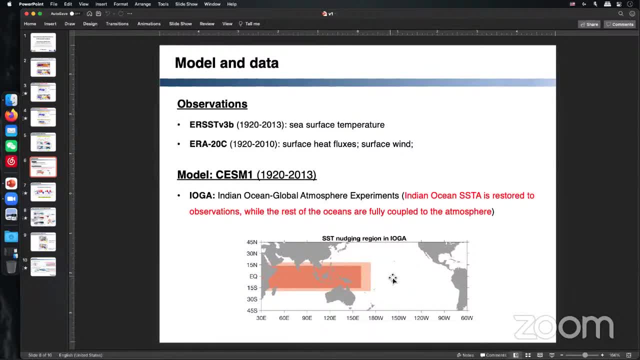 Well, I think ENSO is not. It's also forced by large numbers of people, It's also forced by large scale influences. And so you know, for the Indian Ocean to affect the Pacific, the Pacific needs to be in a proper state. 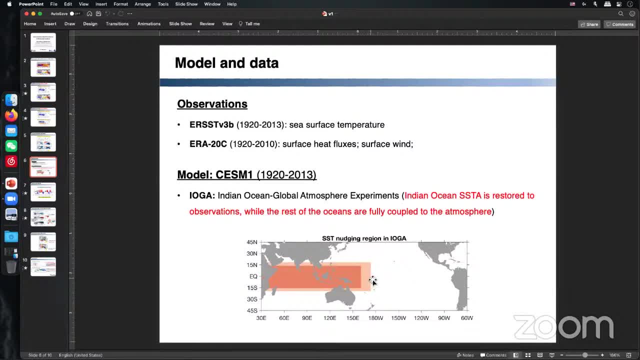 And maybe, like meridional modes or other extratropical influences, need to be, you know, conducive to the evolution of the system. So I was wondering if, in those particular years, you also looked at the larger scale conditions. Yeah, Yeah, That's a good question. 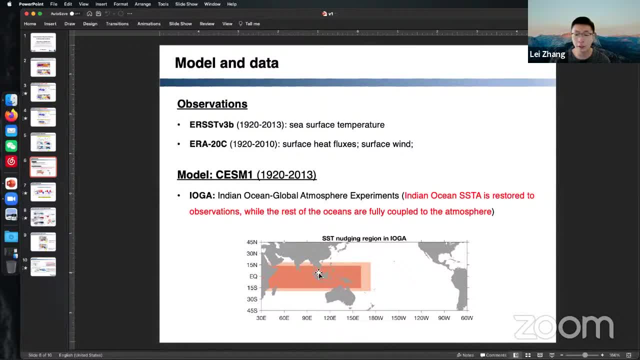 So Because we are analyzing the Indian Ocean pacemaker experiments and the ensemble average results are mostly due to the Indian Ocean forcing. But I agree with you, It could be. It is also possible that Indian Ocean may affect some other regions and then affect the Pacific. 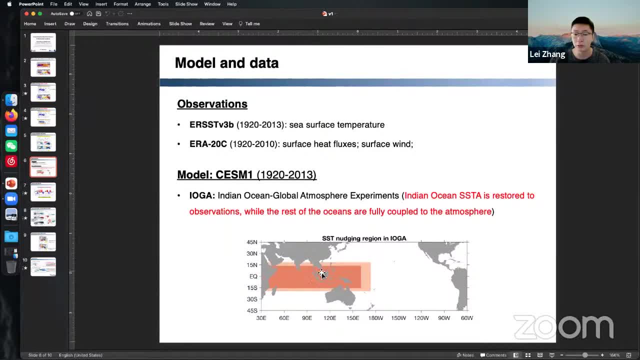 In other words, there may be another pathway through this instead of just the Southeast Indian Ocean, But we haven't looked at that yet. But we can look at that, But we can look at it in the future. Thanks, Now we move on to the next stop. 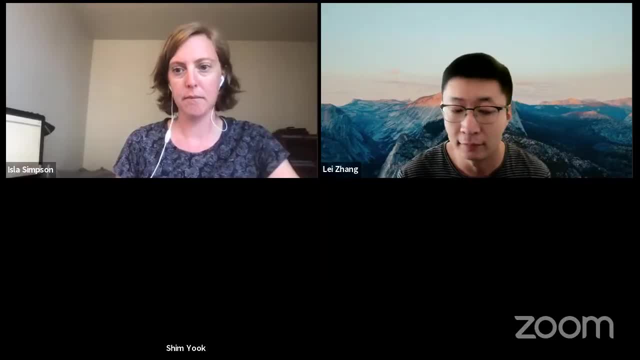 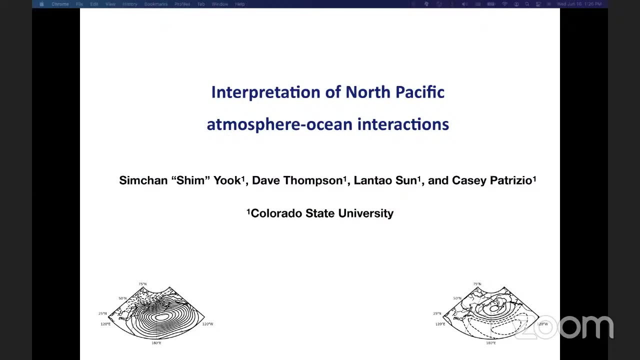 You will think by. So talk about the interaction. All right, Can you see my screen? Yep, Thank you. So my name is Shim Yu. I'm a PhD student at Colorado State University. Today, I'm going to be talking about the work that I've been doing recently, along with 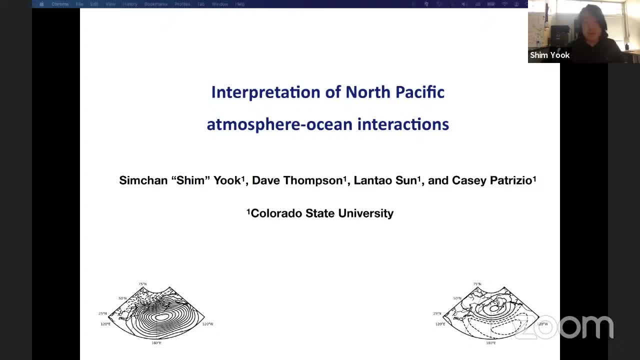 my advisor, Dave Thompson, and other collaborators at CSU, and also with Casey Patricio. So I'm looking at atmospheric response to extra-tropical SST variability over the West China Sea Pacific using a set of simulations run on the CSM. 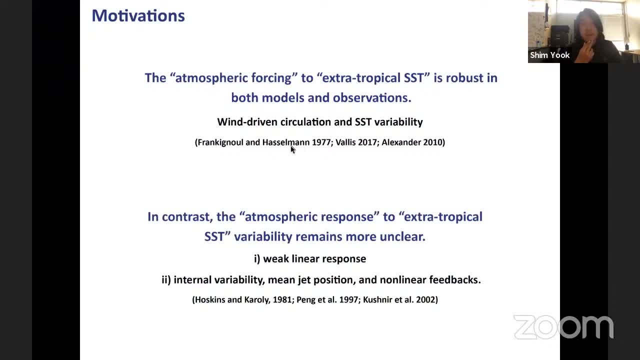 So I'm going to start with providing some background and motivations for this study. It is clear that atmospheric circulation can influence the extra-tropical SST variability through the surface heat fluxes and surface wind stresses. However, the atmospheric response to extra-tropical SST variability is relatively subtle. 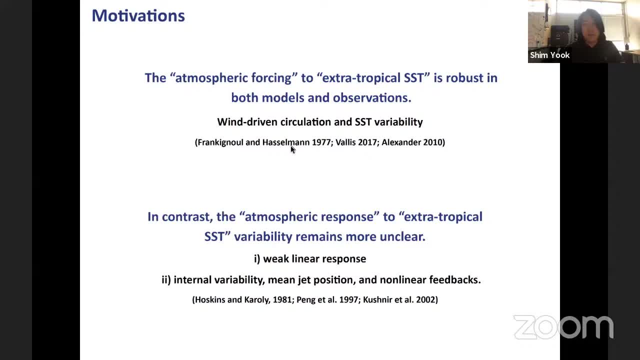 The linear theories predict that any surface heat flux anomalies in the mid-latitude can be easily balanced by small changes in the surface heat flux, For example changes in low-level circulation due to relatively strong horizontal temperature gradient in the mid-latitude. And the atmospheric response in the mid-latitude is even more complicated because of the strong 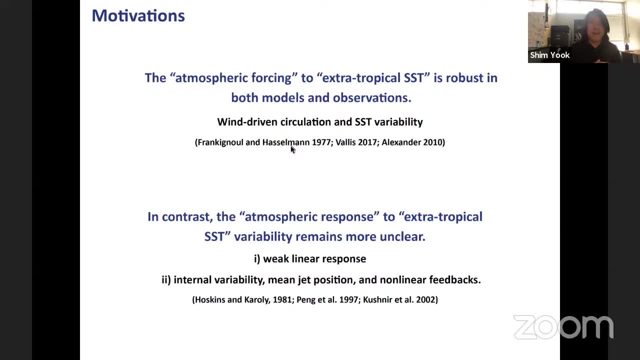 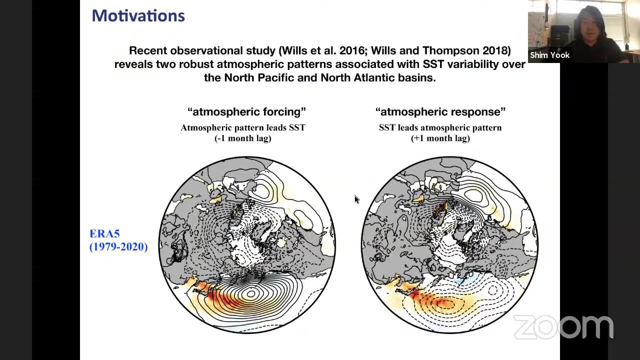 internal variability and the dependence of atmospheric response to mean jet position and nonlinear feedbacks from extra-tropical edges. Thus, theoretically, the atmospheric response to extra-tropical SST variability is much more difficult to isolate and quantify. Nevertheless, a growing body of evidence suggests that the extra-tropical SST can play 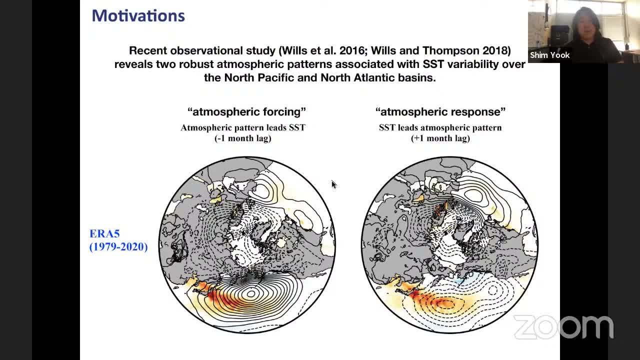 an active role in atmospheric circulation. The recent observational study has suggested two robust patterns of atmospheric circulation that are associated with the SST variability over the North Pacific and North Atlantic basins. In this study, we focused on the North Pacific sector only. If you look at the plot on your left, there are high sea-level pressure anomalies that 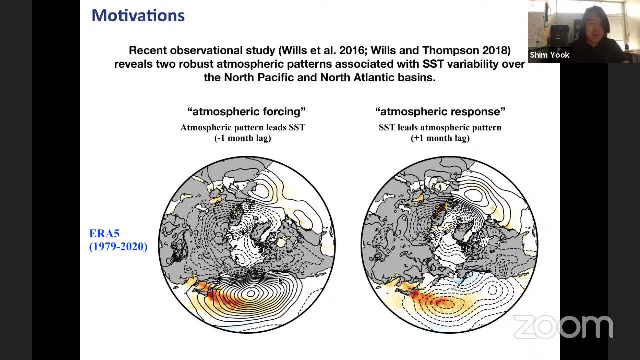 span much of the North Pacific basin and these high-pressure anomalies peak a month before the SST anomalies And it is associated with the northward warm-temperature advection. Thus this pattern is consistent with the atmospheric forcing of the SST And if you look at the plot on your right, there are low sea-level pressure anomalies. 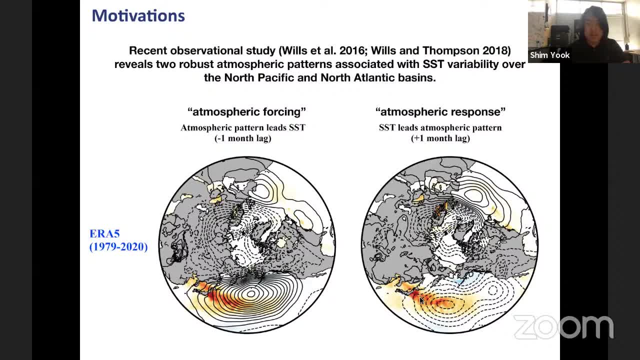 that extend downstream. And if you look at the plot on your left, there are low sea-level pressure anomalies that extend downstream. And if you look at the plot on your right, there are low sea-level pressure anomalies that extend downstream, And this is associated with the southward cold advection. 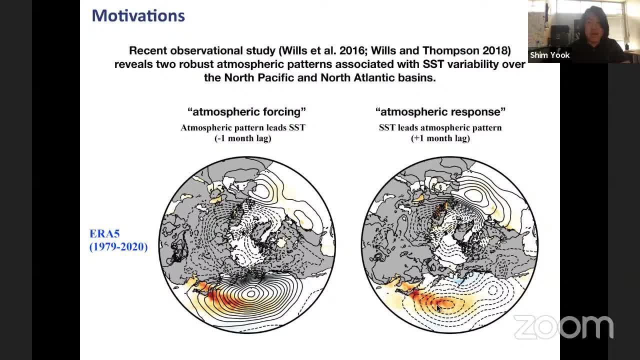 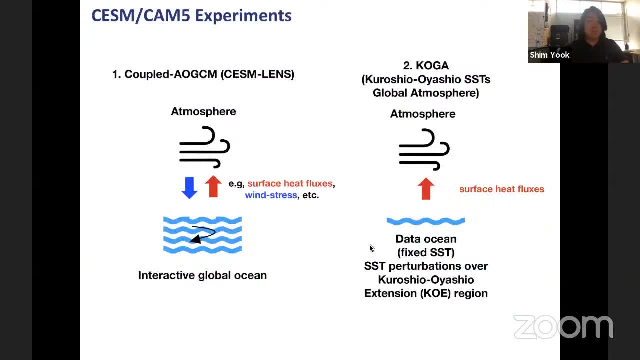 Thus this pattern is consistent with the atmospheric response to cooling of the SST. So in order to test the observed VLAG relationships between the extra-tropical atmospheric circulation and SST variability, we assessed experiments run on two different configurations of the CSM. The first type of simulation is the fully-coupled AO-GCM, which the atmosphere model is coupled. 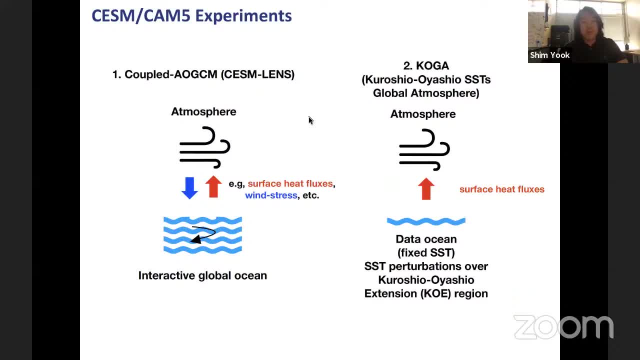 to a fully-active ocean, with SST evolving by internal physics of the ocean model. So here we can assume that both two-way feedbacks between the atmosphere and ocean are included in the coupled simulation And the second one is a pre-scribed SST experiment, which is an atmosphere model simulation. 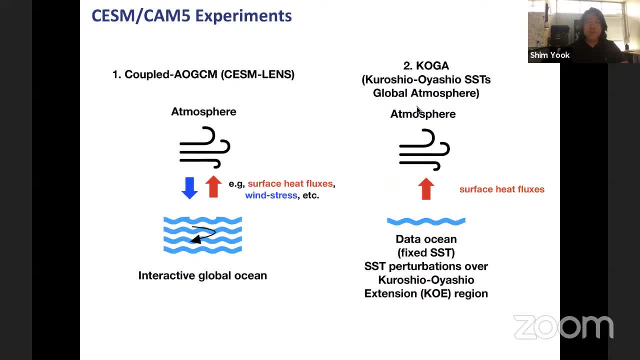 forced by data ocean. So we looked at the two-way feedbacks. So we looked at the two-way feedbacks. We referred to covalent, denoting crocio-oyashio SSTs and global atmosphere simulation. Here the simulation is forced by time-varying historical SSTs over the western North Pacific. 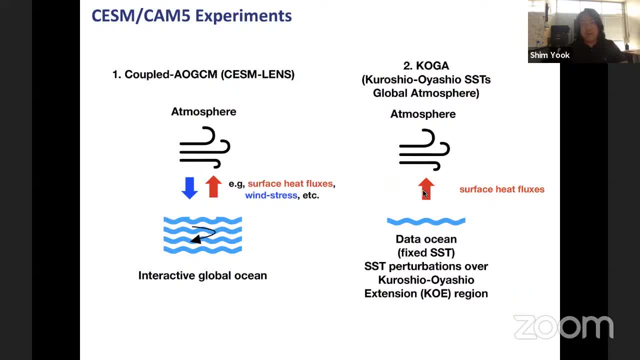 and also with annually repeating climatological seasonal cycle over all other regions. So if you think about the coupling between data, ocean and atmospheric circulation, you'd expect the atmospheric response to the SST forcing but not the atmospheric forcing over the SST, because SST fields are given by the data and it's fixed. 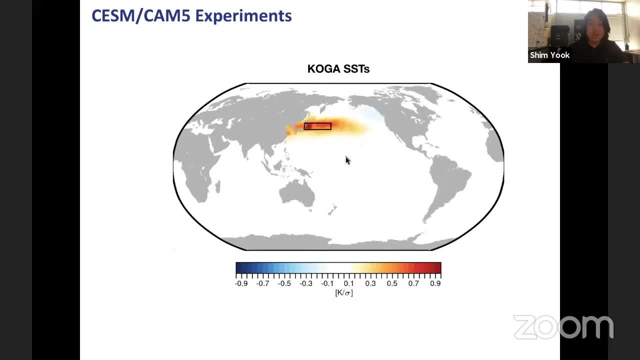 So this shows the pattern of SST anomalies that used to force the COGA simulations. So you can see the largest SST anomalies are focused on the crocio-oyashio extension region and set to be zero elsewhere. So there is no tropical forcing, as well as high latitude forcings. 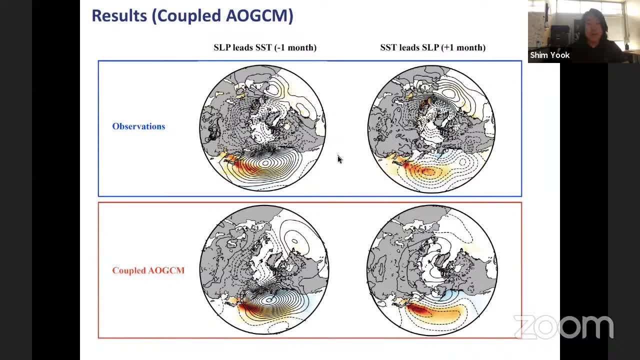 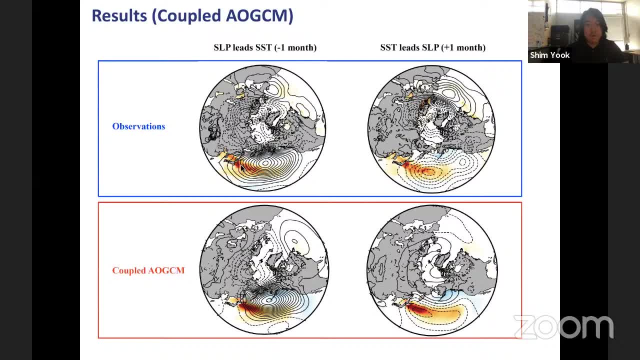 So here again you can see the regressions of SLPs. So here again you can see the regressions of SLPs And you can see the SST and SST regressed onto the SST average over this crocio-oyashio. 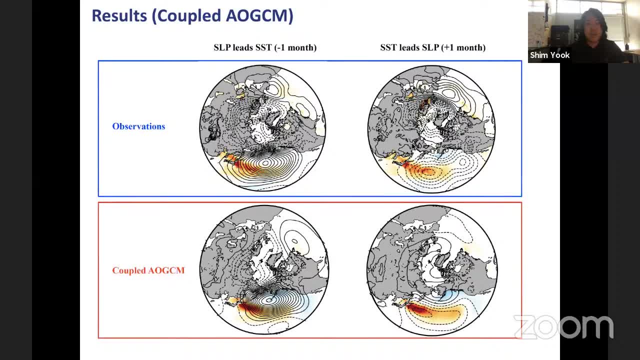 extension region And the upper panels in the blue box are actually the plots that I've shown before. So these are the results from the ERA5, so you can kind of work as reference. And the left column shows the negative lag which shows atmospheric circulation pattern. 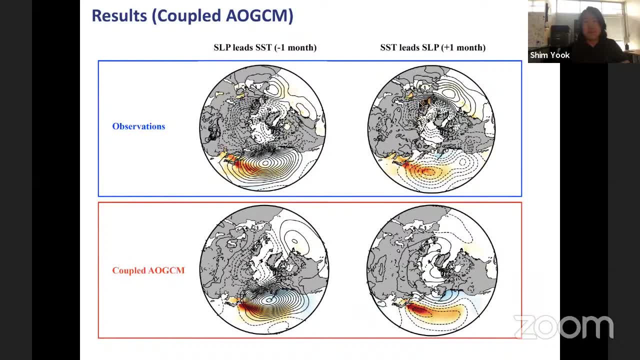 prior to the peak of the SST anomalies. And the right column shows the positive lag, which shows the negative lag, And the right column shows the positive lag, which is the case for SST is leading the atmospheric circulation pattern. So just to reveal there is anticyclonic anomalies at negative lag is associated with the lower. 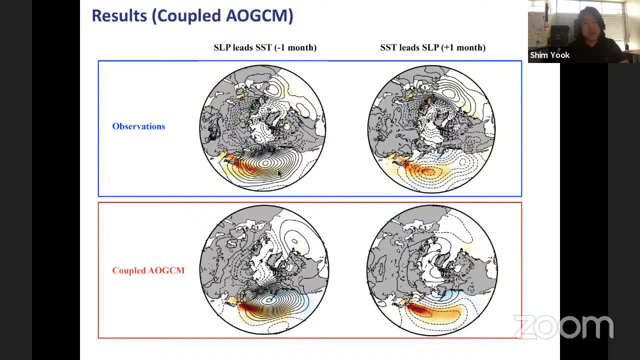 temperature of the reaction And this pattern is consistent with the atmospheric forcing of the SST. And if you look at the upper right, there are low sea level pressure anomalies. that lags the peak of the SST anomaly by a month And it is consistent with the atmospheric response to SST. 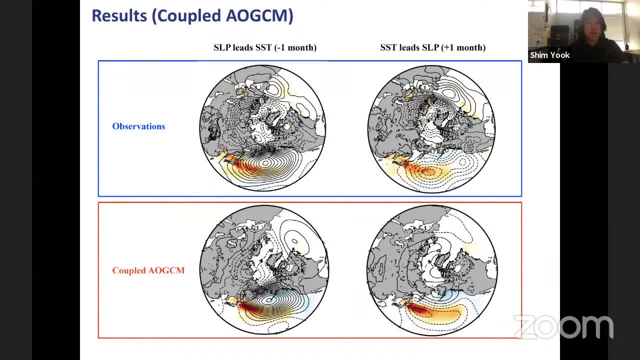 And it is consistent with the atmospheric force of the SST, the cooling of the SSTs. So the lower panels in the red box are the results from the coupled AOGCM. So if you compare the upper panels and the lower panels, you can see the results from. 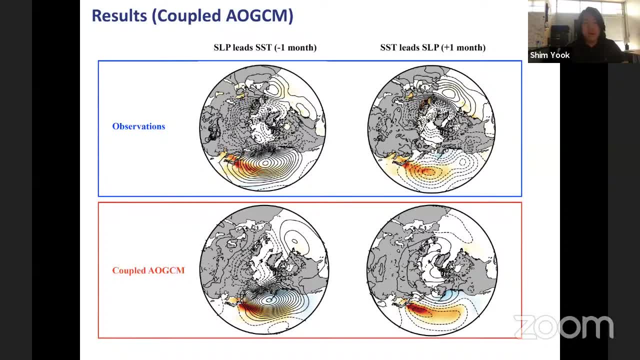 the observations and the coupled AOGCMs are actually very similar to each other. So we can see both the atmospheric forcing pattern as well as atmospheric response pattern are well represented in the coupled AOGCM, although the amplitude of these low pressure anomalies are 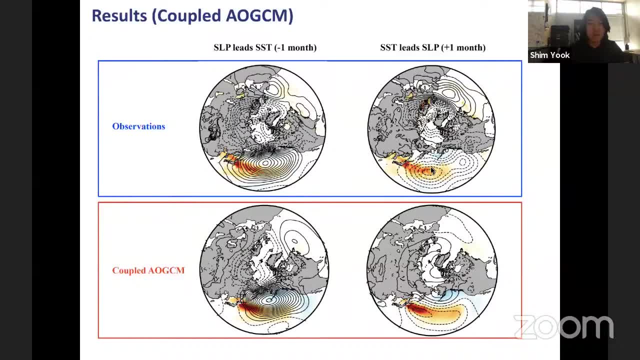 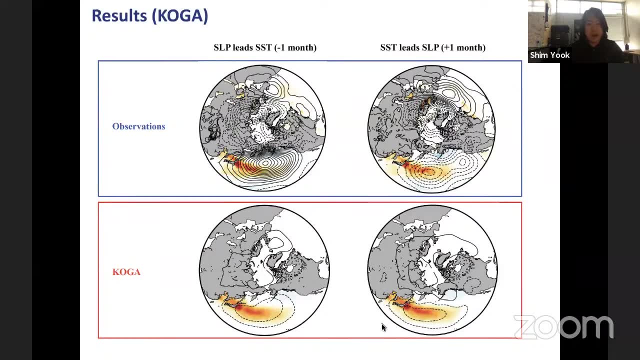 already weaker in the simulation than in the observation. Now the upper panels in the blue box are the same as the previous slide, but the lower panels in the red box are the results from the COGA runs. So if you look at the left column, there is no distinct atmospheric forcing pattern. 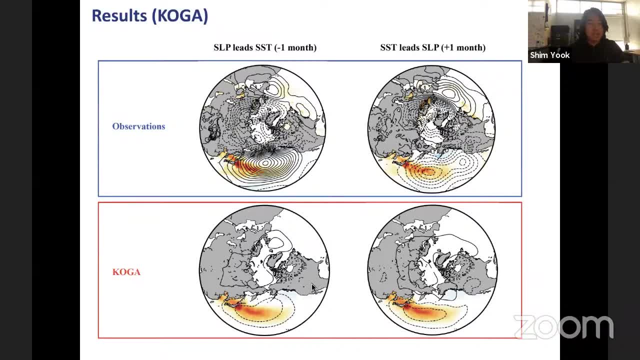 shown in the negative lag of the COGA simulation. This is expected because the SSTs are given as data and thus the low level temperature direction by atmosphere is incapable of influencing the ssd field. rather, the results from cogaron show the this low pressure anomalies. 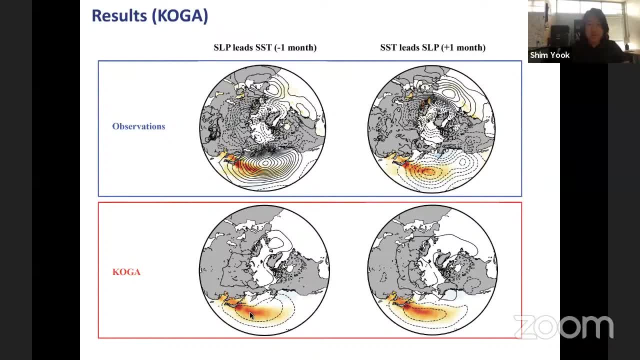 at all legs and by construction. atmospheric parents shown in the cogas runs are all representing the atmospheric response to the prescribed ssd forcing. so this close similarity between the atmospheric response pair net cobas run and the inferred answer responses- uh, positive lag in the observation- suggests that the letter pattern is actually the atmospheric response to the local 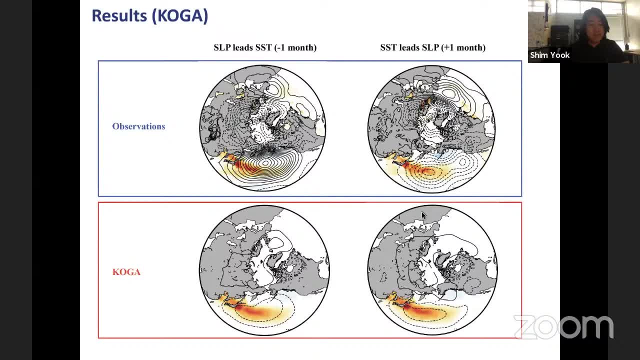 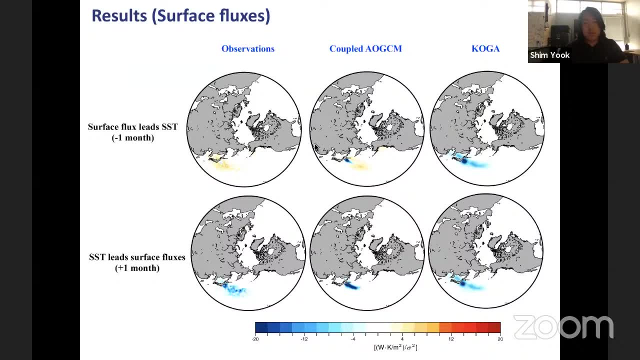 ssd anomalies over the western pacific region. so our interpretation of atmospheric circulation pattern is further supported by attendant changes in surface hip fluxes. here surface hip fluxes are defined as a sum of Justice and dicen, Circus and iq and latent heat fluxes. 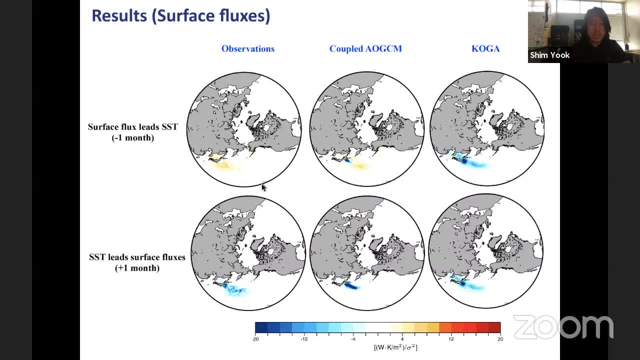 So this plot showed the product of SST and surface heat fluxes. So the regions with positive values indicate the area with the warming of SST through the downward surface heat fluxes from atmosphere into the ocean mix layer, And the regions with negative values show the area with cooling of SST. 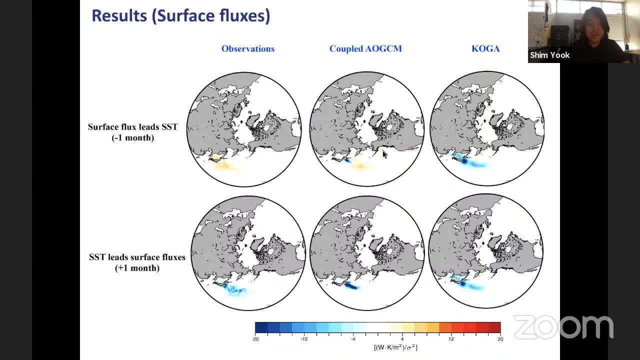 through the upper surface fluxes from ocean into the atmosphere. So if you look at the left, two columns in the upper panels, the result from the observations and the couple of AO-GCM shows that at negative lag there is a warming of ocean mix layer through the downward surface. 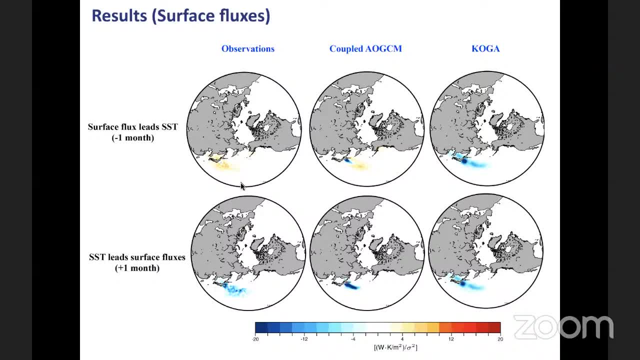 fluxing from atmosphere into the ocean And at positive lag there is a cooling of SST associated with the upper heat fluxes from ocean into the atmosphere. So at negative lag the atmosphere circulation pattern is consistent with the atmosphere forcing of SST. And again at positive lag, atmosphere circulation. 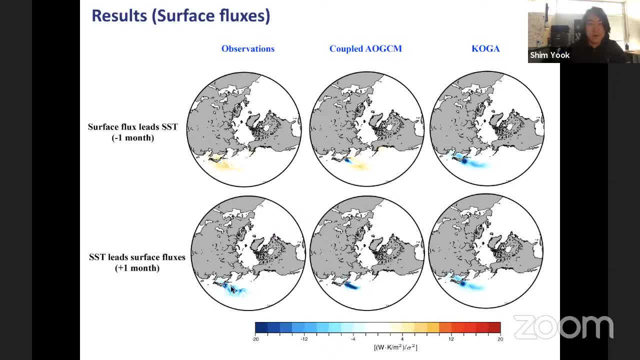 pair represents the atmospheric response to over heat fluxes And if you look at the right column, the Koga results show the over fluxes at all lags. The atmospheric patterns shown in Koga results are again and consistent with the atmospheric response to the overt heat fluxes. 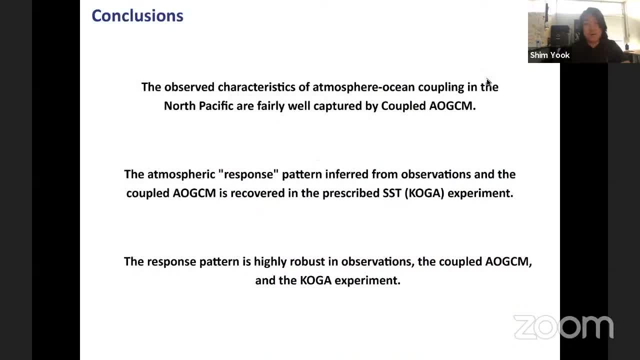 To summarize, the observed characteristics of atmospheric-ocean coupling in the North Pacific are fairly well captured by the coupled AOGCM and the atmospheric ferritic response pattern inferred from both the observations and the coupled AOGCM is recovered in the pre-scribed COGA experiment and the response pattern is highly robust in the observations. 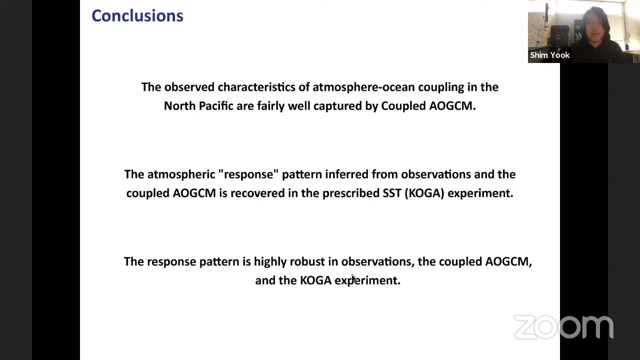 and the coupled AOGCM and the COGA experiment. Thank you for your attention and I'm happy to take any of your questions. Thank you, Questions: There's one in the chat, Not yet. Robert, Do you want to answer your question? 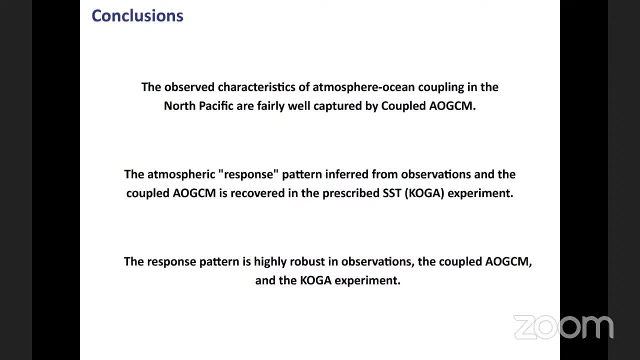 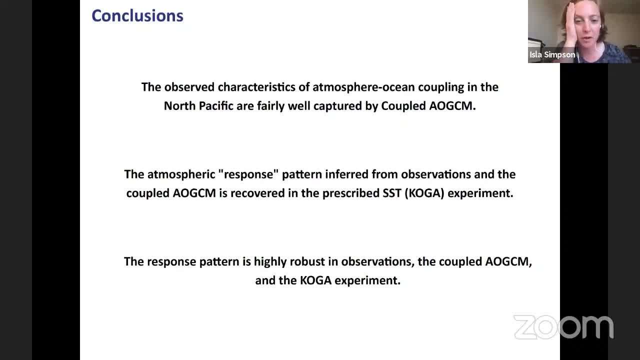 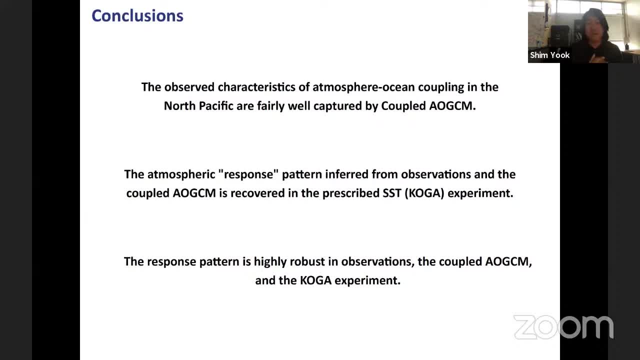 depend a lot on resolution. What resolution are you using and are you planning to investigate the sensitivity to resolution? Yeah, I know there are papers showing the atmospheric response pattern, especially at the vertical extent, depending a lot on the resolution degree. standard resolution only. 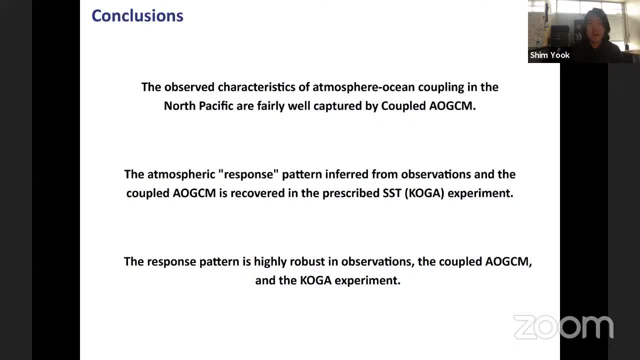 And the response pair was confined to the lower levels, like below 700 hectopascal. I think is consistent with the low resolution version of the similar experiment. But yeah, I don't think I can do the high resolution experiment again. But yeah, at least within the standard resolution. 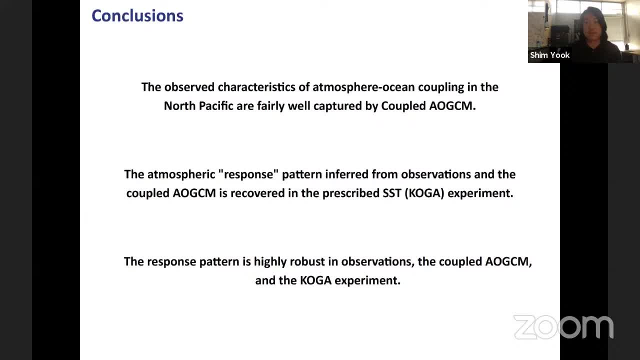 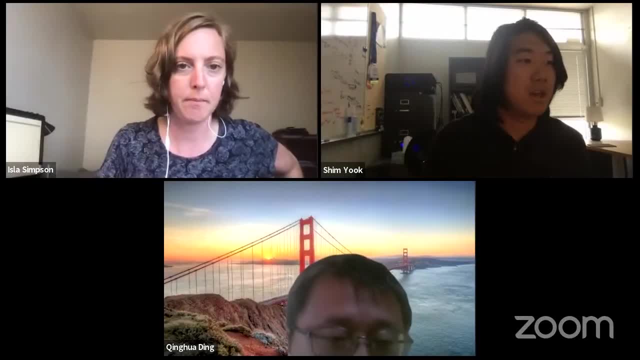 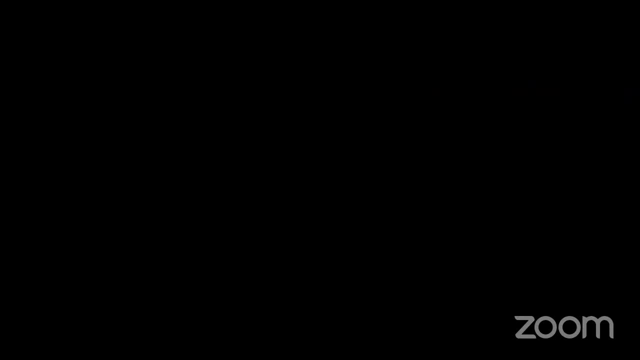 it wasn't sensitive to the resolution of the hemisphere. OK, thank you, And we can move on. Next I will give to Qinghua Jin on this screen and topical-precipital convection. OK, Qinghua, go ahead. 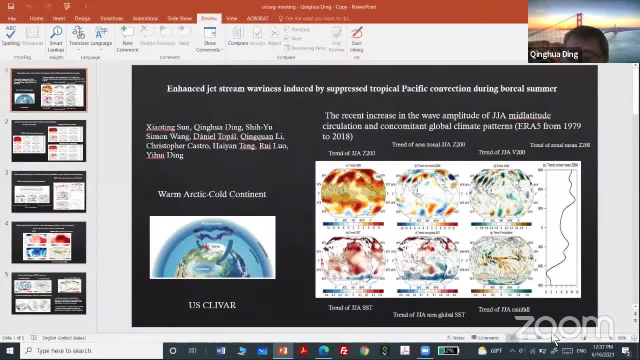 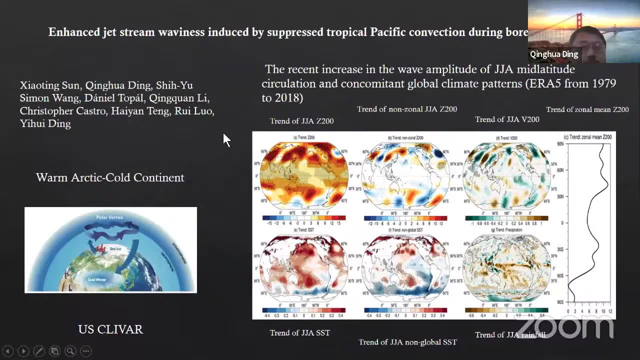 OK, thank you. So yeah, first I'd like to thank the appreciated contribution from my collaborator. I put their name there so I have no time to read, And you can see This is a teamwork And the main goal is very straightforward. 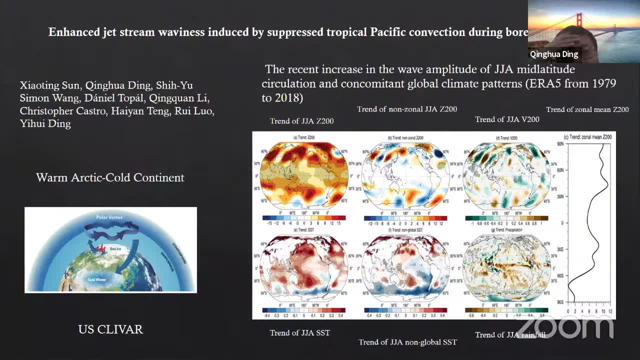 just to try to understand this. the so-called enhanced gesturing waviness feature observed over the past 40 years And the consensus of the community is something like some study tried to argue. this is the enhanced gesturing waviness mainly in Northern Hemisphere. 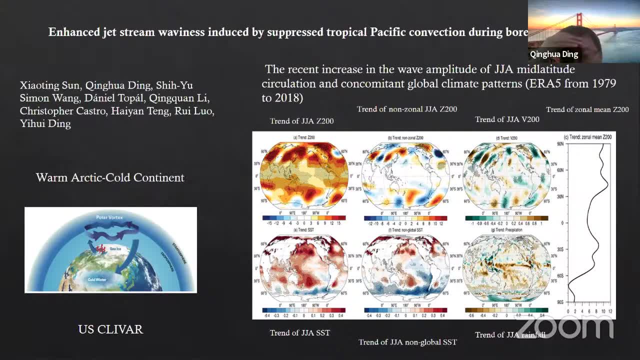 It's mainly driven by this Arctic amplification, or CO2-induced AA effect. The idea is the AA effect is faster than the global mean temperature. That can reduce the tropical Arctic temperature gradient, So that can enhance the waviness and reduce the jet. 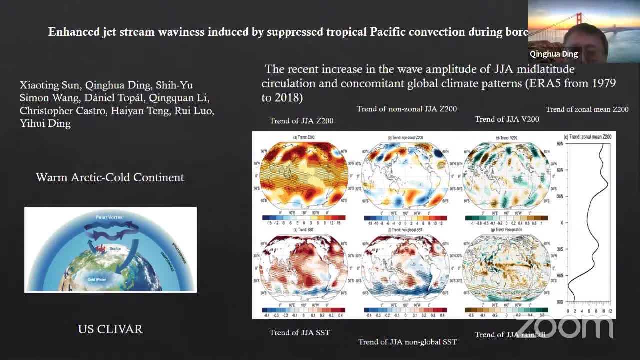 But here we try to argue over the same time. over the past 40 years not only AA is prominent but at the same time there is the cooling phase of the IPO interdicator of Pacific Oscillation staying in some cooling phase. 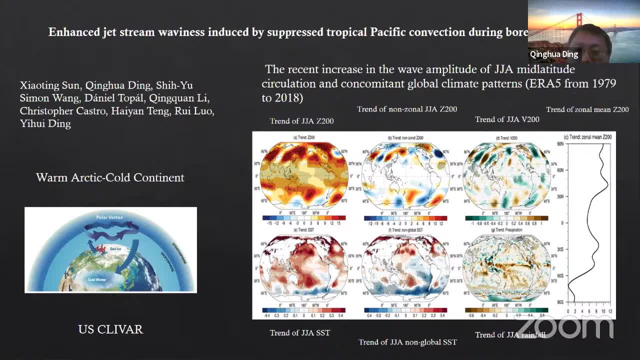 That may also can reduce the temperature gradient, because it's a tug-of-war scenario. like the Arctic warming can reduce the temperature gradient, But if there's internal IPO cooling signal, this signal can also reduce temperature gradient. So we try to argue. probably we try. 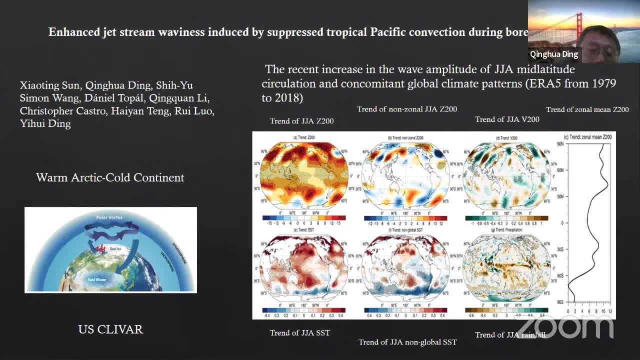 to give an alternative perspective to explain the same thing, that is, this internal, or we call it surprise. the ITCZ convection during summertime could also contribute to this reduction of the jet stream. So we try to argue that the and the other way to explain this feature. And from the in the right hand side you can see there's like six panel. Oh sorry, six panel And so this six panel, there's seven panels And this is the trend of the JJA-Z200 from ERA5.. 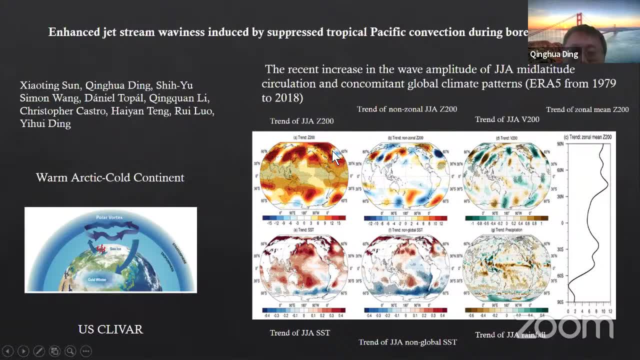 And this is the trend of the JJA-Z200 from ERA5.. And this is the trend of the JJA-Z200 from ERA5. And we're using this one to show you. actually, this wave is enhanced, indeed, over the past four years along the jet stream. 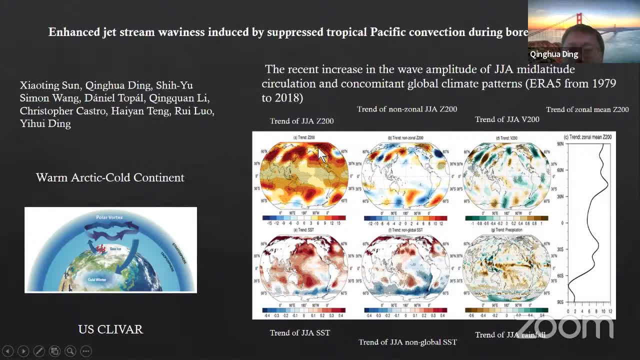 Northern Hemisphere in summertime. So you can see there's a high, low, high pressure, high, low, high chain of a high, low, high pressure anomaly and the pattern. And if you remove the zoonotic component, this wave structure has become more clear. 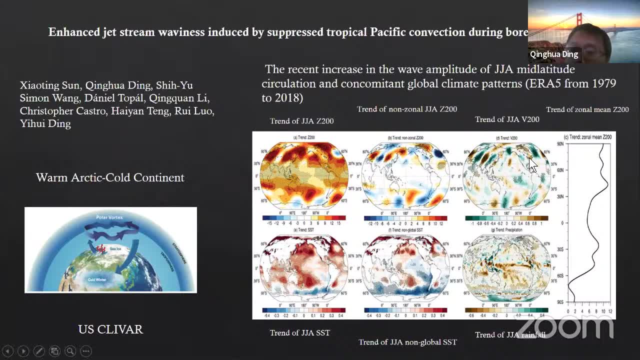 And so. but if you look at the trend of the Meridiano wind, you can find there's a lot of enhanced wave and it's along the jet stream And this is the zoonotic component of the Z200.. So you can see the maximum height rise. 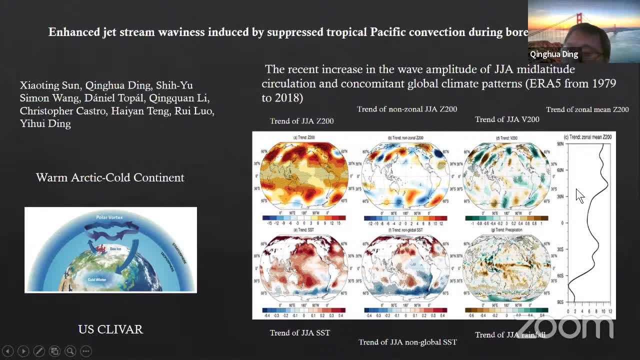 in terms of zoonotic components, is located over 40 degree north, just along the jet, And at the same time. meanwhile, if you look at the trend of the JJA-Z200 for 40 years, you can find that there's a global warming signal very clear. 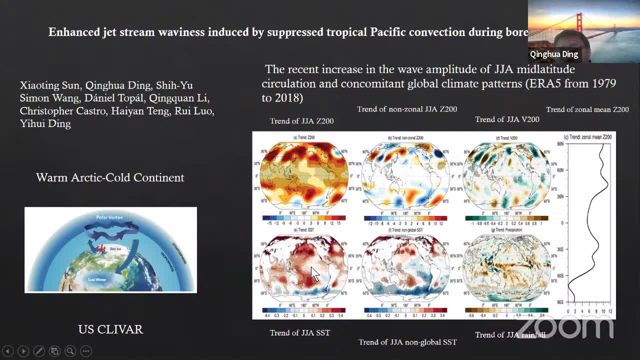 but also there's like internal cooling. So we think this is probably due to IPO phase shifting to this cooling phase And this is a kind of non-global- I said he does a using this trend to subtract a global average warming signal. So you can see there's a clear cooling phase. 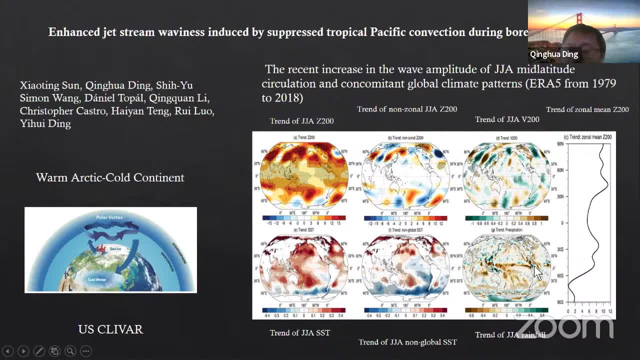 over eastern Pacific And here is a precipitation, just like a JJA trend over the same period. So you can see a clear is a draining, So this is a shading, this is a draining of like ITCZ along this ITCZ position. 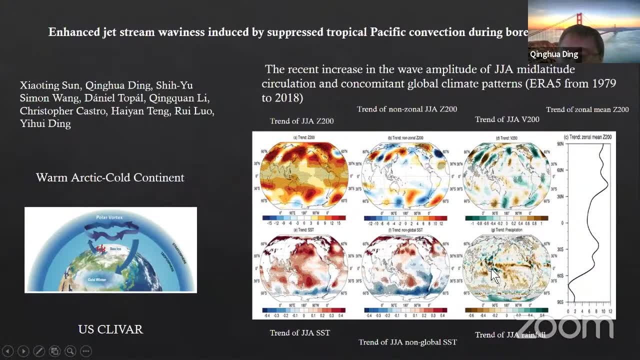 And there's another warming, an increase of precipitation, not warming, increase of precipitation monitoring or is the maritime continent over this part? So we think that this structure is important to to maybe contribute to this wave in this, enhance the wave in this. 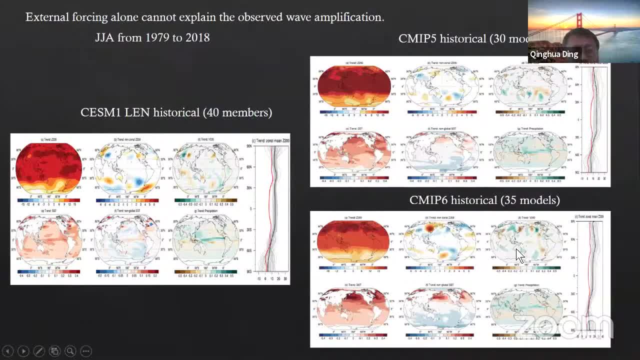 So then we first thing we want to check is this: external forcing a historical run from different sources, like the historical CSM1, larger sample for the member, add them together. same layout as a private one and the seven panel and the same variable. 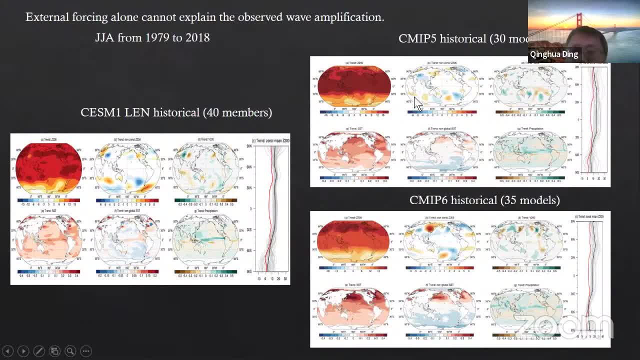 same non-global, non-zonal things And the CMB5 historical run certain model and CMB6 model. we put all together. So you can- yeah, it's really busy, but you can clearly see- is that the main point is that 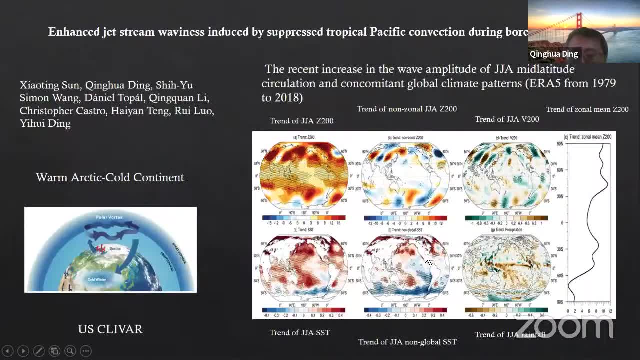 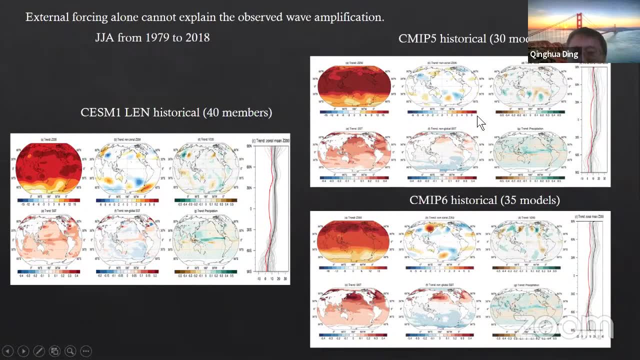 the first thing is a tropical SIT cooling model cannot capture and just the model. if the raw, raw trend or non-global or give like an you know like pattern, no matter in CMB5, CMB6,, CMB6 not as strong. 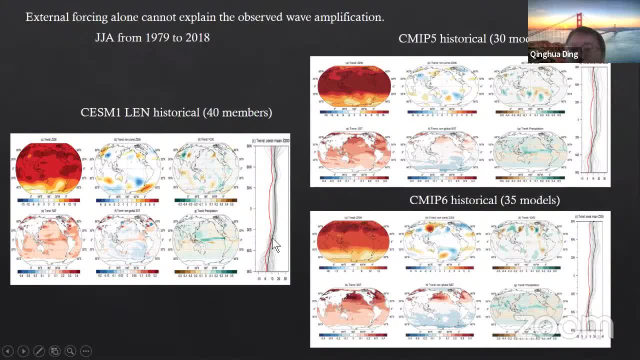 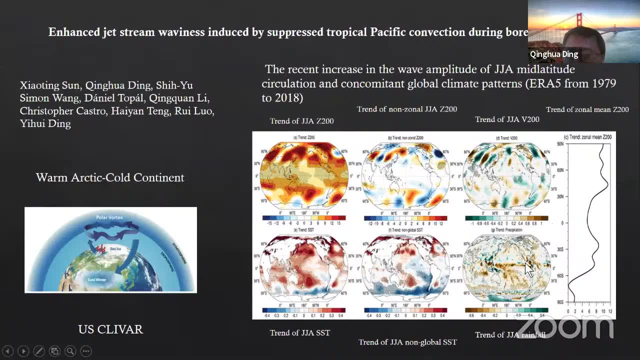 but CSM pretty strong And the rainfall change is like the increase, like the ITCZ, but in observation we see this a decrease of ITCZ, a decrease, a surprise, of convection along ITCZ. And another thing is the waviness. 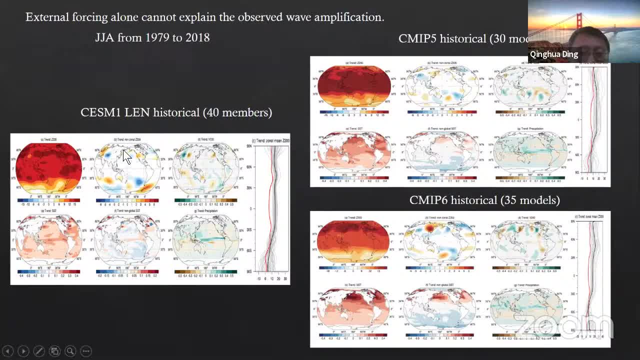 The waviness. we don't see very clear waviness, If you want to, using like the non-zonal Z200 or meridional wind to quantify that. we see that the magnitude is much smaller than observation And the observation is something like this: 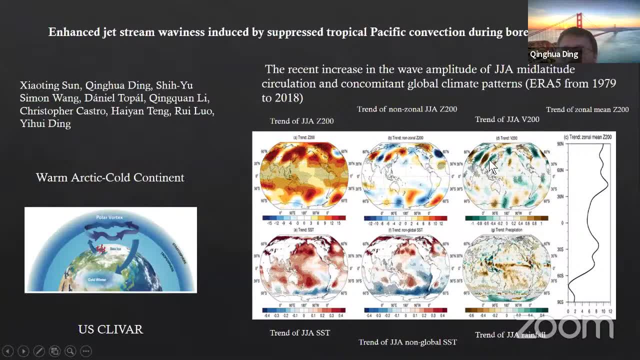 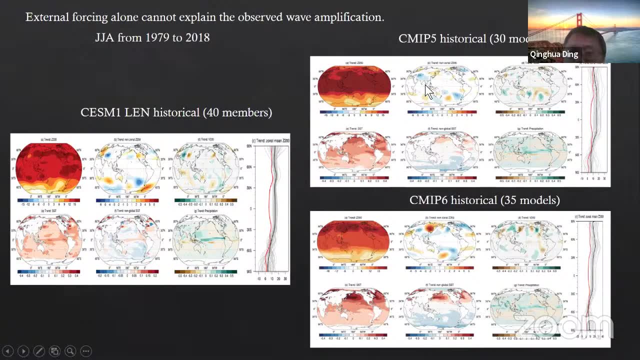 the unit here is a per decade, So this is like one meter per second per decade And here is like the 10th, But if you look at the multi-model mean so you see, is the non-zonal is not as strong as CMB5,. 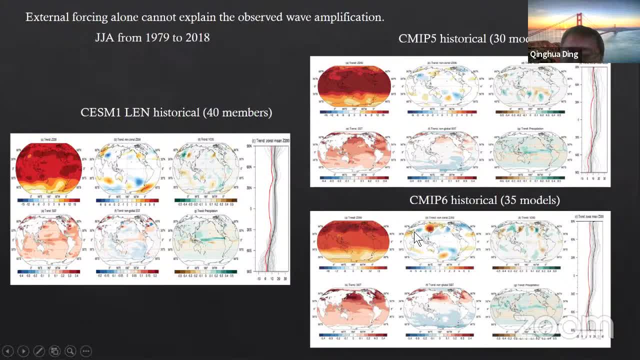 CMB6 improve a little bit and capture this. It's a waviness a little, but it's much weaker. It's one-third of observed magnitude and meridional wind not that strong And the CSM1 shows some waviness here. 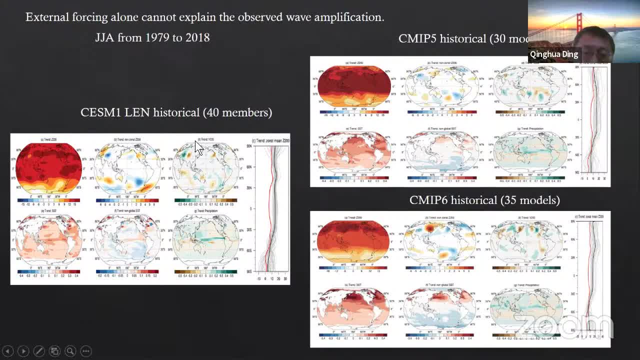 but not so connected throughout along the jet. Another thing we see is the zonal mean component: 40 member average or all member average. It seems like to overestimate a tropical warming because you see, it all is a height of rise. It's a much stronger. 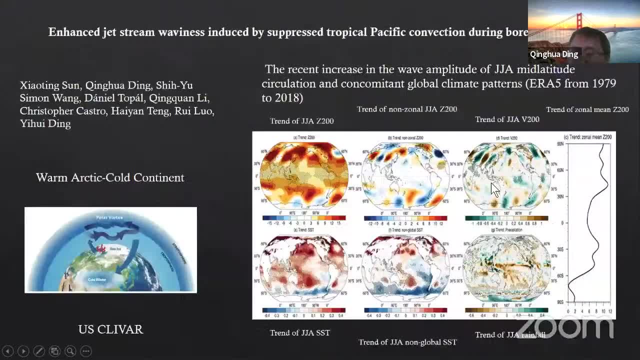 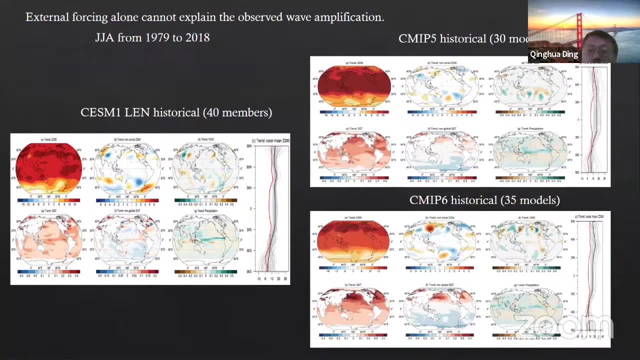 than observation. Observation is the red one, This is the red one. just to simply copy from this plot, from this is curve this line. So idea here: is that external. so another thing I like to argue is: they see, the Arctic warming is also well captured. 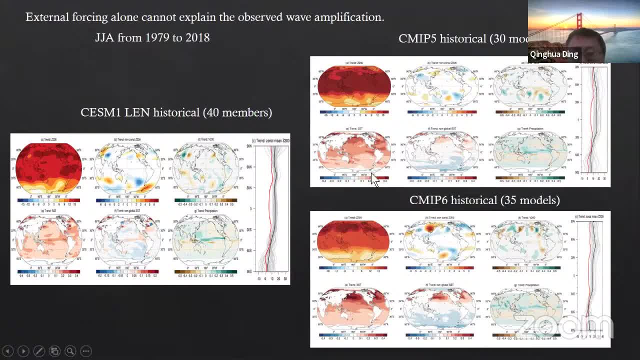 So by or it's a model, because the AA can easily trigger by this CO2 increase. But when the AA is present and Arctic CO2 forcing is strong, but just in house of waviness, it's not that clear. So we think to, probably due to there's the 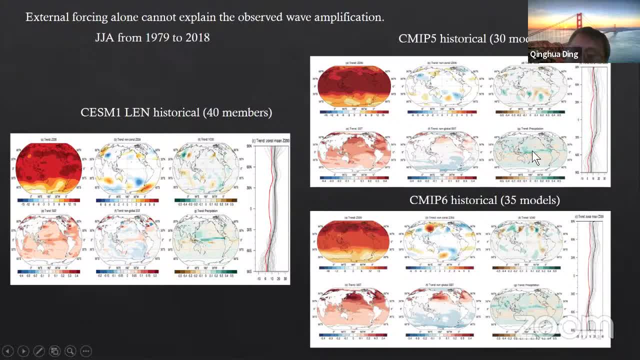 a little bit biased the simulation of a tropical convection, because in observation we see there's the cooling signal or draining ITCZ, but the model give us C2 forcing, give us like the wetting signal there. So we think the internal tropical acid cooling. 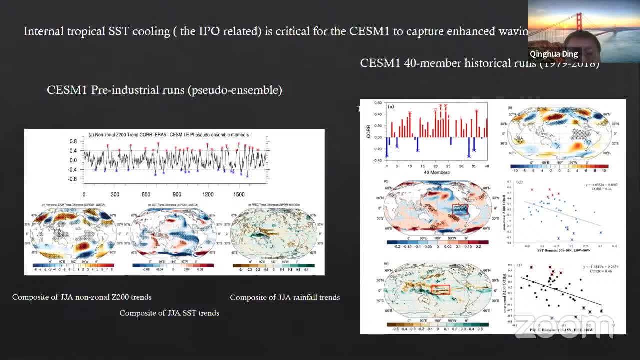 just like IPO related is important, but we're using two approach to prove that. The first one is we just are using model itself. We don't do any like the inhouse experiment, So we just are simply got it okay in house. 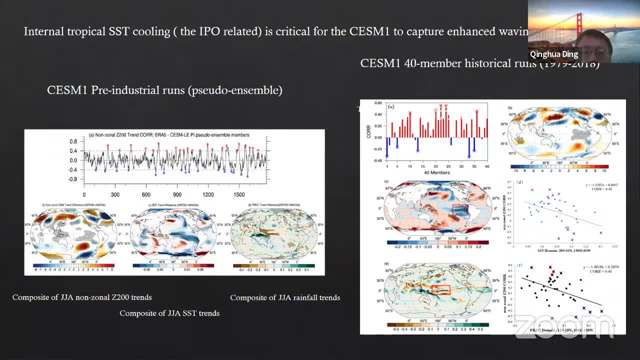 free round, no CO2 falls in there, just like a long control round and trimmed to very short four years period so that can compare with observation. So we have many, many like a sliding window. We can have many, many like four years of period. 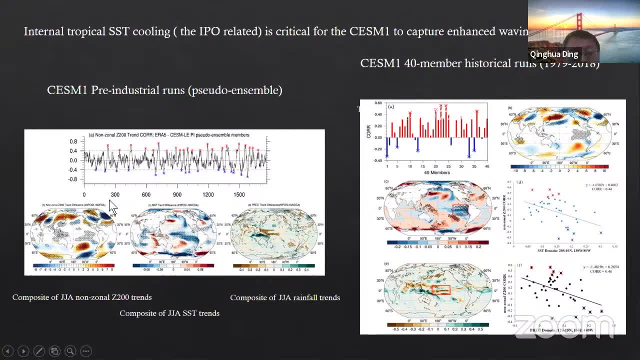 So we constrain, so we ask this model have to capture its waviness by using like a spatial correlation to constrain that one. So we find some member really capture its waviness and some member capture like opposite face, like the blue one, And we can pause it as a red one minus a blue one. 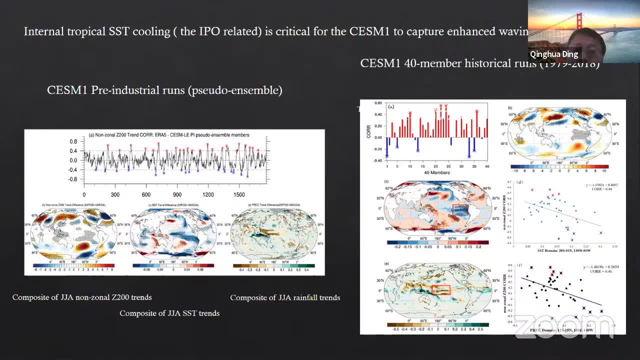 So we want to see, because we are constrained only over along the jet, like a 20 North to 60 North, So we want to see that what would happen outside of it is the mid latitude. So we want to see if a model by chance. 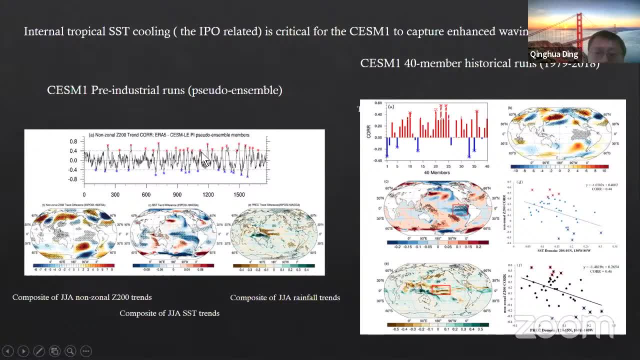 capture its waviness. because we ask a model to do this right, we force model to capture this by design And we want to see what happen, what would happen outside in our and the tropics, But what do we see is always a member. 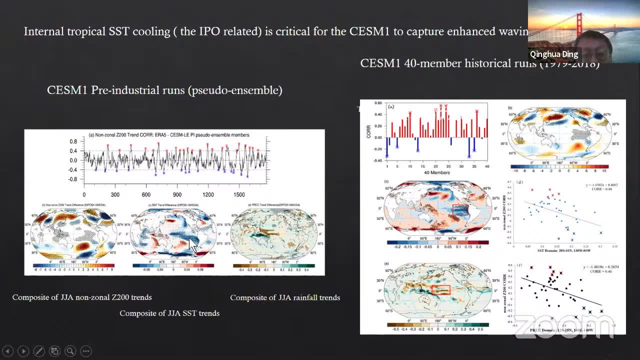 give us the picture like that or a member tend to have as a cooling in the tropics, like IPO and the joining like a long ITCZ and no article warning. So this tells us something like in this model world as AA is not necessary. 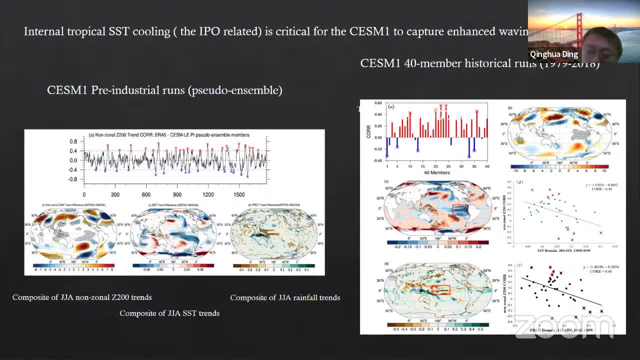 And it's an internal cooling- become more important to concurrent with this enhanced waviness. We also looked for a member historical run because we know in that moment doesn't do well to capture is enhanced waviness. But if you looked at, if we looked at individual members, 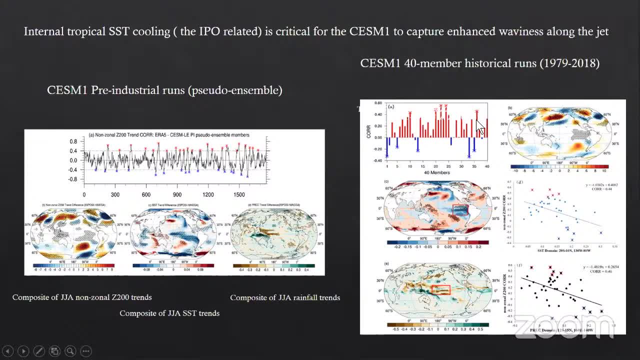 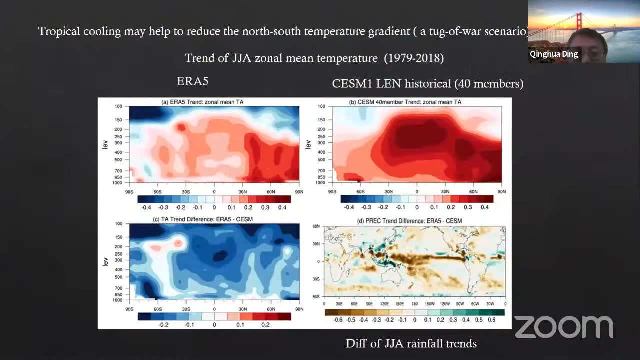 some members do better than other members, So this is a really sorry. Oh so. so so it's the same thing Like if a model by chance capture, internal cooling can also capture well, this waviness. So we want to. so this last two plot is that: 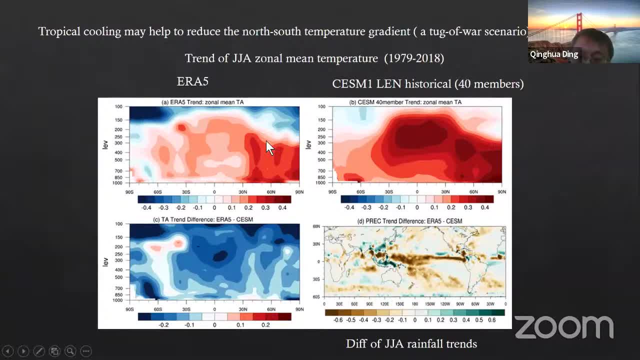 so we think that the tropical cooling may have to reduce the temperature gradient. So it's observation, it's the model and it's a difference. We find this cooling And we think there's the joining, this presentation, different ERA minus ESM. large sample. 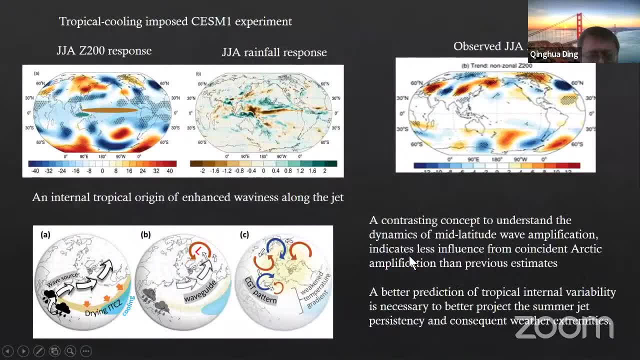 So they still there's a cooling may help. So this is my last slide, So we do some like experiment. we just put this pattern: ITCZ suppression and this enhanced maritime continent, the presentation in the model to see in CSM1. 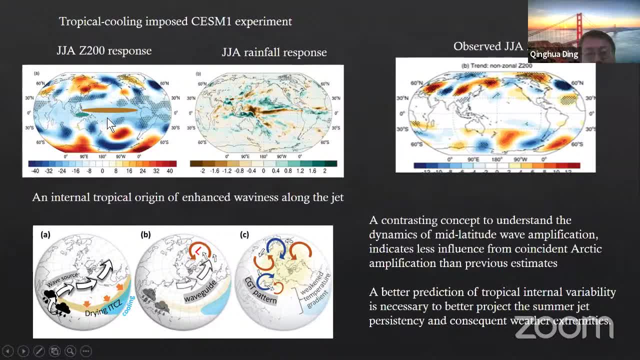 and compare control and this It's like a snapshot model to one year one and the 10 members and compared with the control one And it is the presentation change. and it's a one year one and the 10 members and compare with the control one And it is the presentation change. 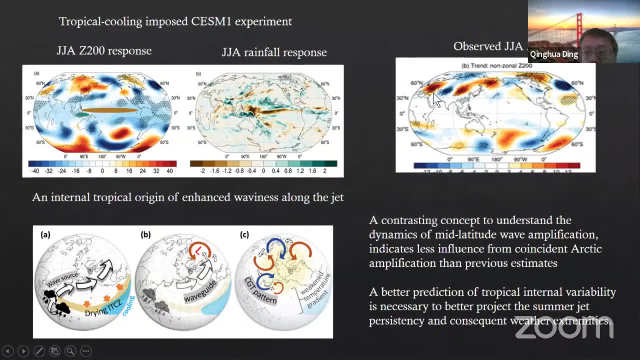 and it is waviness. So we find the model can capture this waviness if you compare with observation, Not completely, but roughly captured, enhanced waviness. So this is our cartoon summarize. our main idea is that this ITCZ shift due to this IPO, cooling and general some waviness. 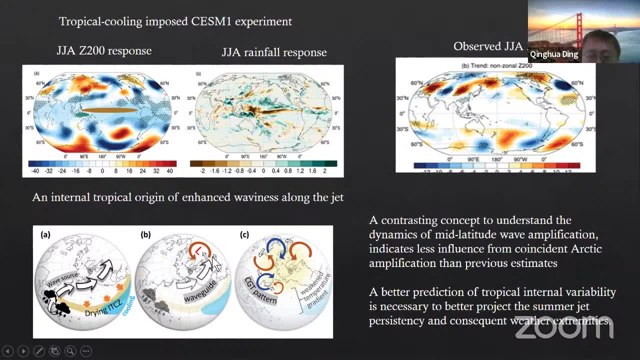 and this- maybe there's like a jet stream- favors the barotropic instability enhancement and favors the waviness. So there are two things. One thing is the cooling favor- weaken this temperature gradient, but at the same time it's the tropical precipitation change and we also 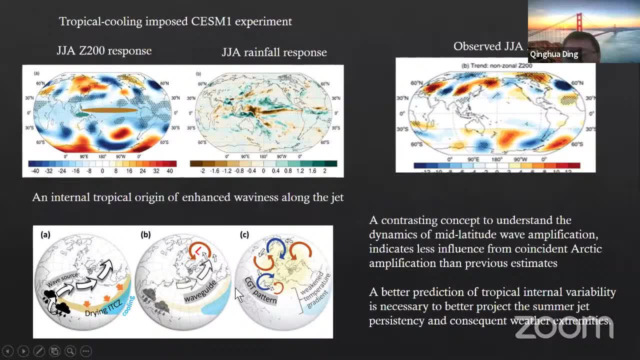 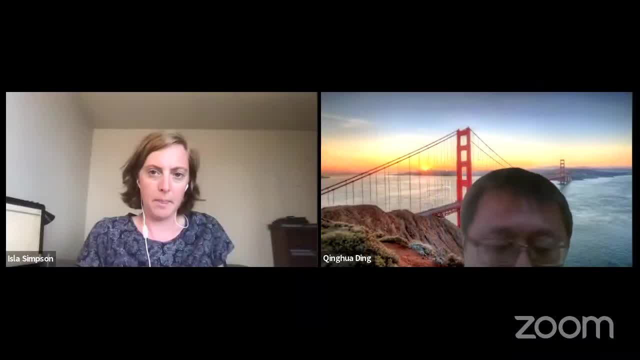 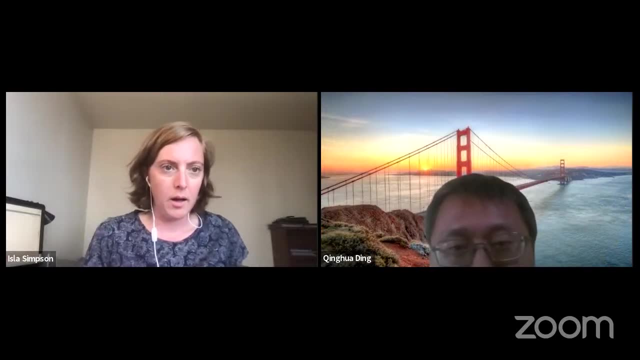 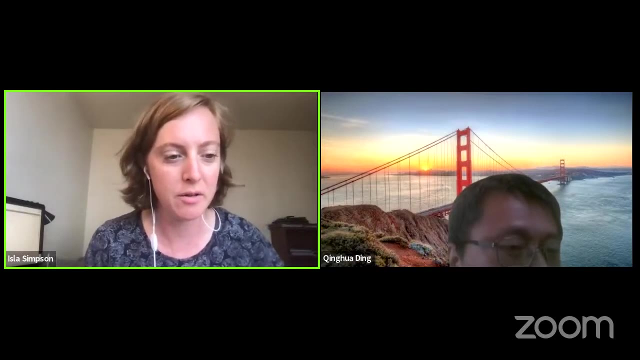 favor is the generation of the wave pattern. Yeah, so this is the whole story, Thank you. Thank you. I was just wondering if you looked at the AMF runs or the pacemaker runs to see if prescribing the SSTs gives you the waviness trends. 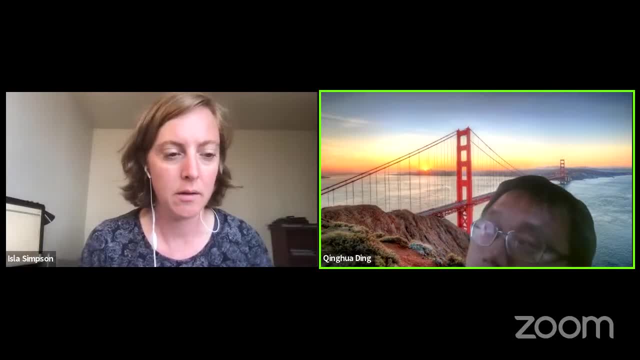 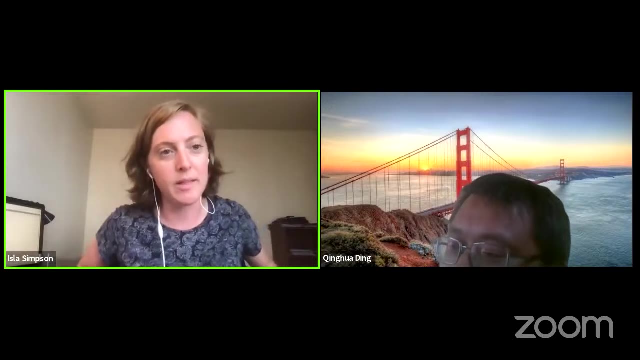 Okay, thank you, I would like to do that, but I'm not sure. Yeah, the summer runs also add CO2 together at the same time, so we want to use some AMF without adding a tropical acidity only. So, yeah, I will check the data archive to make sure And, I guess, comparing them with the large ensemble. 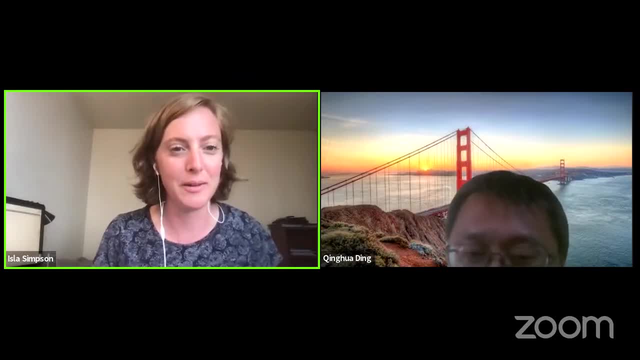 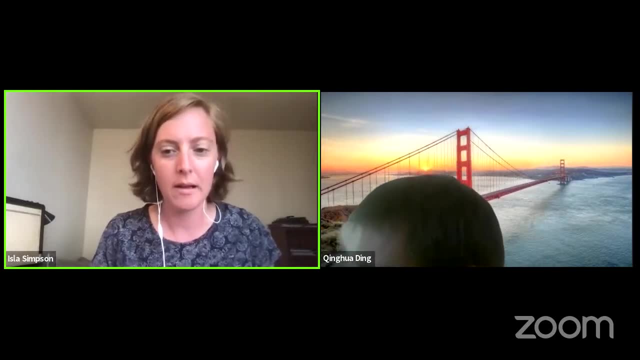 the large ensemble doesn't get it, then the CO2 is not doing it right now because we have 10 member ensembles of the GOGA runs. Okay, Thank you. Okay, there's no other question, So let's move ahead to the 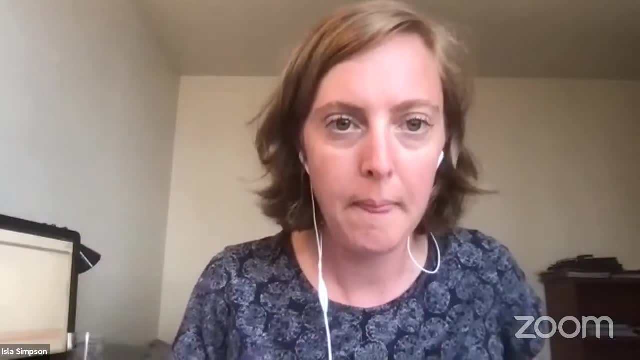 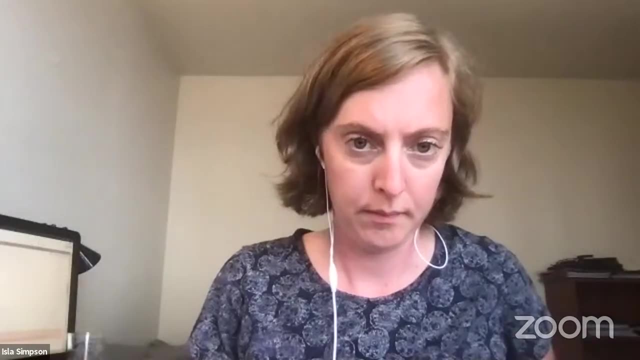 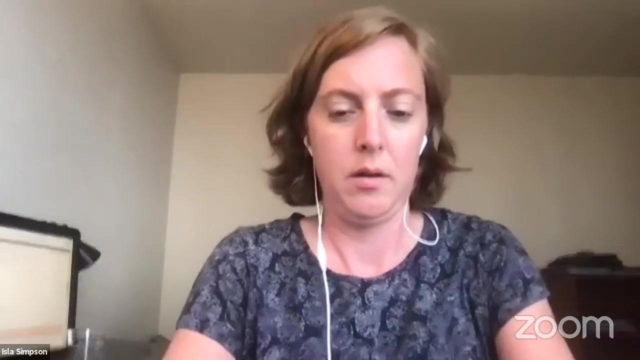 desktop. This will be given by Ming-Hung Zhang On the surface equation change over the top for landing in one month. and hey, Ming-Hung Hi. so I just share my screen. Can you see my screen now? Uh, yes, it's not in the. 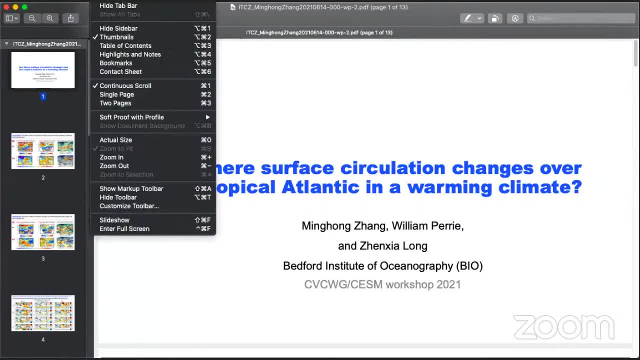 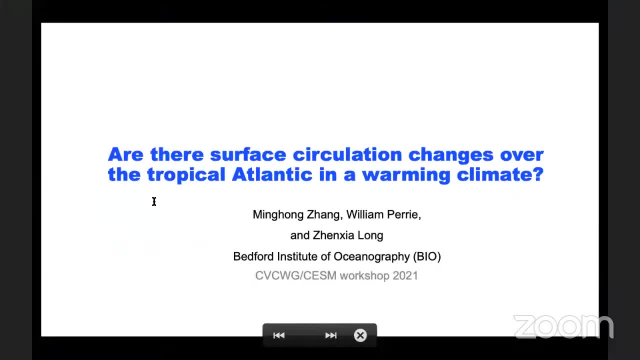 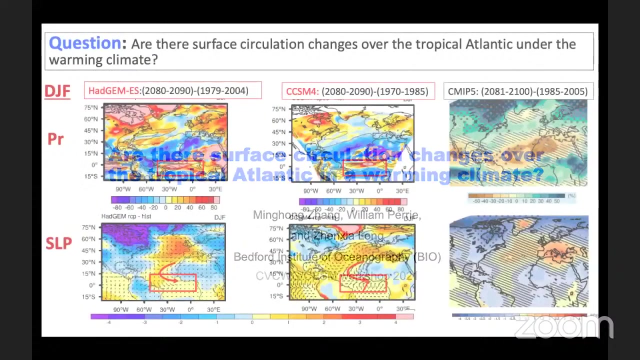 Okay, yeah, Great, Oh sorry, Yeah, uh, hi everyone, Good afternoon. Today my talk talk is Azir. What's going on? Hi everyone, Good afternoon. Today my talk talk is Azir. What's going on? So Azir is an associate professor of the Department of Ocean Technology at the 🎵MESA. 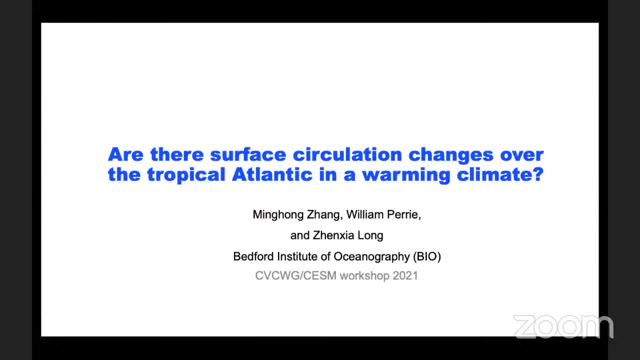 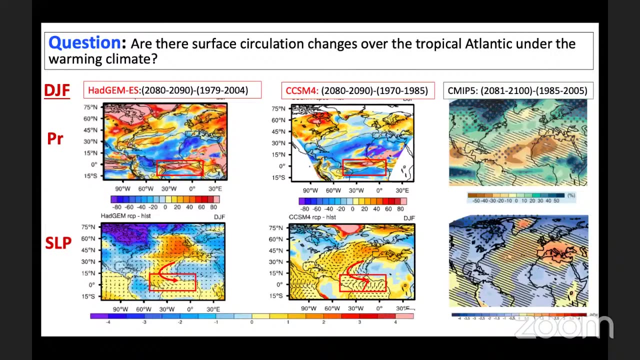 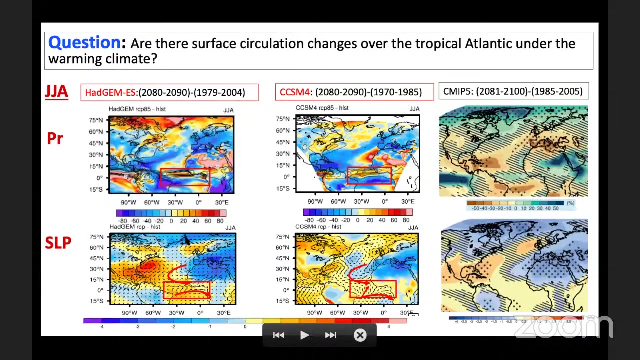 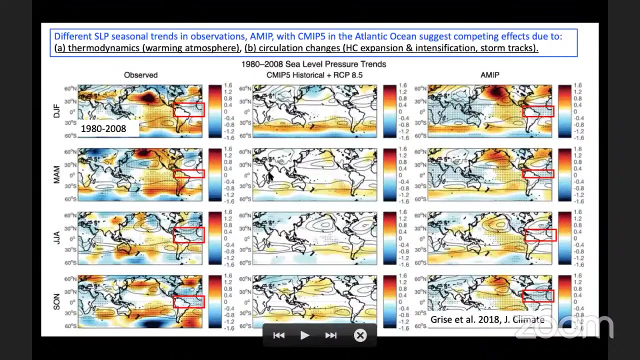 Center for Sustainable Environment and Ecosystem and bodies. results show that there is a robust increased presentation of the RTCZ region, but there is not much change in the surface wind and sea level pressure. It is a similar phenomenon seen in summer. So, however, if we look at the observed sea level pressure, 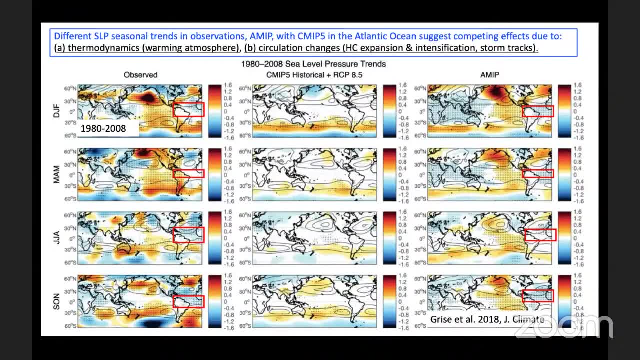 signal trend we can see there is a decreased sea level pressure alarmingly over the tropical Atlantic Ocean And the AMIPO experiment also suggests decreased sea level pressure over the tropical Atlantic Ocean, while there is not much change in the simplified climate model. 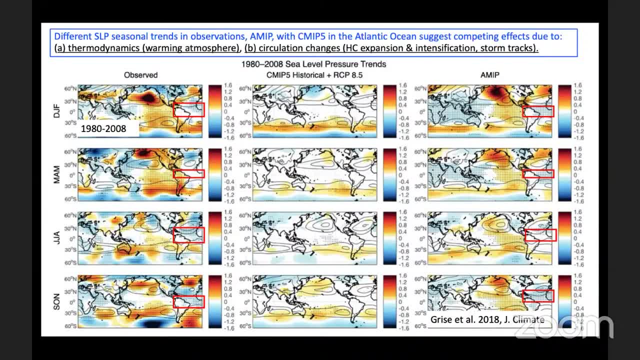 So it suggests that there is a very large uncertainty in the changes of the surface circulation over the tropical Atlantic Ocean. It could be due to the competing effect, such as the thermodynamics effect over warm atmosphere, and the circulation change, such as the expansion. 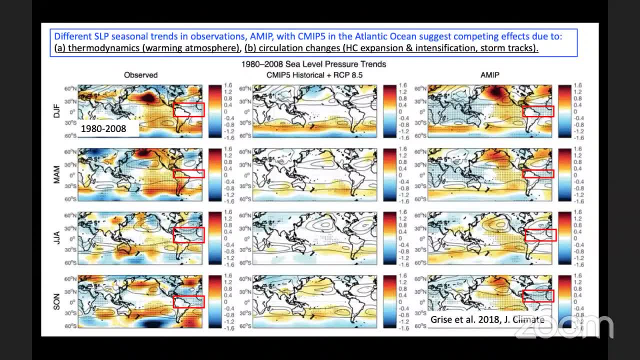 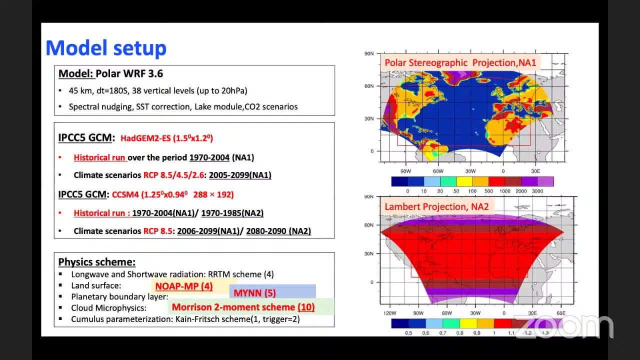 or the changes in the storm track. In our project we can conduct several downscaling simulations of the North Atlantic climate using PolarWolf, driven by hardware center-assisted model and 6SM4, following three scenarios: RCP 8.5,, 4.5, and 2.6.. 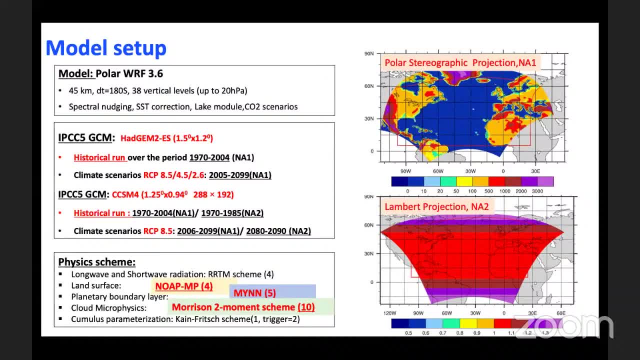 We get some interesting results regarding the surface circulation over the tropical Atlantic Ocean. That's the reason why I guess I'm going to give this talk. The upper panel shows the first wolf domain. The reason why I choose such domain is to cover the ocean domain that is shown by this red box. 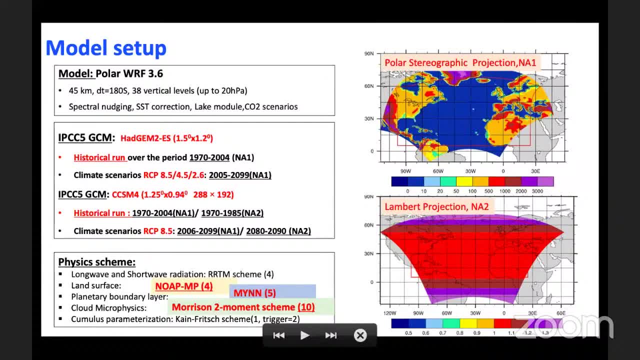 To save the computing time, I try to minimize my model grid. So the source boundary of my model domain is located over the ITCZ region. The source boundary of my model domain is located over the ITCZ region. The source boundary of my model domain is located over the ITCZ region. 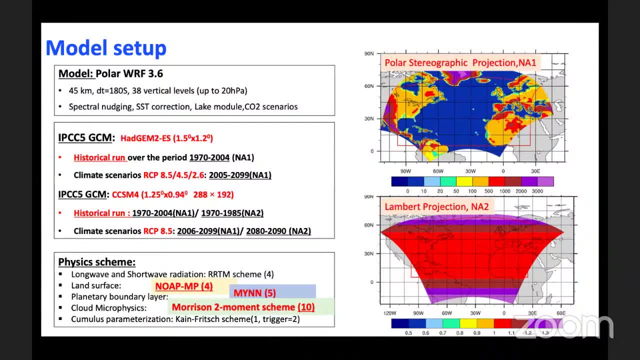 The results prove it is not a good idea. So I build the second wolf domain to cover the ITCZ region, Although it is not fully cover the ITCZ but it works for our regional oceanic modeling. So this second domain is NA2.. 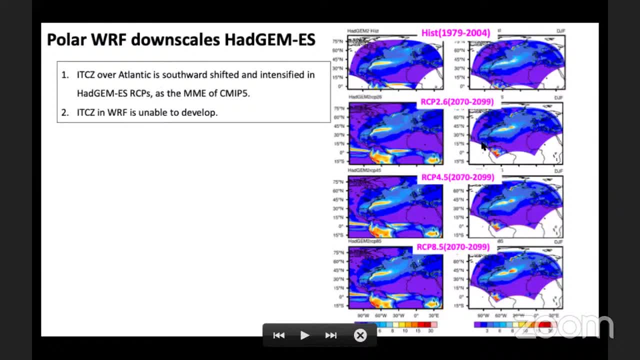 The first domain is NA1.. In the next several slides I will show some downscaling results. First let's look at the precipitation from the Hadassah Center's model result and the Worf-Dunskinny result in the historic and three RCP scenarios. We can see Worf did a fairly good. 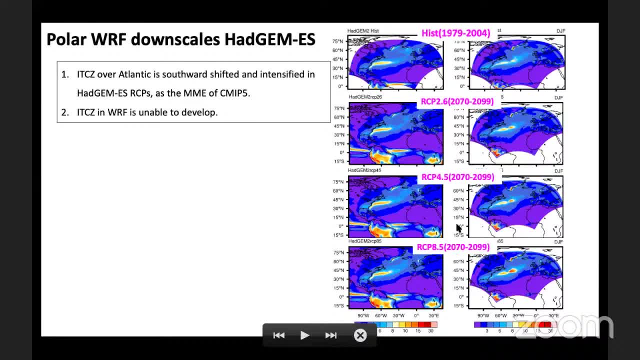 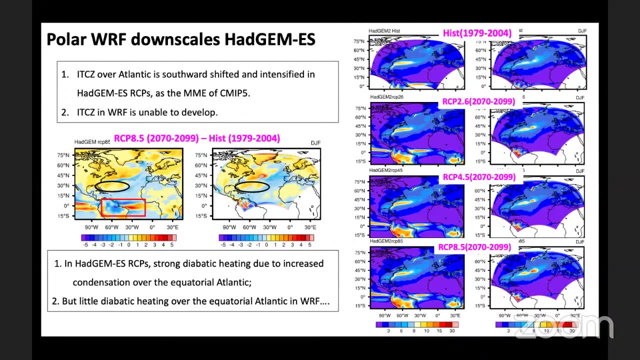 job over the extra-tropical precipitation zone compared with the Hadassah Center's model result. However, the HCC in Worf is unable to develop. So when we look at the difference plot between RCP in matters of historical scenario, we can see there is no much signal. 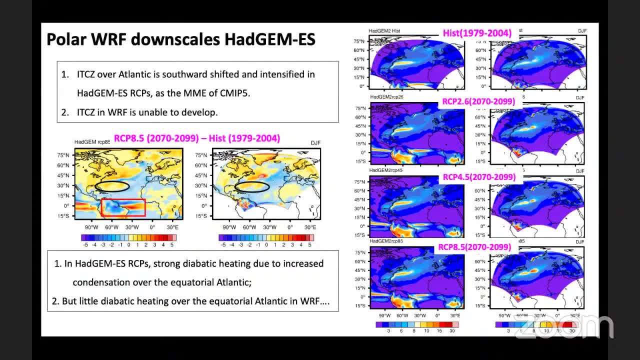 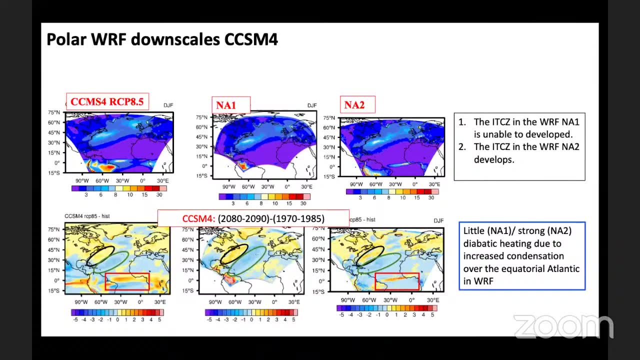 of the precipitation over the HCC region in Worf compared to very robust increased precipitation over the ITCZ region. This slide shows the downscaling result driven by a 6SM4 RCP 2.5.. When we look at the precipitation result, 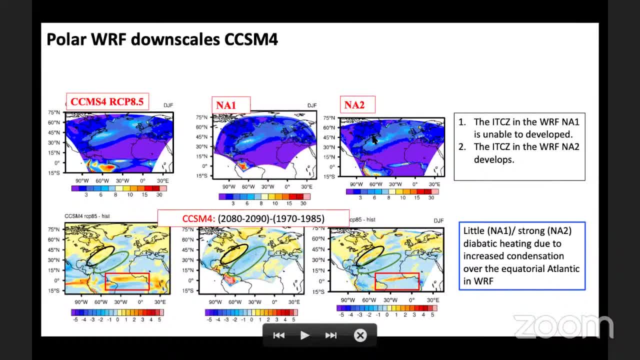 from two-worth simulation over this two-worth domain we can see it's similar. The worth did a fairly good job in the precipitation over the extra-tropical region, but the ITCZ in this smaller worth domain is unable to develop. 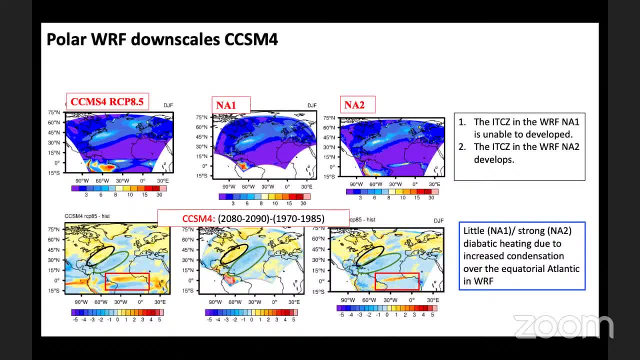 And the ITCZ in the second-worth domain develops, but it's much later compared with the 6SM4 model result. Then we look at the difference plot between RCP minus the historical scenario, We can see it's a very similar situation. 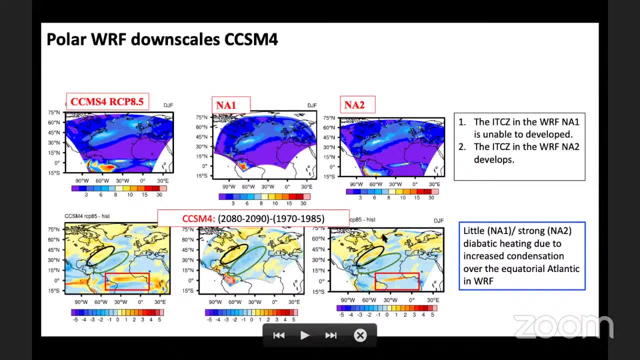 A two-worth simulation shows similar precipitation chance over the extra-tropical region compared with the 6SM4 result, But over the ITCZ region there is an increased precipitation in the worth for NI2 result, but it is still very narrow. 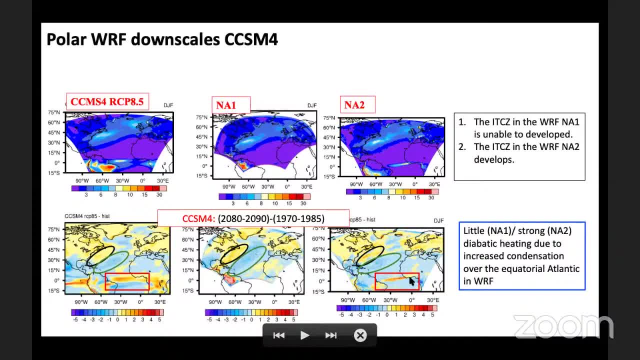 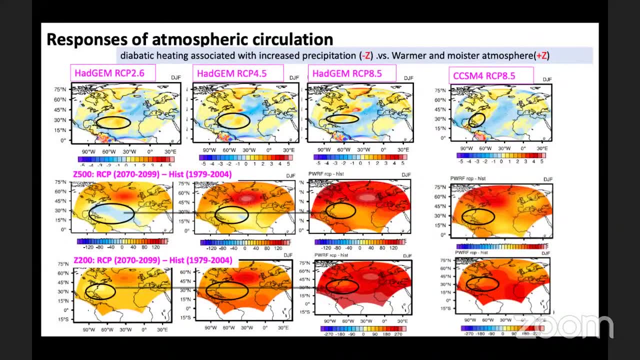 It is still very narrow. It is still very narrow, So it's a lot more difficult to calculate compared to the 6SM4 results. It is still very narrow compared to the 6SM4 results. Then this slide shows the response of the atmospheric circulation. 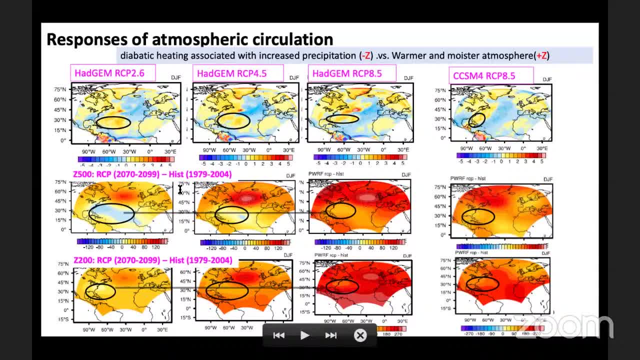 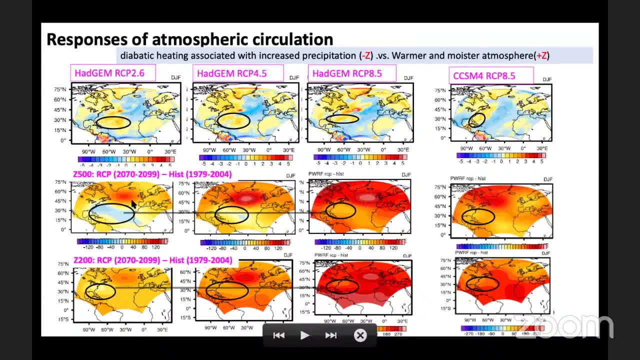 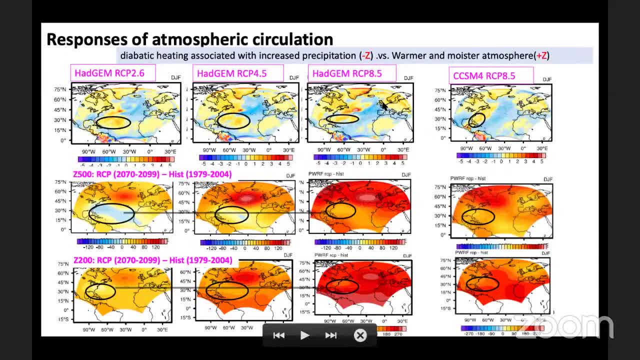 scenarios. However, we can see it's a kind of different chance in the 500 geopotential high among these three scenarios. That's because the increased presentation alone is consistent with the negative geopotential high chance. But the warm thermodynamic effect. 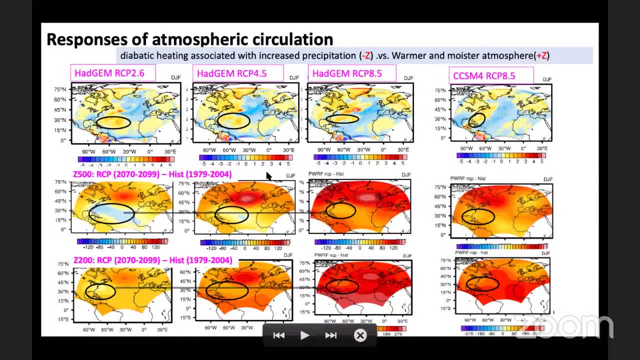 of the atmosphere will tend to compensate this negative geopotential high As a result. this negative geopotential high chance becomes more positive with the RCPs. But over the ITCD region we can see the atmosphere just become warmer. the geopotential 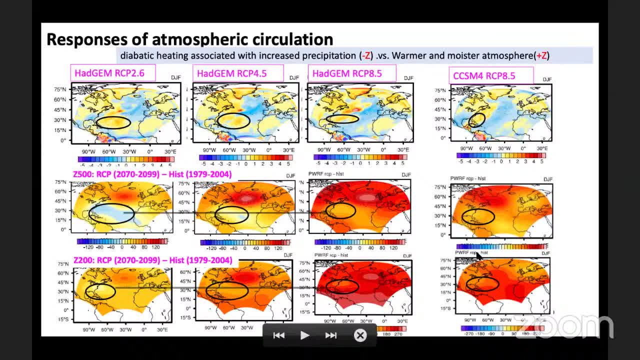 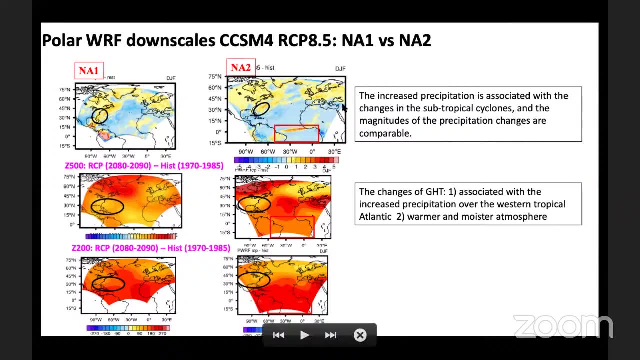 high, become larger. It is a similar result from the Donskini result drawn by CCSM4.. Now I want to compare the two simulations over the world over the two different domains drawn by CCSM4. We can see there's a quite similar presentation chance over the exotropic region. 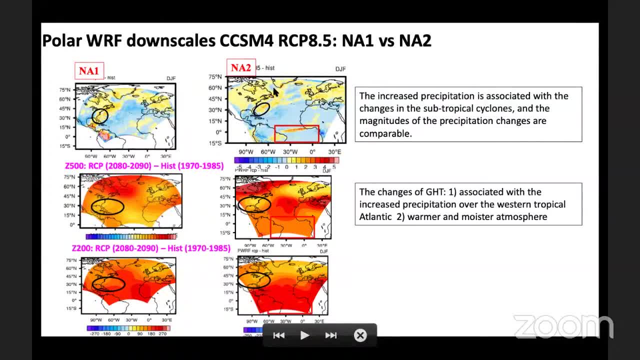 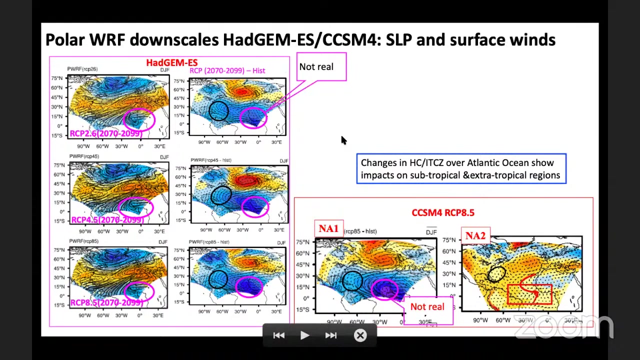 over the geopotential person. We just can see the corresponding changes over the geopotential high at the 500 minibar and 200 minibar just over this western subtropical Atlantic region. I think you have two minutes left, Okay, So then I want to show the sea level pressure and the surface circulation chance to. I just shorten my talk. 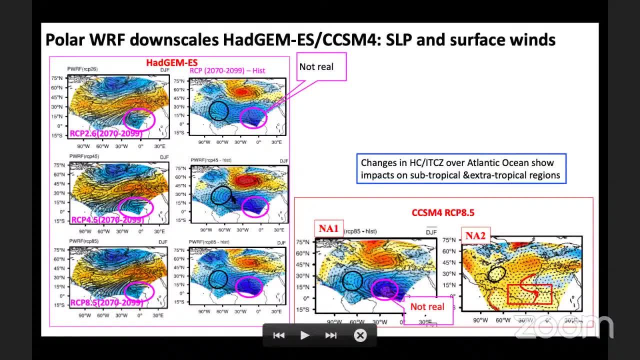 So we can see there's a significant cyclonic sea level pressure chance just over the subtropical western Atlantic Ocean. that is corresponding to the increased precipitation there. However, we also note that this robust negative sea level pressure chance, in this fall wharf downscaling simulation. 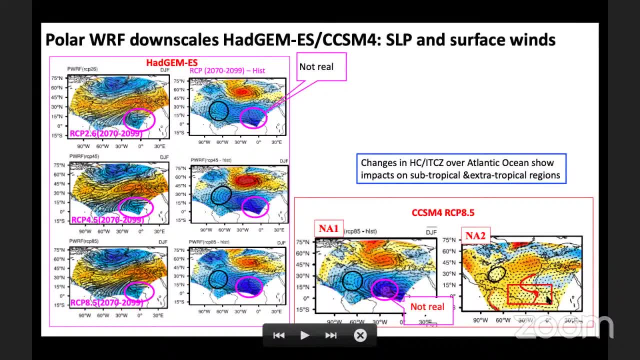 But there's no such negative sea level pressure anomaly in this wharf simulation over the large, large domain. We can see this is a very big negative sea level pressure anomaly. It's from the intensification over this sub, over this tropical north, over the western Africa. 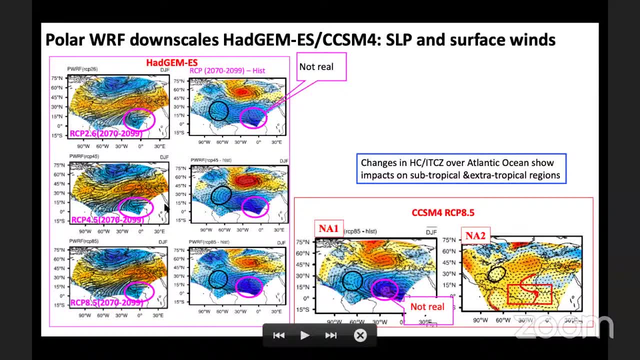 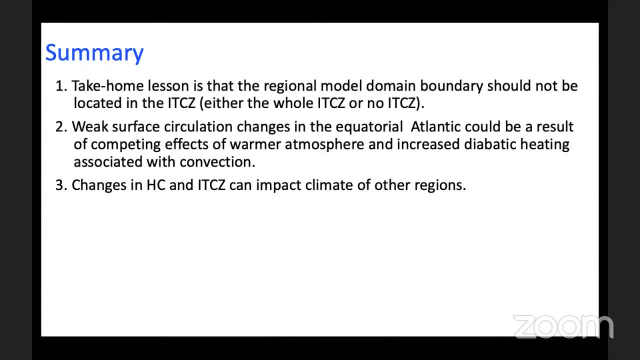 But it is not physical, it is not a real response over the circulation in the warming climate. I don't know why, but it must relate with the domain soil and boundary domain over the wharf. So I just go my summary: The take-home lesson is that regional model domain, boundary domain, 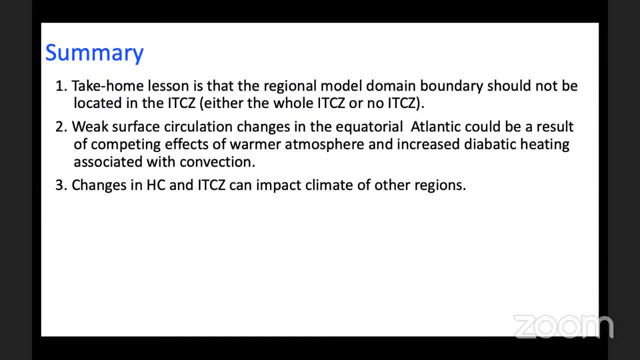 Take-home lesson is that regional model domain boundary domain Should not be located in the ITCZ. Should not be located in the ITCZ. And the warmer. a weak surface circulation changing the equatorial Atlantic Ocean could be a result of the competing effect of a warmer atmosphere and the increased diabetic heating associated with the convection. 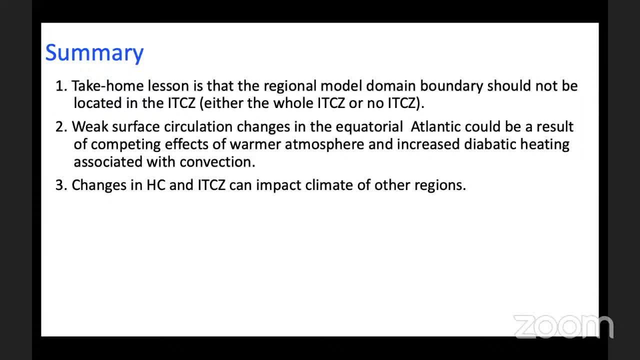 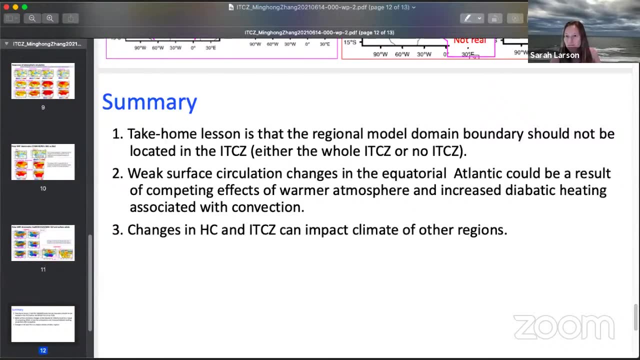 Also the chance in the heart cell and the ITCZ will impact the climate of other regions. Thank you for your attention. Do we have any questions? Yeah, Ayla, I'm sorry if you showed this and I missed it, but did you compare the circulation with what was in the driving GCM? 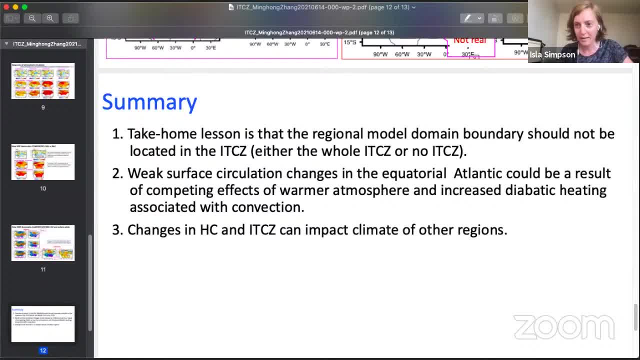 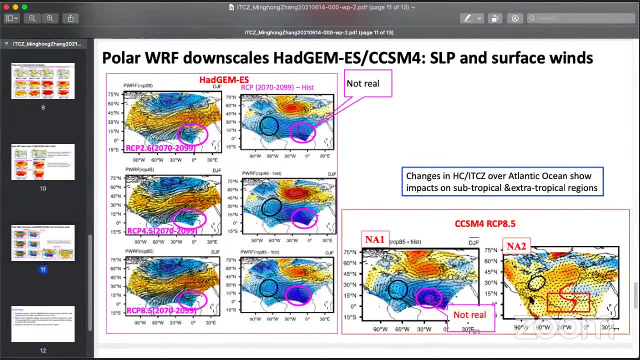 Like if the high resolution of wharf makes a big difference. Yes, Basically the result GCM's result is similar with the result wharf result over this large domain. Okay Yeah, There's no such large serial pressure anomaly over this Western Africa region. 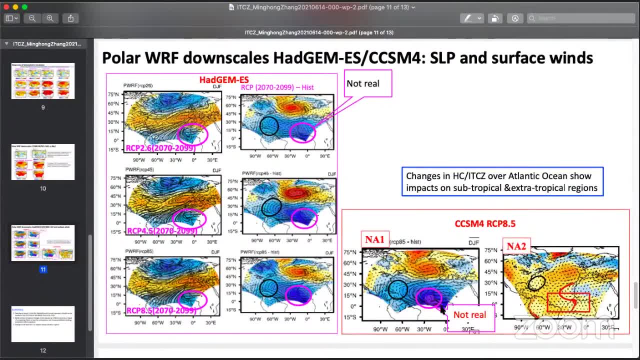 It is not a real response. Okay, I don't know why, but it is caused by the domain soil and boundary over the domain. Okay, Any other questions? All right? Thanks, Minghong. Thank you, All right. 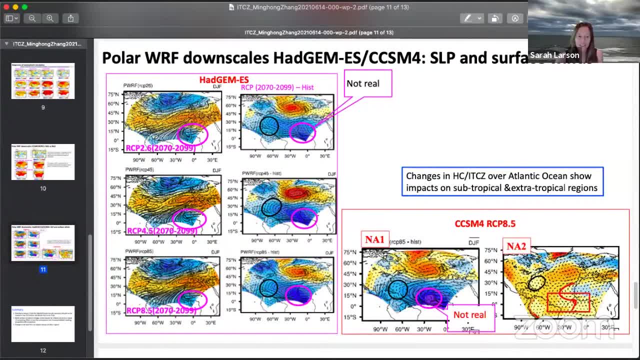 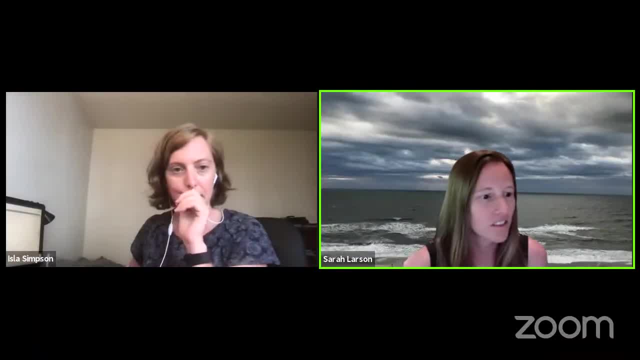 And just a reminder, we're in session two, So long-term climate variability and change, And so I'm your chair for this session, Sarah Larson. And so next we have Yana and Duong: Evolution of long-term temperature trends. in very, very short time. 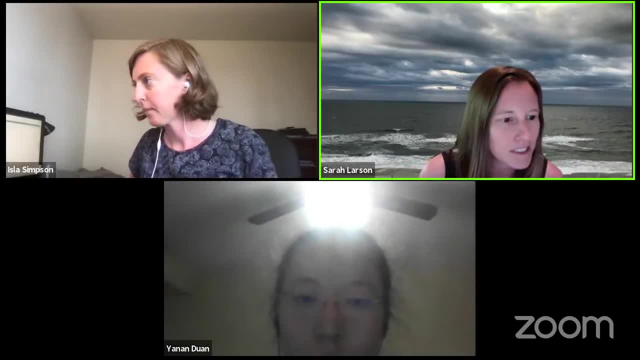 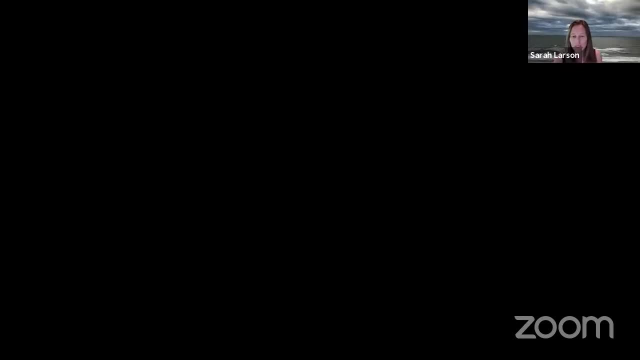 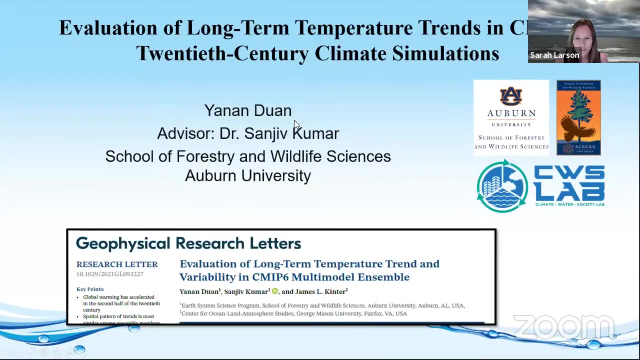 We're going to talk about long-term temperature trend and variability in CMIP6 multi-model ensemble. Hello everyone, My research topic is evaluation of the long-term temperature trend in CMIP6 in two-time period. We had already published this paper in geophysical research letters. 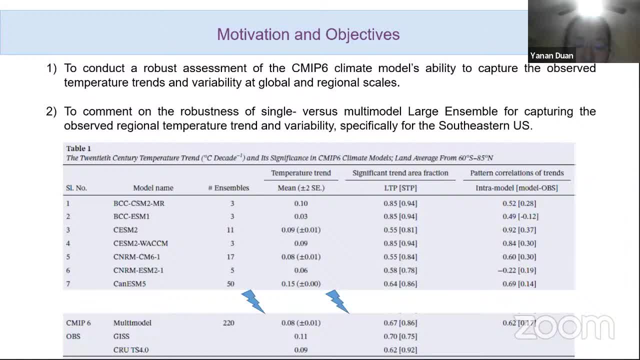 The motivation and objectives of this study is to conduct robust assessment of the CMIP6 climate model's ability to capture the observed and temperature trend and variability, And also we want to comment on the single large ensemble versus multi-model large ensemble's ability to capture the observed and temperature trend and variability. 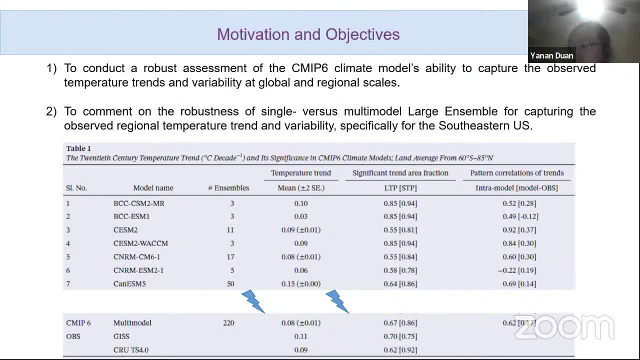 Especially in the sources, US and the global continent. This table shows the models we use in this study. Until we close this paper, we already had 33 ensemble member ensemble models, And some are very large ensemble models and some are very small. 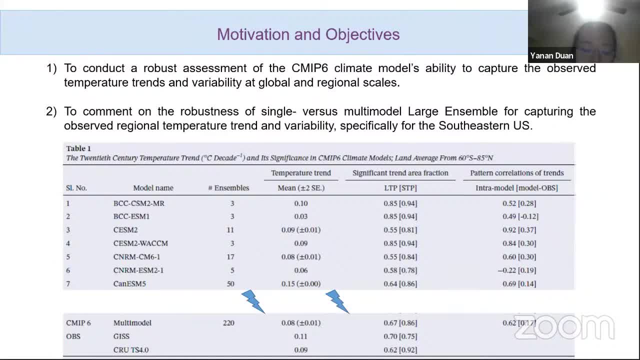 Only has one ensemble member In this table, the second column. this column is temperature trend with the unit of 0.3 per decade, And we also calculate the two standard deviation of the error To test the significance of the trend. we calculate the long-term persistence and short-term persistence. 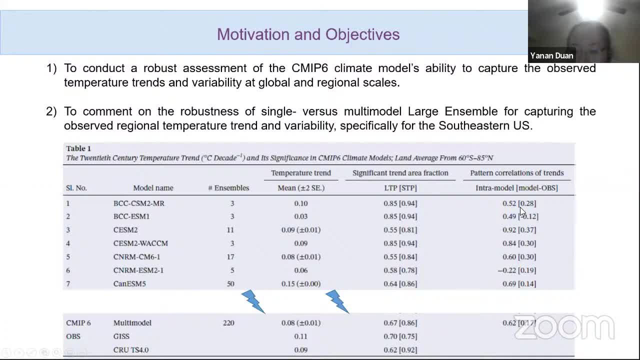 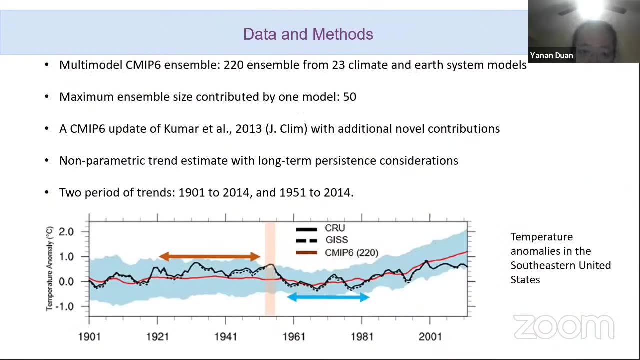 I will introduce it later. After that, we want to compare, we want to calculate the pattern correlation within the individual model and also the model observation In order to get a general idea about the model accuracy. The data methods I used, as I introduced in the formal slide, 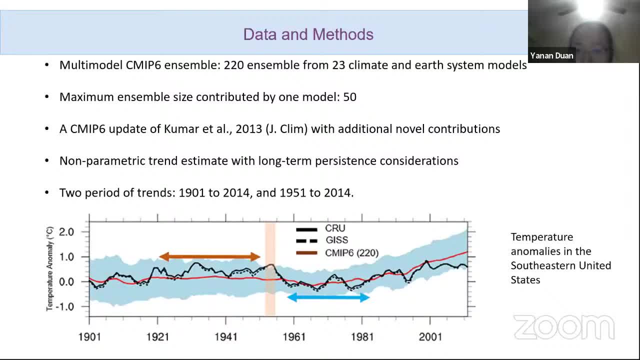 We use CMIP6.. We have 220 ensemble members from the 23 climate models And in this study we use a method based on COOMETAL 2030. The paper published in Journal of Climate, And we do some further study to discuss more about the CMIP6 properties. 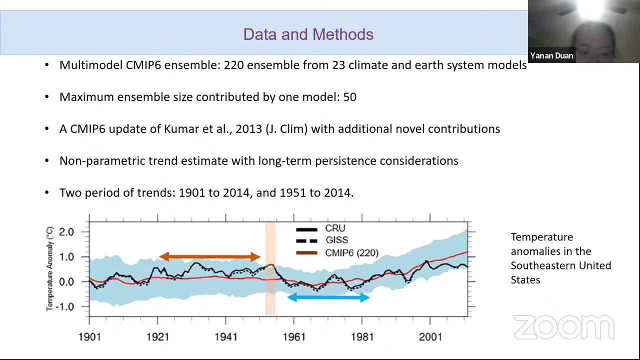 The long-term trend persistence calculation method is non-parametric trend estimation methods. The significant test calculation is. calculation methods are long-term persistence and short-term persistence, as introduced in the formal slide. We want to study the trend in two types: The trend in two time periods. 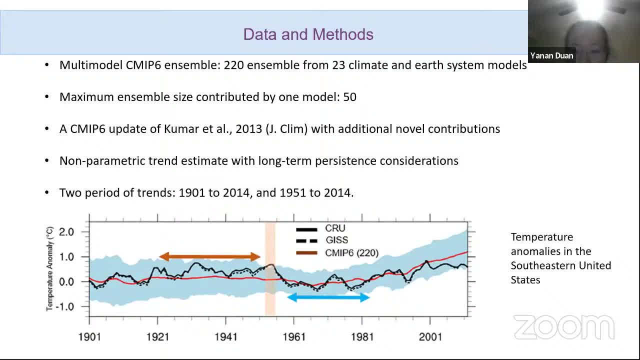 One is 1901 to 2014.. Another is 1951 to 2014.. Because, as the following time series figures show, within several decades and within 100 years the trend looks very different compared with each other, Especially in the source ECOS. 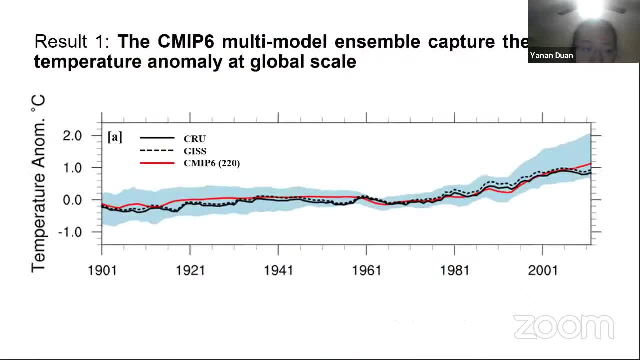 I will introduce more in the following slides. Here is the temperature. Here is the temperature normally in global continent region. We calculate the weighted average, And so we can find that the CMIP6 multimodal ensemble can capture the observed temperature normally at the global scale. 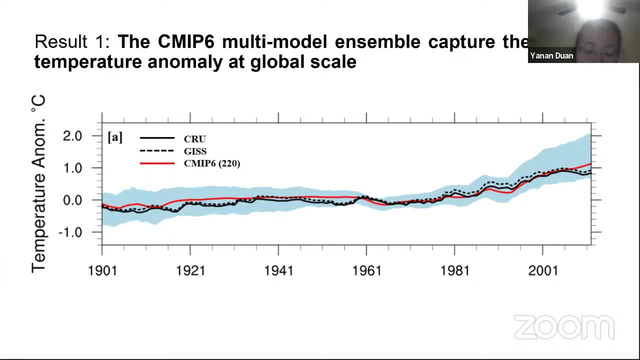 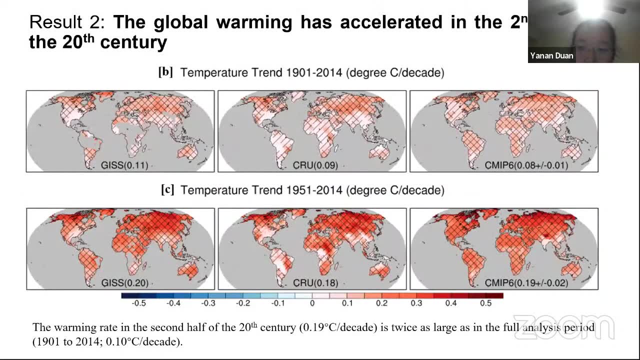 It corresponds to a very large uncertainty structure in the CMIP6.. I will discuss it further in this slide. In this slide we compare the temperature increasing trend for the two periods. We find that the recent several decades, the recent 64 years. 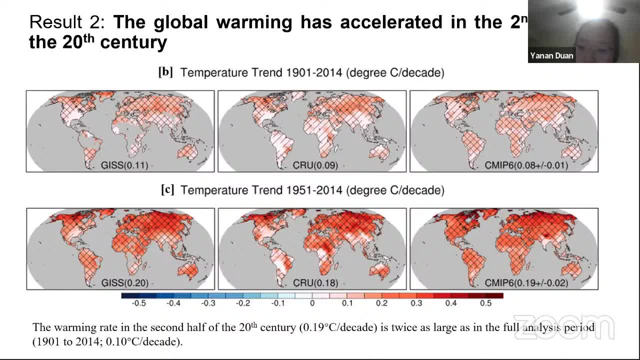 the temperature trend increased much greater than the long-term average, Almost double the accelerated rate with 0.2 compared with 0.08.. And also we find that the CMIP6 multimodal ensemble can capture the original scale variability much better for the short-term period compared with a very long-term average. 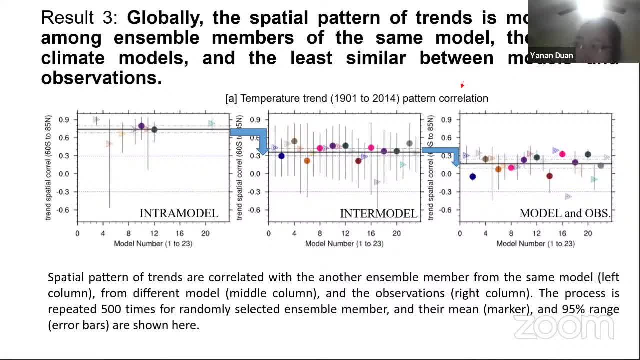 Then we calculate the trend pattern correlation within the individual model And within the 220 ensemble models, the CMIP6, and also the model observation for each individual model to get some idea about the model accuracy Globally. all of them are global continent results. 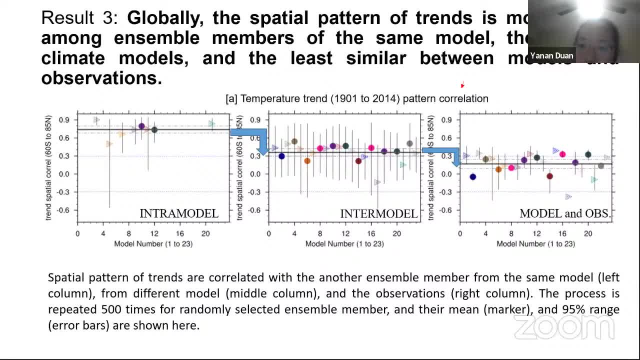 Globally, the spatial pattern of the trends is more similar among the ensemble members of the same model. It's much greater than the intro model comparison. The intro model means we randomly selected the ensemble members from the 220.. We take the CMIP6 as a poor tool. 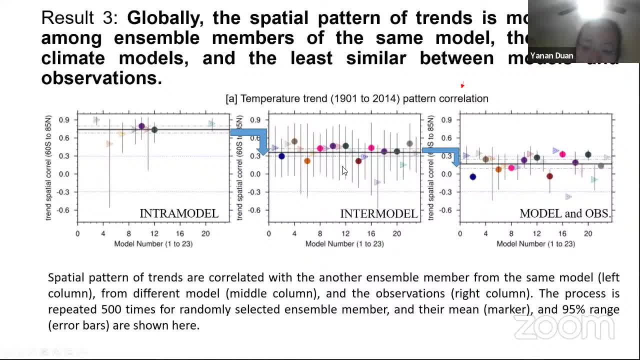 to calculate the intro model pattern correlation And this one is a model observation pattern correlation. So a higher number represents the accuracy we have For the random selected process. we repeat the process for 500 times, So the point represents the 500 times average. 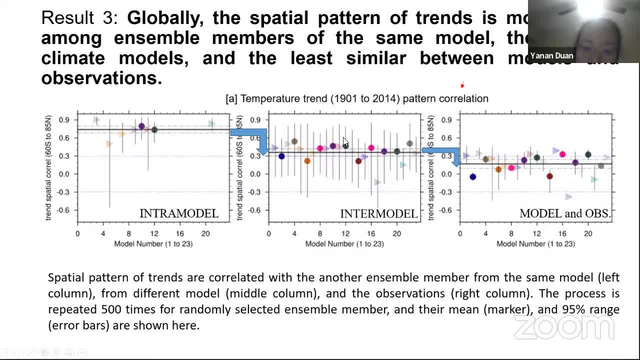 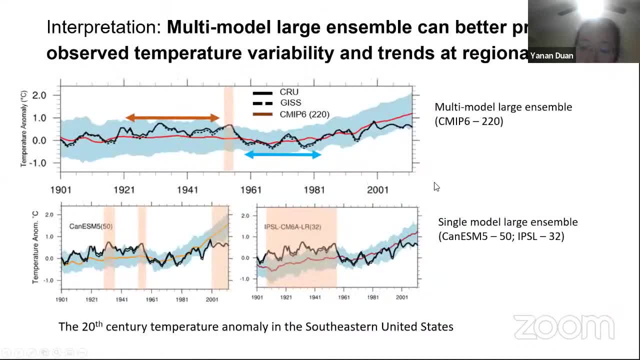 And here is a 95 percentile range of this correlation. So we want to compare the multi-modal large ensemble CMIP6 and also some single model with very large ensemble size. We want to compare the accuracy, The yellow- this one is global sources US. 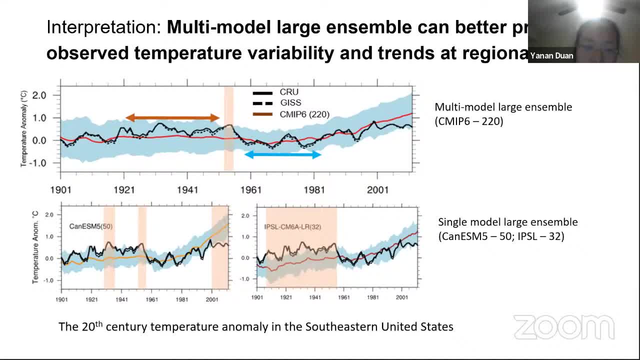 temperature normally average the time series from the 1901 to 2014.. And the yellow one: the yellow bar shows the yellow band shows the failure zone where the climate model cannot capture the observation. So the CMIP6 performance is much better than the single model large ensemble. 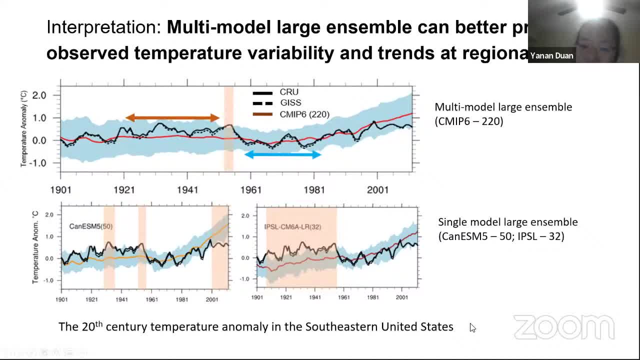 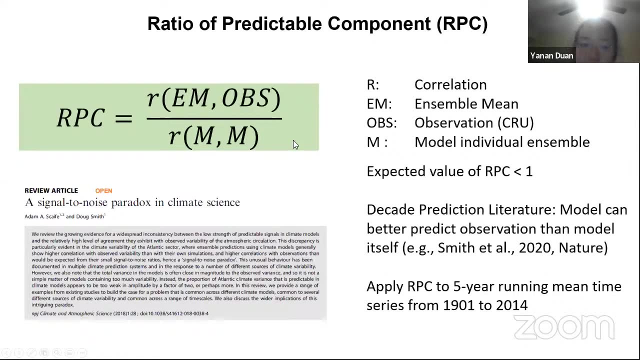 due to the large, very large uncertainty range. But it will increase another problem, the signal-to-noise ratio problem. So I will introduce it later In order to test the model signal-to-noise paradox. we have to solve this problem. 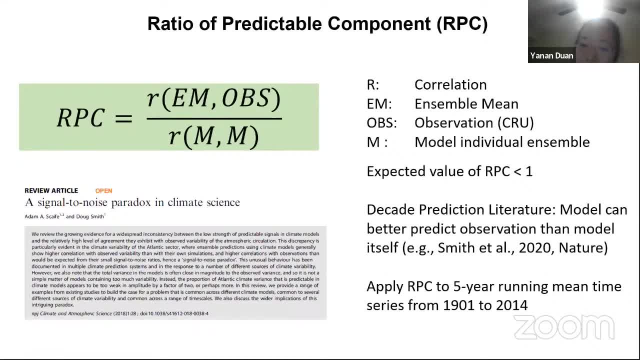 because the model. sometimes the model can predict the observation much better, but it is caused by the large uncertainty in the model itself. So we want to test the balance if it requires it or not. The RPC is the algorithm of predictable components. 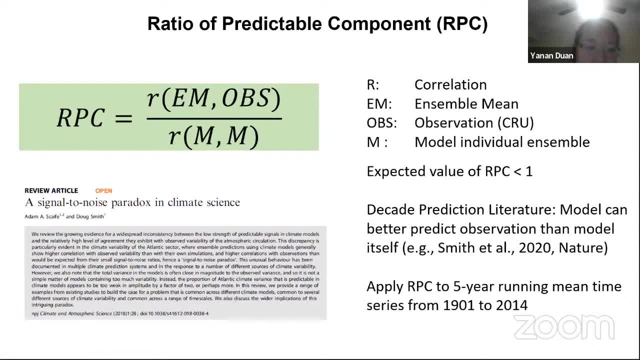 This method is introducing the signal-to-noise paradox in this paper And in this matrix. the numerator is the correlation between the ensemble mean and observation. It means the model's ability to predict, to capture the observations. The denominator is the model versus model correlation. 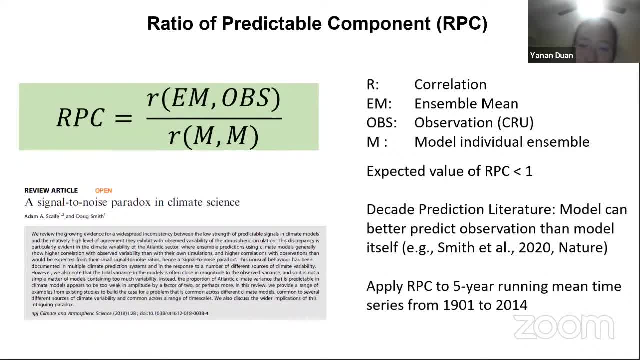 It means model model's ability to predict itself. In the perfect situation, the RPC should be one, but we expect value to be smaller than one, since the model can predict itself much better than to predict the observation In this study. we use five years running. 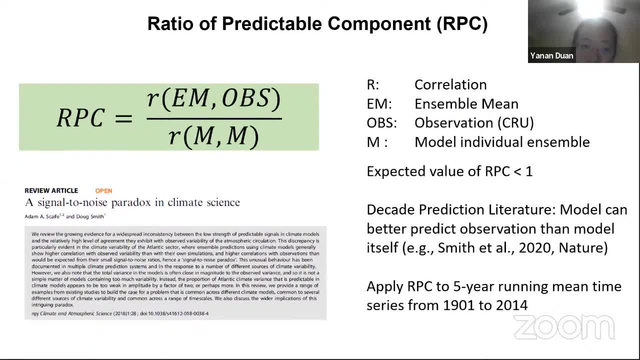 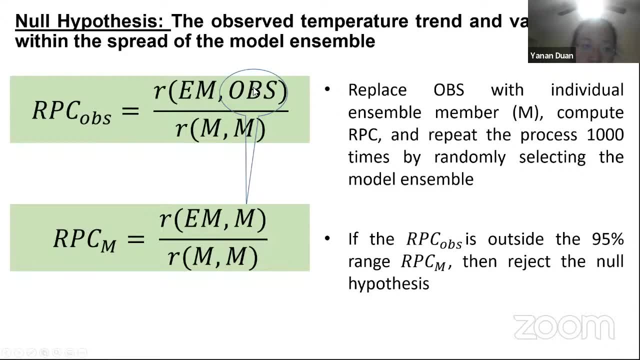 time to calculate the RPC And to in order to test the significance of the RPC, we use some. we use non-hypothesis, as the observed temperature trend and variability lie within the spread of the model ensemble. It means if we replace the observation, 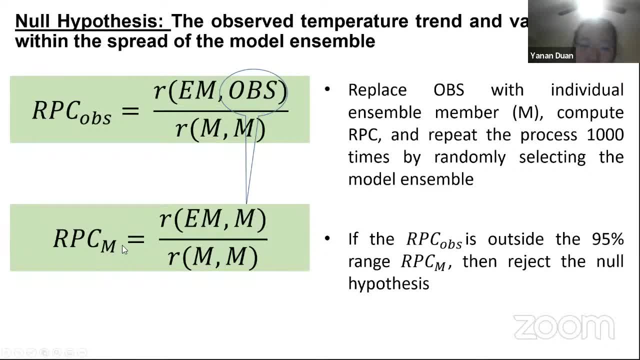 with any random selecting model itself. the RPC should be the same. It means the model can capture the observations. So we want this situation to be the true case for the model we have. And if we reject non-hypothesis, it means if we replace it with a model. 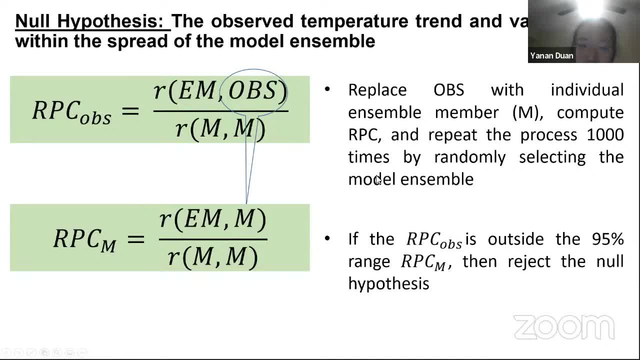 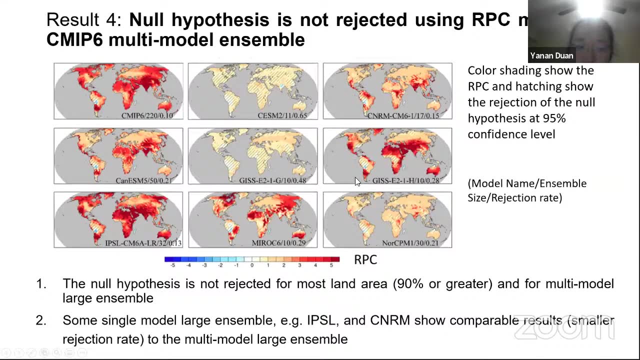 the RPC should be different. We will repeat the random select process one thousand times, So we will show the 95% percentile range. Here is the results we have. This one is semi-P6.. Another is ensemble models with a number greater than 10,. 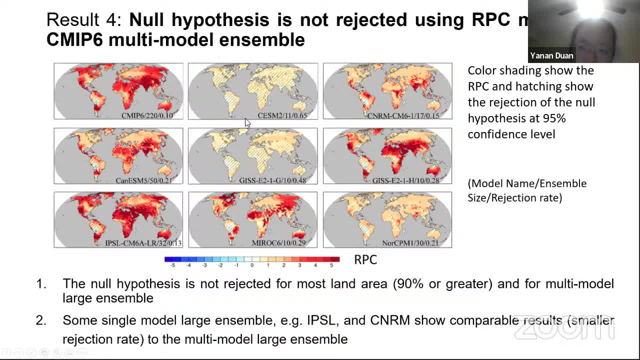 greater or equal with 10.. In the RPC: RPC value. if the absolute value of RPC is greater than one, it means model can predict observation much better than predict itself. If it is smaller than one, the inverse is right: The model can predict itself much better. 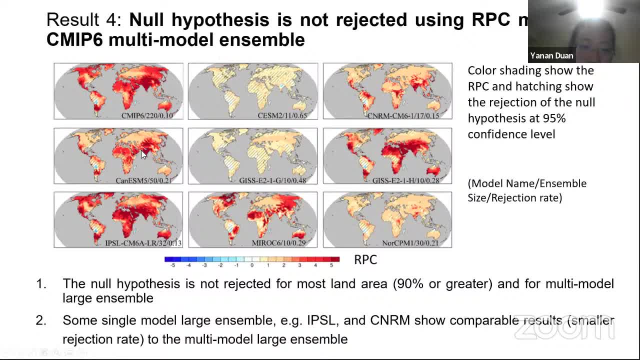 than predicts observation. So in this figure the rejection rate means the model cannot predict the observation much better than predict itself. So the rejection rate always occurs in the yellow range. There is no wonder semi-P6 has a very low rejection rate, because it can better predict the observation. 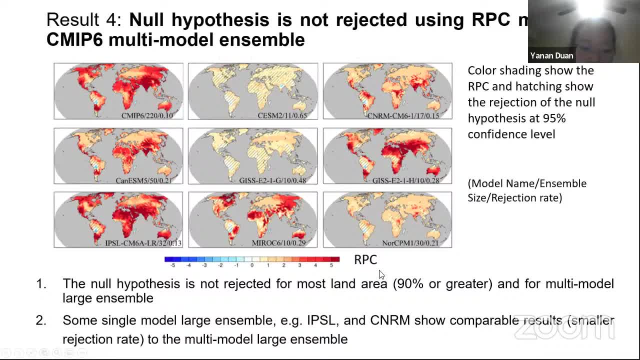 And the same situation occurs in some relatively small single models Like the IPSR and the CNRM. They have a much smaller ensemble size: IPSR only with 32, and also the CNRM- They only have 17,. but the rejection rate is low enough. 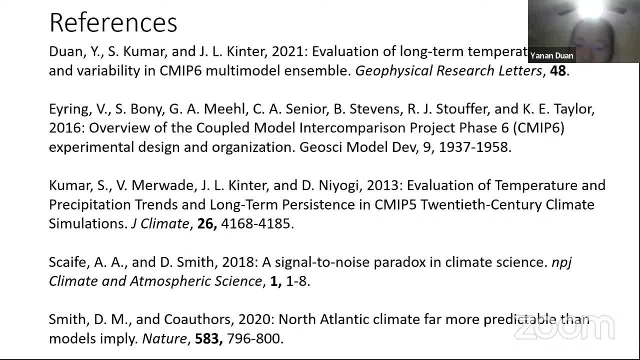 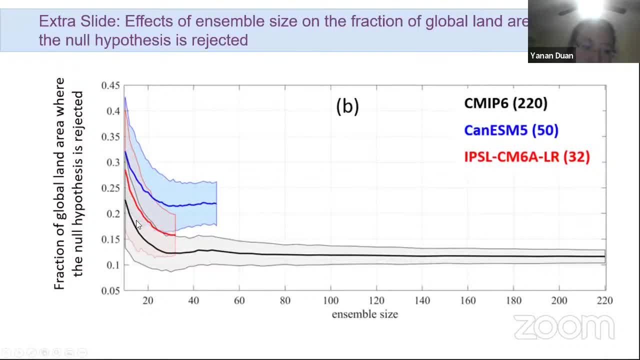 So here, here is the references I use, And this one is ensemble size and also ensemble size. so ensemble size relation with a fraction of the rejection rate. If we increase ensemble size, the rejection rate decrease, as we expected. It seems like if over 60,. 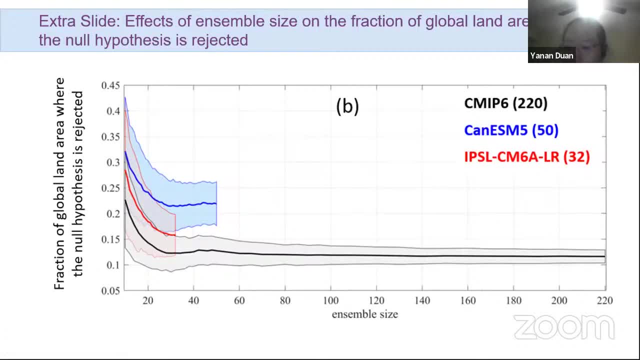 it goes to saturation. That's it, Great thanks. Do we have any questions? Yeah, I can ask one. Have you been able to look at any of the downscaled versions of CMIP5 that are kind of geared towards looking at the more specific? 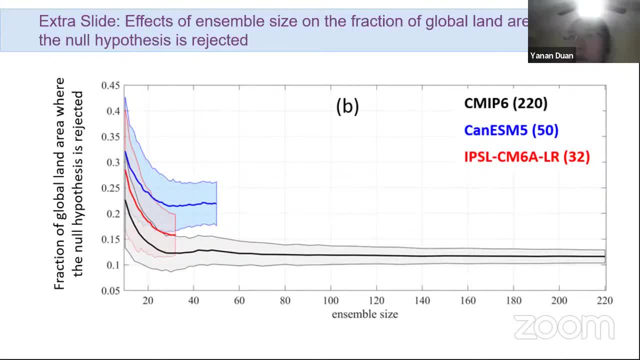 regional differences. Oh no, No, not yet. It's a good suggestion For the resolution problem. yeah, when we do another analysis about CSM29, we find such problem with a different resolution, results will be slightly different. We need to do more in the future. 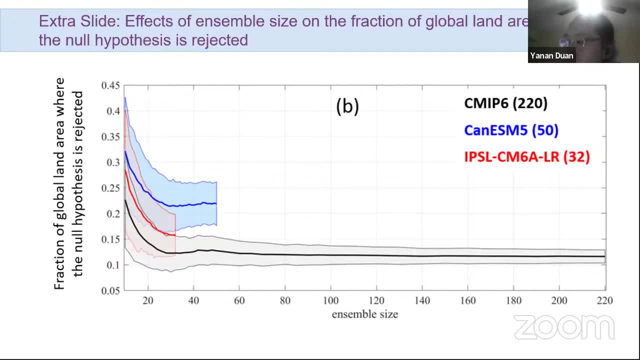 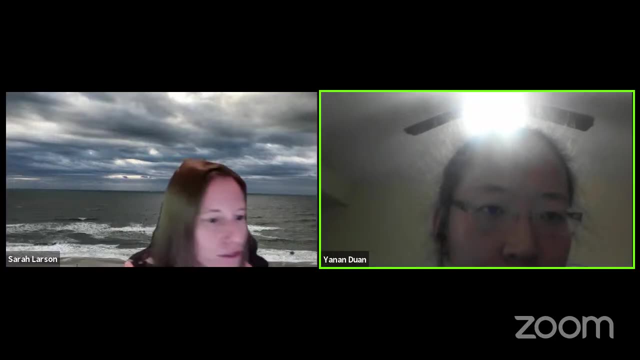 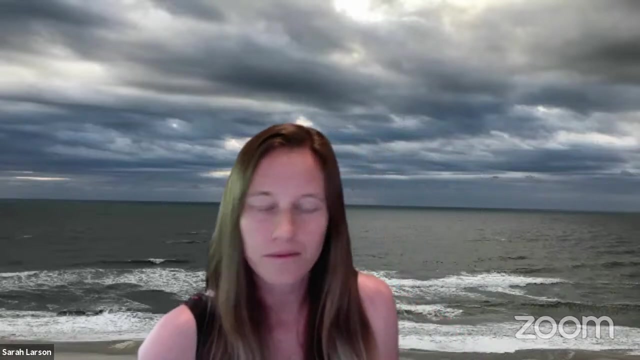 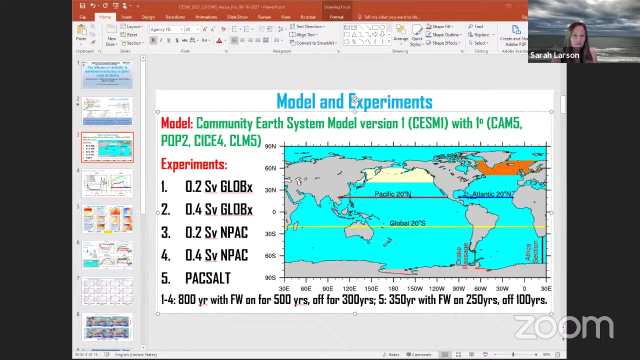 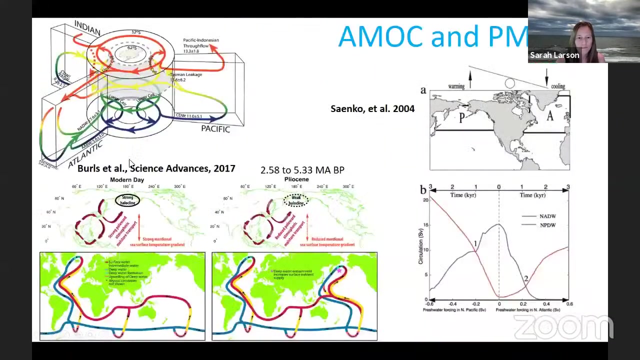 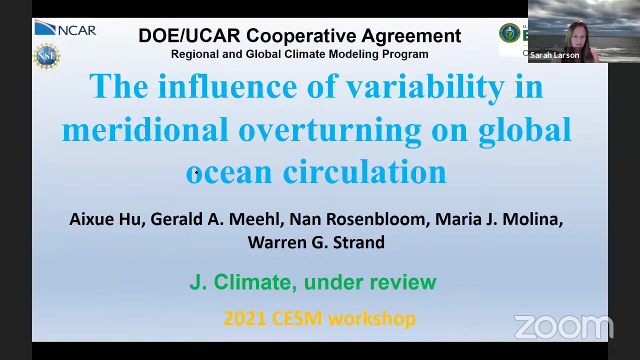 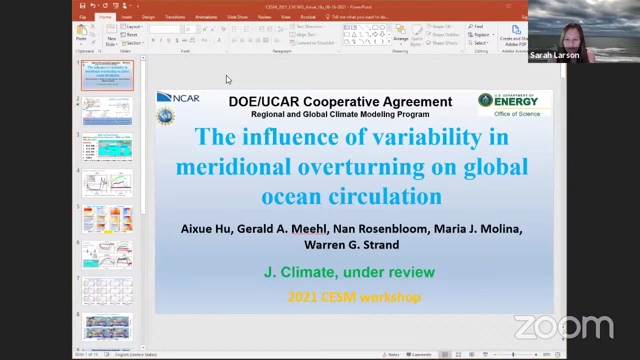 Thank you for this. Any other questions? All right, we'll move on to the next talk. So next we have Aishu Hu, with variations in meridional overturning circulation and their influence on global ocean. Aishu, I think you're muted. 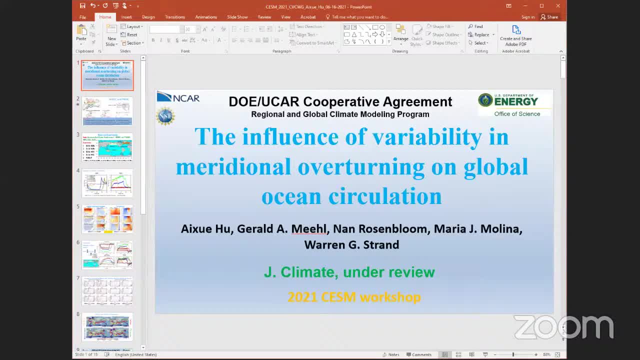 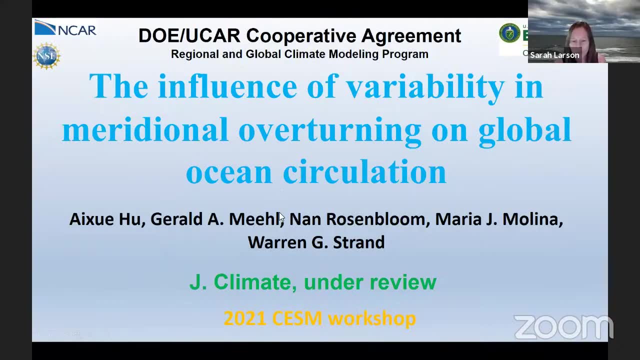 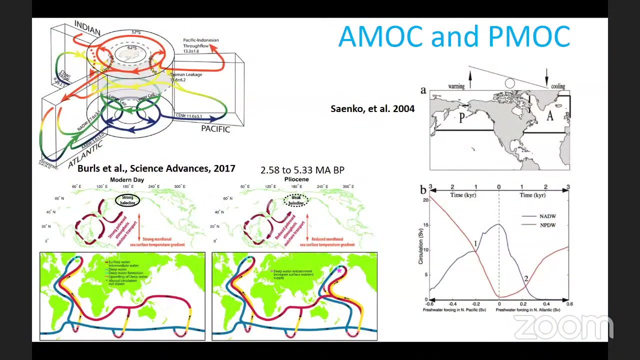 Okay, now It's not. Oh, perfect, Okay. This work is in collaboration with Jeremie Lange, Rosenblum, Maria Molina and Gary Stratton. Right now, the paper is under review by Jeremie Lange. The Atlantic Meridional Overturning Circulation. 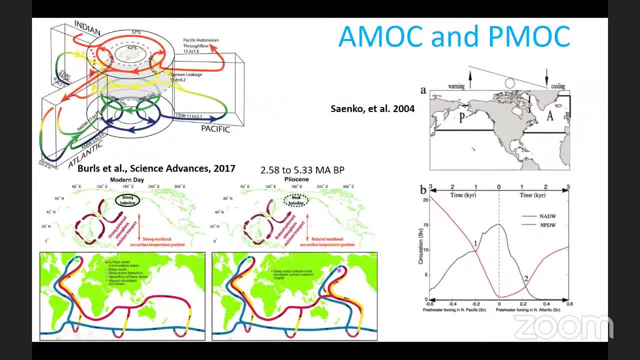 or AIMA, is a global-scale ocean circulation which transports upper ocean warmer and saltier water into South Pole and North Atlantic, where this water's loose heat becomes thin and sink to depth and flows southward and outwells elsewhere over the world ocean. 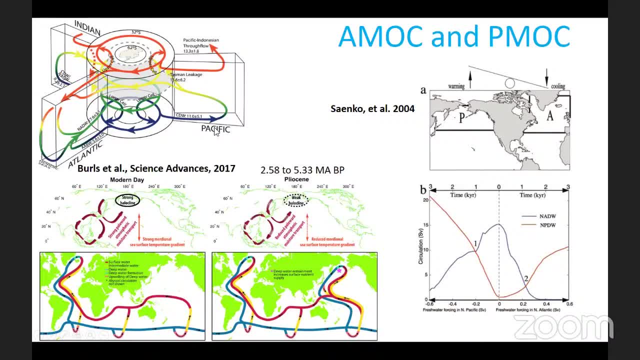 Under present conditions there's no deep convention in the South Pole and North Pacific, But studies show that about 2.5 to 5 million years ago there might be in Aishu both the AIMA and the Pacific deep meridional overturning circulation. 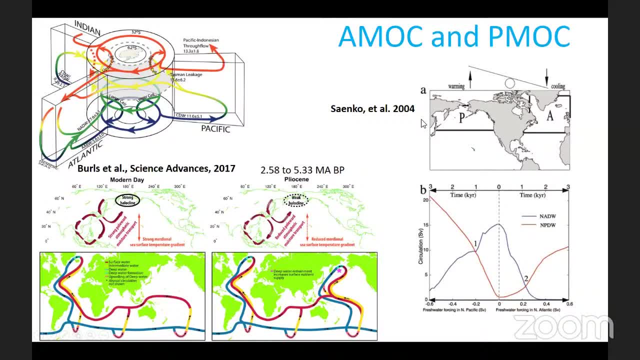 or AIMA. A similar model study showed that a strengthening of the AIMA can cause an awakening of the AIMA and a strengthening of the AIMA. So in this research we asked two questions. One is whether AIMA and TMA form a natural pair. 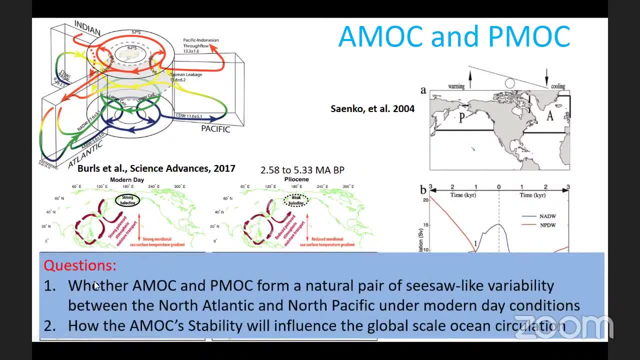 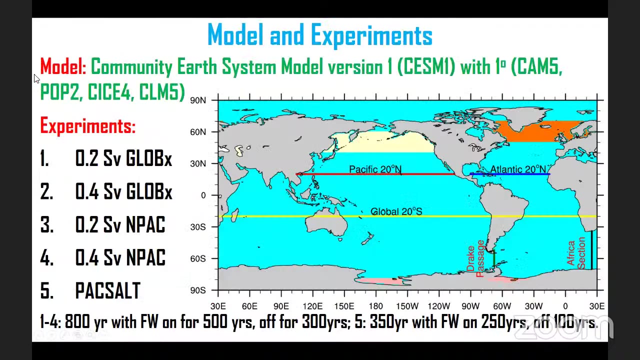 of sea salt-like variability between North Atlantic and North Pacific under modern day conditions. Two is how the AIMA's stability will influence the global-scale ocean circulation. To do this, we use the AIMA and TMA, we use the TSM-1. 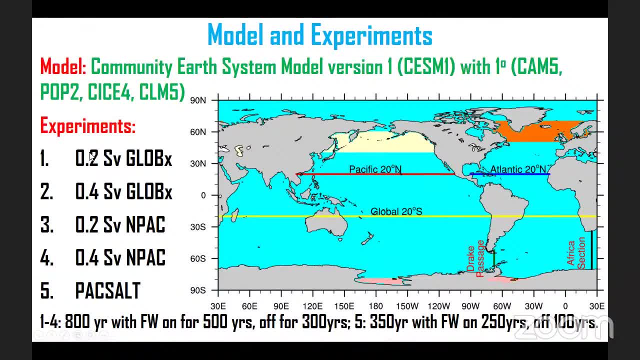 as one-degree horizontal resolution, carried out five experiments. For the first four experiments, we ran for 800 years, with fresh water floating on for 500 years, and up for 300 years. For the last experiment, we ran the simulation for 350 years. 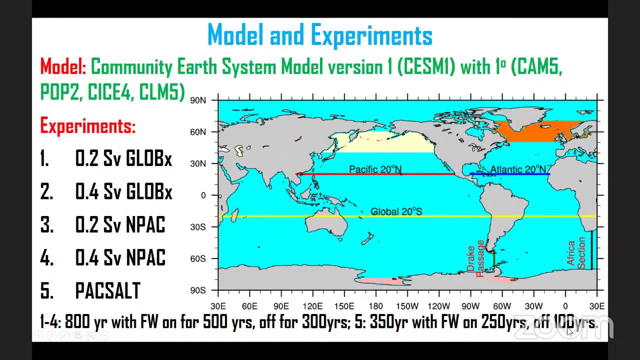 with fresh water floating on for 250 years and up for 100 years. In the first four experiments, additional fresh water floating is added into South Polar North Atlantic between 50 and 70 kilo knots with a strength of 0.2 or 0.4 virgals. 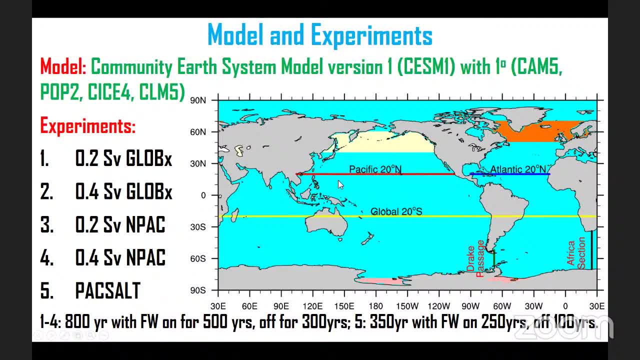 This fresh water floating is compensated elsewhere in the world ocean of the global-stealthy environment and compensated at the South Polar North Pacific only in the MPEG experiment. For the last experiment, we put additional salt into South Polar North Pacific and this salt blot is compensated. 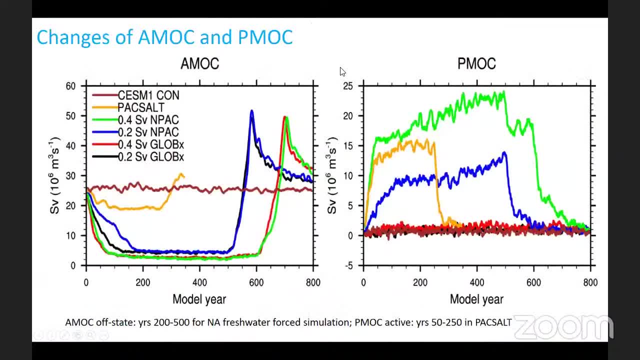 elsewhere of the world ocean. This is the derived AMOX and PMOX. The definition of this index is the maximum of the Atlantic meridian stream function below 500 meter depth for AMOX and the Pacific meridian stream function the maximum below 500 meter depth for PMOX. We can see that in the first four experiments both 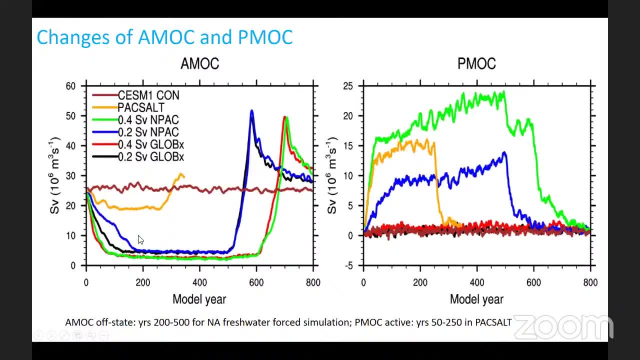 these simulations show a collapse of the AMOX, but when the first water function is compensated and not specific, the collapsing is slightly slower than that compensated by the global ocean When the first water function stops at year 500, the experiment with Pound 2's. 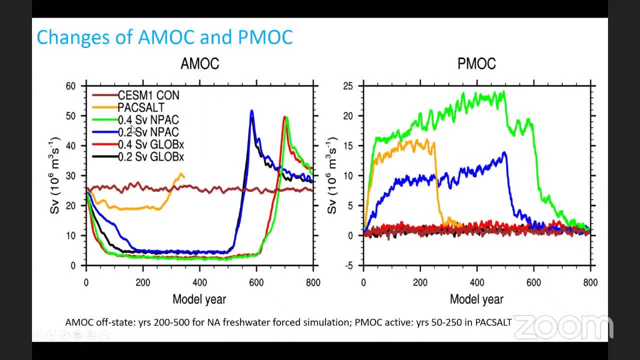 virtual forcing is recovered immediately, but with Pound 4, it's delayed by 100 years. but they both overshoot In the Pacific side with the compensation in a global there's no PMOX formation. The PMOX formation is only happening in two experiments with compensation as a non-specific. That means 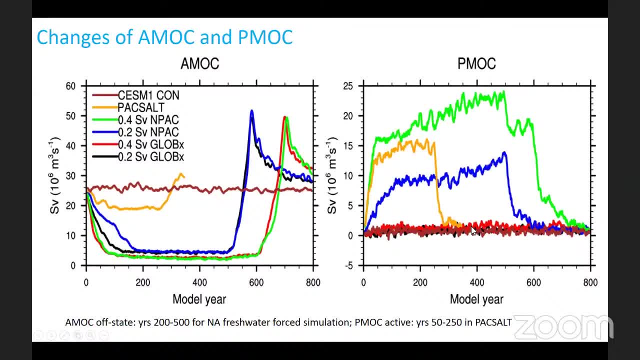 the collapsing of AMOX itself will not automatically cause a setup of PMOX in our simulation. So to test a setup of PMOX whether it will affect the AMOX, we add adenosol in the sample, not specific to force the setup with PMOX. 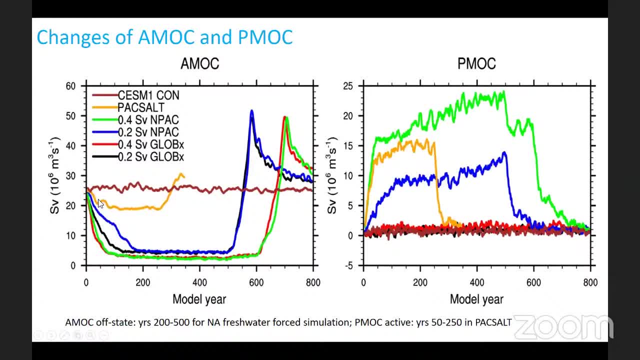 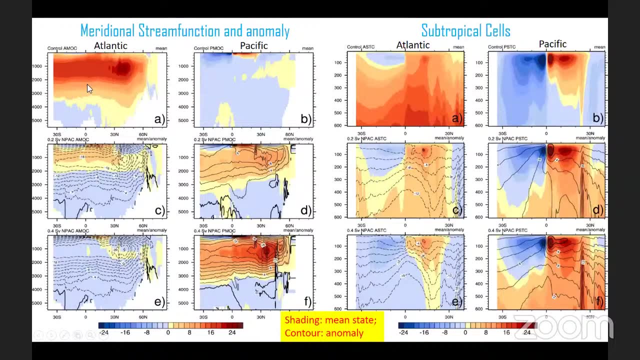 And then we look at Atlantic. we do see awakening of the AMOX by strengthening of the PMOX. That means if we force APOC to setup it does affect the circulation in the Atlantic. This is the meridian stream function in a control range for the Atlantic and Pacific And this is 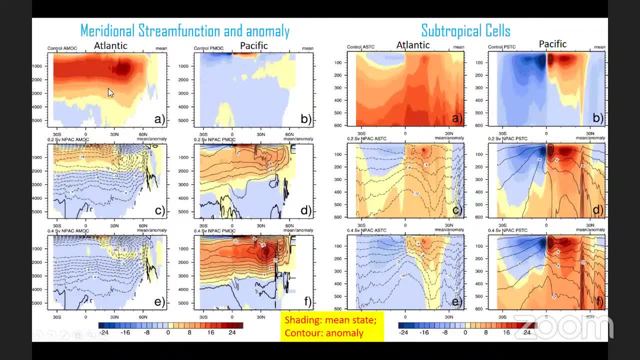 in the experiment with PMOX. This is the meridian stream function in a control range for the Atlantic and Pacific And this is in the experiment with PMOX. This is the posture. We can see that in the control range there're strong As overthrow things in Atlantic but mostly absent in Pacific. 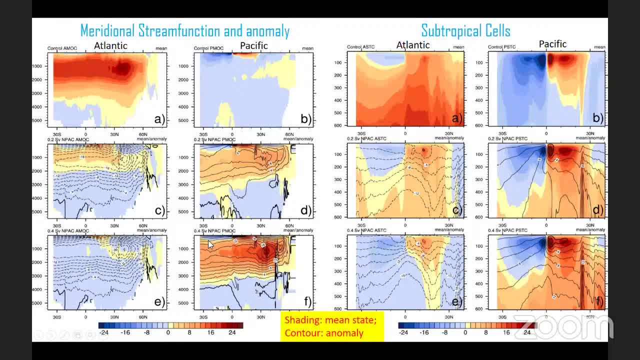 There's, you see, a similar meridian stream function in the Pacific and in Atlantic in the control range, but right now is that the AMOX causing collapse. This change not only affects the deep circular, it also affects the shallow circulation, such as the subtropical cell in the control fireland. 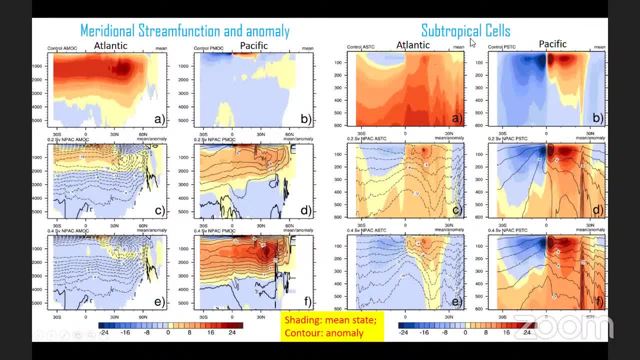 The selection is also affected by shallow circulation, such as the subtropical cell In the control range. the Atlantic southerly cell is certainly also affected by這邊 fazem Dude and ends with. theador came out with tomato inflammation in the location. 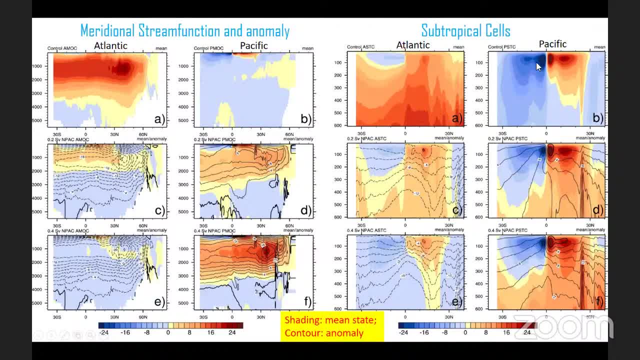 In the control range. the Atlanticwerk is intense plant growth. The radio 가장 often remains in thepause of the AHMCA cycleיide control run. the Atlantic subtropical cell is weaker than that in the Pacific. When the A-mark collapse and the T-mark set up we see the strengthening of the subtropical. 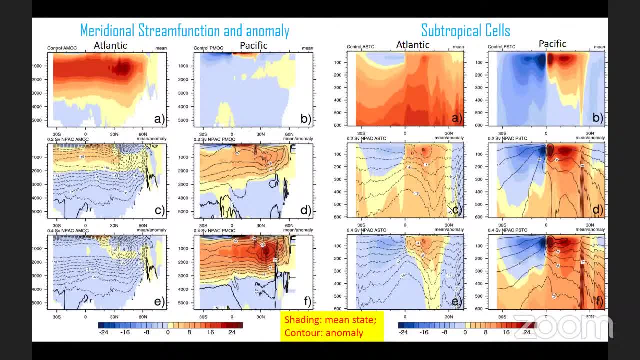 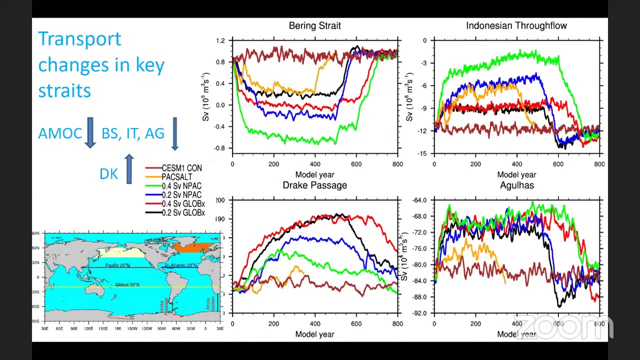 cell in the South Atlantic and the weakening of that in the North Atlantic. In the Pacific side, with the set up of the P-mark, the shallow orbital circulation in the Pacific is weakening in the South Pacific but strengthening in the North Pacific. Since the A-mark is the global scale orbital circulation, the change of A-marks also affects 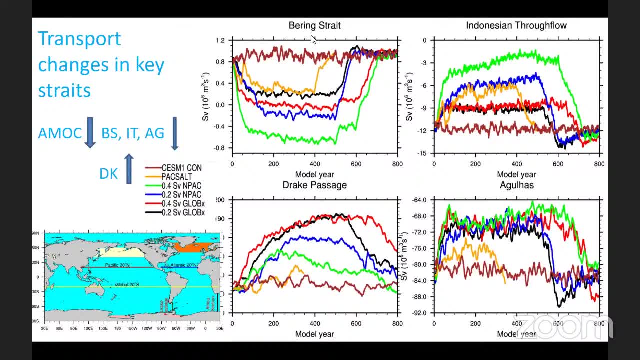 the circulation in other places, which was, for example, the Bering Strait, the Neatest Roof Lobe, Big Passage and Adelaide Park. We can see that the weakening of the A-mark causes a weakening of the Bering Strait, which is the T-mark, and also a weakening of the Neatest Roof Lobe and the weakening of the. 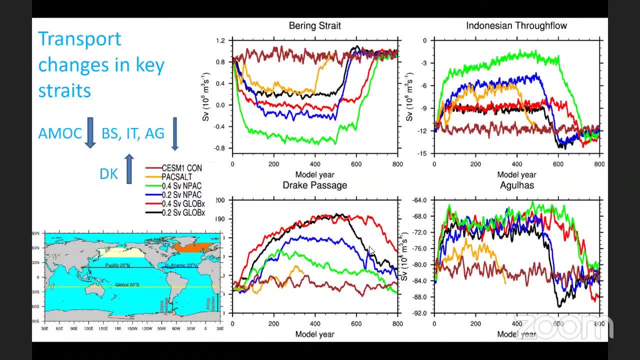 Adelaide Park but a strengthening of the Big Passage which is the set up of the T-mark, The Bering Strait T-mark is further weakening and also further weakening in the Neatest Roof Lobe, but the effect on the Adelaide Park is small. 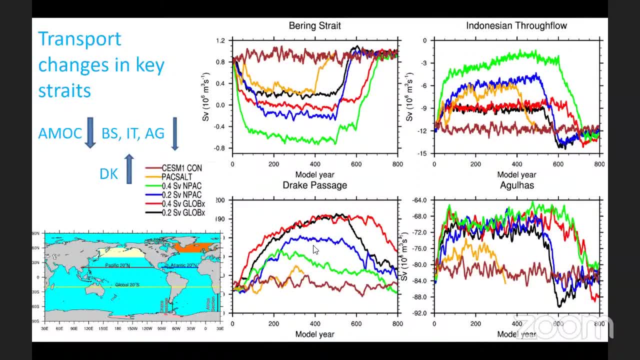 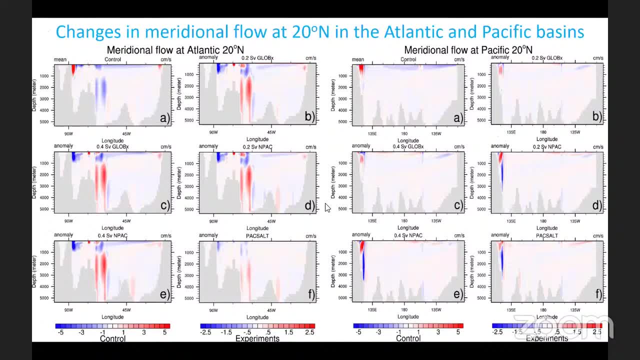 And the strengthening of the Big Passage T-mark is also weaker when the T-mark sets up. Thank you. Next I will show an example of how it affects the three-dimensional ocean circulation as the changes of meridians flow at 22 degrees North in the Atlantic and the Pacific. 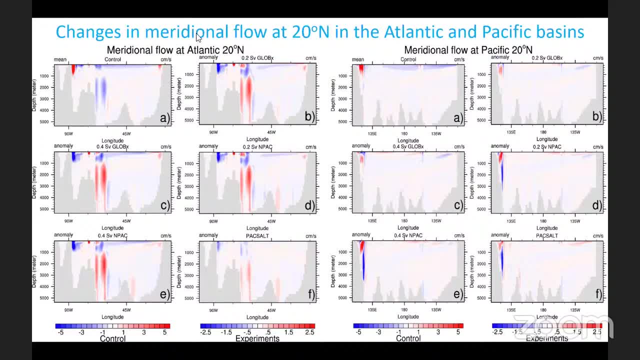 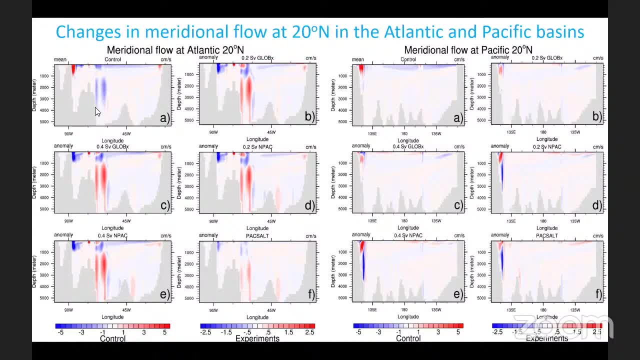 In the control. this represents the northward direction. The helium flow at 22 degrees North is a weakening effect on the meridians flow. This is also reflected in the southward return current of the A-mark. With collapsing of the A-mark in this poor experiment we see very similar changes of 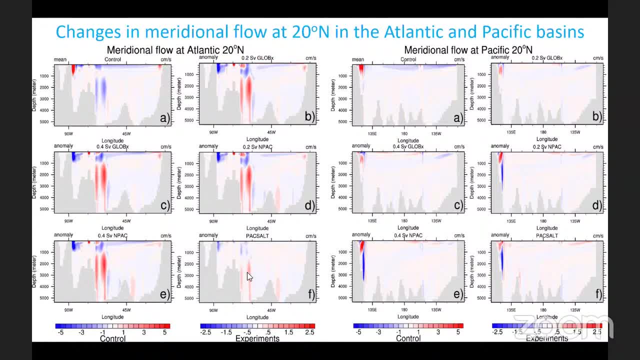 the meridians flow in the Atlantic—a weakening of the Gulf Stream and almost collapsed of the southward return current In the Pacific south experiment. we also see this weakening of the Gulf Stream and weakening of deep current In the control run. we see this non-sword-flowing crucial current. 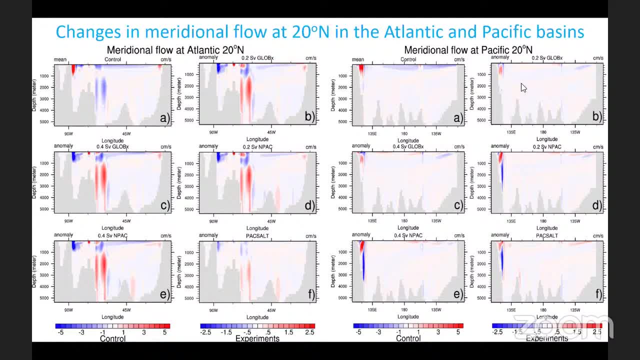 With the collapsing A-mark, without the set-up of C-mark, this crucial current, the deeper part, is strengthened by the surface after the evaporation. With the set-up of C-mark, we see a significantly strengthened, non-sword-flowing, crucial current. 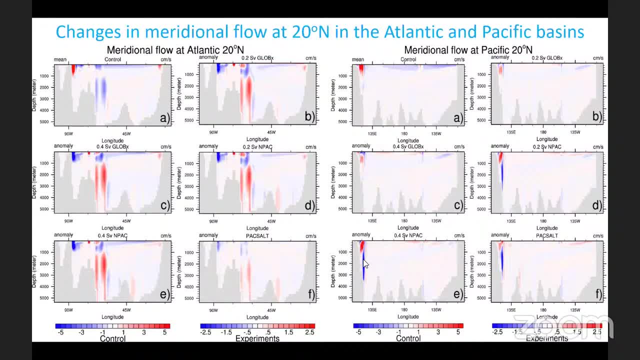 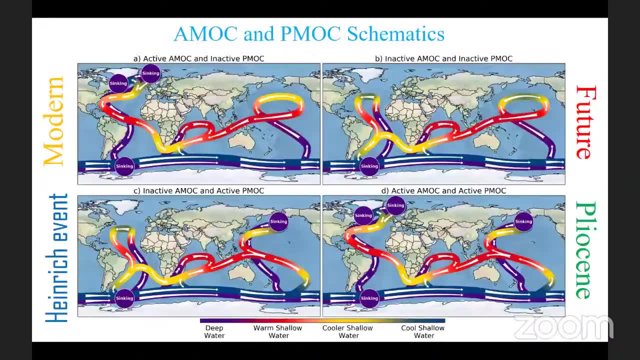 and also this strong sulfur-flowing western boundary current which represents the return flow in the deeper part of the ocean. So in our experiment, basically, we have four different states of A-mark and C-mark: Active A-mark and inactive C-mark, which represent the modern-day conditions. 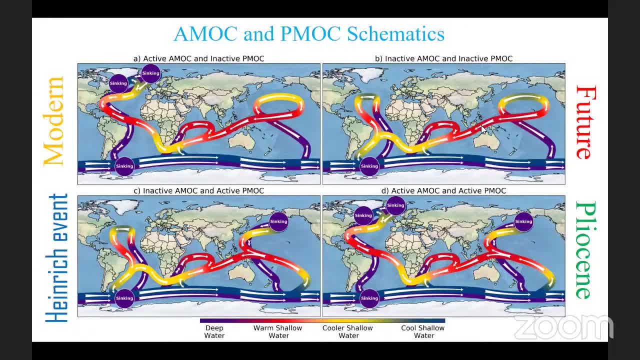 And inactive A-mark and inactive C-mark which may represent the future climate change, And inactive A-mark and inactive C-mark which may represent the future climate change. And also we have a state is that we have active C-mark but collapsed A-mark. 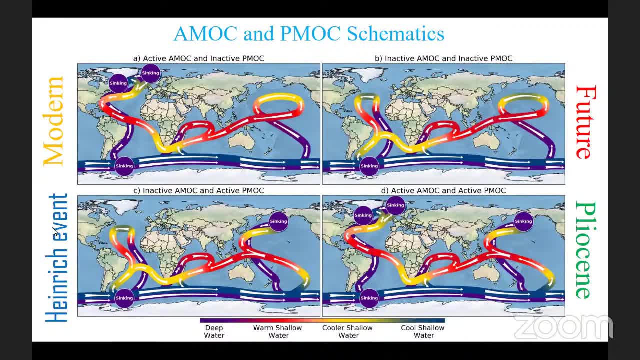 This situation may represent a hundred events during the last declassification period And the last one is we have active A-mark and active C-mark. This may represent the failed state conditions But under our modern-day conditions, except this active A-mark and inactive C-mark state, 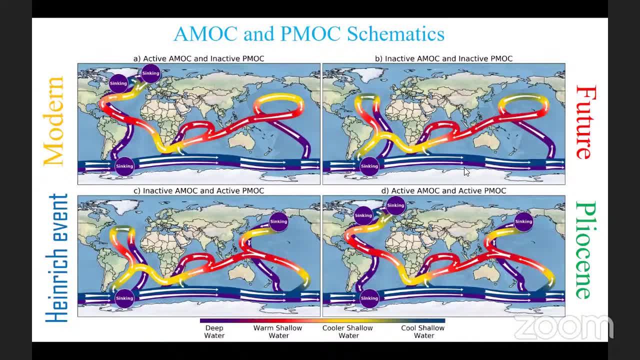 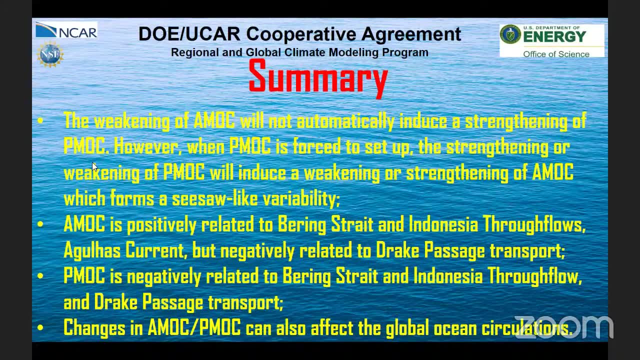 the other three states are the same. They are not stable. So, in summary, the weakening of the A-mark will not automatically induce a strengthening of the T-mark. However, when T-mark is forced to set up, the strengthening or weakening of the T-mark will induce a weakening or strengthening of A-mark. 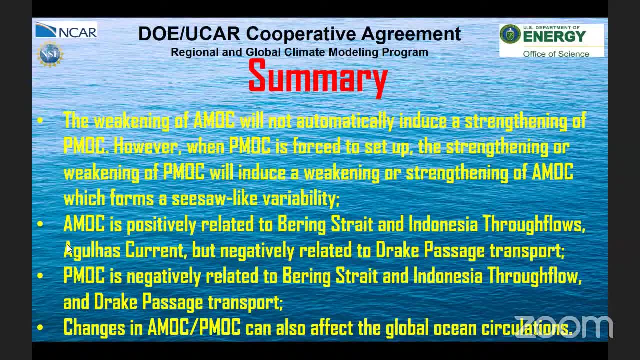 which forms a C-solid variability. An A-mark is potentially, but is positively, related to a variant 3 in either through-flow and above the current. The next is related to a big heavy sunspot. For the T-mark, it is the next related to a branching sunspot and an immediate through-flow and also a big heavy sunspot. 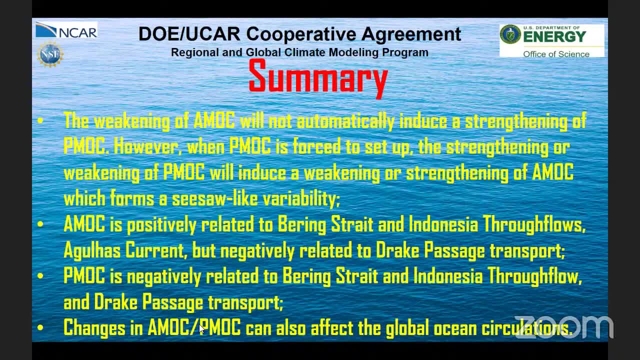 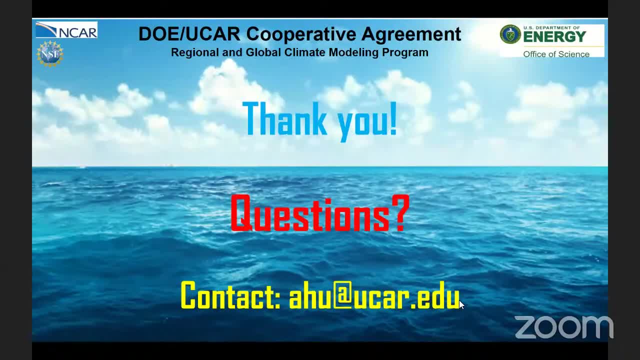 Our results also show that the changes in T-mark and A-mark can also affect the global ocean circulation elsewhere. Thank you. Thanks for that perfect on-time finish. We definitely have time for a few questions. We have one from Gokhan, Just a quick question. 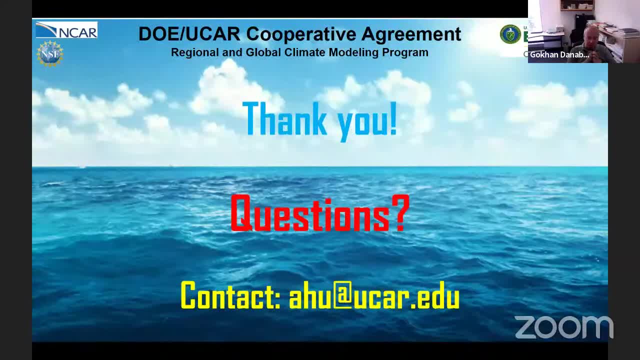 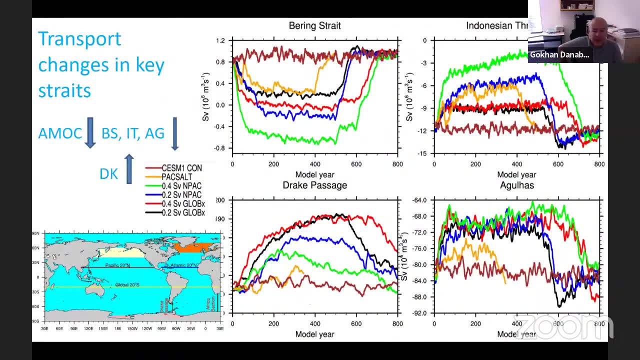 What is the mechanistic relationship between A-mark, P-mark and the Drake Passage transport? How do they essentially impact each other? A Drake Passage transport is when we weaken the A-mark. basically, it causes a strengthening of the southern ocean range, which is strengthening the Drake Passage transport. 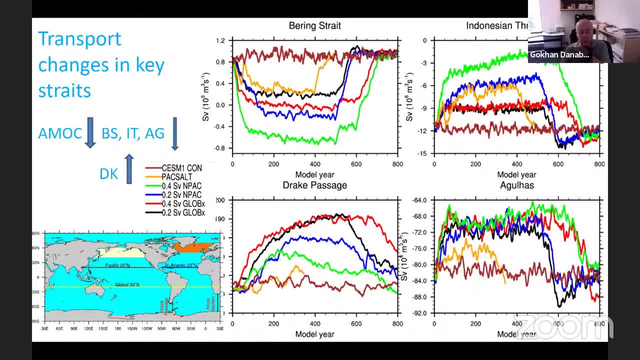 Okay, so it's through the wind surface forcing, but not through the ocean stratification. Not exactly through ocean stratification, But on the other hand, with SQ-A-mark there's a flow from the Atlantic into the Pacific. It's about a field virgo. 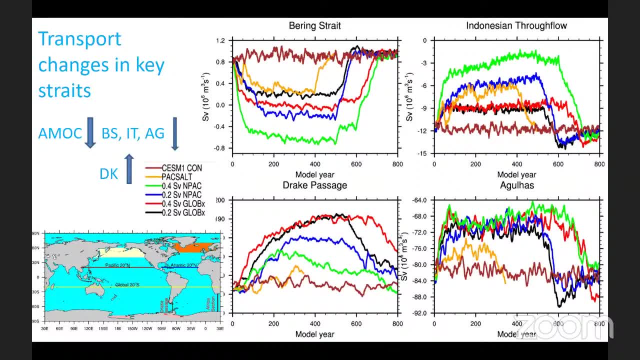 With a collapsed A-mark. that flow is beginning to weaken, Also current to the strengthening of the Drake Passage. But if it's small we can still see. Okay, thank you. Other questions? Yeah, I had one. You showed on one of your earlier slides that two of your experiments had an A-mark collapse. 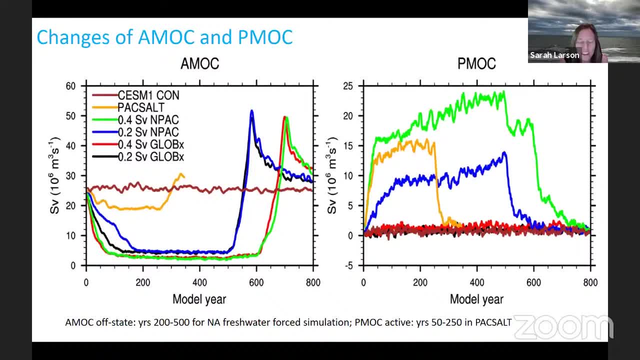 or there were three and there was this overshoot. Do you have any idea what's dictating the amplitude of that overshoot? Because it seems like each of those experiments goes to the same, close to you know, 50 spheretropes. 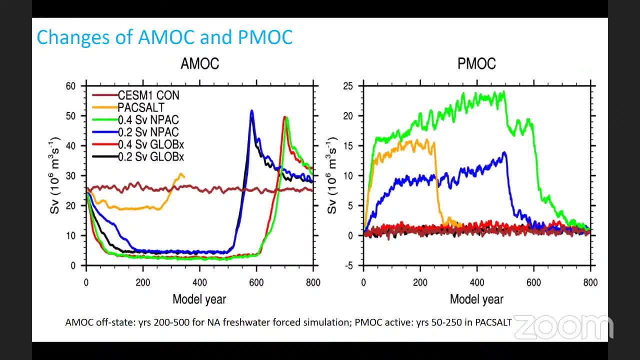 Yes, I have some idea When we have the A-mark collapse because we use this very strong forcing. it's just a filter function on and off. So when we apply this forcing, some of the fresh water actually we put into the surface. 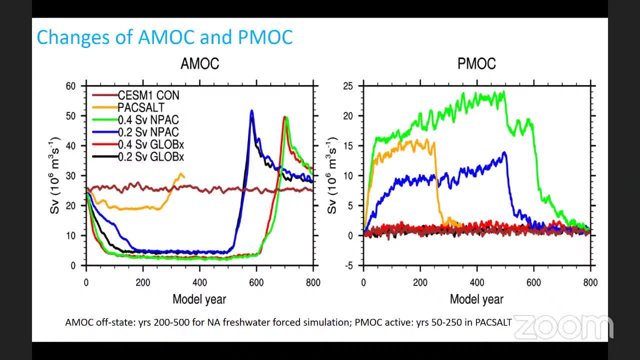 it will transport into the sub-surface and then it basically stays there and A-mark collapse And when the fresh water falls and stops, we will have an initial start because of the cooling in the sub-polar North Atlantic and it causes the strengthening of the A-mark. 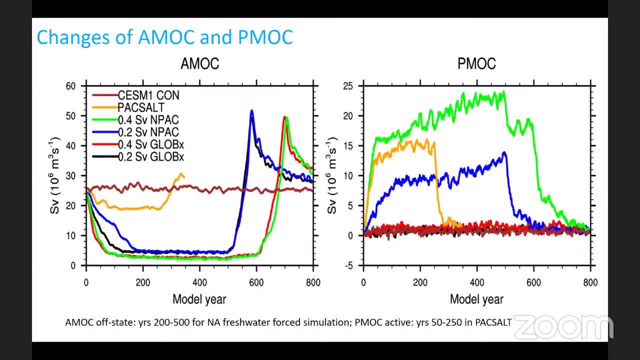 And that strengthening will cool more of this saltier water actually from the subtropical Atlantic into the subtropical Atlantic, which is a compound effect with the subsurface water. actually now it's a bit fresher, That's why it's overshoot. 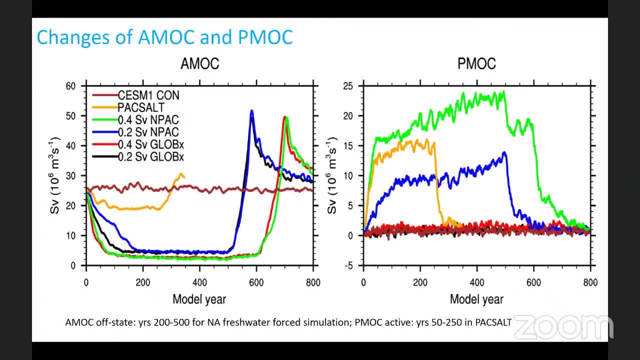 But why is it that you go to like a 50 spheretropes? I haven't looked at that yet. All right, thanks, We'll move on to the next talk. The next we have, Xiaowei Li. The title is: 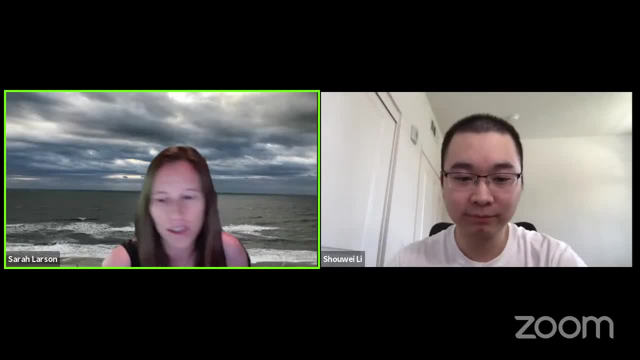 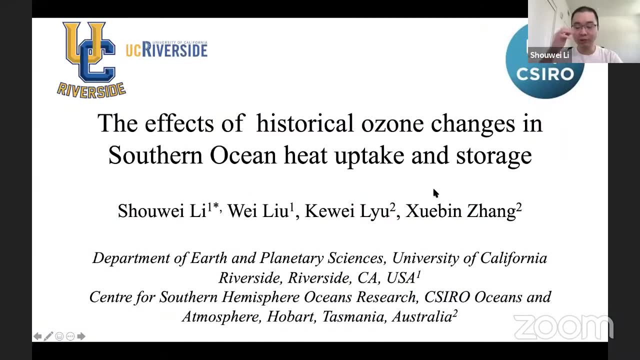 The Effects of Historical Ozone Changes in Southern Ocean: Heat Uptakes and Storage. Thank you, Can you see my slides? Yeah, it looks good. Okay, thank you. Hello everyone, This is Xiaowei Li. I'm a PhD student from the University of California, Riverside. 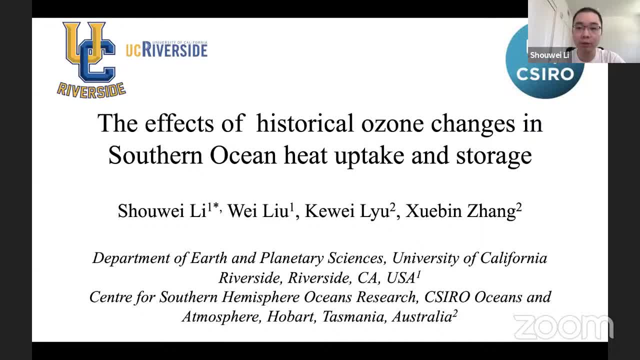 And today I'm going to talk about the effects of historical ozone changes in Southern Ocean heat uptake and storage. On this project, I collaborate with my advisor, Professor Wei Li, and I also collaborate with Kewei Li and Shijin Zhang from Australia. 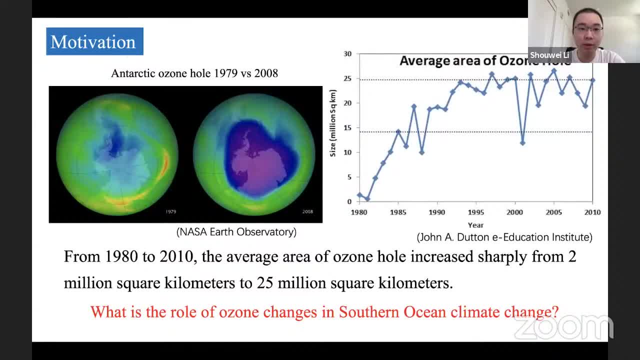 The left figure here shows the untacted ozone concentration, as well as the ozone hole in 1979 and in 2008.. While the right figure here shows the time series of the average area of ozone hole. So we can find that due to human activities. 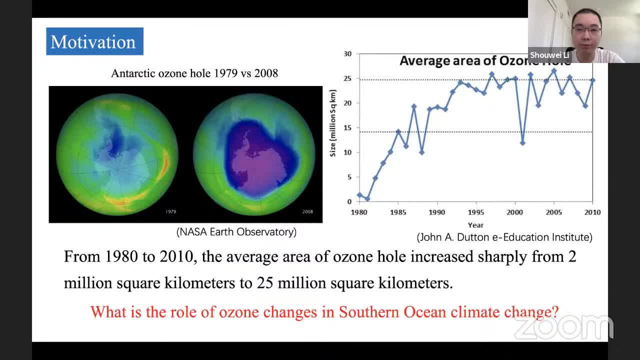 the untacted ozone hole has increased a lot in the past few decades And as a candle of greenhouse gas. so the changes in ozone concentrations is supposed to affect the climate, particularly in the Southern Hemisphere. So in this project we wanted to know what is the role of ozone changes. 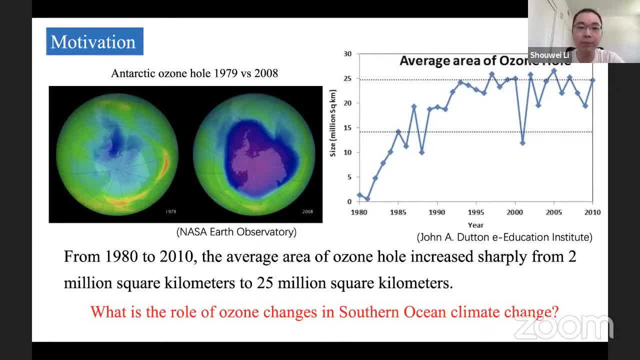 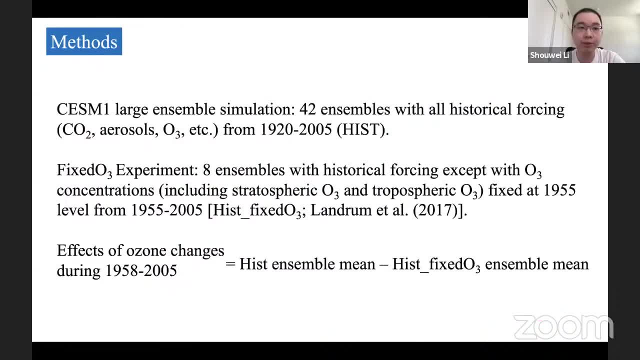 in Southern Ocean climate change. Particularly, we focused on the Southern Ocean heat uptake and storage. In this project we used one large ozone zone simulation which consists of 42 ozone members with all historical forcings and is named as historic simulation. 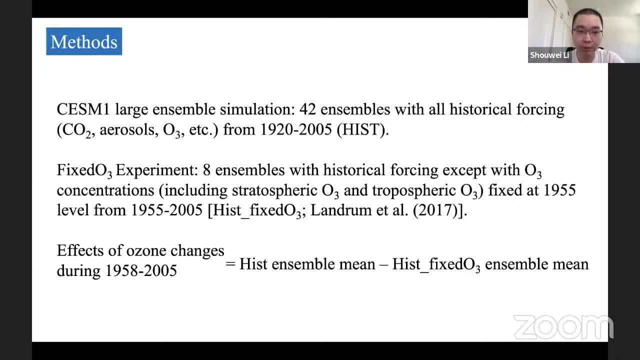 And meanwhile we have another experiment, which is fixed ozone experiment, which consists of 80 ozone members and the forcings are as in the. However, the ozone concentrations, including both stratospheric ozone and the tropospheric ozone, are fixed at 1955 levels. 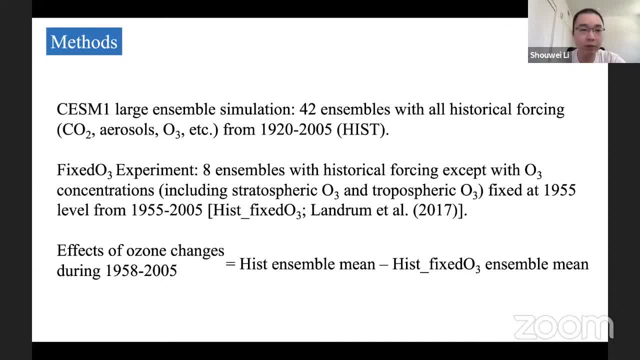 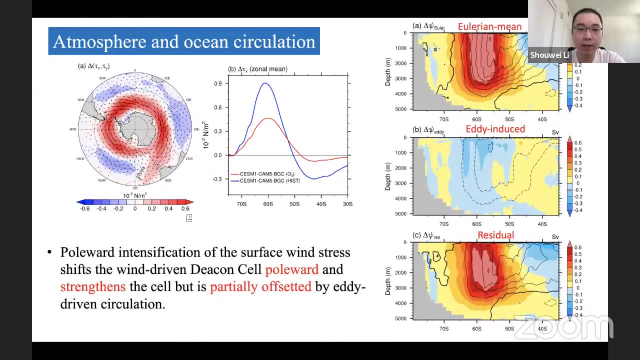 And it's named as historic fixed ozone simulations. So in this project we can analyze the effects of historic ozone changes during 1958 to 2005,, analyzing the difference between the two simulations. here And here are some of the results. We started with analyzing changes. 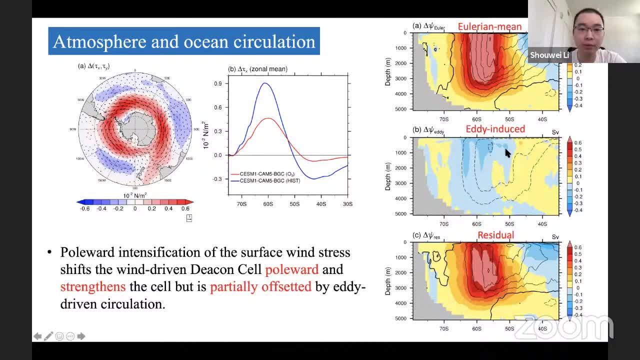 in the atmosphere. We can find that the ozone changes leads to various strong polar intensification of the surface wind stress. The red curve in panel B here. and the ozone induced changes contribute to about half of the historic surface wind stress. the blue curve here. 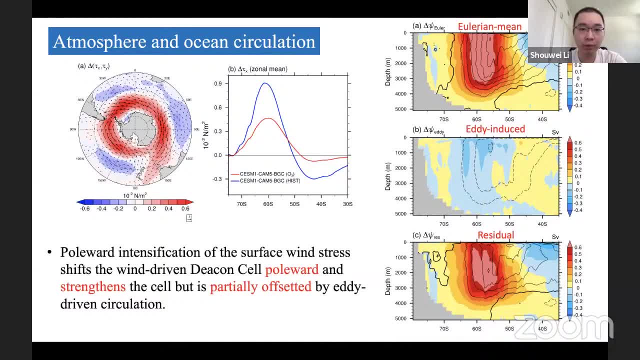 And the changes of the surface wind may alter the ocean, may alter the wind-driven ocean circulation in the Southern Ocean, which is a. So we find that the olamine or meridional ovatory circulation is also poleward shifted and also enhanced in this process. 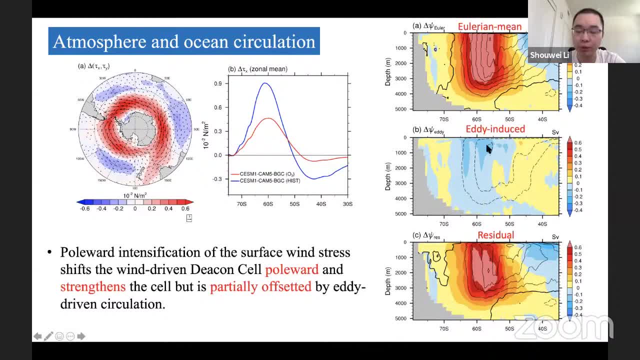 Meanwhile we find that the eddy-induced MOC is also enhanced in this process, which partially offset the olamine-induced MOC. that's producing a residual MOC generally follows changes in the olamine MOC with a poleward intensification in response to ozone changes. 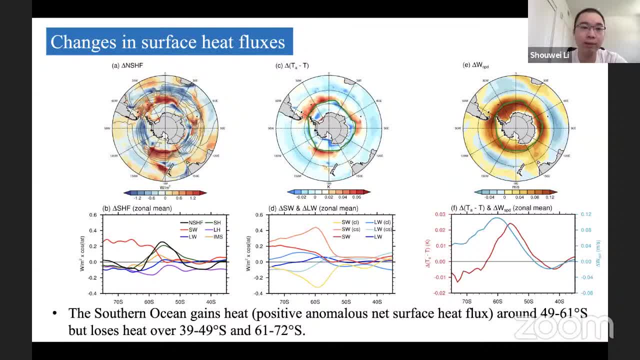 Besides the changes in ocean circulations we find that the ozone changes can also alter the surface heat flux, And the panel A here shows the special pattern of changes in the net surface heat flux. So we find that generally in response to ozone changes 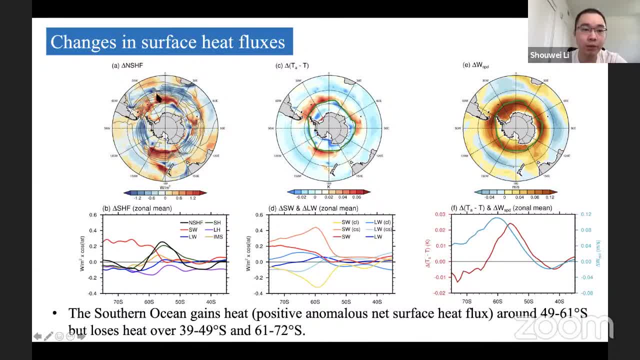 the ocean can absorb heat from the atmosphere generally with a general range of about 50 to 60 degrees Celsius in the ocean, in the Pacific, also in the Atlantic, And the zonally average changes in net surface heat flux is shown as the black curve in panel B here. 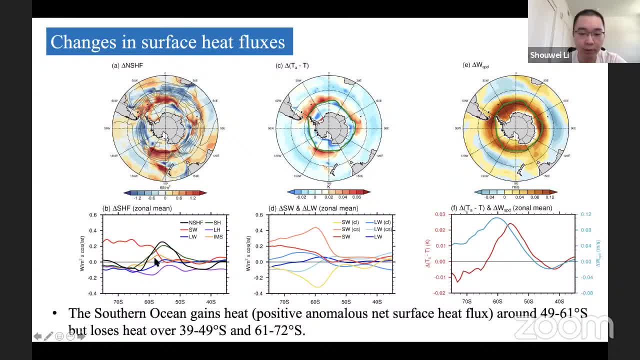 So we find that the southern ocean gains heat from the atmosphere around 49 to 61 degrees Celsius, but lose heat over 39 to 49 and also over 61 to 72 degrees Celsius, And many heat fluxes can contribute to net change. 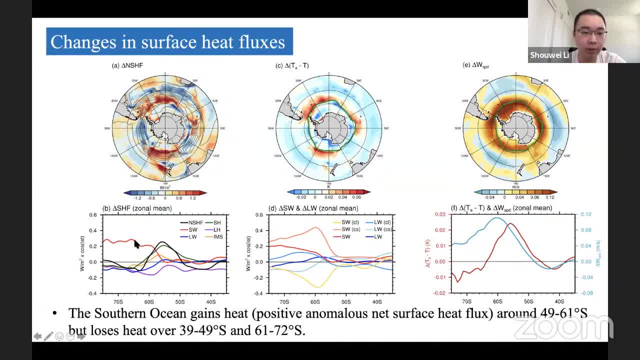 So here we find that the ozone changes induce very strong shortwave warming to the source of about 55 degrees Celsius, And the shortwave warming is the incompression between a reduced shortwave reflection- the coral curve in panel D here- and the amplified shortwave reflection. 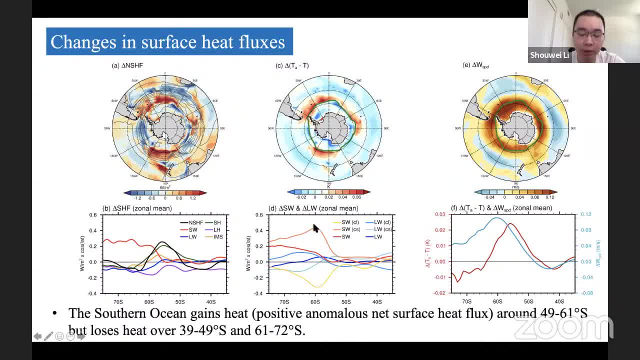 which is gold curve in panel D. here, The reduced shortwave reflection is associated with an Arctic sea ice retreating as well as the asteroid feedback, While the gold curve, which is the amplified shortwave reflection, is associated with changes in chaos. 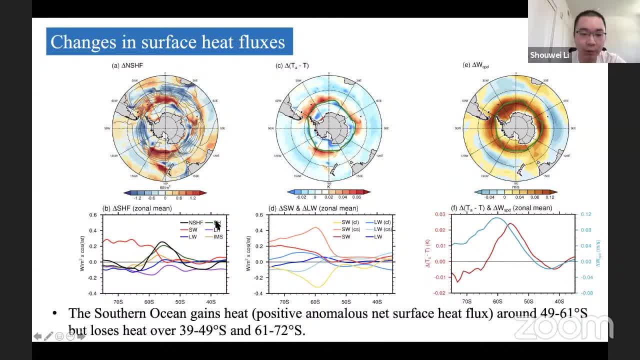 And besides the shortwave warming we find that the sense of heat, which is the green curve in panel B, here the sense of heat generally follows the patterns in net surface heat flux here And the sense of heat is altered by the air-sea temperature contrast. 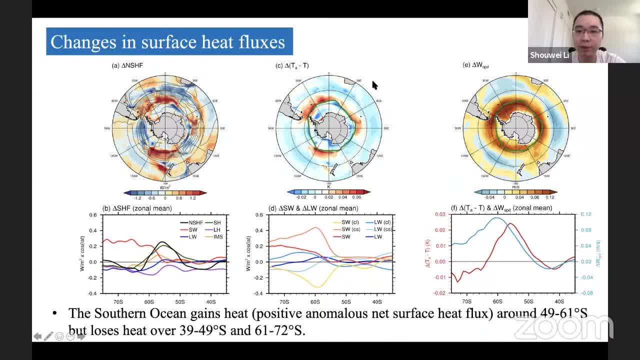 and the surface wind speed, the special pattern in panel C and E here and the zone average in panel F here. And also we find that the ozone changes lead to latent heat cooling- the purple line in panel B here And the latent heat cooling. 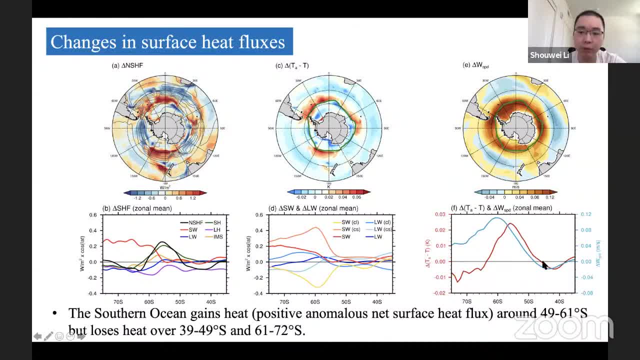 is probably due to the changes in the surface heat flux in panel B here, And also we find that the Cs can directly change the surface heat flux, which is the orange curve in panel B here It leads to positive anomalies with about 50 to 60 degrees Celsius. 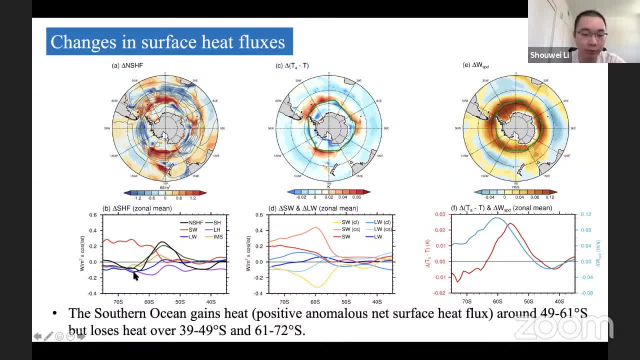 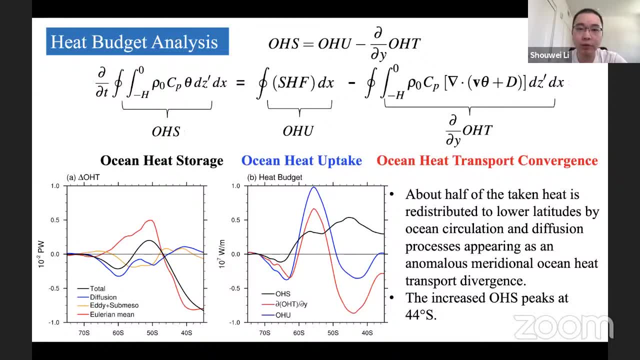 while negative change to the source of 60 degrees Celsius in the Southern Ocean With the results in the surface heat flux and ocean circulations. here we want to link the ocean heat uptake and the ocean circulation induced changes in maritime ocean heat, transport convergence. 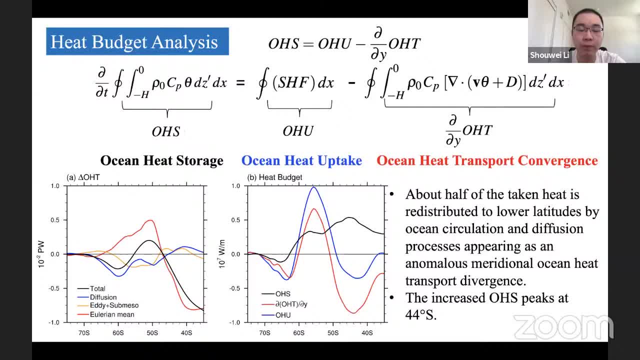 So here we analyze the heat budget, in which we define the ocean heat storage as the difference between ocean heat uptake and the maritime ocean heat transport convergence, And the results are shown in panel B here. So we find that the blue curve here, which refers to ocean heat uptake, 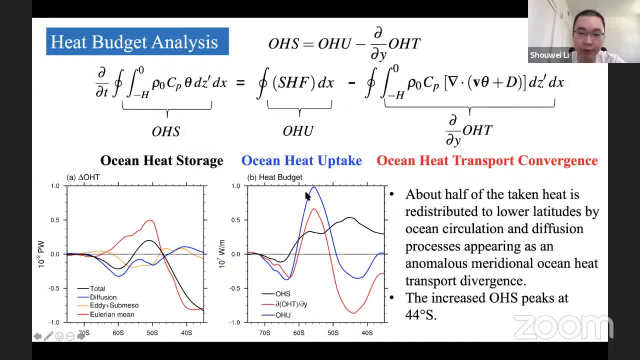 we find that the Southern Ocean gets heat from the atmosphere with a range about 49 to 61 degrees Celsius. However, due to the effects of ocean circulations and the fueling process, which may transport the heat to lower latitudes, which is the red curve here, 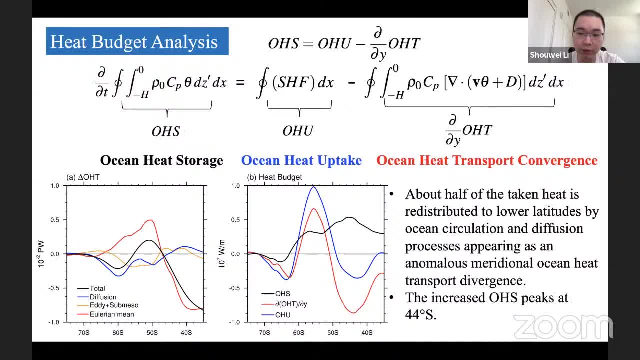 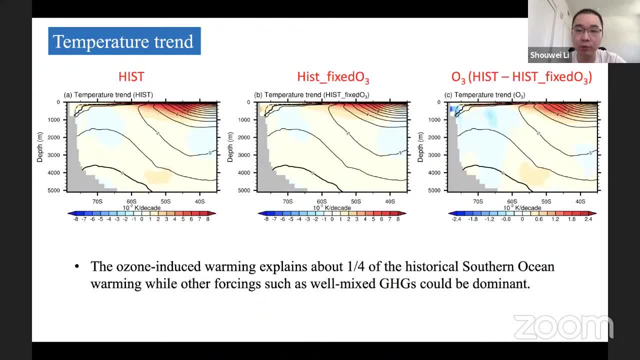 So that's the ocean heat storage at lower latitudes, about 44 degrees Celsius. here, Corresponding to the changes in the ocean heat storage, we find that the ozone-induced Southern Ocean warming, which is the panel C here, the ozone-induced Southern Ocean warming. 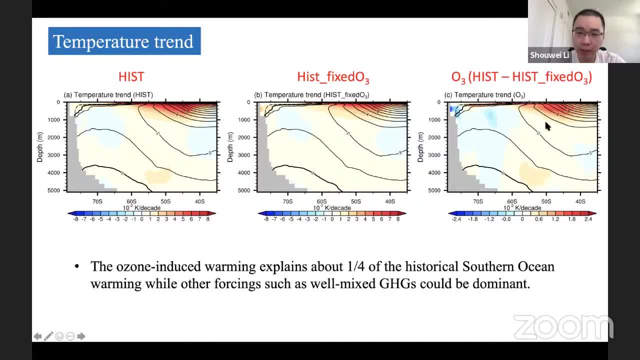 peaks around 45 degrees Celsius, And comparing the ozone-induced warming with the historical warming, the panel E here notice that the color bars here are different. So we find that the ozone-induced warming experience about one-fourth of the historic Southern Ocean warming. 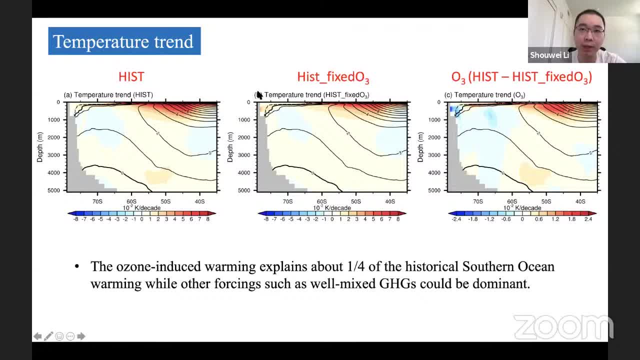 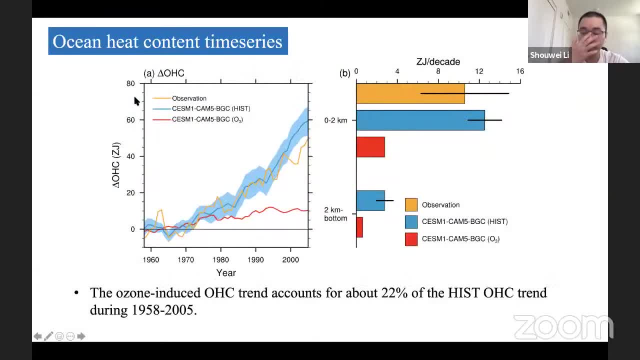 while other forces- the panel B here- other forces such as a well-mixed greenhouse gas, may still be dominant for the historic simulation here. Yeah, With the changes in temperature we further analyze the ocean heat content time series. We wanted to know to what extent. 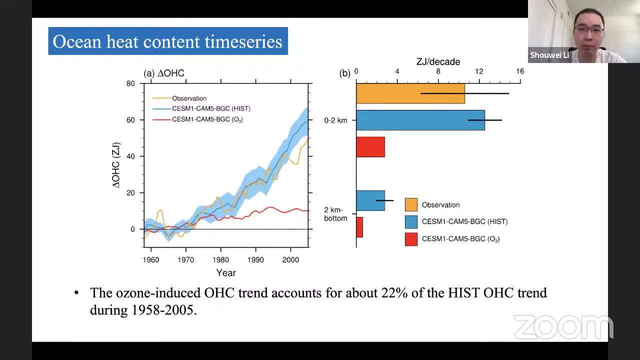 can the ozone changes contribute to the ocean heat content anomaly in the Southern Ocean. And the panel E here shows the baseline integrated flow depth ocean heat content anomaly since 1958.. And the red curve here refers to the ozone-induced anomaly, while the blue curve here refers 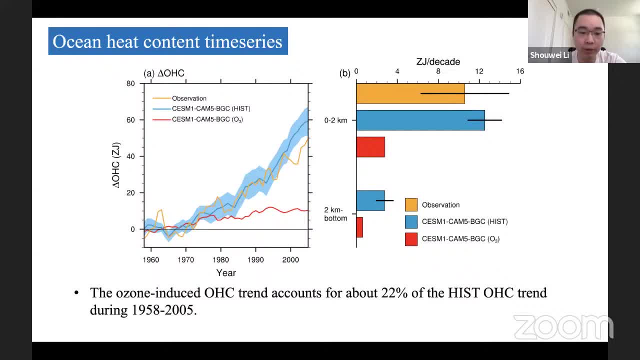 to the historical anomaly And we find that the ozone-induced anomaly ocean heat content trend accounts for about 22% of the historic ocean heat content anomaly in the Southern Ocean And we further separated the flow depths into the upper ocean and the deeper ocean. 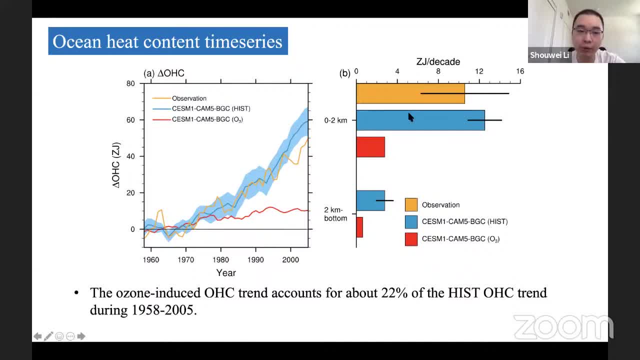 which is the panel B. here We found that the ozone-induced ocean heat content anomaly is most stored in the upper 2,000 meters there. Yeah, To better understand the ozone-induced temperature change, here we further decomposed the changes into sparseness. 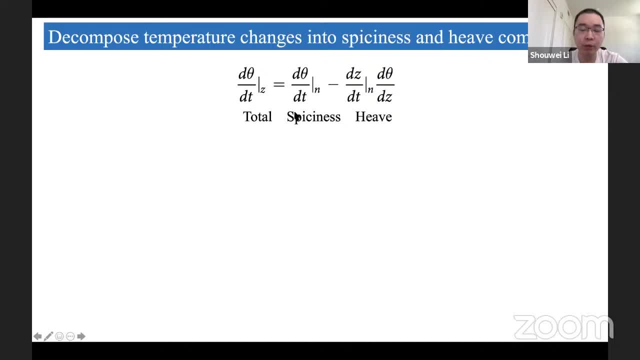 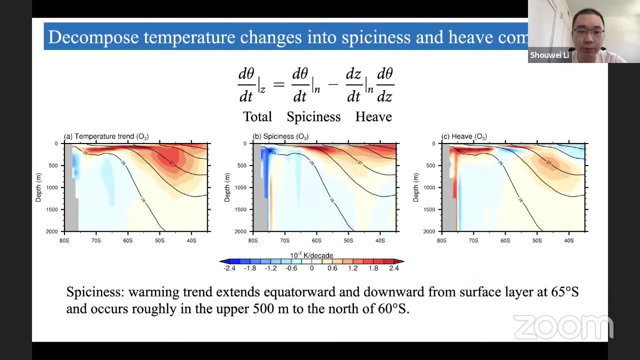 and heat component. The sparseness component refers to the changes on density coordinate, which is associated with changes in water mass properties, while the heat component is associated with vertical movement of the aspic knots. And here are the decomposition, and the panel B here shows: 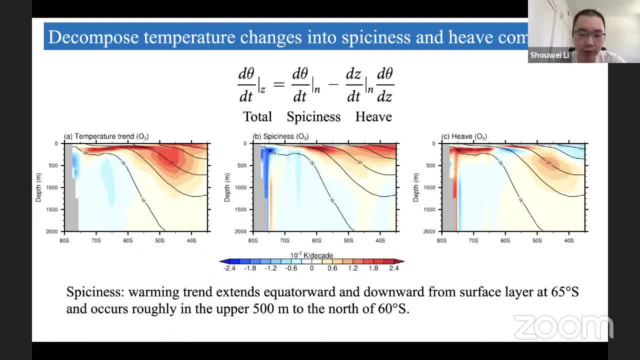 the sparseness component. So we find that, due to ozone changes, the warming trend extends down equatorward and downward from surface layer at 65 degrees Celsius And the warming roughly occurs in the upper 500 meters to the north of 60 degrees Celsius. 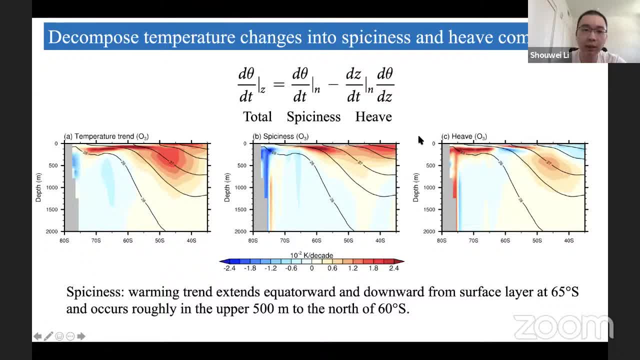 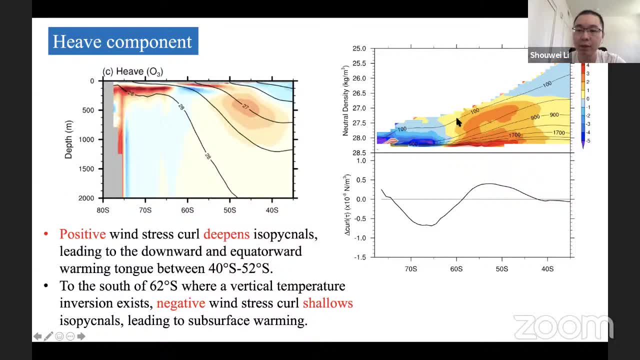 And then the panel C. here is the heat component. The heat component here is associated with the vertical movement of the aspic knots, which is the red figure here. So we find that the vertical movement of the aspic knots is most dominated by the surface wind stress curve anomaly. 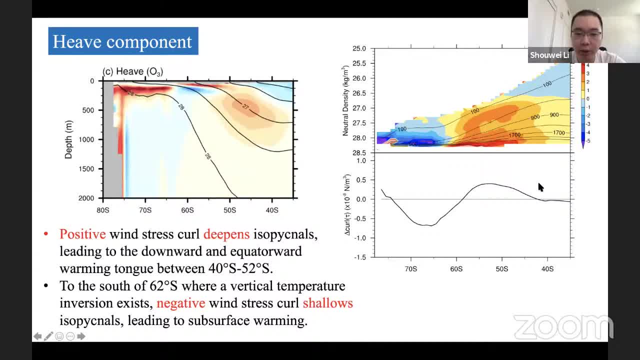 So in particular the positive wind stress curve anomaly between 40 to about 52 degrees Celsius. it depends to the aspic knots. Therefore it contributed to the equatorward and the warming trend there And, however, to the source of 62 degrees Celsius. 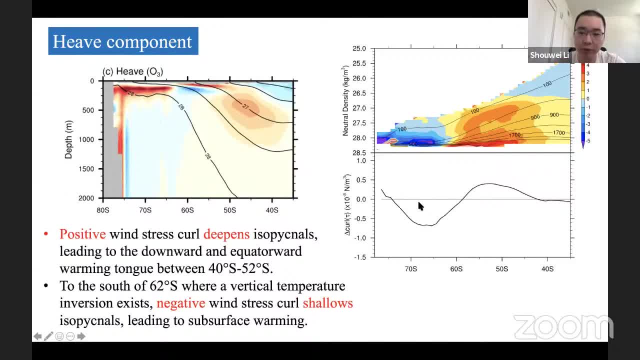 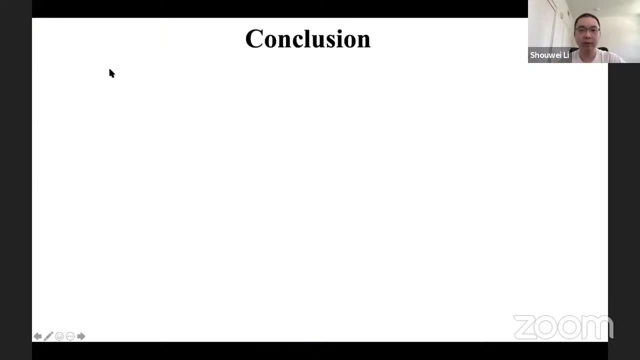 the negative aspic knots, the negative wind stress curve anomaly. it shallows the aspic knots. However, due to the vertical temperature invariant in this region, the shallowing aspic knots will lead to subsurface warming in this region. And here are some of the conclusions. 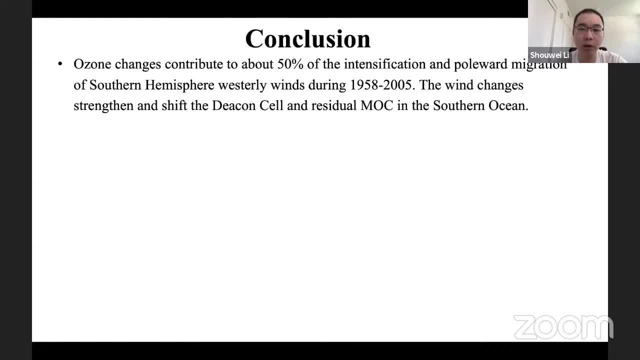 First of all, we find that the ocean changes contribute to about half of the historical intensification of polar world migration of the southern hemisphere- wisteria winds during 1958 to 2005.. And the wind can also change the ocean circulations, leading to the polar world intensification. 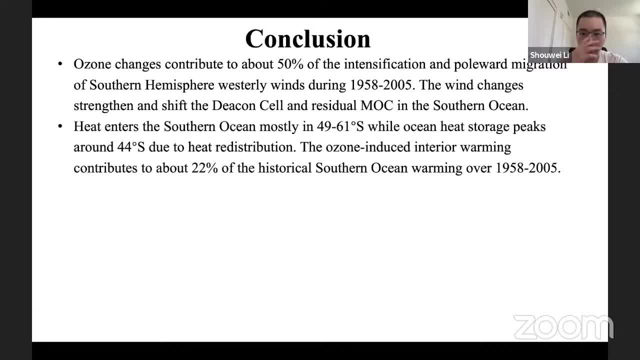 of the Deacon Steel as well as the residual milk in the southern ocean, And we also find that the ocean heat barge analysis suggests that the heat enters the ocean in the southern ocean most within 49 to 61 degrees Celsius. 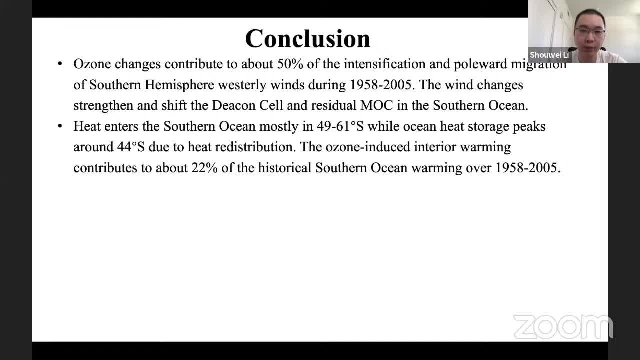 However, due to the effects of ocean circulations and the diffusion process, the ocean heat storage appears at a lower latitude, around 44 degrees Celsius, And we also find that the ozone induced warming contributes to about 22% of the historic southern ocean warming. 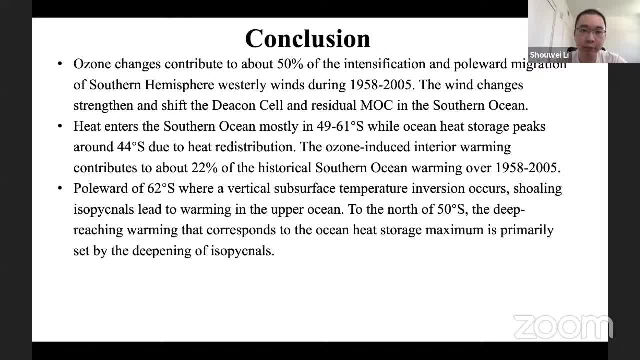 during this period And the specimen and the heat decomposition suggests that polar world of 62 degrees Celsius, where our vertical temperature invariant occurs, the shallowing aspignals can lead to subsurface warming And, however, to the loss of 50 degrees Celsius. 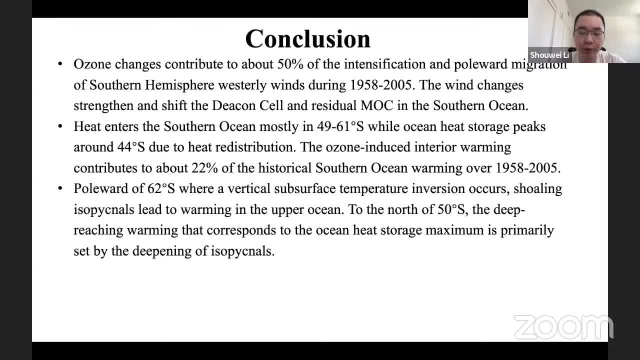 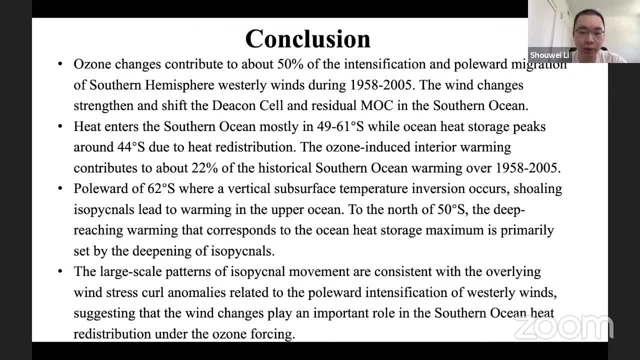 the depletion warming that corresponds to the ocean heat storage. mixing is primarily due to the deepening aspignals And we also find that large scale patterns of aspignal movement are consistent with the surface overlaying of the surface curve anomaly, which are identifying 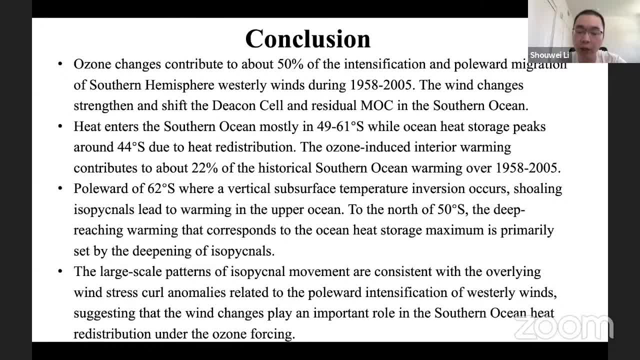 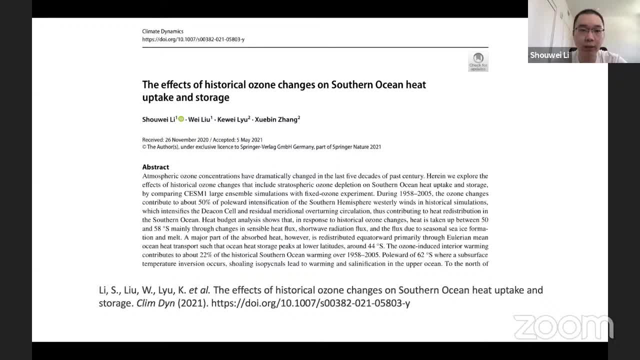 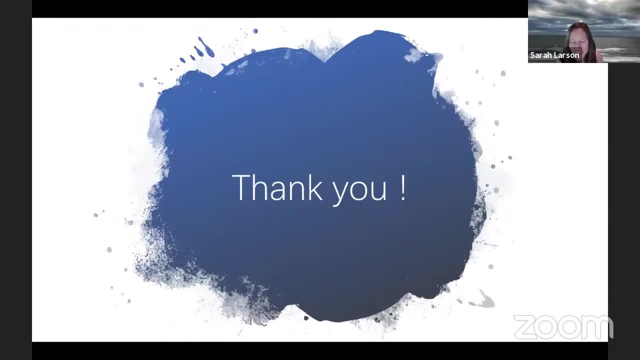 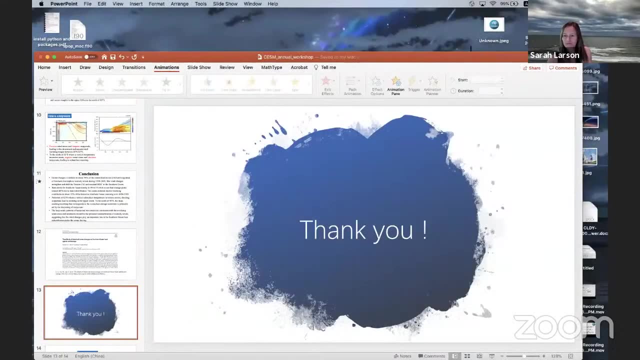 the important role of wind changes in the southern ocean, heat redistribution in response to ozone forcing, And all the results at present here have been published on Climate Dynamics. Yeah, thank you, Great thanks. Do we have any questions? Yeah, we got one from Gokhan. 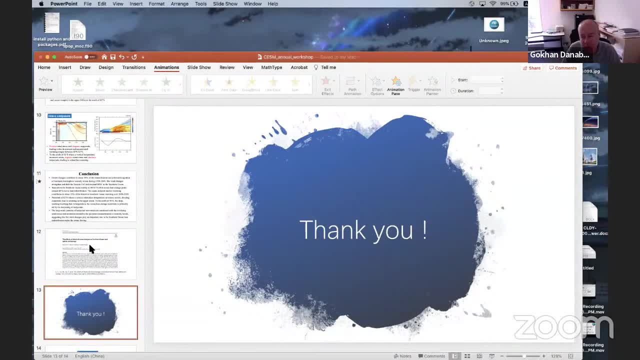 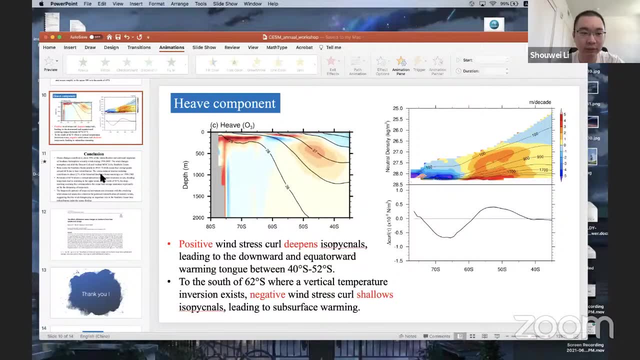 Yeah, just at the last point, you indicated that the wind stress curl is playing a bigger role than wind stress itself. Why is that? Oh, you mean this one. Well, in your last conclusion, yeah, the fourth one- it says the wind stress. 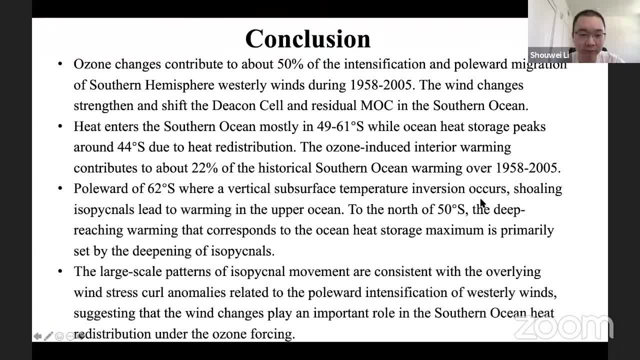 curl anomaly is right, Yeah, So it's not the zone of wind stress itself, but it's the curl. That's what you're saying, right? Yeah, the wind is the zone of wind stress can alter the ocean circulations. 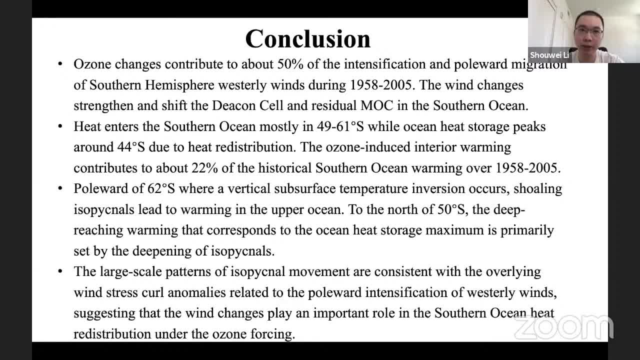 while the wind stress curve anomaly may lead to the such as Eggman pumping, so it will lead to aspignal movement there. Okay, They're both important, I should say. All right, I think we'll move on to our last talk. 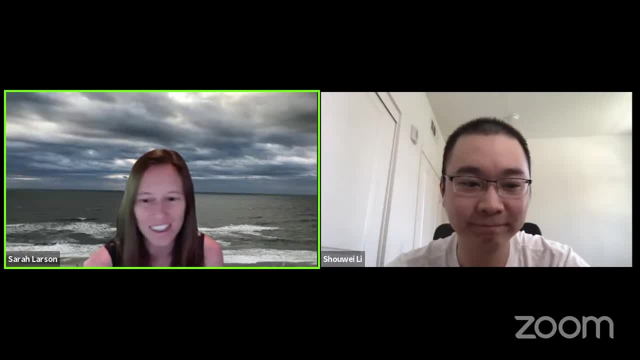 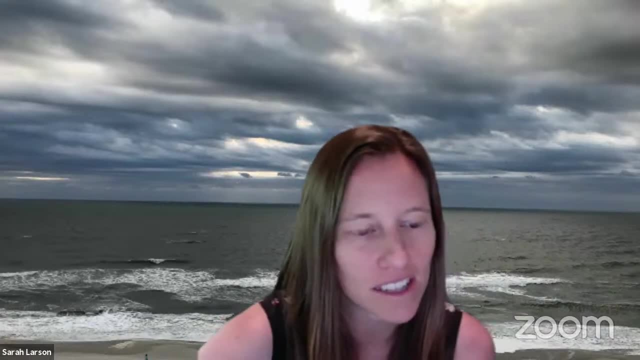 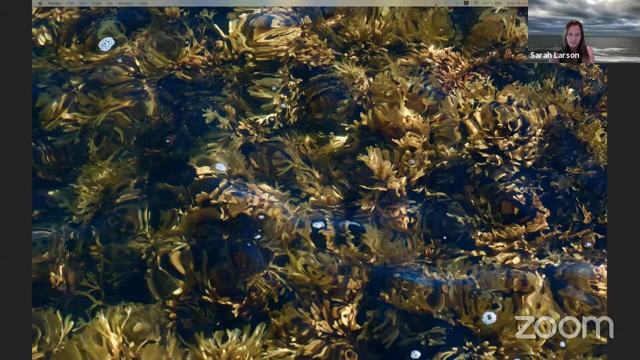 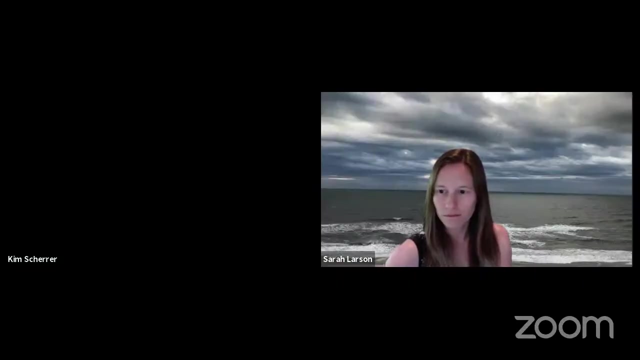 of this session. We're very close to staying on time here, So our last talk will be from Kim Shearer. The question is the title: is Marine Wild Capture Fisheries After Nuclear War? I guess I first have to unmute myself, Okay. 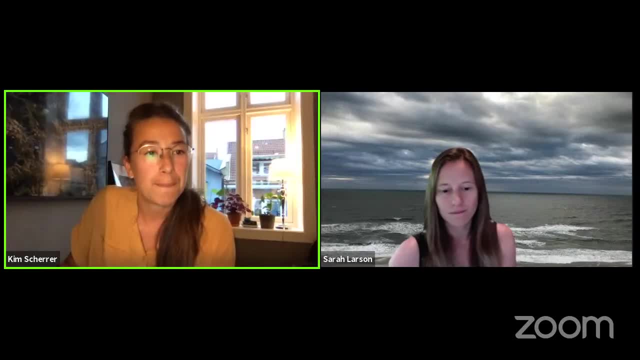 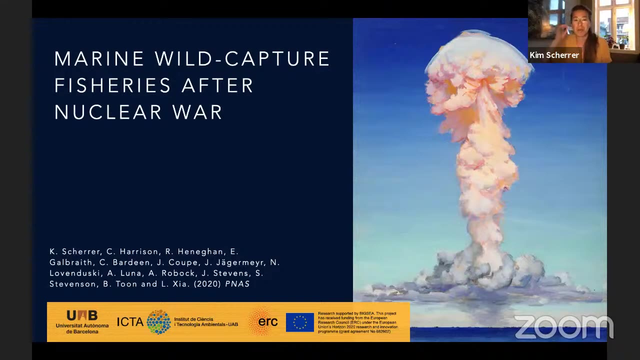 Now I'm going to start sharing the screen. All right, Can you see that everyone? We can't. It's coming out. Yep, there, it is Perfect. Okay, great Thanks. I'm a postdoctoral researcher at the Autonomous University. 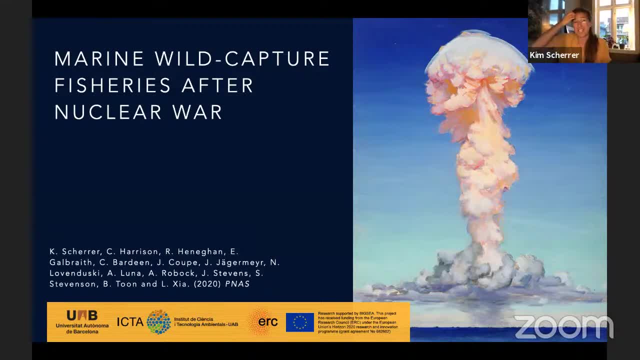 of Barcelona And here today, I wanted to present some things slightly different. I'm going to shift the topic to catastrophic and sudden climatic change and to fisheries, And I've squeezed a lot of things in here, But the point is to give you an example. 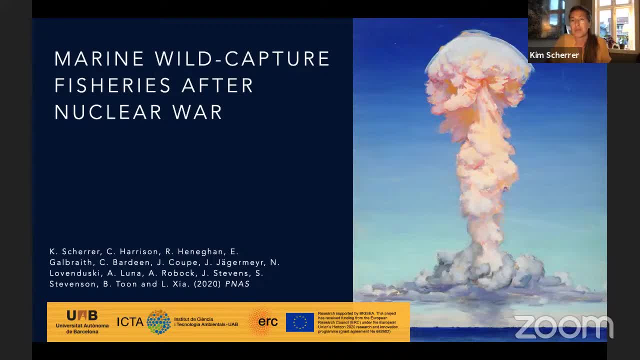 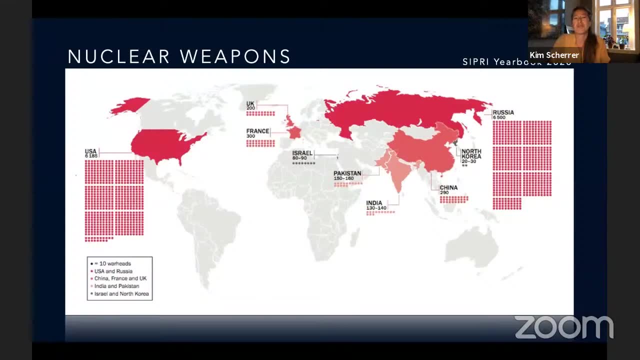 of what kind of questions that CESM outputs can be used to investigate. Right, But first, why is it important to think about the consequences of nuclear war? This figure from SIPRI shows the number of nuclear warheads by country in 2019.. 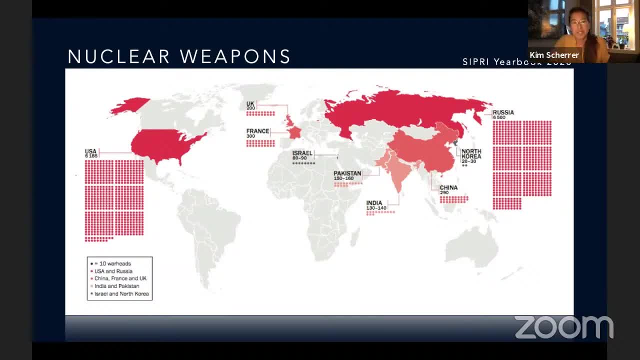 And even though there's been a large decrease in the number of weapons since the Cold War, there's definitely enough warheads currently to cause huge destruction. So there's also an increasing number of countries that have these weapons, for example, notably India and Pakistan. 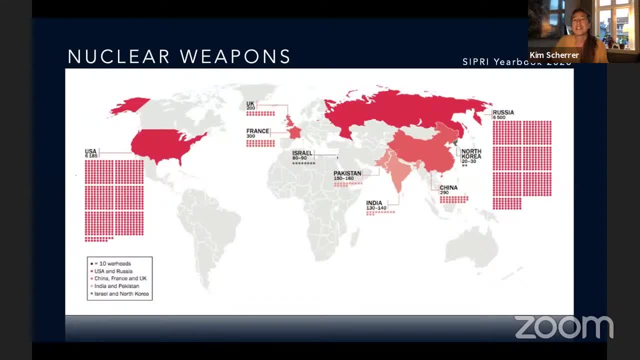 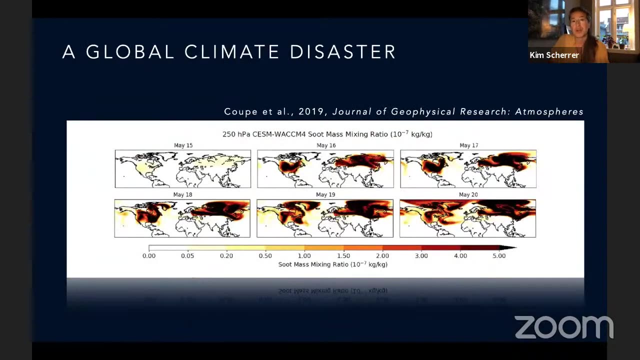 have rapidly growing weapons arsenals, And these two neighboring countries have been in armed conflict several times in the past decades. So the existence of these weapons means that a large scale conflict is possible And, beyond the direct destruction, a nuclear war could also create a global. 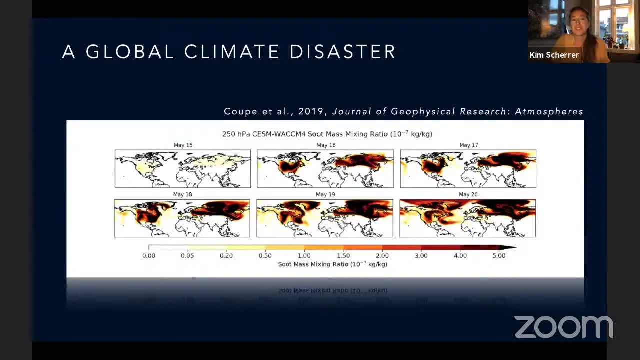 climate disaster. Detonations of weapons in urban areas could cause huge fires and firestorms, And so the soot from these fires could rise into the upper atmosphere, So similar as during large volcanic eruptions. these emissions could block out sunlight and cool the earth. 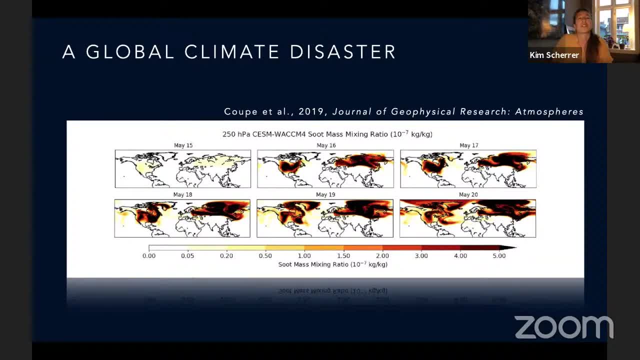 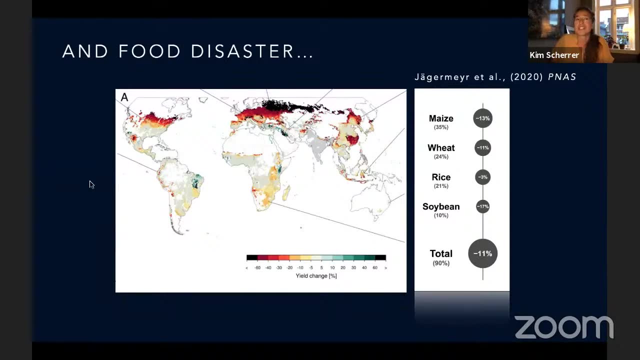 for several years, And this is where CSM or other earth system models comes in. The figure here shows the simulated spread of soot from the US-Russia nuclear exchange, simulated by Coupadel, And this in turn could create a global food disaster. 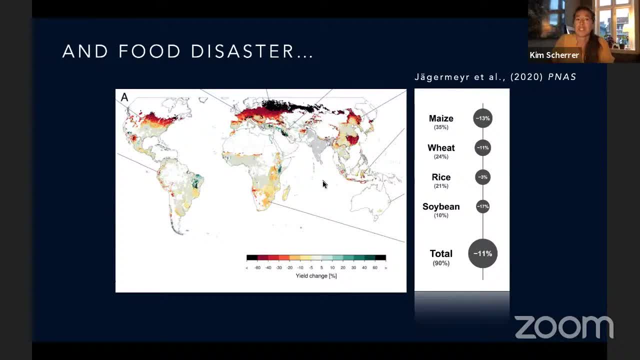 So a study by Jonas Jägermeier and colleagues published last year used simulations from CSM of a regional conflict between India and Pakistan to force global crop models, And they estimated that a regional war could cause 11% global decline in calories. 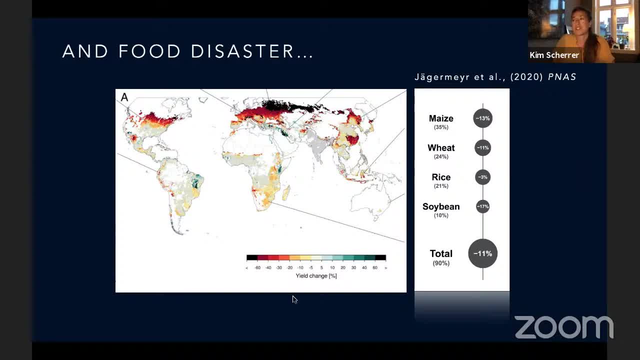 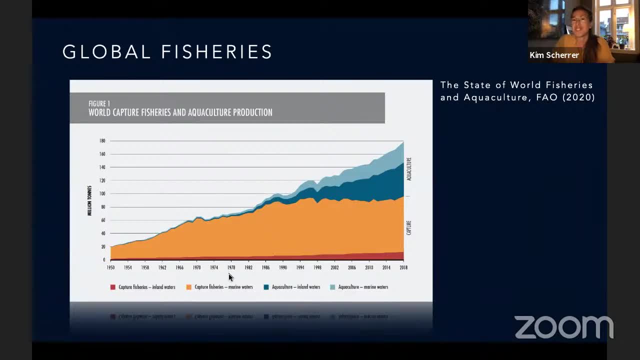 from four of the major crops globally sustained during five years. But I am a fisheries person so I will give you a quick overview of global fisheries production or global fish production. And the figure from FAO shows the total fish and seafood production from 1950. 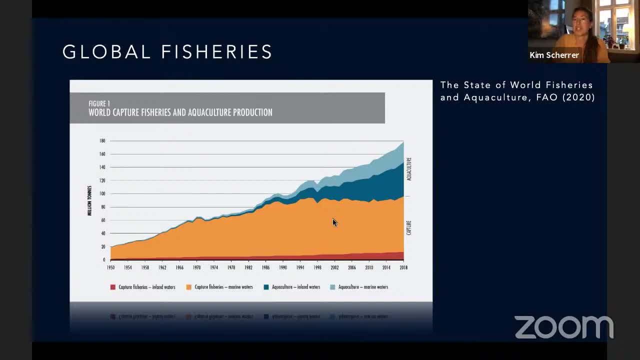 until present And, as you can see, the major part has historically been from marine capture fisheries. this orange chunk here, Although today marine and inland aquaculture combined is equally large in terms of food production globally, And even though this is very small in terms. 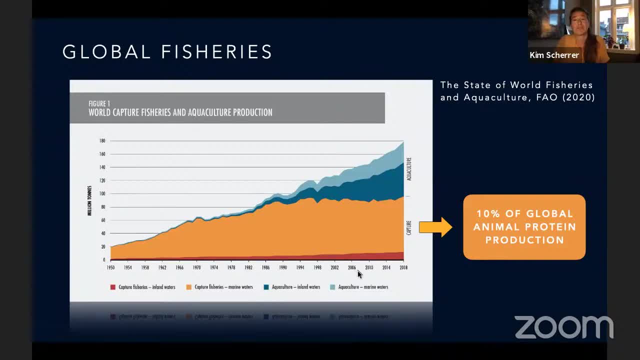 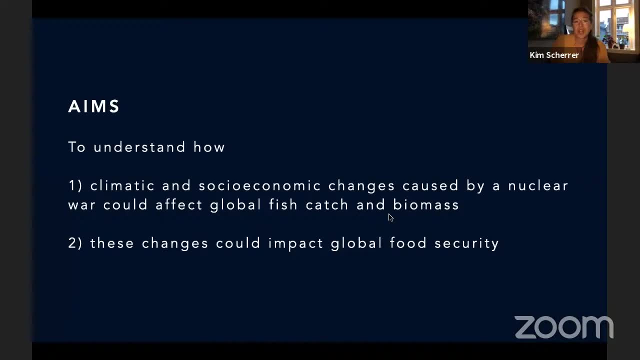 of calories and also relative to other animal production. fisheries could be a pretty important food source if land based production systems begin to fail. So the aims of our study are to understand how we model global fisheries, and Cheryl talked about this this morning, But there are 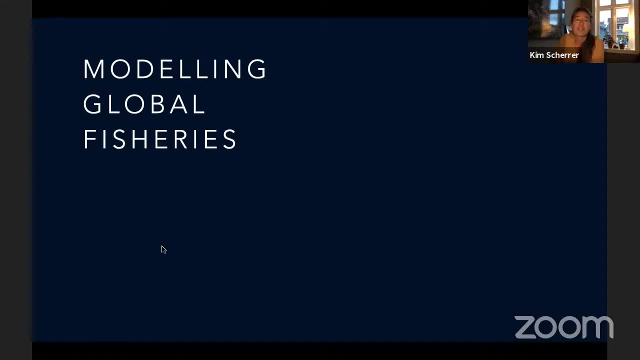 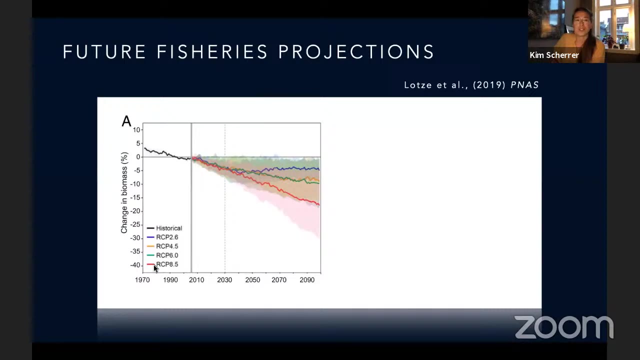 for those of you who didn't hear, there are several global fisheries models that use, gridded, either two or three dimensional environmental variables, like the figures Cheryl also showed, But similar. just like there's a sea map for climate models, there's a fish. 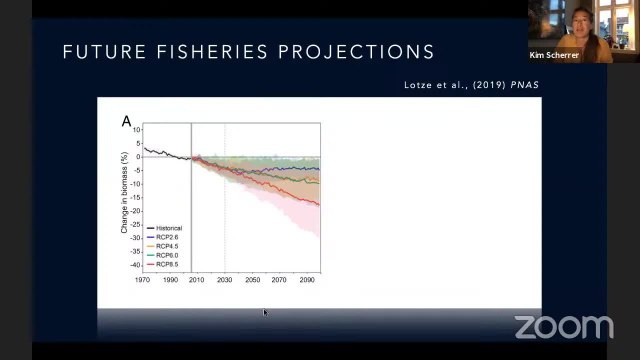 map for marine ecosystem and fisheries models And this study by Lotse and colleagues made ensemble model projections for fisheries and the climate change with six global marine ecosystem models. To the right we have RCP 8.5, where each model projection is outlined. 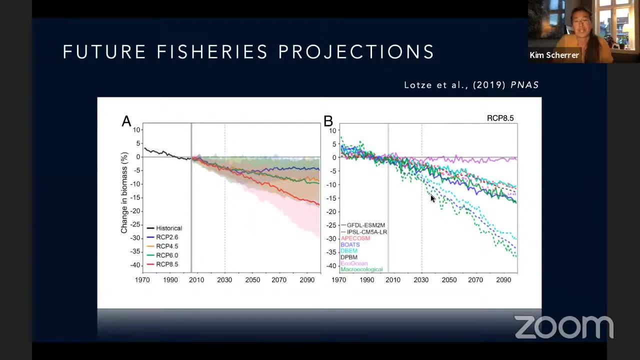 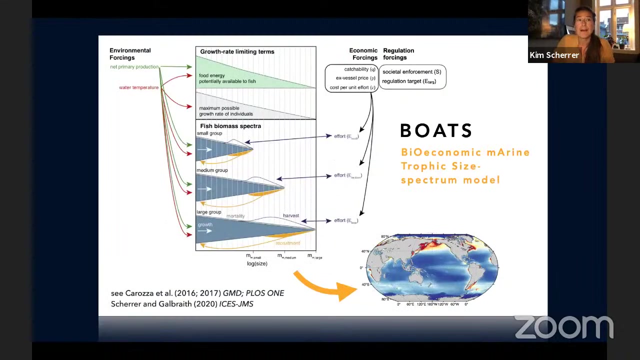 and also dashed and solid lines show the different results from wind forcing with GFDL or IPSL. So with our system outputs we can try to calculate the different effects of climate change and climate change in the environment. So we have six models included. 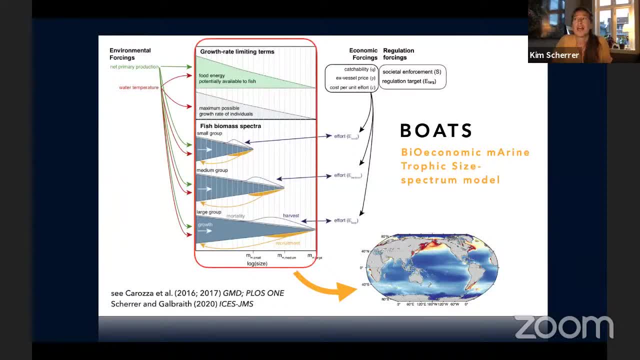 in this fish study. This is a quick overview of boats. In the model we simulate the water temperature and the MPP constraints on how much fish can grow, both in terms of providing food energy- represented up here- but also by constraining the maximal possible. 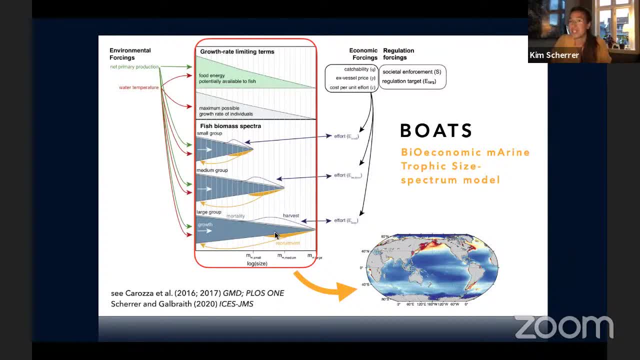 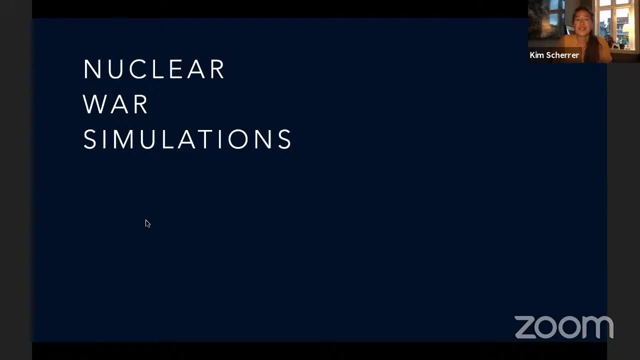 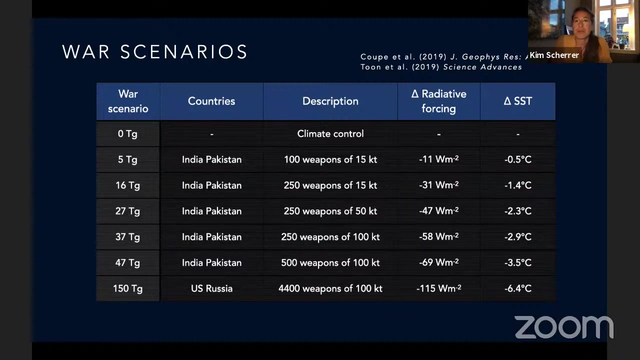 growth rate of fish in the ocean. So this is an example of how much energy we spend on catching fish. This model is determined by how much fish there is available and by the amount of fish that are in the ocean. So this is a model. 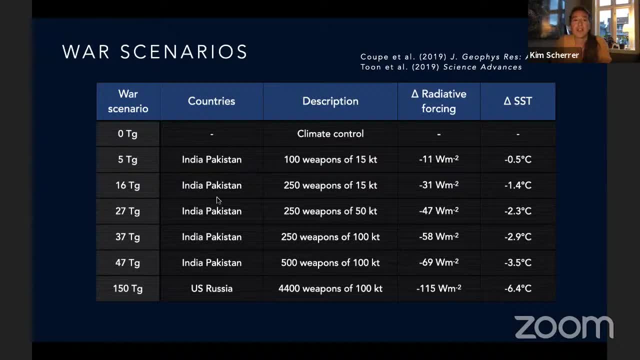 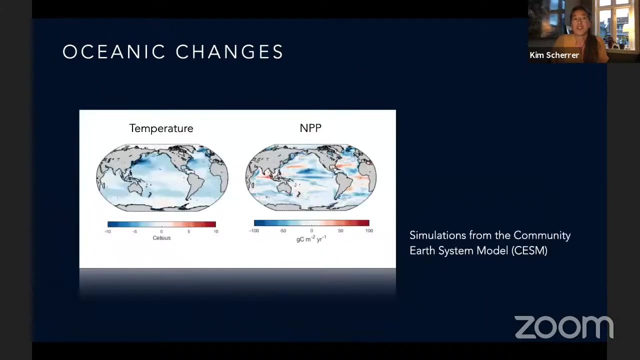 of how much energy we use. in this study We use six different nuclear war scenarios to simulate the maximum annual global means post-war, And this five teragram scenario, the smallest one, is the one that was expected to cause the 11% decline. 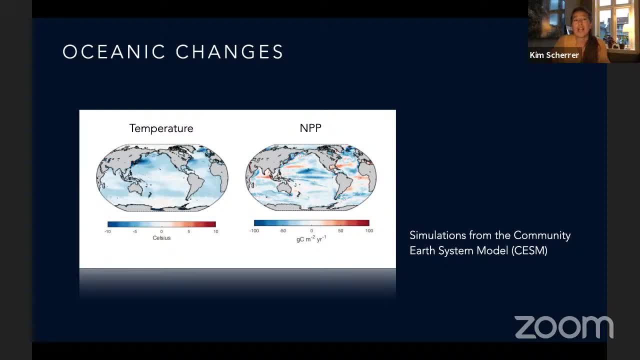 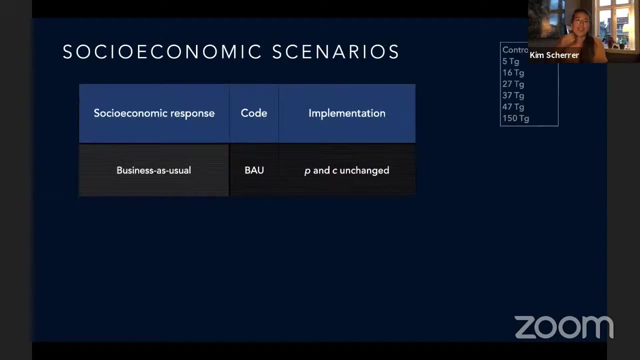 in global crop and global climate And we simply took the changes in sea surface temperature and MPP and used it as inputs to boats to estimate the impacts on fish and fisheries. But a key question is whether people would fish the same after a long period. 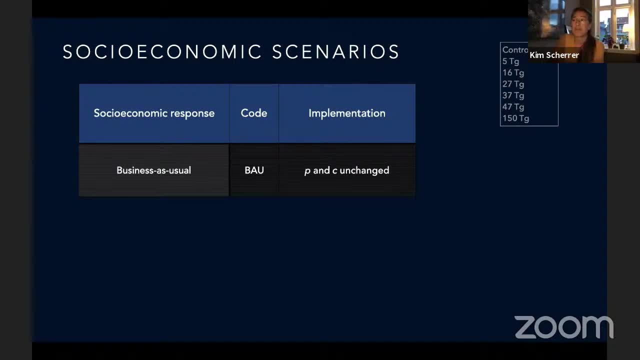 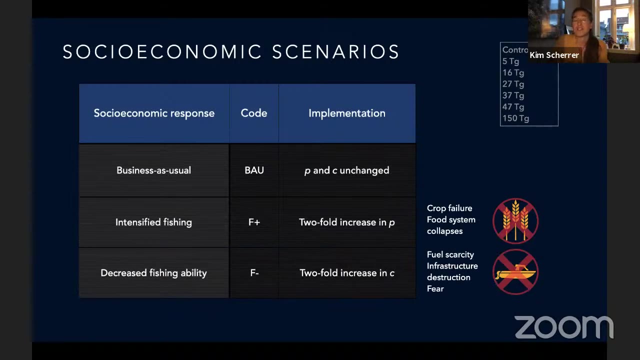 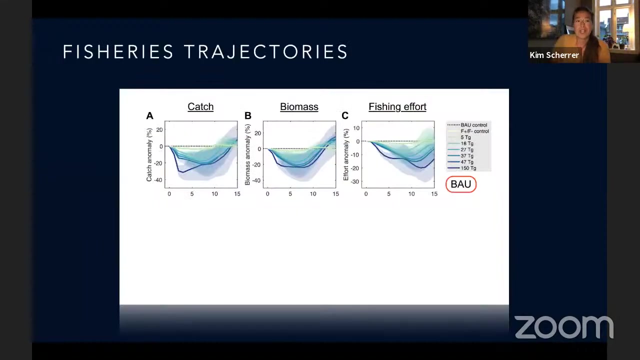 of time. So we have two scenarios. The first is the control scenario, where fishing goes about the same way as before, business as usual. Second is possible that lack of control in the world can affect the future of the world. And the third scenario: 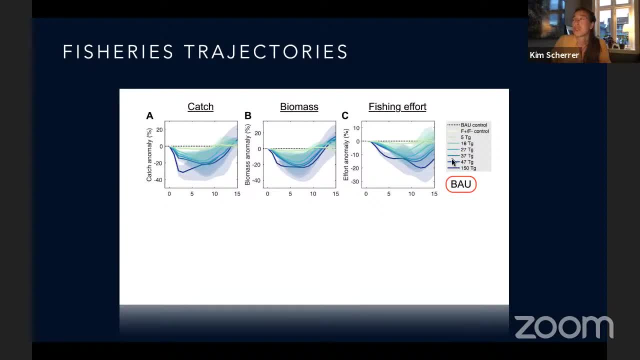 is the change in total global fish catch, total global biomass and also in the second scenario. The third scenario is the decrease in biomass in the catch. The third scenario is the decrease in biomass in the catch. The third scenario is the decrease in biomass. 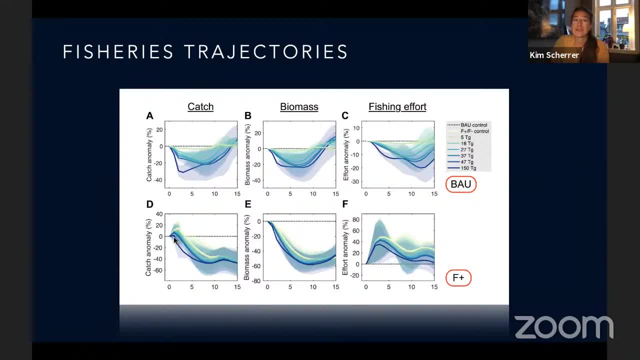 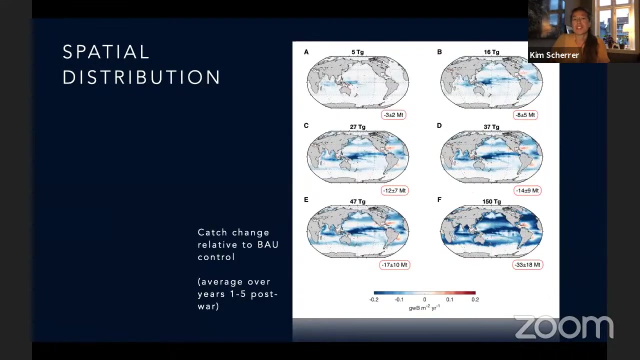 in the remaining fish. The fourth scenario is the increase in biomass in the remaining fish. The fourth scenario is the decrease in biomass in the catch. The fifth scenario is the decrease in biomass in the catch. The fifth scenario is the decrease in biomass in. 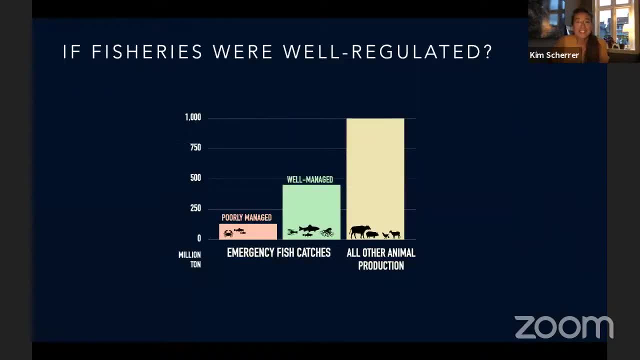 the catch. The sixth scenario is the decrease in biomass in the poor, overfish state, where the biomass has been depleted, while other fisheries are well managed with healthy, abundant fish stocks. In the paper we investigated the difference in the amount of food produced in the first 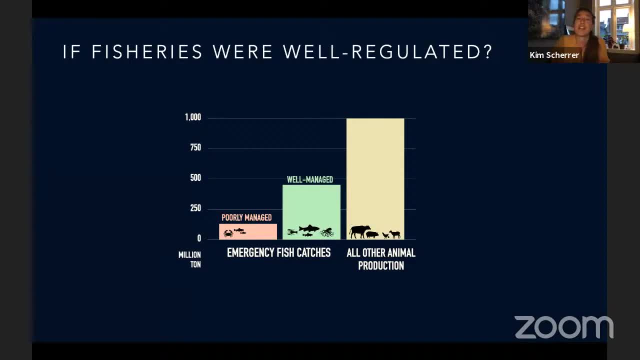 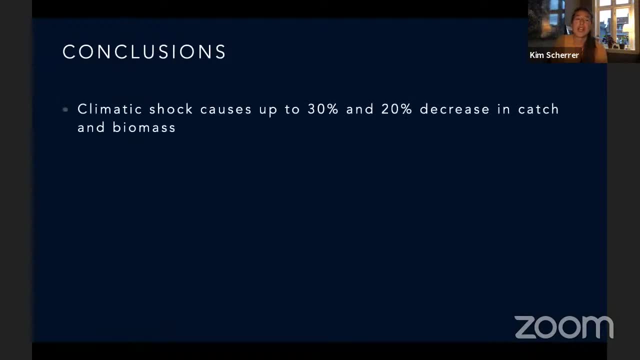 year after the war to replace almost 40% of all other animal production. In conclusion, the climatic shock causes up to 30% and 20% decrease in the MPP, which translates into a decrease in the catch, But the outcome depends. 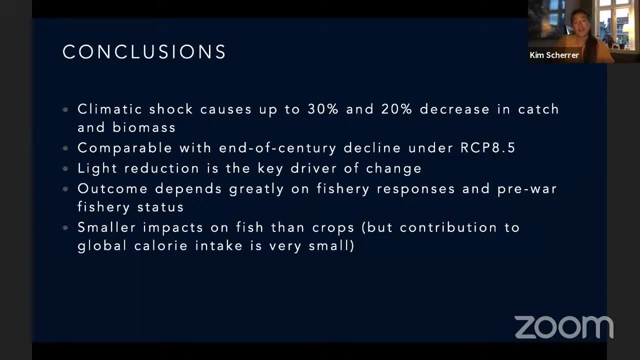 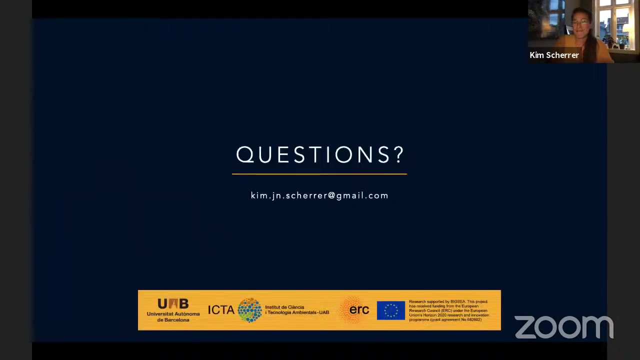 a lot on the fishery responses. We find smaller impacts on fish than on crops and we find that well-regulated fisheries could briefly replace about 40% of all other protein. So that's it for me. I don't know if there's. 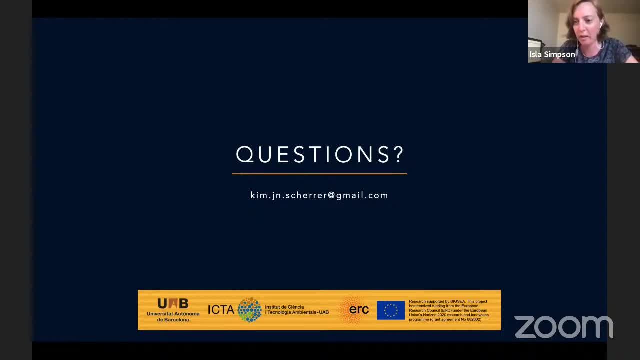 time for questions. Any questions for us? Yeah, so I'm going to most likely start a post-op with Cheryl Harrison by Christmas more or less, and then we're definitely going to look at the effects of geoengineering and I'm hopefully going to 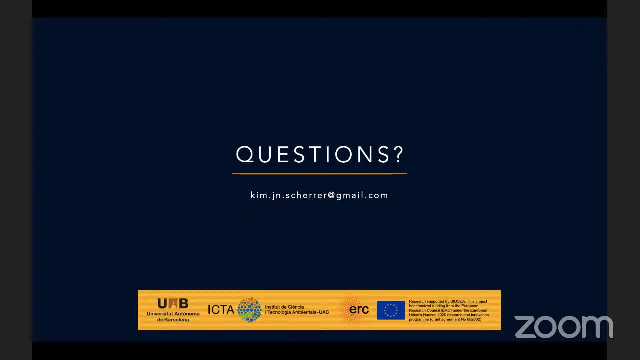 start a post-op with Cheryl Harrison and then we'll go to the next question. So the question is right now: the fish. they will not change, but by the nuclear radiation they may change the face, the gene of the face, so the face may grow differently. 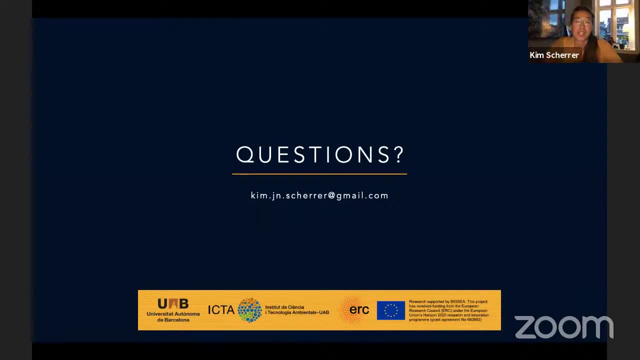 They may grow like a bigger or smaller and but that will affect the result. So we haven't made when during nuclear weapons testings, but also studies looking at the effects of, for example, the Fukushima disaster on neighboring fish. and to my understanding, I don't. I 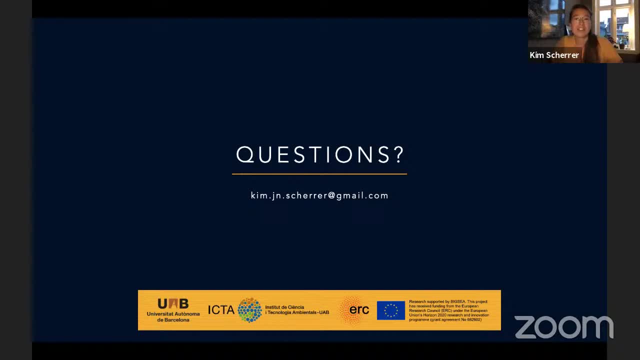 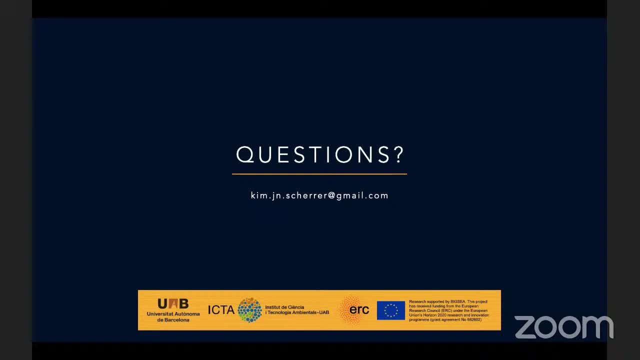 make, make sure that all, all, all of all of all the, the, the Nixon And your maps seem to confirm that in the northern hemisphere, But when you show and you say that the main driver of the fisheries impact is in fact sunlight, So why isn't that hemispheric asymmetry reflected? 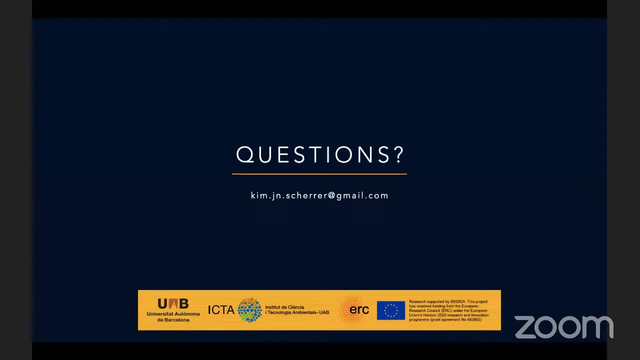 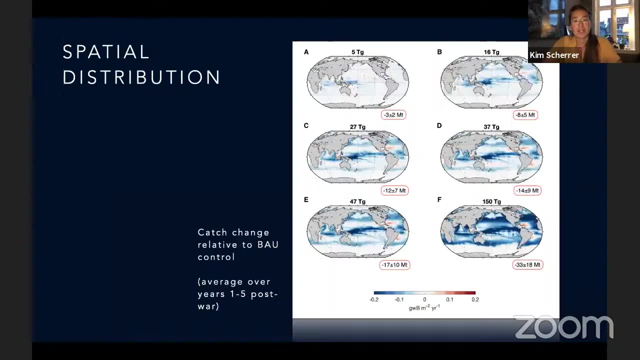 in the maps of catch changes. So I'm not an expert here, but from what I understand- and we can at least look at the maps, from what I understand- so this depends on the scenario For the US, Russia of course we're. 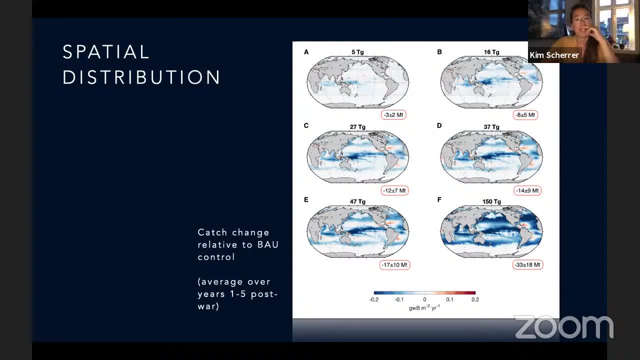 going to have most of the emissions in the northern hemisphere. For India, Pakistan, it's going to be more centralized around the equator or very localized in that area And, from what I understand, the simulation suggests that soot is going to rise high enough for the soot. 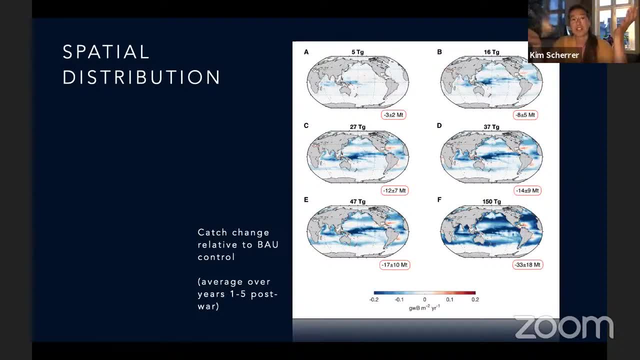 to spread into the atmosphere and cover almost the environment. Thank you, Yes, entire globe. so in the at least a couple of years after, there's going to be effects not only close to the actual uh conflict areas but around the earth. so i think that's why we don't see. 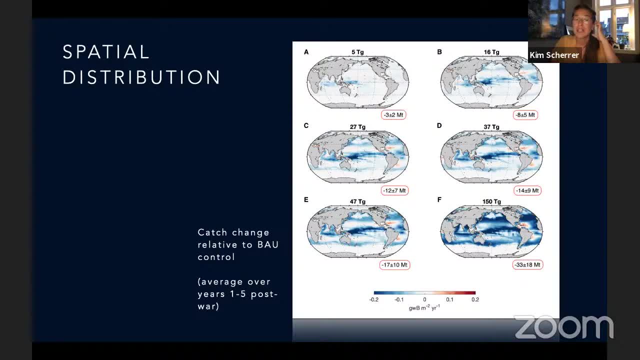 any clear regional effects from that? i don't know if cheryl can, is she there? maybe she has something to add about this. yeah, i'm here, alan is here. alan is here. yeah, uh, yeah, that's right. the. the smoke gets heated, goes up in the stratosphere and spreads around the world. 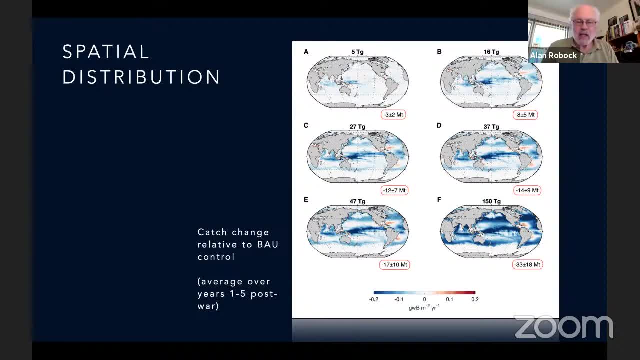 it lasts for years and we've seen forest fires recently that demonstrate that from australia. the smoke got heated and went up 20 kilometers in the stratosphere, so that's a much less smoke than we were modeling. thank you all right, so we'll take a very short break. um isla, is there anything you want to add? um? 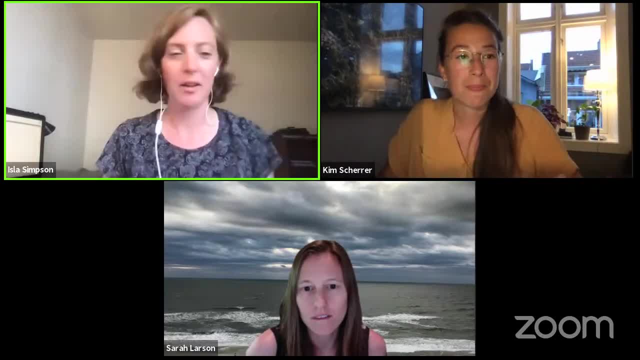 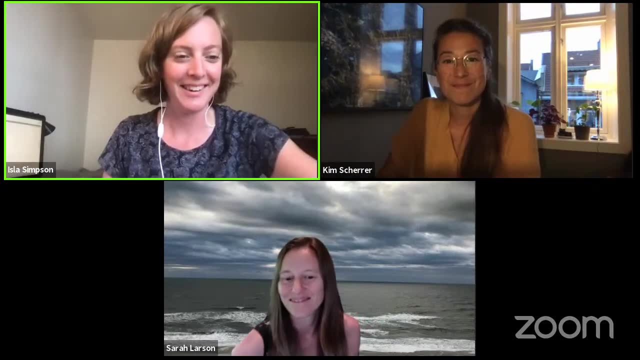 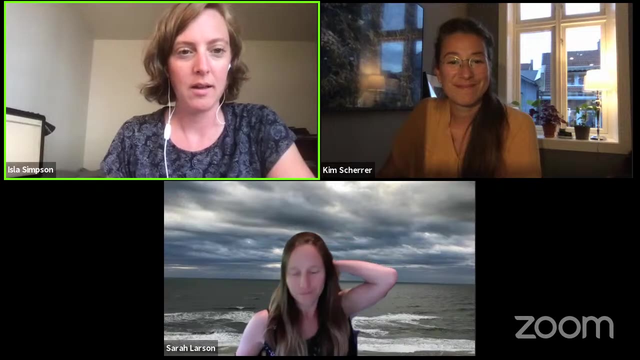 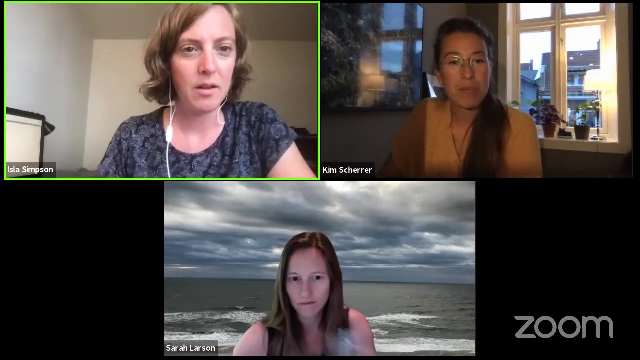 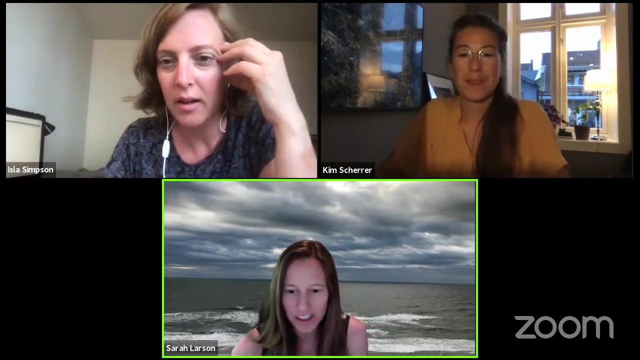 logistically. um um no, i think we'll just start again at three. uh, just to keep on time. so sorry, it's a short break. so, sarah, do you know how to? if you're a host where you see the polls? yeah, usually it's just at the bottom. 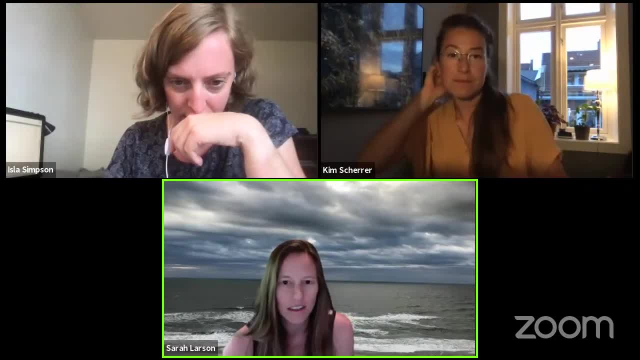 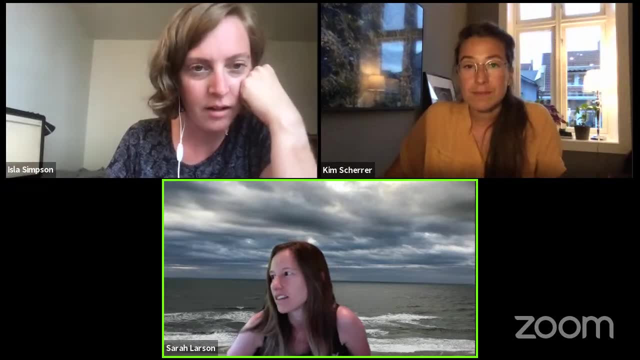 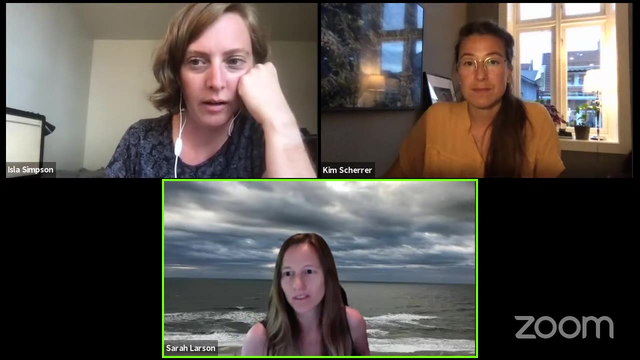 there's, like the participants, chat etc. and one of them is usually a poll. so it, but i think it has to be when the meeting is set up. it has to be set up as an option to add polls. it's possible that it wasn't set up that way. 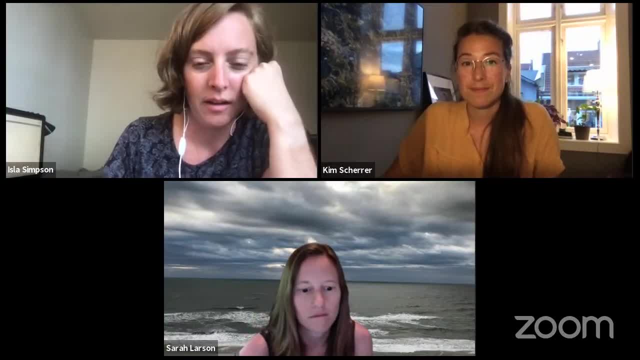 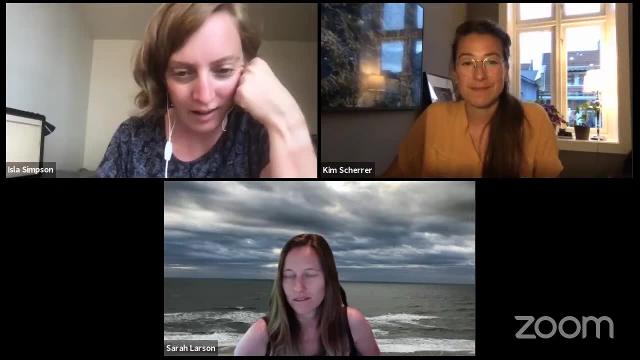 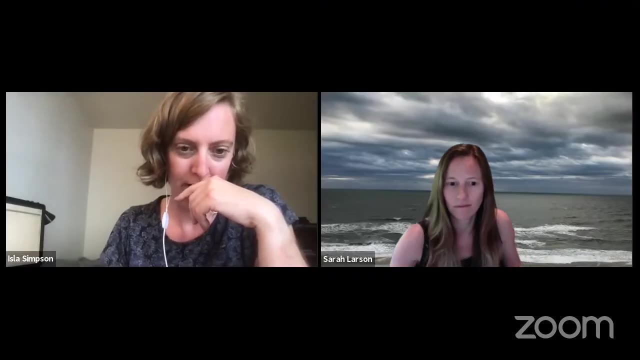 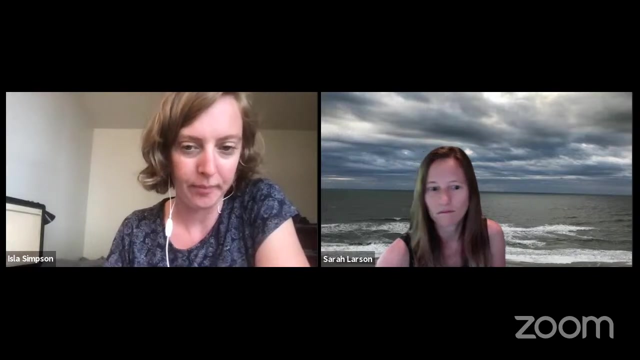 okay, i have a poll on mine. oh, you do. okay, did i make you the host so you can see? uh, yeah, sure, so on mine it's between the participants and the chat it says polls, so hold on. i'll have to um, switch it back, unless you want to be the one that stops all the 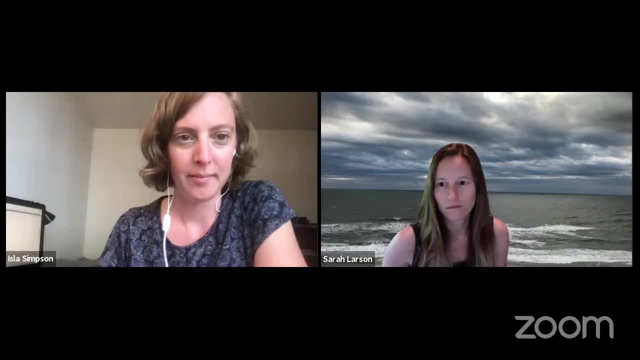 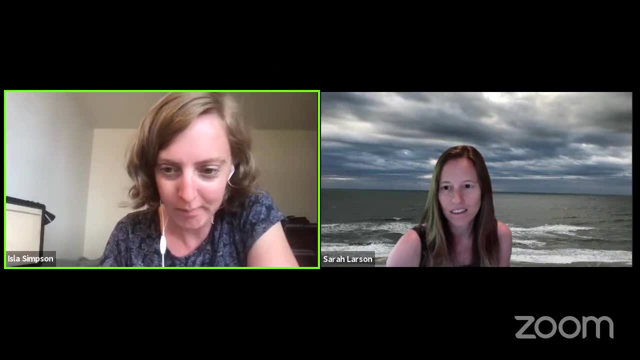 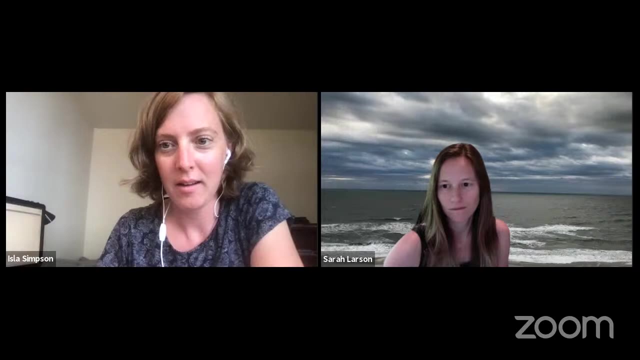 live stream and recording, which you're very capable of. so now, um, the whole feature went away on mine and you're very capable of selecting all the data Gravity, returning it backix, and maybe you should make me co-host. i don't, i don't have it. 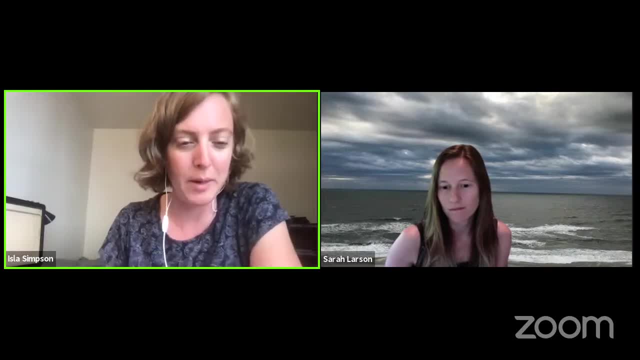 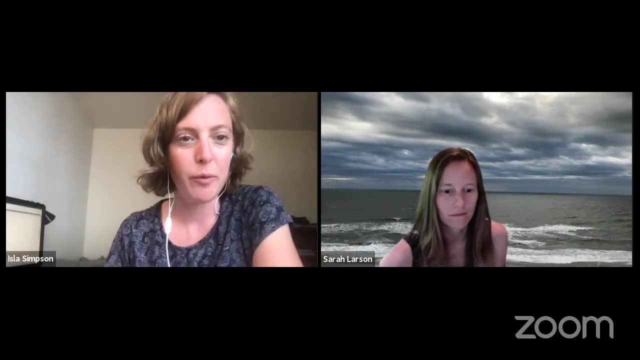 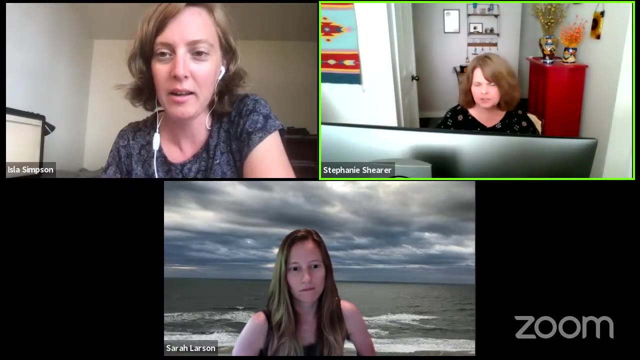 maybe it's just because you made the meeting. well, if you want to do it, i guess i guess. do you have it back now or let me make somebody? yeah, i still can see it. it went away all right, okay, for a second, but now i can see it again. you hover over the bottom of the screen, yeah, and 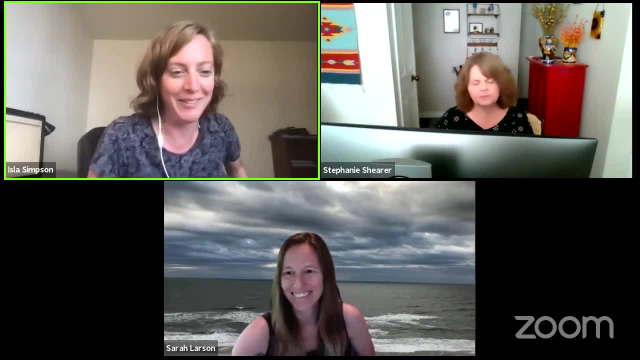 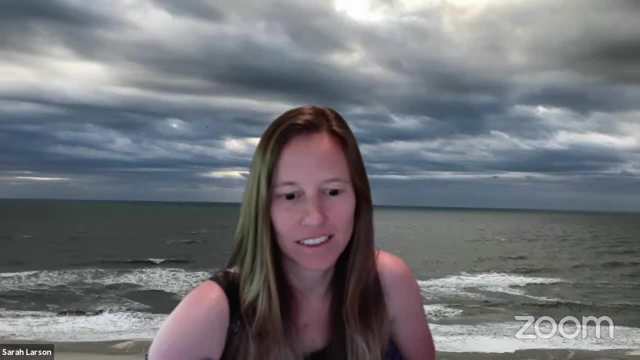 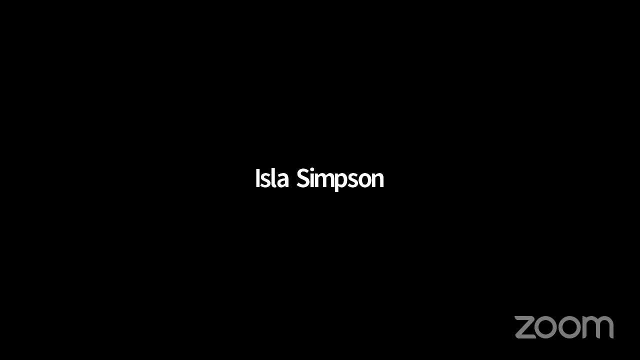 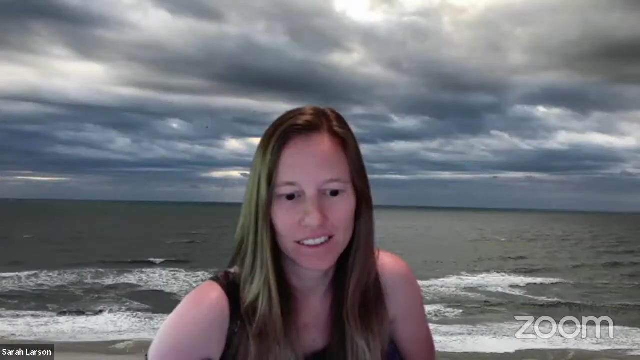 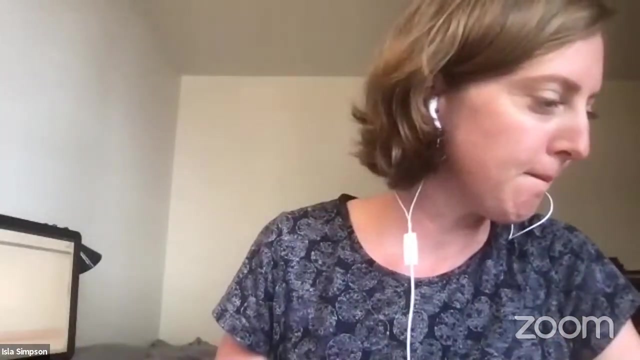 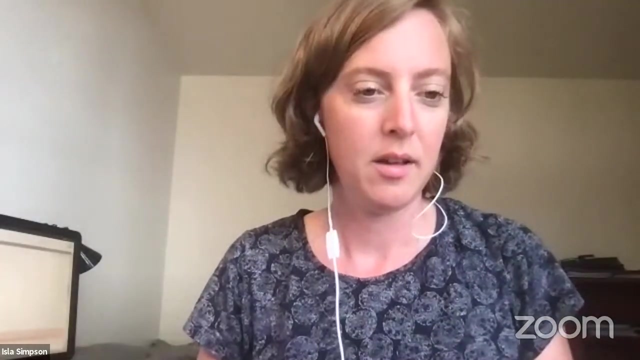 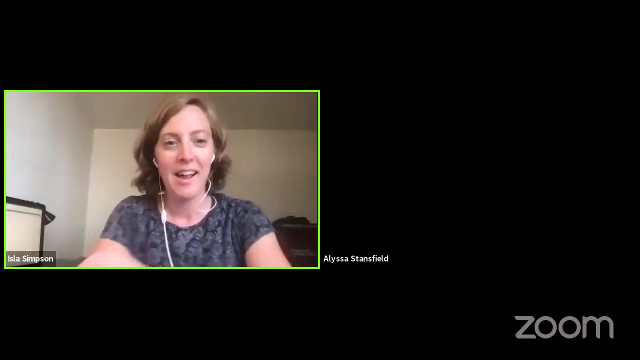 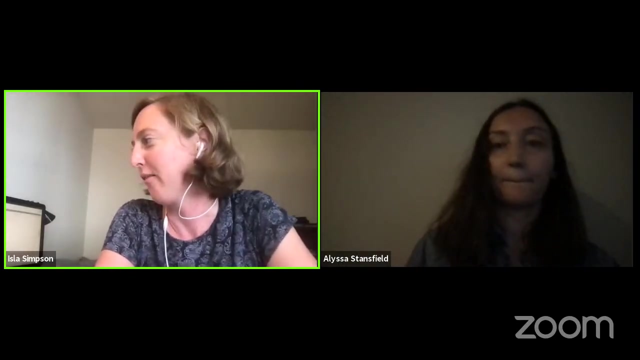 we're just going to go to the restroom before we start again. okay, we can figure it out. okay, you, you, you all, right, hello, it's uh three o'clock. sorry, that was a short break. um, we'll get started with the the final session of our uh working group meeting before we have a discussion, and so this session is. 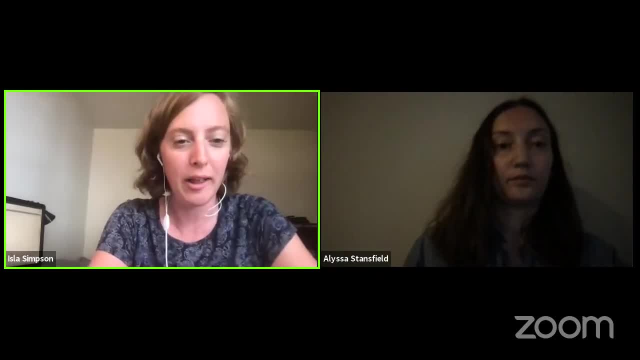 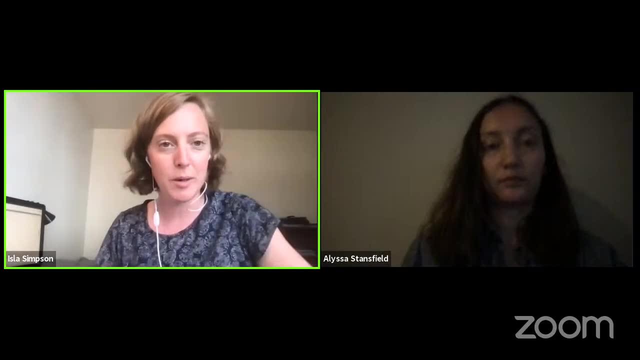 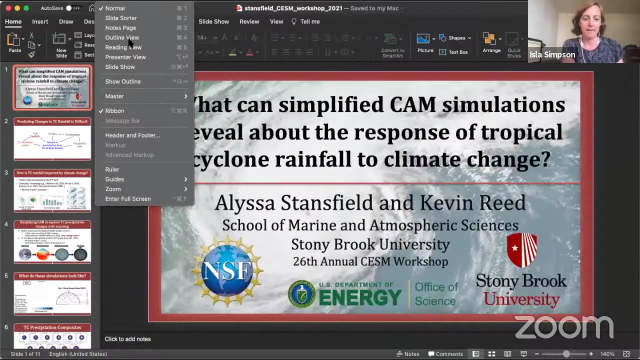 about extremes and severe weather and the hydroclimate. so we'll start with alissa stansfield and just a reminder for the speakers, i'll give you a two minute warning- warning at eight minutes- and then we'll stop at 10 minutes. okay, great, thank you. can you see my slides? 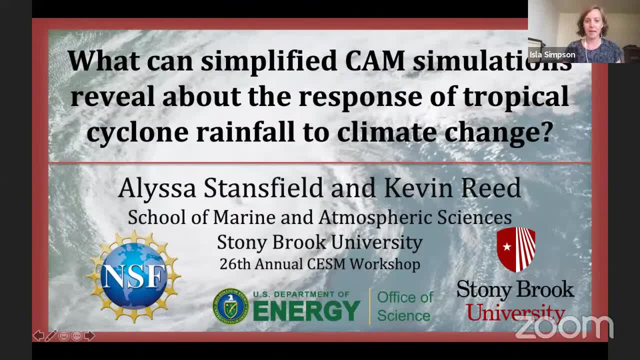 um, yes, okay, great, um, so thank you. my name is alissa stansfield, i'm a phd candidate at stony burke university, and this is work i've been doing alongside my advisor, kevin reed, and so we are trying to use simplified cam simulations to try to understand the response of tropical cyclone rainfall to 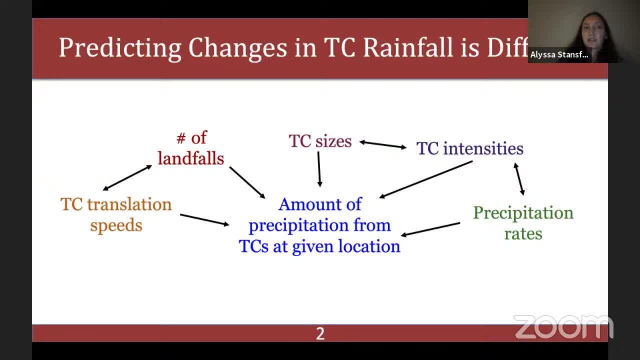 climate change, and so it probably comes as a surprise to no one here that predicting changes in tropical cyclone rainfall is difficult. um, there's a lot of things that go into predicting the amount of precipitation from tcs at a given location, such as the number of landfalls, the 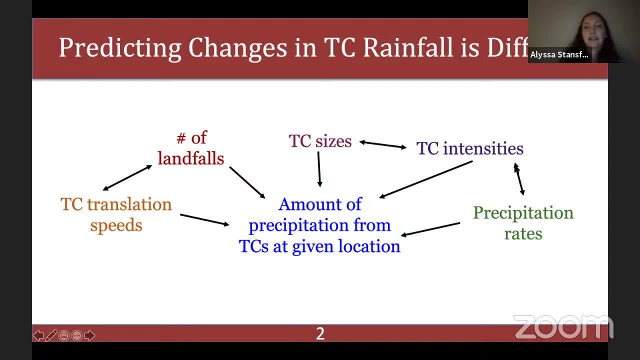 translation. speeds of the storms, their sizes, intensities and the precipitation rates, and also the amount of precipitation that we're predicting is difficult to predict because all of these factors also interplay amongst each other, to you know, produce the amount of rainfall from tropical cyclones, and this is important because rainfall from tropical 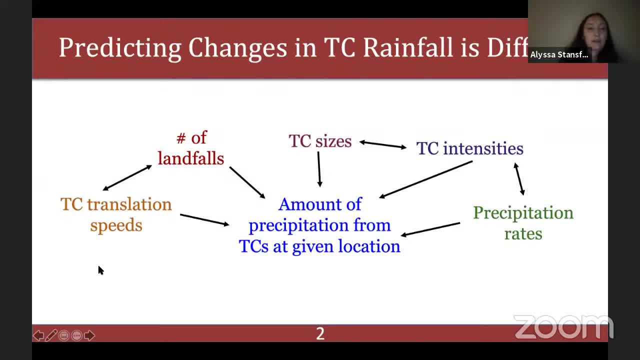 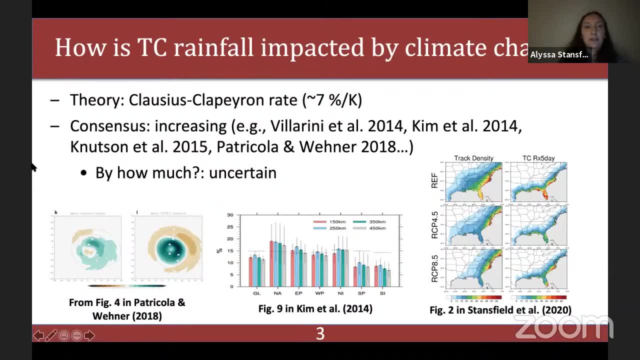 cyclones can be not only deadly but also very economically destructive, and so what do we know about? um how tc rainfall is impacted by climate change? so the theory, um kind of behind this, the predictions, is the clausius claperon rate, which so basically the thought is that since water, the amount of water vapor the air can hold. 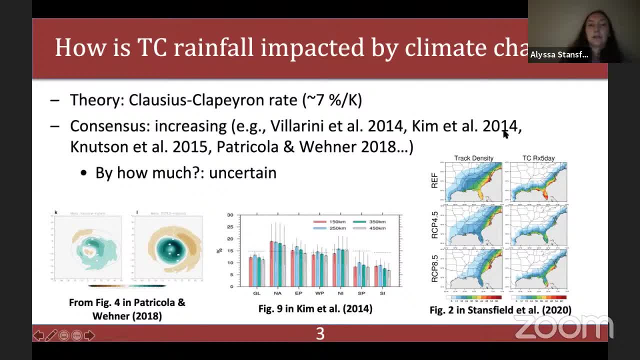 increases by about seven percent per degree of warming, um that the rainfall from extreme events like tropical cyclones will follow that rate. um and so um. the consensus from different modeling studies is certainly that, yes, tc rainfall should increase in the future, but by exactly how much um. 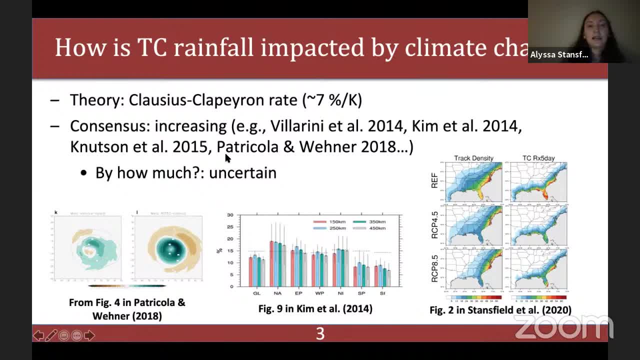 and if that's going to follow the clausius claperon rate is kind of uncertain and so we're going to roll these off with a several topic, that about a couple dates, um, that are failure to predict if any of you need to follow along, and so with that we're gonna try to, you know. 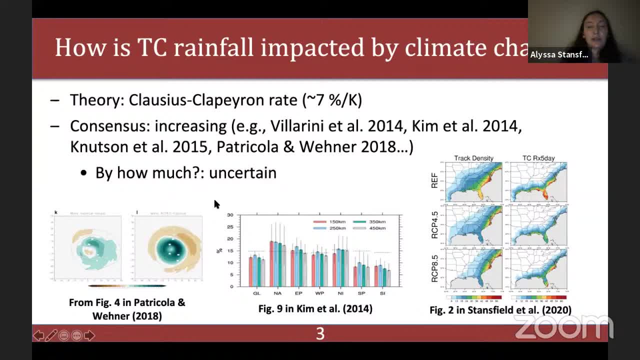 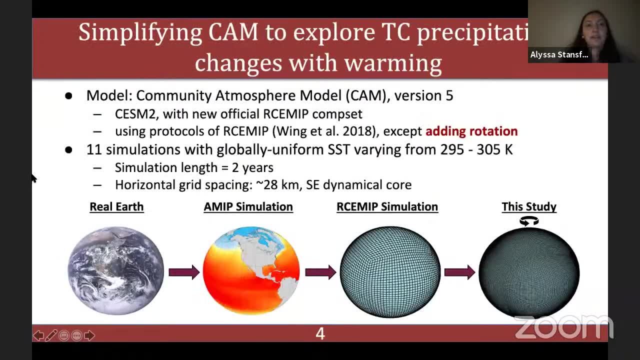 understand that we wanted to figure out in about of these Lehrman Law, which i we'll give a couple guided notes specifically. so during this the we won the trial period that we wanted to simulate before looking at, and so the first kind of question that came up of that was: 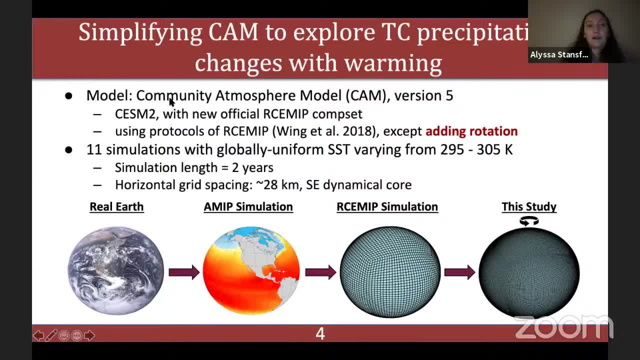 what would we now actually be basing this fruition on now? so, with the official RCE-MIP comp set that has come out with CESM2, and I'm using the protocols of RCE-MIP, which are detailed in Wing It All 2018, except I'm adding rotation- 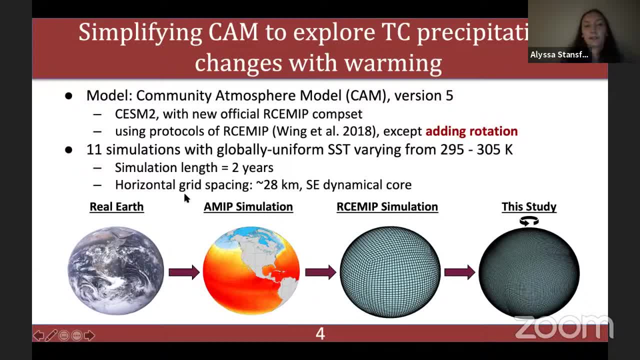 And so the idea is that, you know, we start with the real Earth. we can represent the real Earth using, like AMIP-style, more realistic simulations, Then we can simplify further to the RCE-MIP simulations, which are aqua planets, uniform. 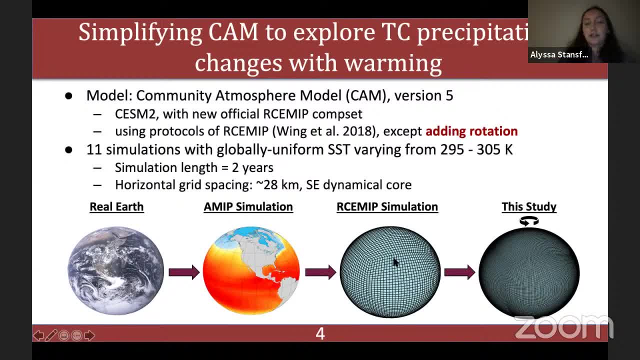 SST everywhere. the solar insulation is uniform all over the globe and the aerosols are constant, And so again. then we get to my simulation, which is like RCE-MIP, except the Earth rotates and we are running the cam at about 28-kilometer resolution. 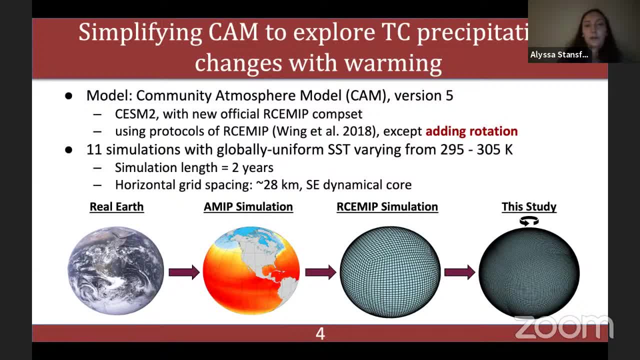 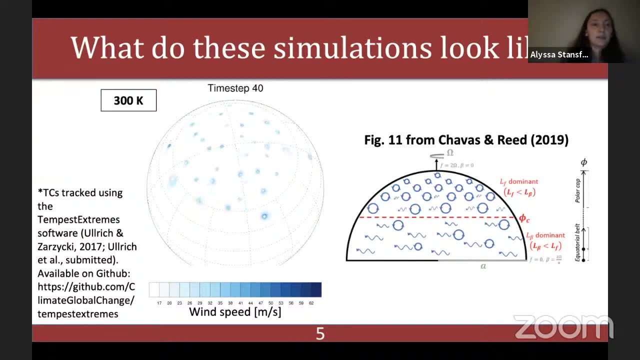 So I run 11 simulations With a globally uniform SST varying from 295 to 305 Kelvin. again, I'm using 28-kilometer grid spacing and the SE dynamical core. And so quickly, what do these simulations look like? 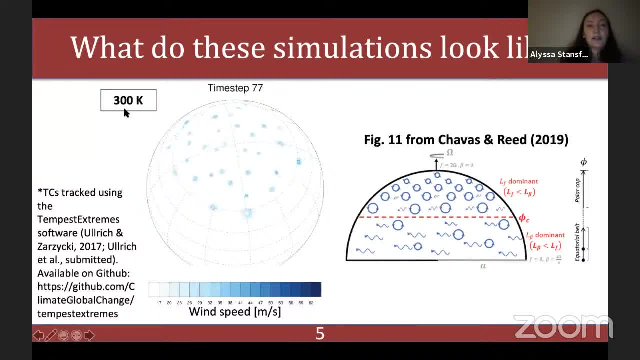 So you'll see on the left an animation of wind speed and the 300 Kelvin simulation, And so all of these little dots here are tropical cyclones tracked using the Tempest Extreme software, And so what we see is that TCs in these TC worlds tend to form in the tropics and subtropics. 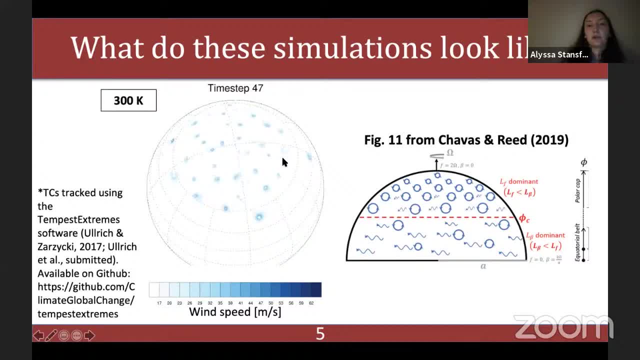 move poleward with beta drift and then kind of accumulate up near the poles, And so we're not the first to use these type of simulations. Chivas and Reed 2019 did a kind of more dynamical look at these simulations, But what I'll just note here is that, for the precipitation analysis that I'm going to show, 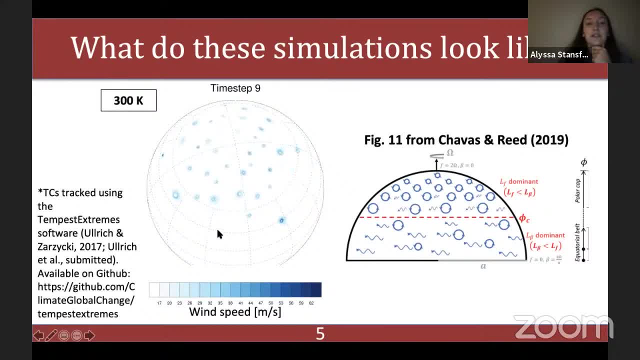 you, we limit it to 40 degrees, And so we're not the first to use these types of simulations, So we're not the first to use these types of simulations, So we're not the first to use these types of simulations. But we've got about 30 degrees south to 40 degrees north, because we kind of want to. 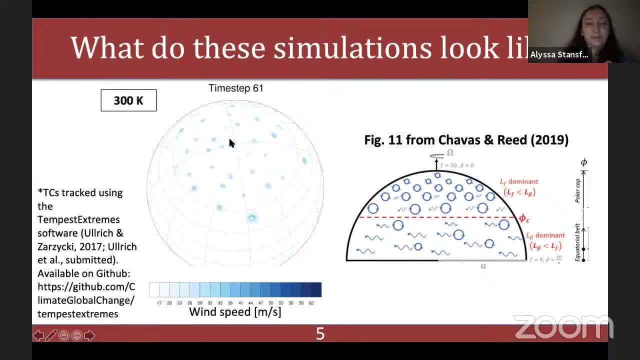 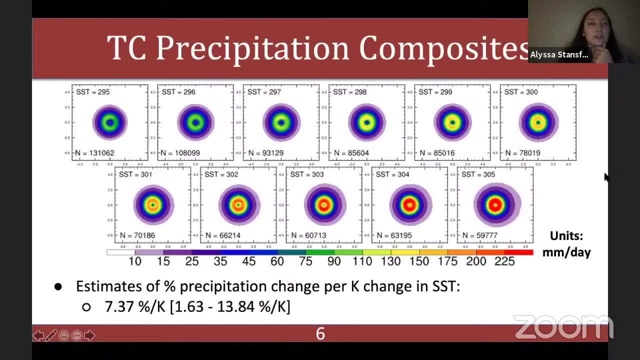 avoid the complications of the TCs that are near the poles and the interactions between them. We don't want to deal with that. So here's just some TC precipitation composites. So each box is a different simulation with a different SST. that's up on the top left. 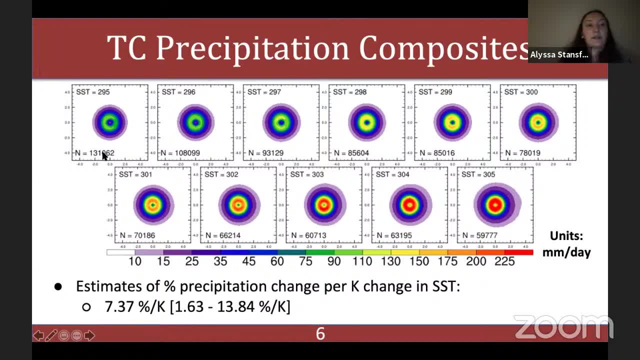 And then the number of snapshots that go into these composites. it's on the bottom. So what we see here is that definitely in the inner core the TC precipitation increases And then also it seems that as the SST increases the precipitation field seems to expand a. 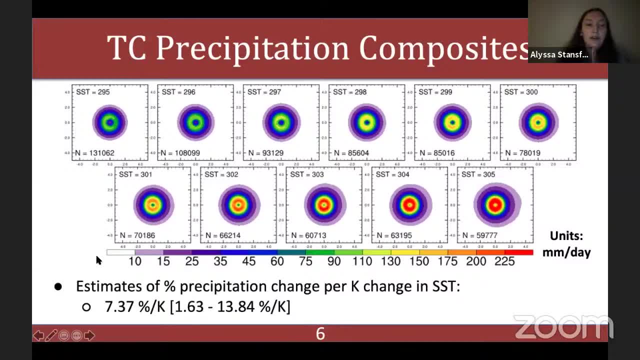 little bit as well, And so if I do a simple estimate of the percentage precipitation change per Kelvin change in SST, we get about 7.37% per Kelvin change, which is probably slightly above Clausius Clapeyron, although there's a kind of a large range of uncertainty in the way that we calculated. 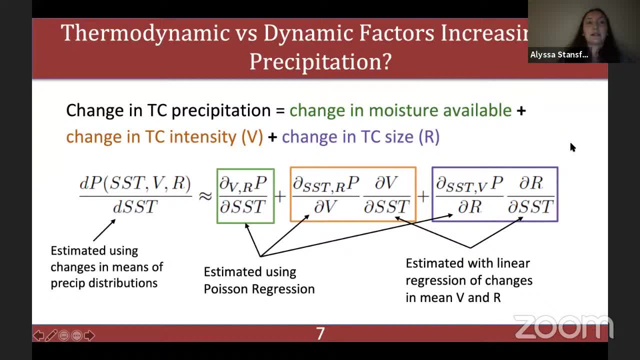 that. So next we want to ask: how much do the thermodynamic versus the dynamic factors increase affect the increasing TC precipitation? So we kind of created this equation that estimates the change in TC precipitation is equal to change in the moisture availability, which is the thermodynamic factor plus the change. 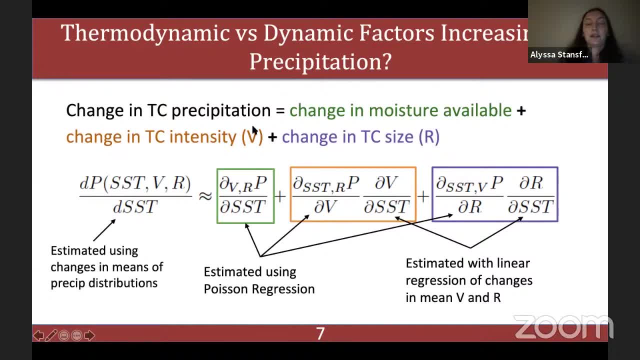 in TC intensity plus the change in TC size, which we consider the changes in intensity and size, the dynamic changes, And so we kind of divide this up into these partial derivatives. I won't go too far into this equation because I don't have time, but basically we estimate: 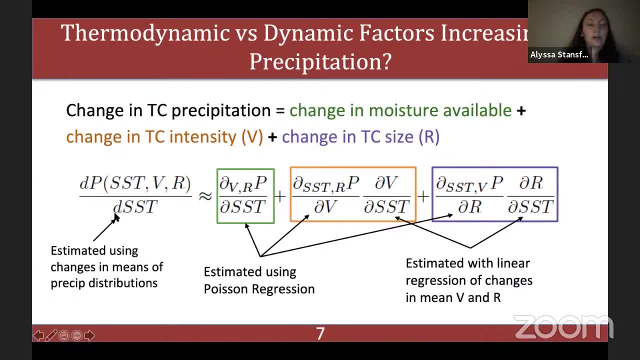 the total change in precipitation per SST change on the left using the changes in the means of the precipitation distributions within the TC. The DP changes, based just on the changes in SST, change in intensity and change in size, are estimated using a Poisson regression, And then the changes in intensity and size per change in SST are estimated with linear. 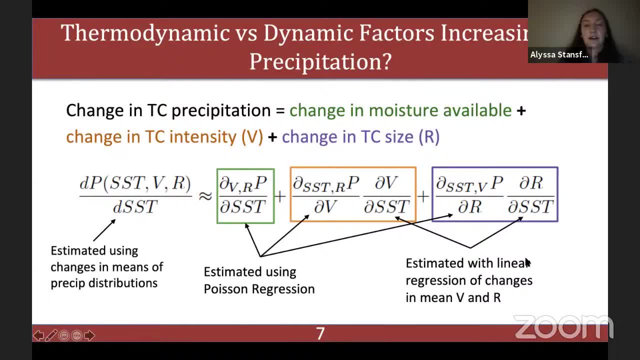 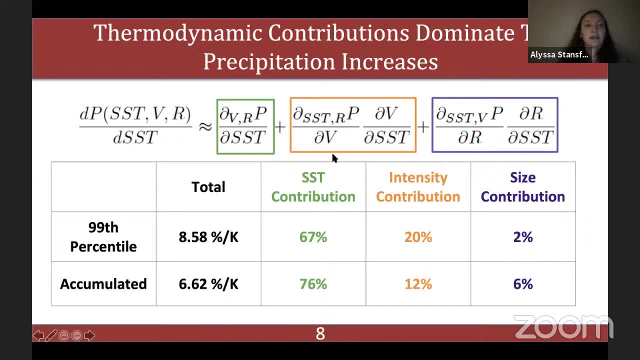 regressions of the changes in mean intensity and size, And so these are the kind of rudimentary results of this analysis. So we look at two different precipitation variables, the 99th percentile and the accumulated TC precipitation, And so the colors correspond to the different kind of contributions. 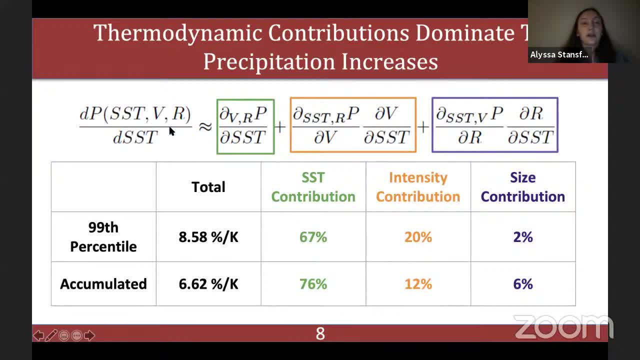 Well, first of all, the total change in precipitation per Kelvin is 8.58 for the 99th percentile precipitation and 6.62 for the accumulated. So they're around Coseus-Cofferon, Although the 99th percentile is 8.58 for the 99th percentile precipitation and 6.62 for. 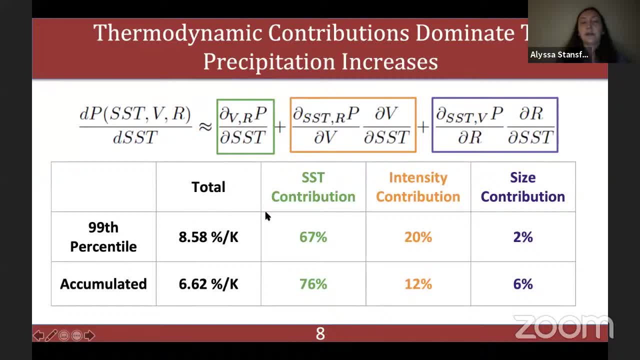 the accumulated. So the 99th percentile is certainly a little bit above, And what we found was that the SC, so the thermodynamic contribution, kind of dominated the precipitation increases for both accumulated and 99th percentile. The intensity, however, contributed a bit more for the 99th percentile, whereas the 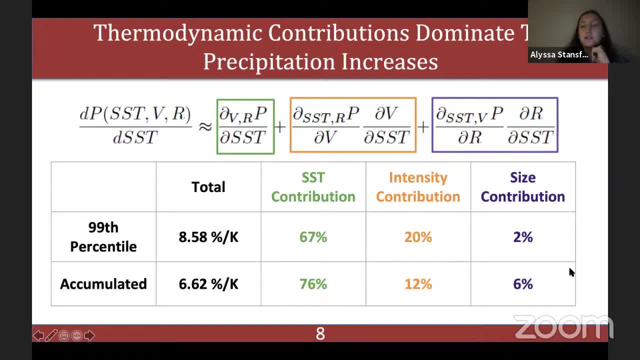 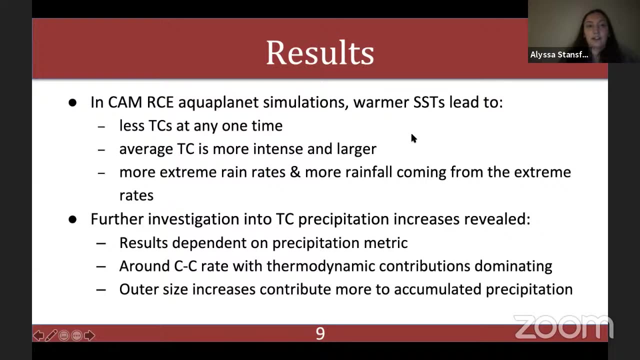 size contributed more for the accumulated, which makes sense, since as a storm gets larger there, So it should be more precipitation. So just some quick results, and these top ones I did not show in this presentation, but I just thought I'd mention them. 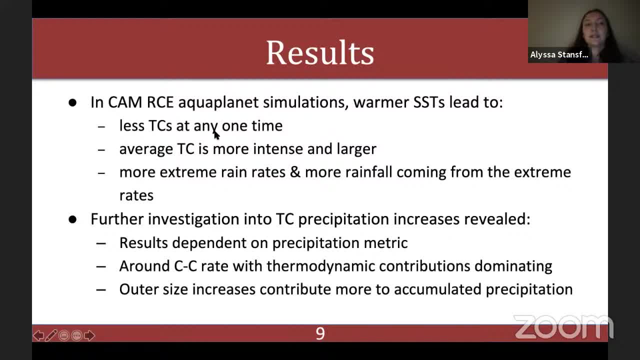 In these simulations, as the SST warms, there's less TCs at any one time. The average TC is more intense and larger and there's more extreme precipitation rates within the TCs and more rainfall is coming from these extreme precipitation rates. 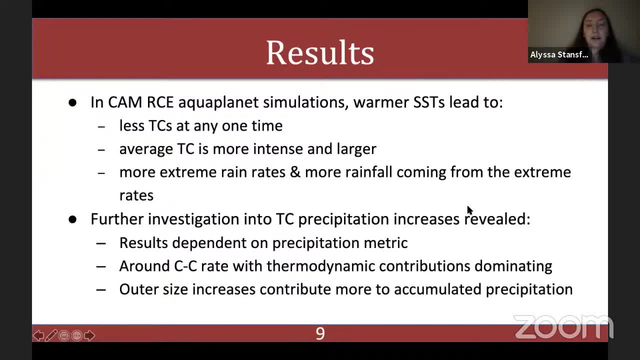 And then when we dove a little bit further into the TC precipitation analysis, we found that the exact results kind of depend on the precipitation metric that you use. The precipitation changes were around the Clausius-Copperon rate, slightly above for the 99th percentile, and the thermodynamic contributions dominated over the dynamic. 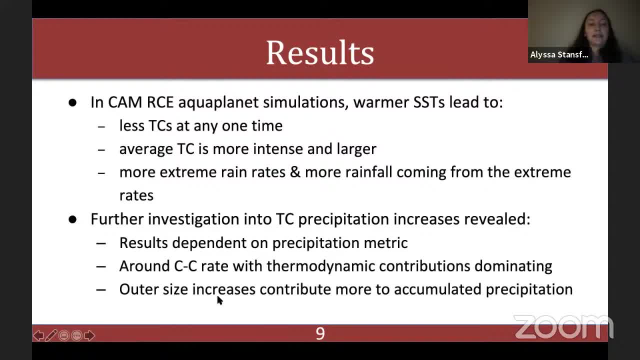 contributions to the change, And, while the intensity contributed more to the precipitation, the precipitation changes were around the Clausius-Copperon rate, slightly above for the 99th percentile, and the thermodynamic contributions were around the Clausius-Copperon rate, slightly above for the precipitation. 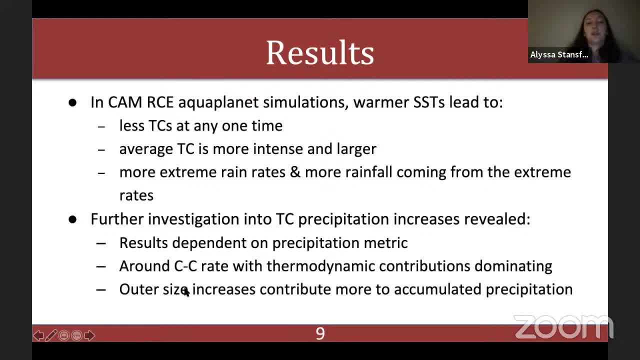 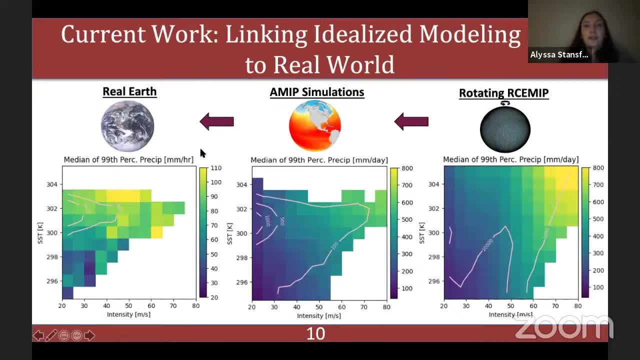 and the thermodynamic contributions were around the 99th percentile change. the outer-size changes contributed more to the accumulated precipitation changes, And so now my current work, which I'll just briefly mention, is: I want to link the idealized modeling back to the real world. 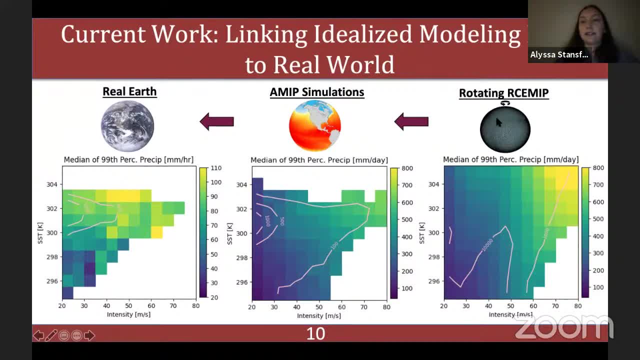 So I want to take this rotating RCE-MIP idealized simulations, see how they compare to AMIP simulations, as well as observations, And so I won't go too much in detail into these plots. But these are joint dependence plots of 99th percentile Tc precipitation. 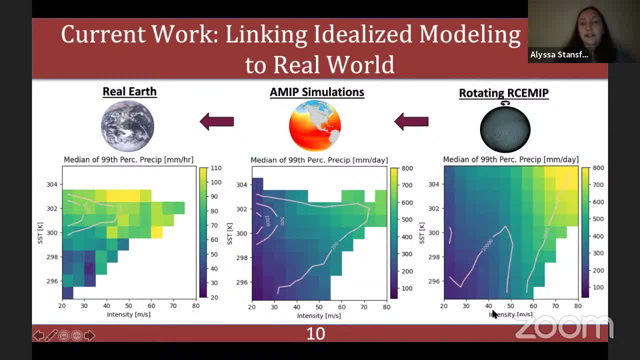 They're dependent on SST, which is the y-axis here, and Tc intensity, which is the x-axis, And so these plots. well, the two on the left are fairly new, so I'm still kind of working on this analysis. 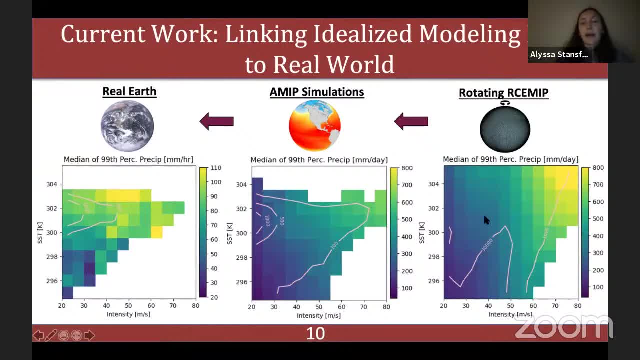 But so far it seems that the kind of pattern of these precipitation changes are consistent between the idealized simulation and the AMIP simulations and these observations which I got from the eMERGE satellite. But I'll probably be using other observations as well. 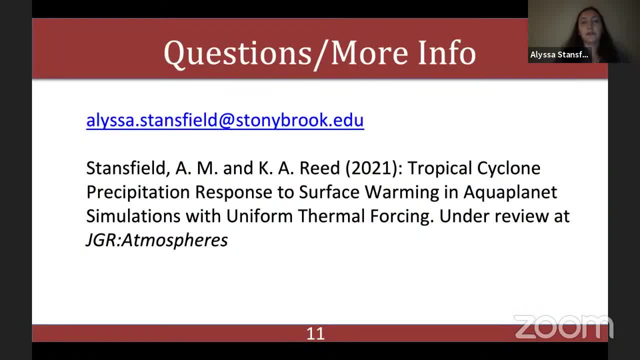 So I'll just mention that most of this work is under review at JGR Atmospheres And if you have any questions or want more information, If I have time for questions I can take them, And if not, my email is up on the slide. 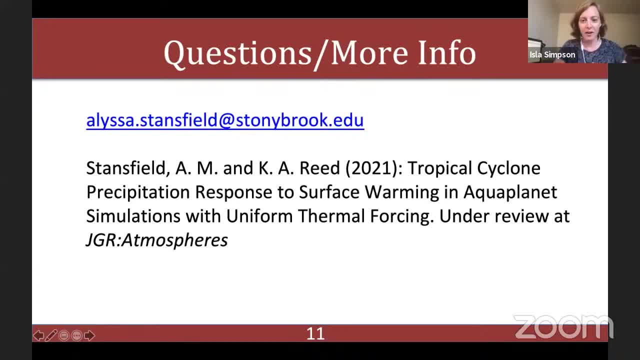 Thank you, Thanks. Are there any questions for Alyssa, I guess I'm wondering whether you see any scope for any kind of other experiments in between the AMIP and your ones, Like if you had meridional gradient and SST or something. do you think that would be helpful? 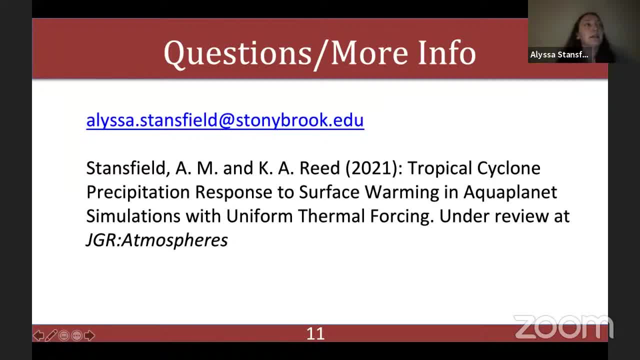 Yeah, that could definitely be kind of an intermediary. Another kind of more intermediary thing I'm thinking of using is reanalysis. So I think I'm going to use the ERA5 reanalysis to do because that's, you know, between maybe observations and AMIP simulations. 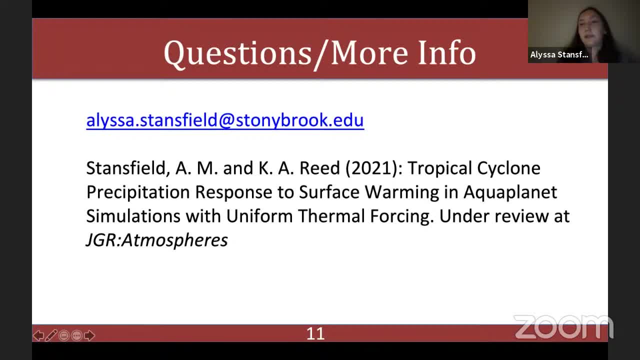 I'm not sure if I'll be able to get any more idealized simulations, as you mentioned in, just because I'm probably finishing my PhD next spring, But that would definitely be helpful. That would definitely be something interesting to do. 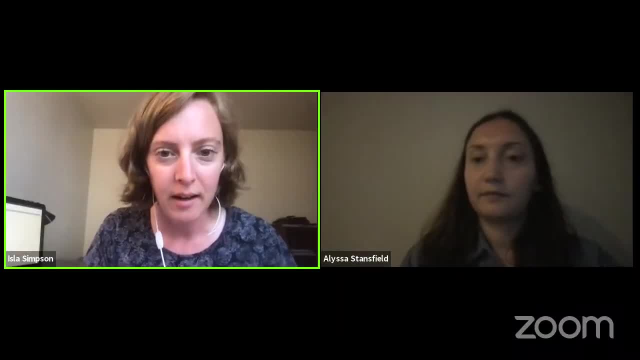 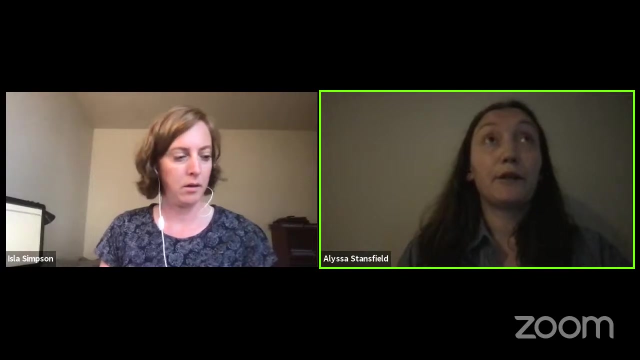 Okay, There's a question in the chat: What is it about the simplified model that makes rainfall fields look more symmetrical than they are in observations and fully coupled simulations? That's a very good question. My first guess is that there is just way more observations. 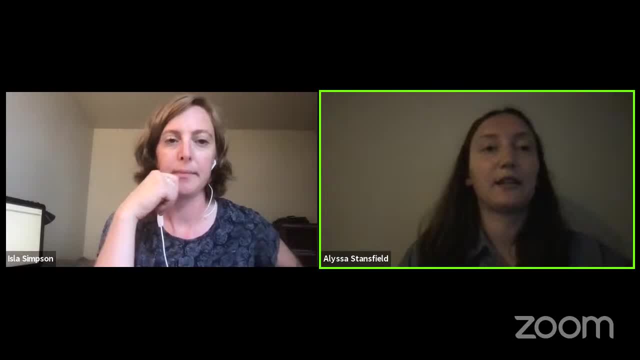 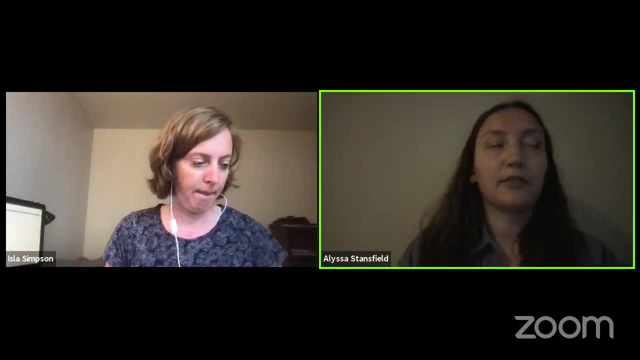 So I don't know if you are way more like snapshots, They go into the composites. that may be making them more symmetrical. Additionally, the other thing is that there's really not a lot of wind shear in these simulations. So you know, there's not any like extra tropical transitioning storms to kind of make a more asymmetrical shape of the storms. 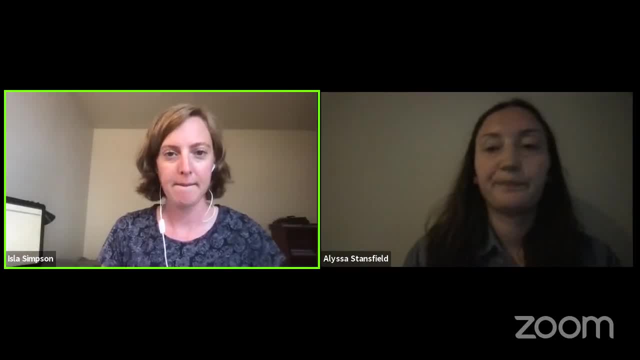 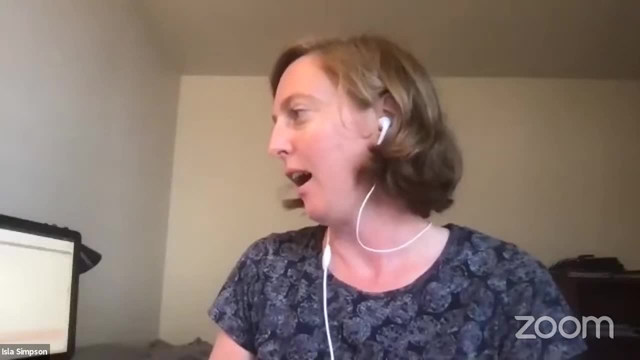 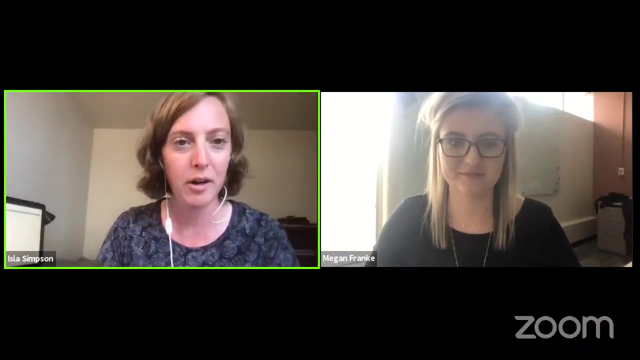 So that's my, my two thoughts. That's an interesting question though. Okay, thanks, We'll move on to the next speaker. If you have more questions for Alyssa, just type them in the chat, Okay, So our next speaker is Megan Frank talking about impacts of large scale and natural variability on severe weather over the United States. 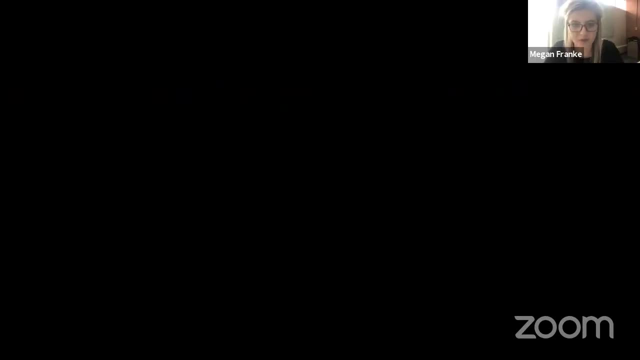 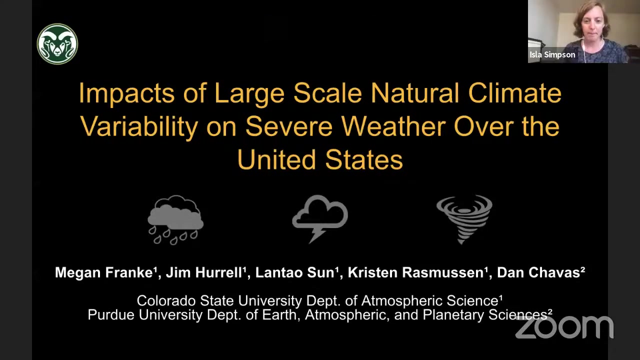 Hi everybody, Let me get this presentation pulled up here and go ahead and get rolling. All right, so I'm assuming you can see my screen, Yep. So hello welcome. My name is Megan Frankie and I am a master's student in the Department of Atmospheric Science at Colorado State University. 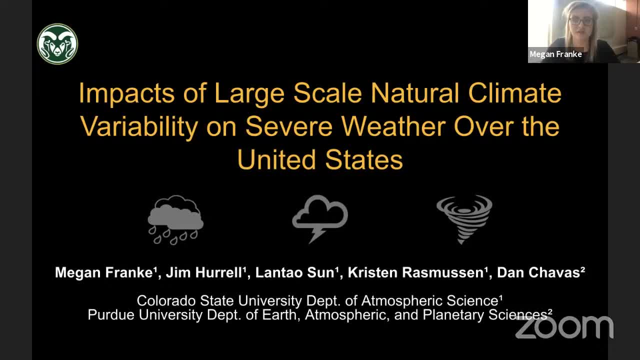 I would first like to take a second to thank the organizers of this workshop and the Climate Variability and Change working group for setting this up and giving me the opportunity to participate. Today, I will be sharing with you some of our work on the impacts of climate variability on large scale severe weather environments over the United States. 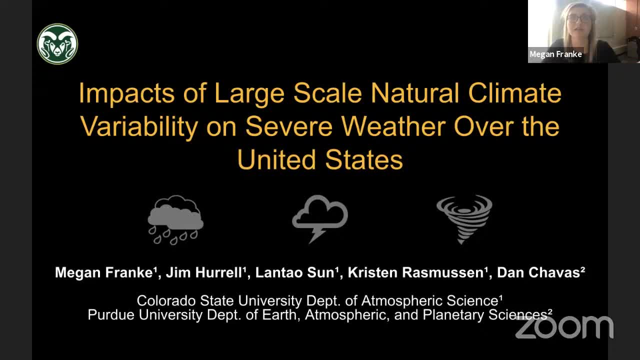 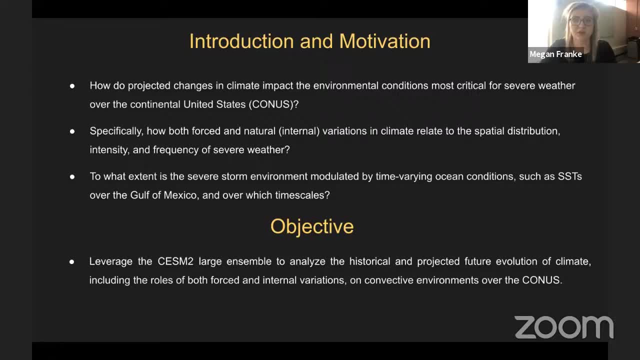 I would also like to acknowledge my collaborators listed at the bottom of the slide. In the United States, spring marks the onset of the severe storm season, which annually accounts for billions of dollars in damage. Therefore, understanding the future projected changes in convective environments could largely help to enhance. 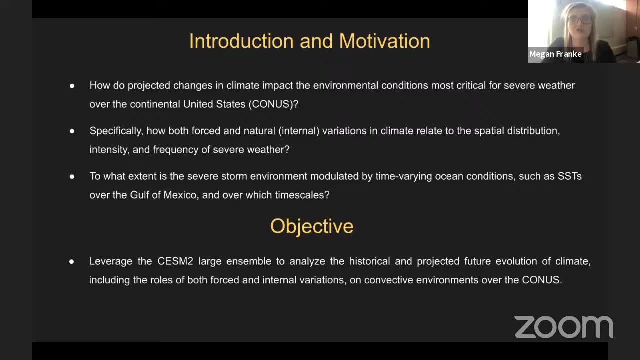 resilience to severe weather outbreaks. The overarching questions driving our research are listed below, but a major focus of our work is to understand how both forest and natural variations in climate relate to the occurrence of severe weather over the continental US by using the CESM-2 Large Ensemble to analyze the historical and projected future evolution of climate. 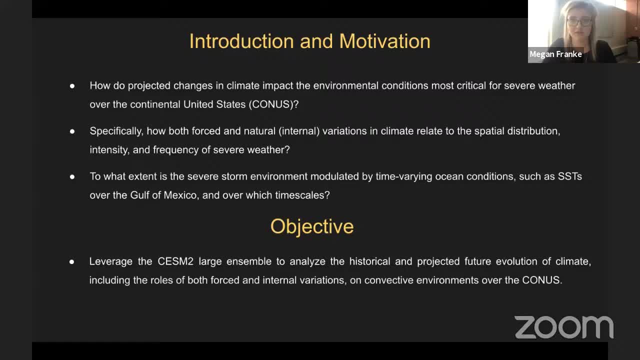 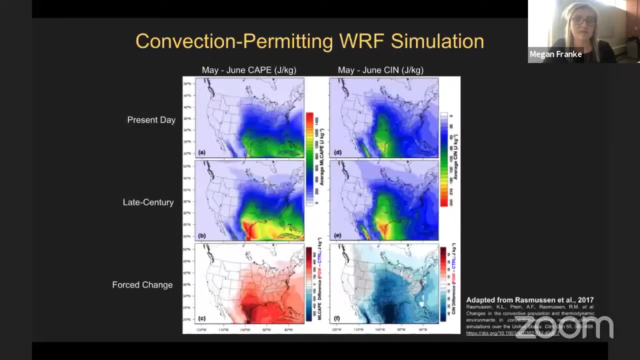 To date, the existing literature on this topic includes a limited number of studies that have used tools such as convection-permitting regional climate simulations under pseudo-global warming scenarios to examine how the forest component of climate change may impact the severe weather environments over the United States by the end of the century. For instance, this figure is from a 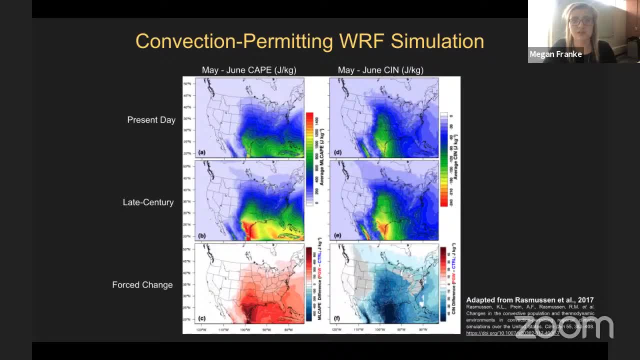 recent paper by Kristen Rasmussen and colleagues. It shows the end-of-century average mixed-layer convective available potential energy in the left column and convective inhibition on the right for the months May through June. They forced WARF with ERA-5 data to produce a control run shown in the 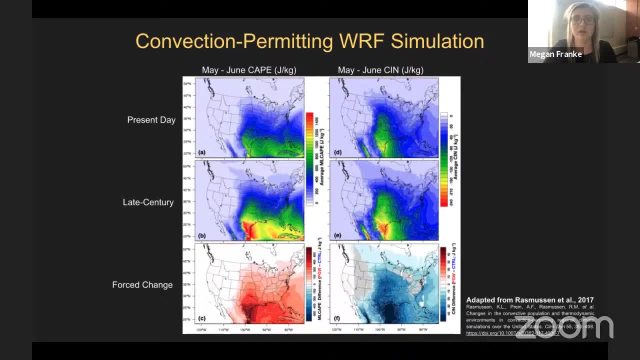 top right. The difference between the two thus can be viewed as the force signal associated with climate change. Briefly, what you notice are large increases in both the end-of-century convective available potential energy and convective inhibition over the eastern half of the US, with the largest. 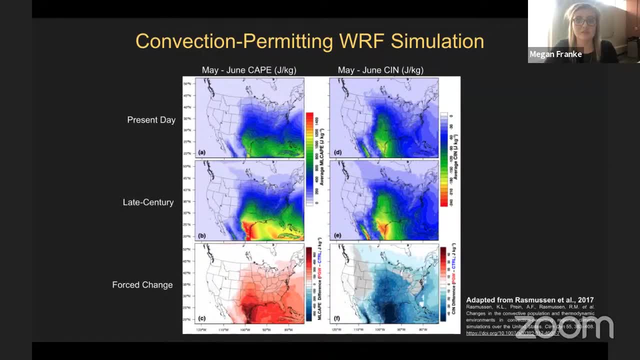 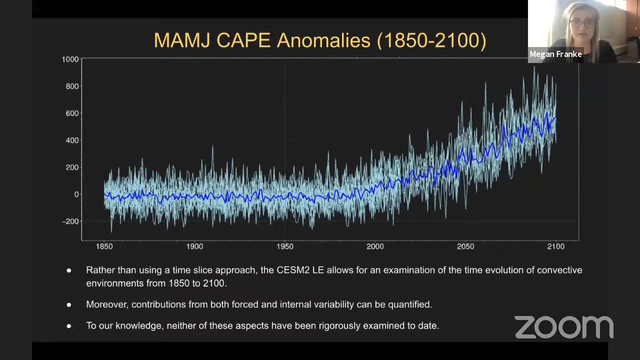 changes over the southern and southeastern regions. Increases in both of these parameters are conducive to producing more intense severe weather. Instead of using a time-slice approach, as was previously seen, we are using CESM-2 large ensemble to compute severe storm parameters directly and examine how they have changed over time. 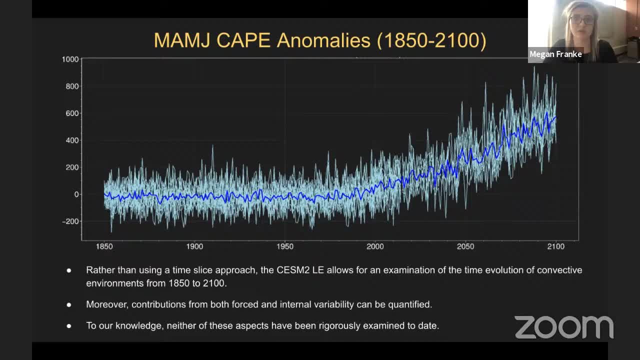 For instance, shown is the CESM-2 ensemble mean of cape from 1850 to 2100. in the dark blue line which illustrates the force response and the variability of individual ensemble members are shown in the background in white-blue, Visualizing a large ensemble approach from the CESM-2 also gives us the capability to evaluate contributions from both forest and internal variability. 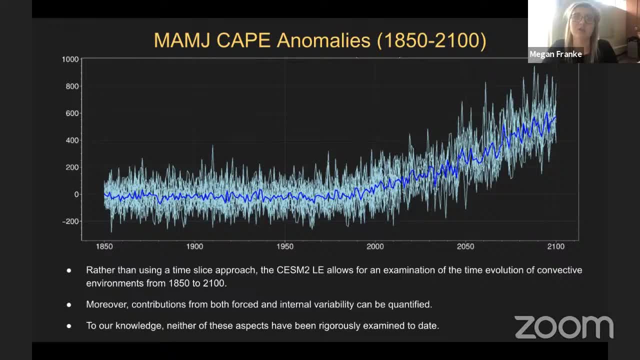 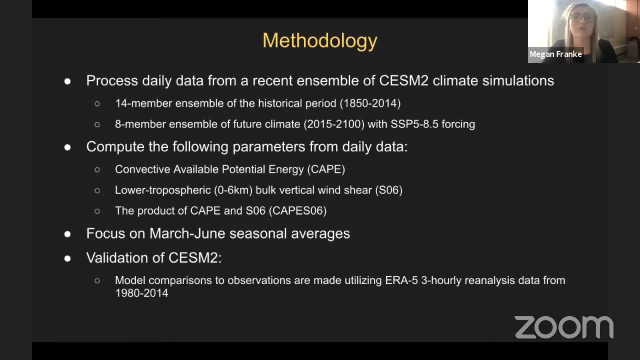 To our knowledge, the full-time evolution of these parameters and the role of the forest versus natural variability had not been rigorously examined to date. More specifically, but briefly, what we have done is process daily data from a 14-member CESM-2 ensemble of the historical period from 1850 to 2014, and an eight-member ensemble of future climate from 2015 to 2100.. 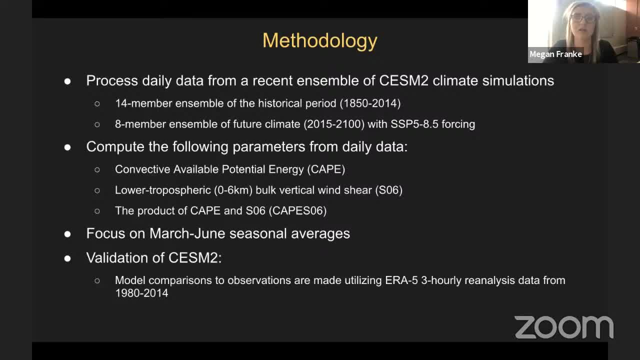 We then computed the following severe weather parameters from daily data. First is the conductive available potential energy, or CAPE, which is a good indicator of how buoyant an air parcel is. Next, the lower tropospheric bulk vertical wind shear, or SO6,. 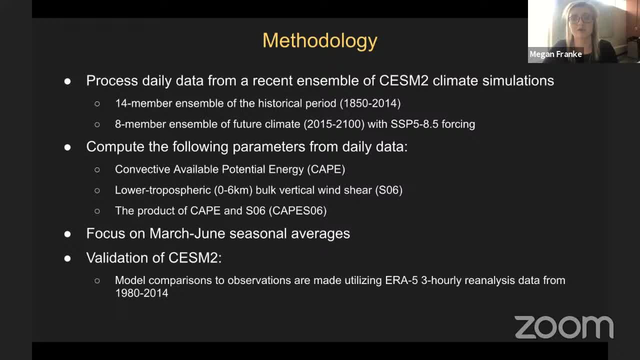 which is a good indicator of how buoyant an air parcel is. This measures the difference between winds at the surface and six kilometers above ground level and is useful in determining storm type and organization. And, lastly, the product of CAPE and SO6, CAPE-SO6,, which is proven to be a useful proxy for capturing both the kinematic and thermodynamic components of a thunderstorm. 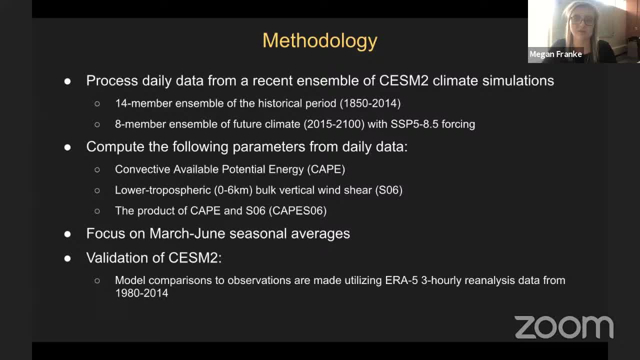 Previous studies have shown CAPE-SO6 to be useful in discriminating between severe and non-severe storms. Our focus is on the March to June seasonal averages, as it is the peak severe weather season. To validate our model, we are using various reanalysis products, but here I will only show results from ERA-5.. 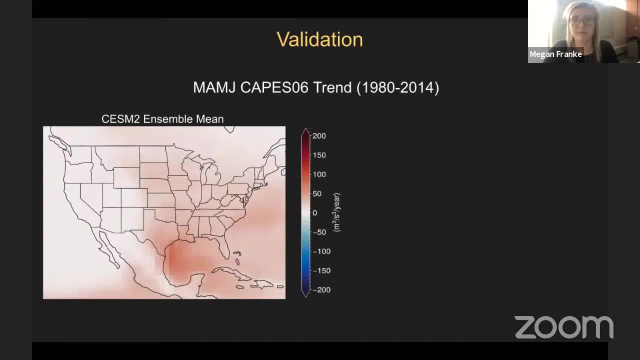 This image shows a 30-year historical period for March through June. CAPE-SO6 ensemble average for all 14 members from CESM, Recalling the force signal of CAPE adapted from Rasmussen and colleagues. we can see similarities in the patterns of end-of-century CAPE and historical CAPE-SO6 trends, especially over the southeast. 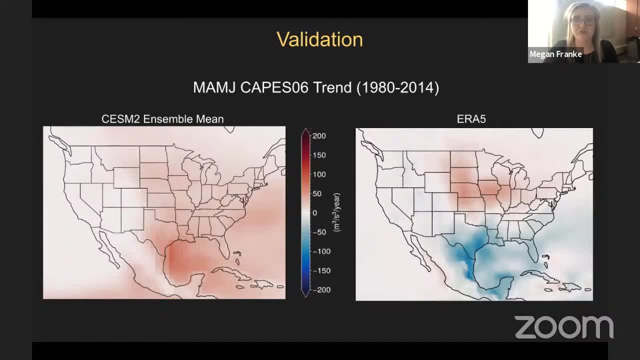 Although when you consider a March through June CAPE-SO6 trends from ERA-5 for the same period, seen here on the right, there is a significant difference in the patterns and magnitudes. Now trends from reanalysis products are problematic to begin with. 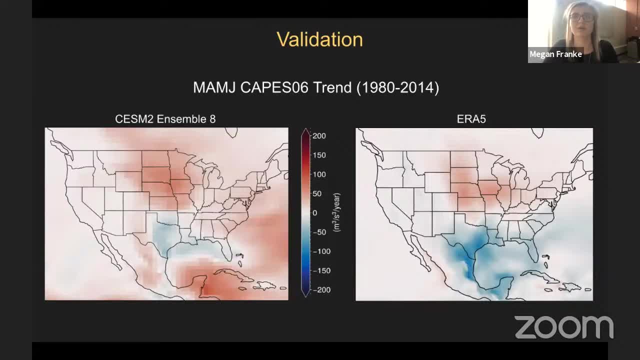 but it is important to note that if we consider a single ensemble member from the CESM, as seen here, rather than the ensemble mean, we see a different story. Now not only are the magnitudes of CAPE-SO6 of similar values. but the patterns of ERA-5 are also different. Now, not only are the magnitudes of CAPE-SO6 of similar values, but the patterns of ERA-5 are also different. But the patterns of ERA-5 are also different. 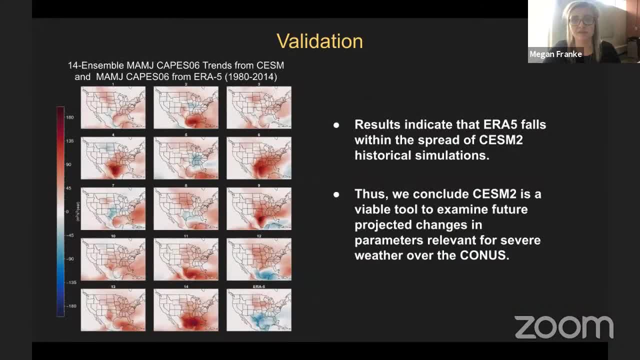 To further illustrate the run-to-run differences due to natural climate variability, here I show the CAPE-SO6 trends of all 14 individual members over the historical 30-year period, as well as the ERA-5 trend for the lower right. 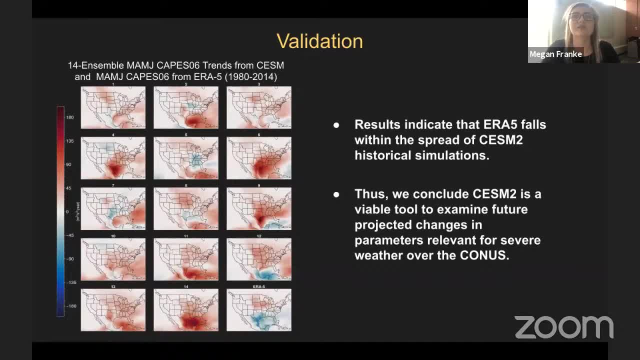 Again, as each ensemble member is a single realization of how nature might have evolved, the ERA-5 falls within a range of plausible outcomes over this period simulated by the CESM. The ERA-5 trend for the lower right is a single realization of how nature might have evolved. the ERA-5 falls within a range of plausible outcomes over this period simulated by the CESM. 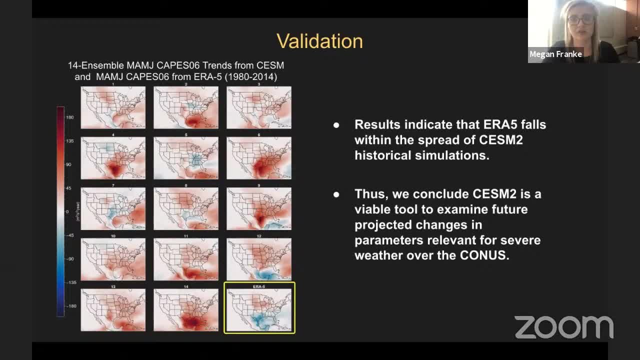 The ERA-5 trend for the lower right is a single realization of how nature might have evolved. the ERA-5 falls within a range of plausible outcomes over this period simulated by the CESM, Therefore giving us confidence in using this model as a tool to look at future projected changes in convective environments, as I will show next. 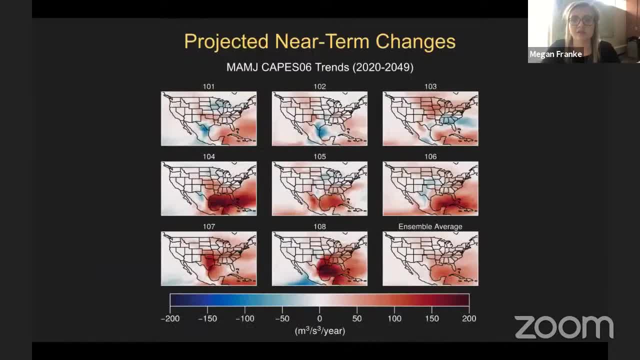 Therefore giving us confidence in using this model as a tool to look at future projected changes in convective environments, as I will show next. Shown here is the evolution of CAPE-SO6 over the next 30 years, from 2020-2049.. 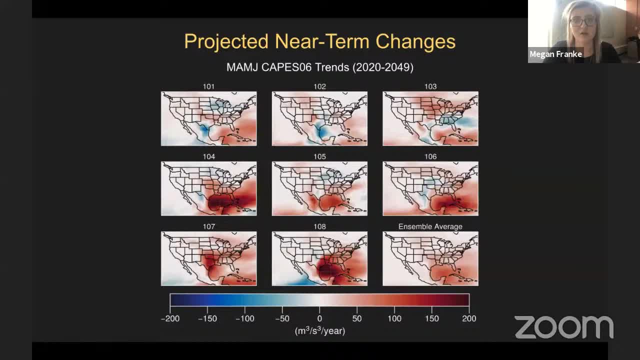 Because of time, I will hereafter only focus on CAPE-SO6, although we are analyzing other parameters as well. As a reminder, the red colors here indicate an increase, while blue indicates a decrease. This figure shows all eight future ensemble members from the CESM. 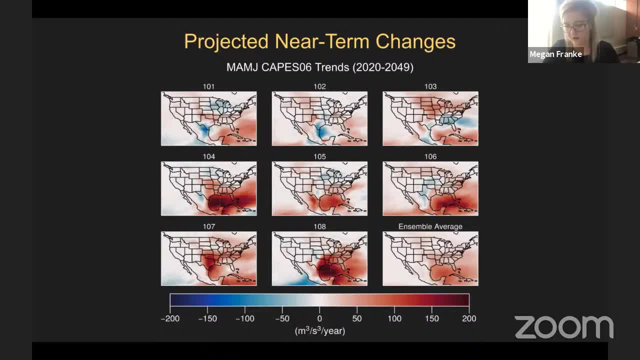 as well as the ensemble members from the CESM, as well as the ensemble members from the ERA-5.. the ensemble mean all forced, with SSP5 8.5 forcing In the bottom right we can see the ensemble mean trend or the forced greenhouse gas response, which shows increases in CAPE-SO6. 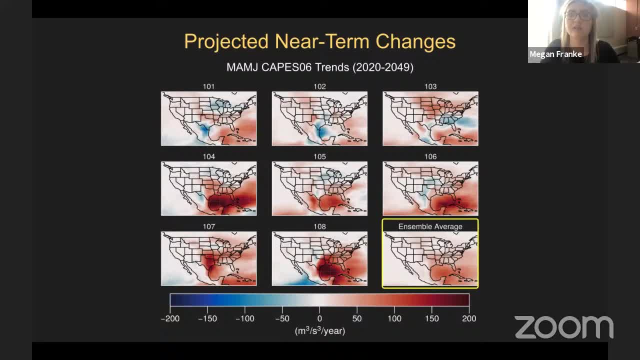 almost everywhere over the continental US, but particularly in the southeast and over the Gulf of Mexico. What is most interesting is that, although the ensemble mean shows increases in CAPE-SO6 similar to historical simulations, there appears to be large deviations between each. 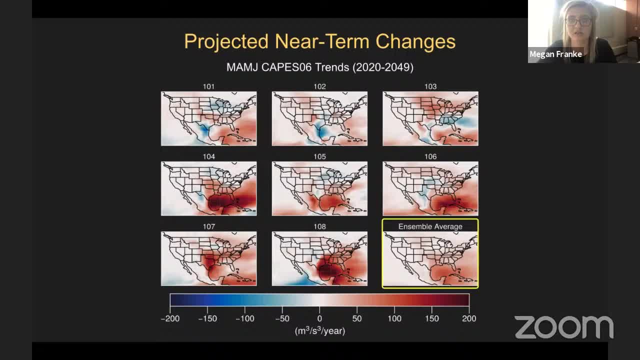 member. For example, to highlight contrasting runs: ensemble member 3 shows negative trends for CAPE-SO6 over the southeast US, which strongly contrasts with ensemble member 8, which instead shows a strong positive trend in this region. Taking this a step further, 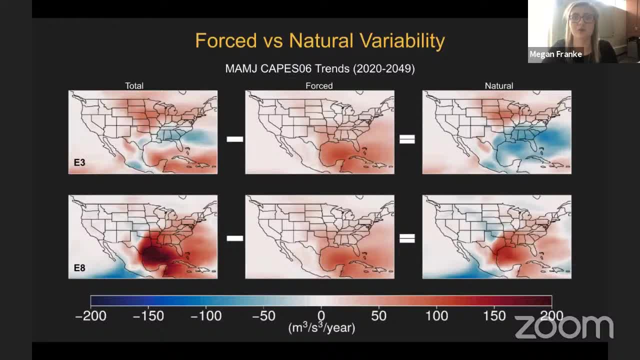 we can use ensemble members 3 and 8 from the previous slides, both with very different trends, and decompose them into the forced and unforced signals to try to better understand and highlight the differences that may be expected due to the natural and internal climate. 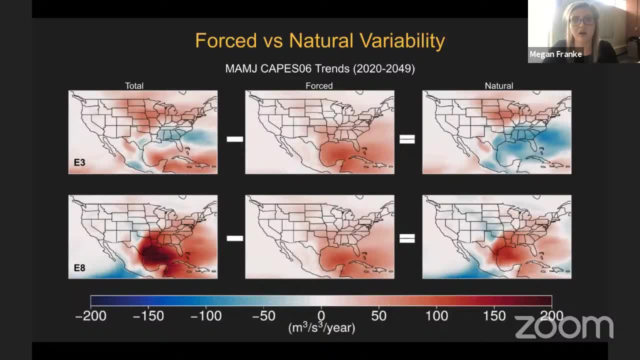 Or internal climate variability alone. Focusing on the right column, or the component of the trend due to natural climate variability, we can see that the natural variability can either act to suppress the increases of CAPE-SO6 due to anthropogenic climate change, which is the case. 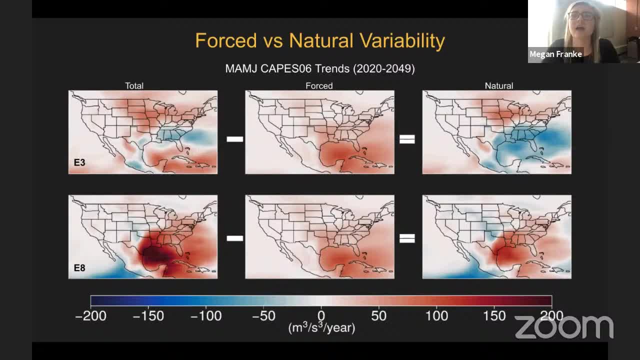 for ensemble member 3 here on the top, or act to add to the increases of CAPE-SO6 due to climate change, as seen with ensemble member 8 on the bottom. The most important point overall is that the unforced variability spatial structure is large and coherent and is of the same magnitude. 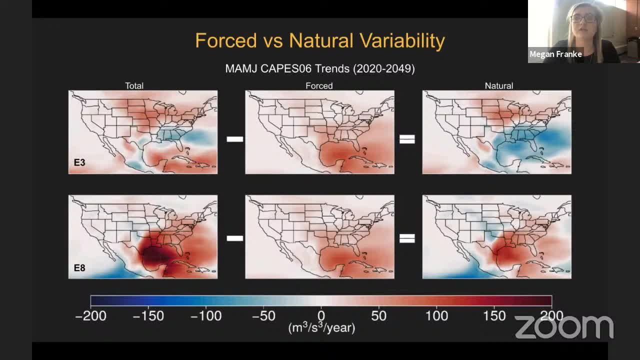 as the ensemble member 8 on the bottom. The most important point overall is that the unforced variabilities need to stay. Unforced variability is just as important to consider. Another aspect of my graduate work in the north karelian cohort is to focus on the specific 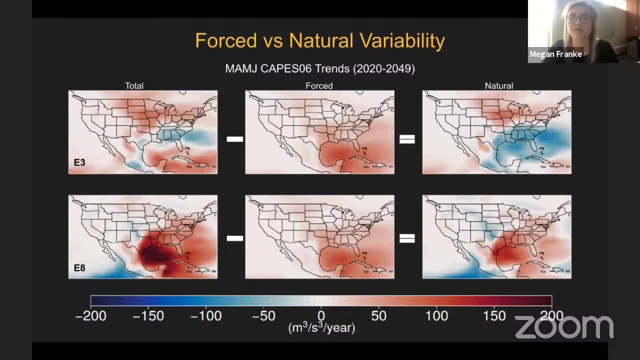 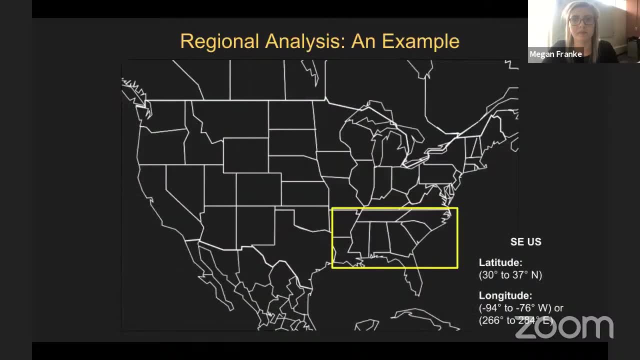 regions, to quantify the role of internal variability and to further understand how natural variability in these conductive parameters might be tied to regional changes in sea surface temperatures. Although I am evaluating various regions, such as changes in conductive environments over the great plains or the south central US, today I am only sharing results over the southeast uS. 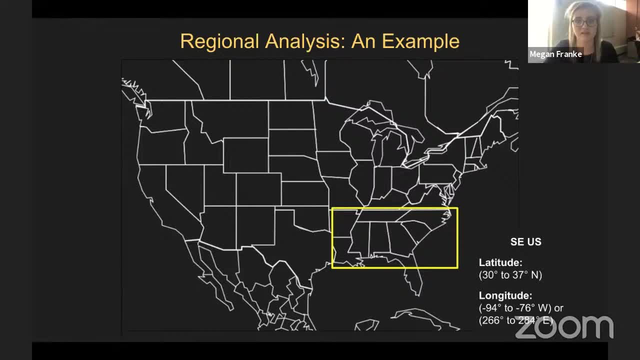 To illustrate the result and change in tissuelated region, we have to Act presuplex relationship between Cape SO6 and SSTs for that region alone. Moreover, as I pointed out in my previous slides, this area is one of the largest variabilities in future Cape SO6 simulations. 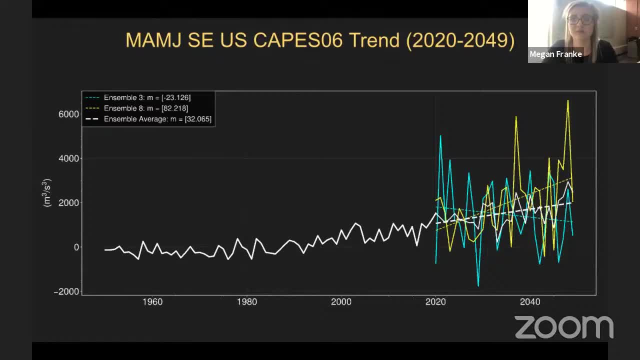 Before we dive into any of the SST relationships, this time series depicts the March through June ensemble mean of Cape SO6 trends in white, as well as the individual members three and eight which show different trends through 2049 over this region. Specifically, while it is clear that, although the large year-to-year variability is present, 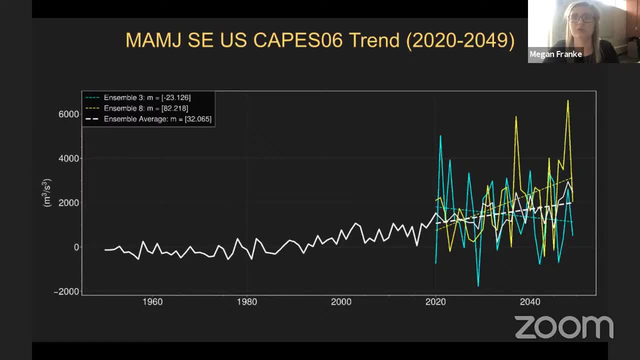 in both ensemble members. ensemble member three, which is shown in blue, is projected to have an overall negative trend and thus a decrease in Cape SO6 over the next 30 years, while ensemble member eight, in yellow, is projected to have a positive trend and thus increase in Cape SO6. 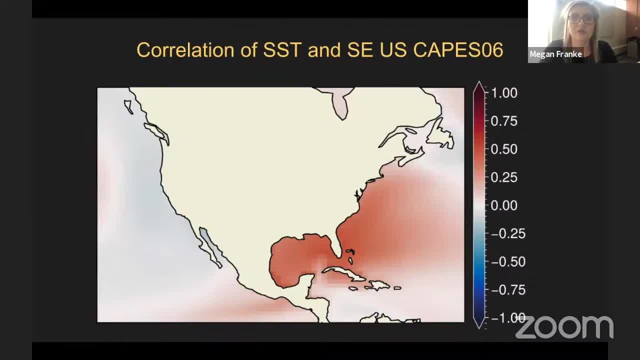 The correlation between Cape SO6 over the southeast-west and local sea surface temperatures shown here indicates that there does appear to be a relationship with year-to-year and longer-term changes in SSTs, especially over the Gulf of Mexico. Although the maximum correlation values in the Gulf are roughly 0.6,, the spatial pattern is still. 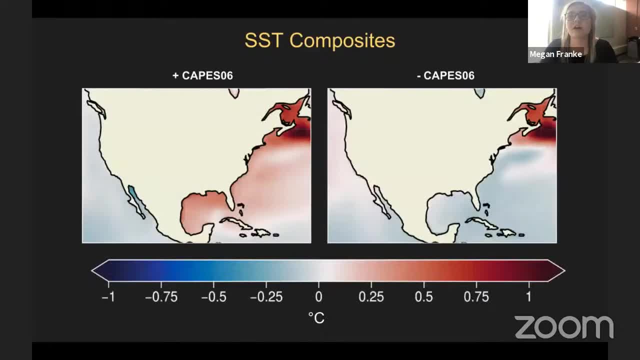 very coherent. To further evaluate the relationship between SST and southeast-US Cape SO6, we computed a composite analysis for those years in which the absolute magnitude of Cape SO6 exceeded one standard deviation. The results confirmed that the years when the model stimulates an 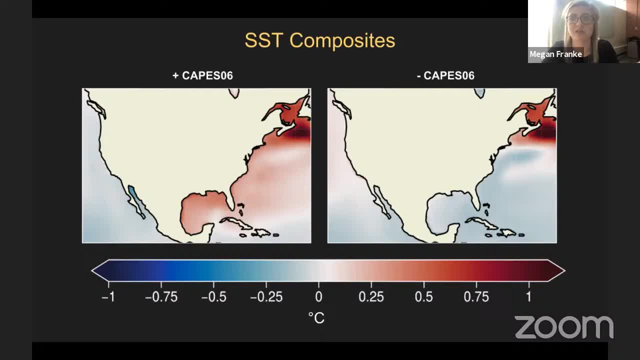 increase in Cape SO6 correlates with the absolute magnitude of Cape SO6.. In the case of Cape SO6, the average sea surface temperatures in the Gulf correspond to years of above-average sea surface temperatures over the Gulf of Mexico. On the other hand, when the model simulated 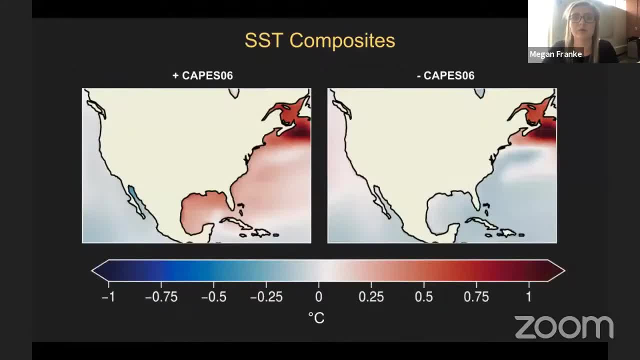 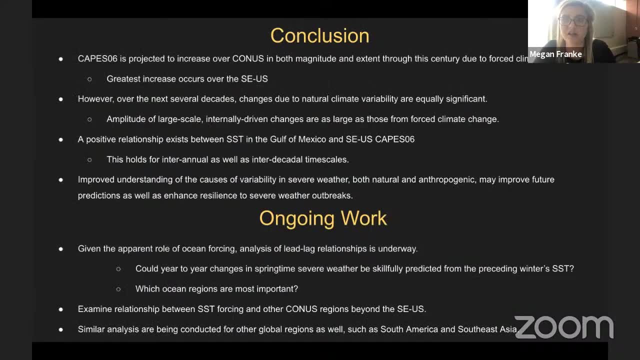 decreases in Cape SO6, there were below-average sea surface temperatures in the Gulf. To conclude, we have shown that Cape SO6 is projected to increase over the United States in both magnitude and extent through the century due to forced climate change, with the greatest increase expected over the southeast US. However, over the next several. 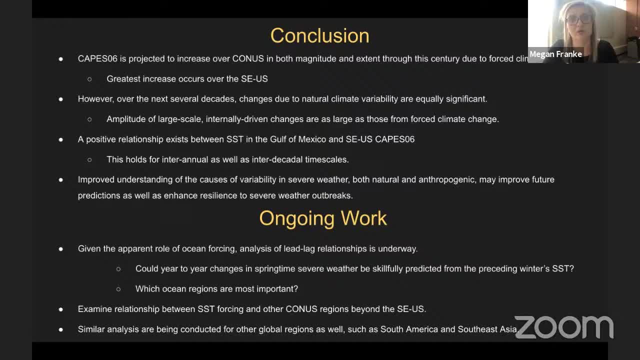 decades. changes due to natural climate variability are equally notable. We also indicated that positive relationships exist between sea surface temperatures in the Gulf of Mexico and southeast-US Cape SO6.. Overall, improved understanding of the causes of variability in severe weather, both natural and anthropogenic, may improve future predictions. 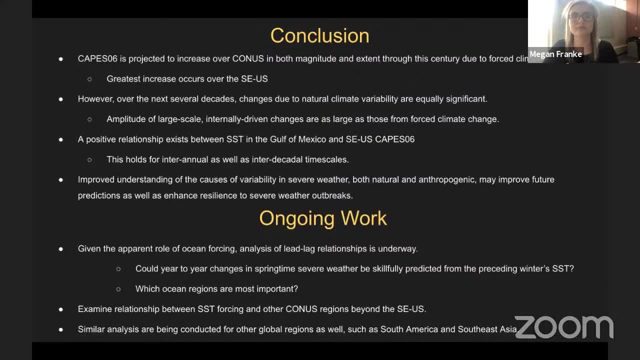 as well as enhance resilience to severe weather outbreaks. Now I know that I am approaching my time limit, so with that I will go ahead and conclude my presentation and take the remaining few minutes for any questions or comments that you might have. Thank you. 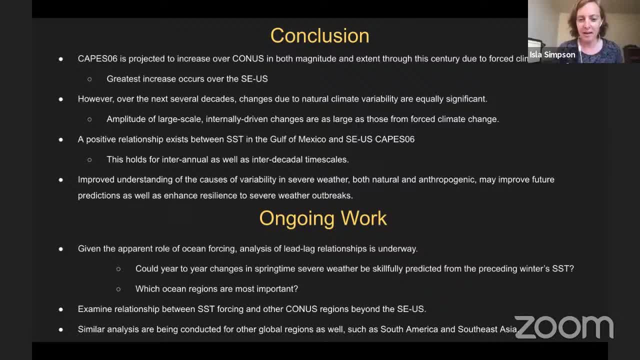 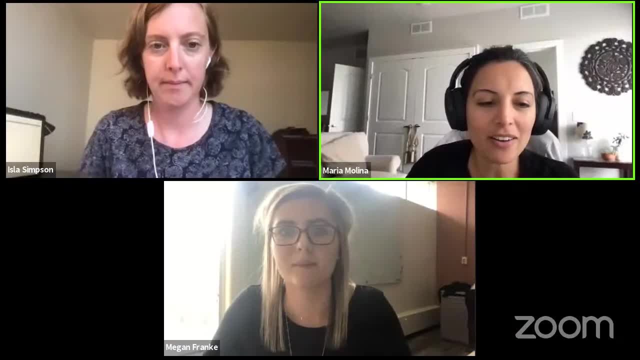 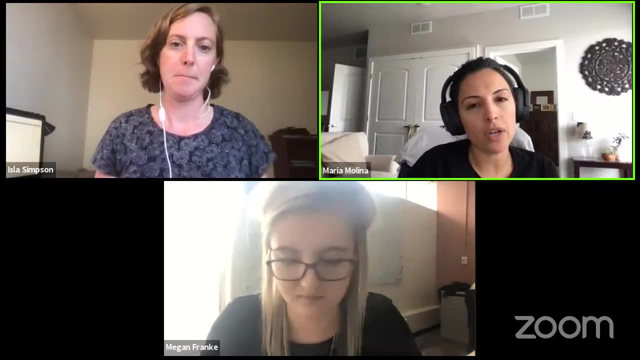 Thank you again for your time and attention. Thanks, Maria. Hello, great talk. Thanks, Yeah, really interesting topic. I was curious. I know you mentioned you didn't have a lot of time and so you omitted some analyses, but when you shared a lot of results for Cape. 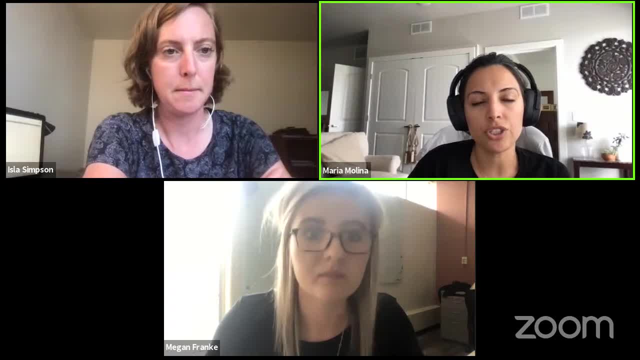 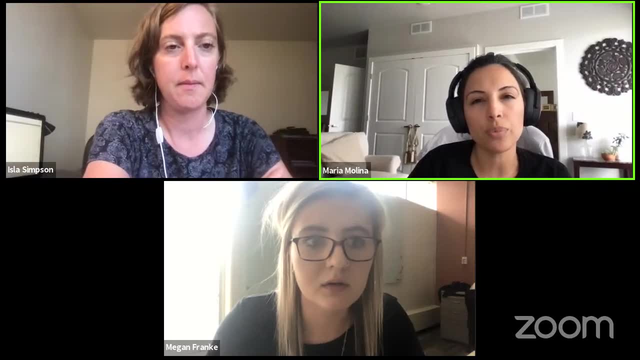 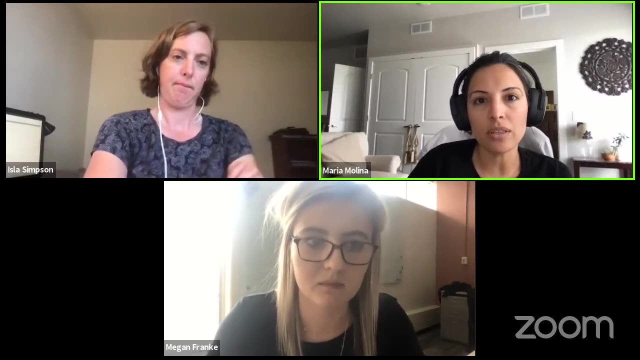 the product of Cape and zero to six bulk layer shear. I think it was Yeah. And yeah I was wondering about: did you see any differing trends between those two different parameters? Because there's always that debate about if we know that Cape is increasing. that's a pretty robust signal. but then the question: 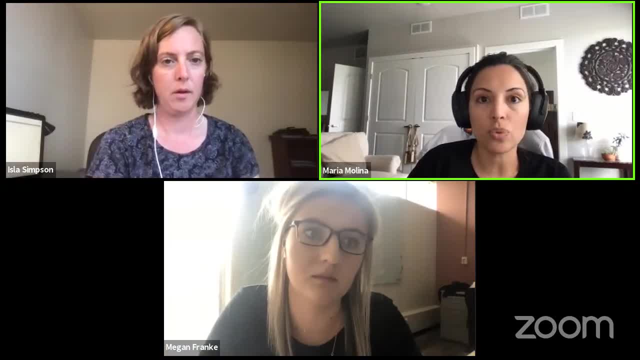 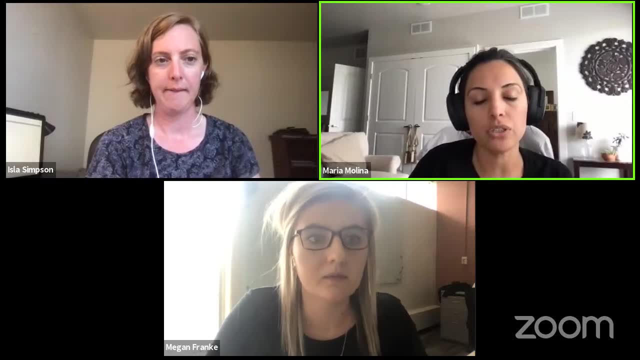 that follows is that there's less confidence in the shear, and that's so relevant for severe thunderstorms. So that's my first question. I have too, But yeah. so I was wondering if you saw differing trends in Cape versus shear. Yeah, we did, As I showed in the beginning of the pre-apartheid. 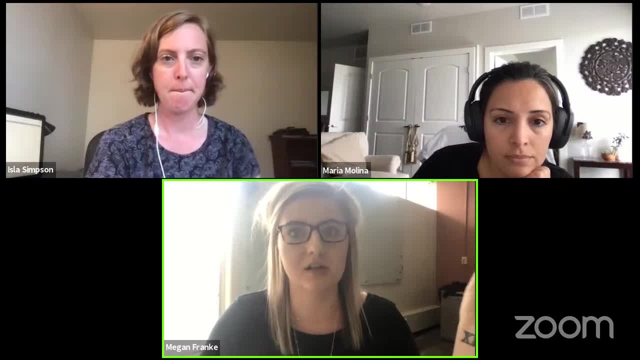 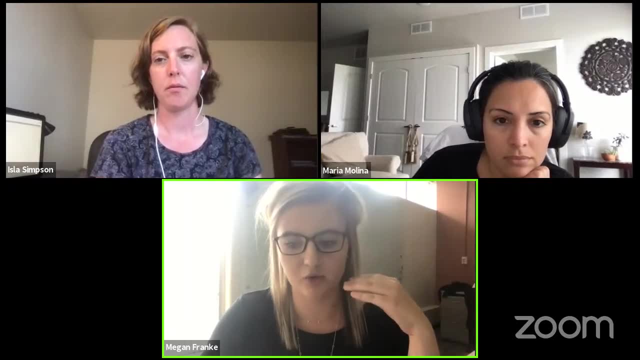 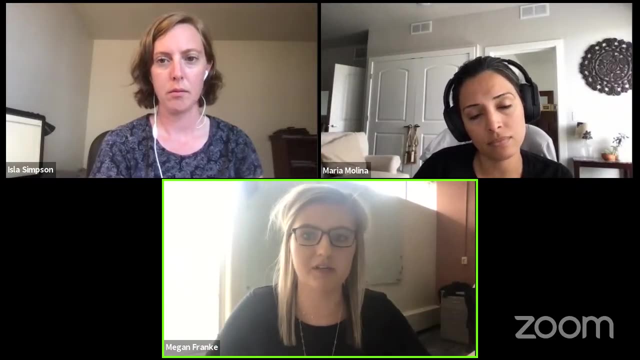 presentation, The Cape. we definitely saw a positive trend over the Southeast US Gulf of Mexico region, as I expressed. And then, as far as SO6 goes, the trend was a little bit different. It was definitely a little bit more horizontal. I guess It appeared to be increases all the way. across the continental US and then a little bit more of a decrease below, over the Gulf of Mexico, Texas region and across those latitudes. But we are looking at both of those individually And overall. when you look at the product of Cape SO6, it does appear that Cape is the main. 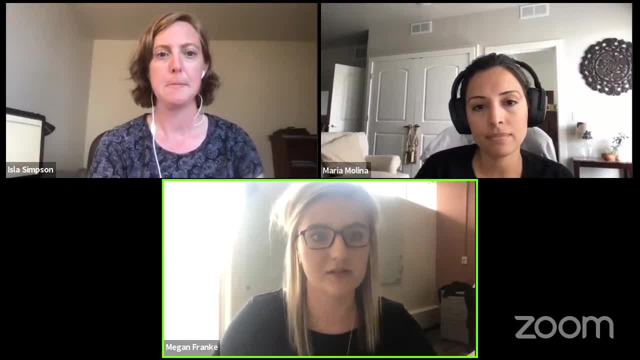 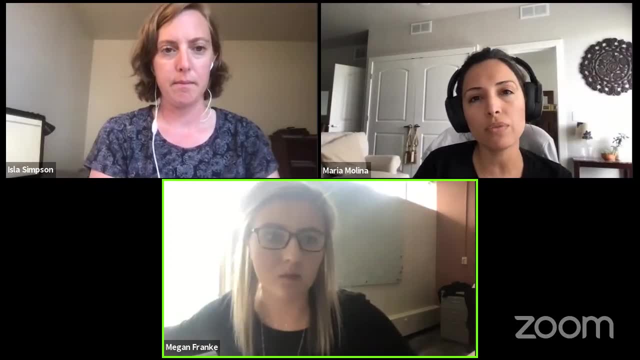 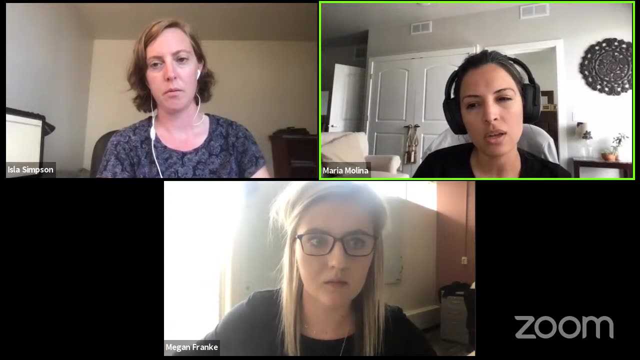 parameter driving the changes between the product of Cape SO6.. That makes sense. And then just a question slash, maybe, suggestion. I was wondering about the motivation for the analysis over water for severe thunderstorms. I think you showed some of those correlations And also. 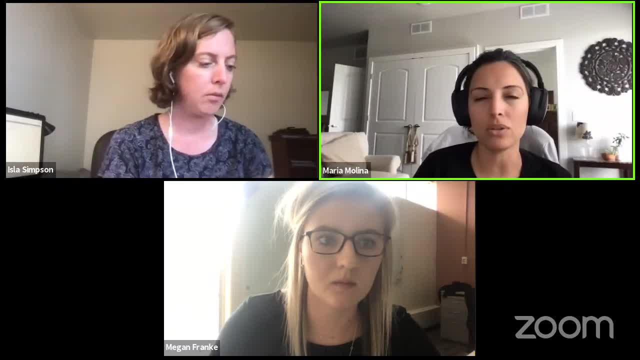 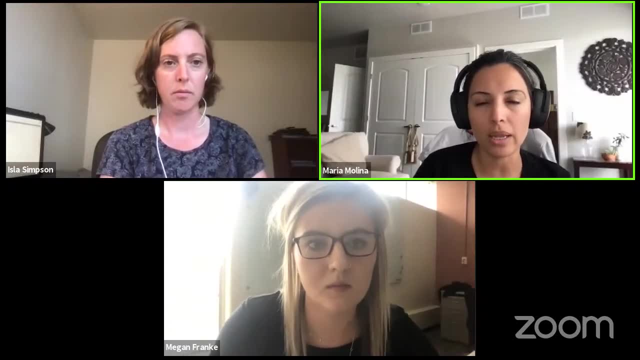 the environmental results, And I guess my suggestion would be maybe to limit it to land, just because, as those environments are affected, over land, they'll be modified and they're blowing out your color bar, your color range, So we can't see the land, But yeah, just. 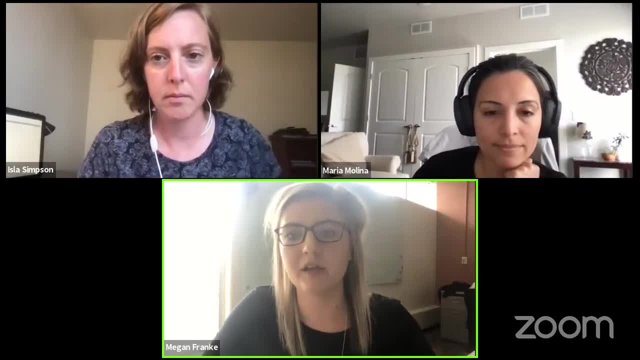 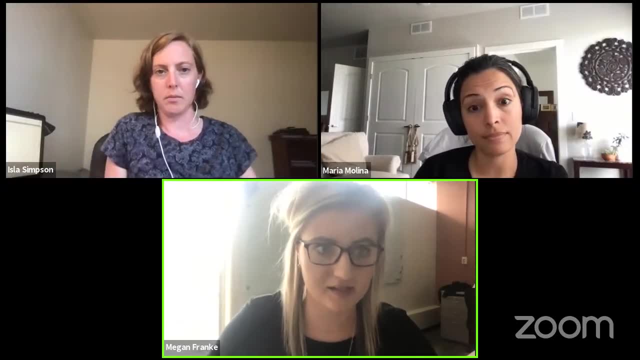 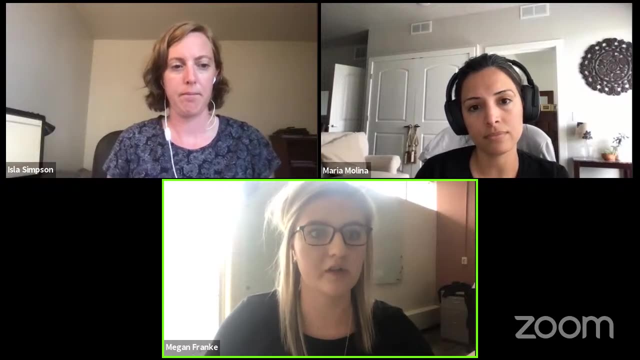 question about motivation. Right, I mean I think I don't think we were really trying to- maybe I misspoke- but we weren't really analyzing any of the severe storms over the water. We were mostly just using the sea. We were just using the surface temperatures to correlate them with the storms over this. 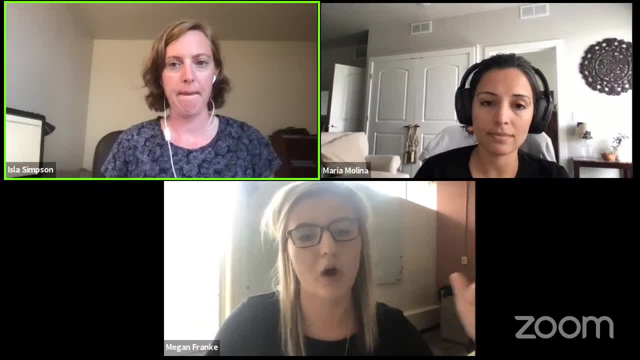 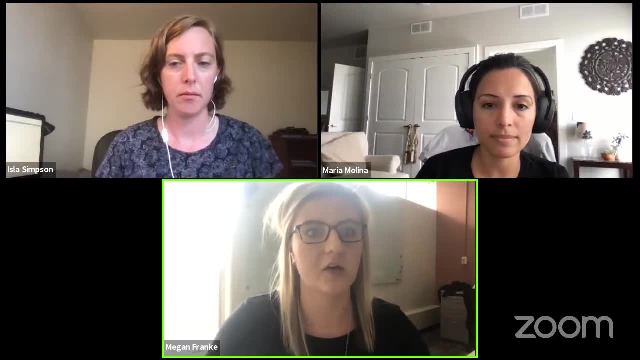 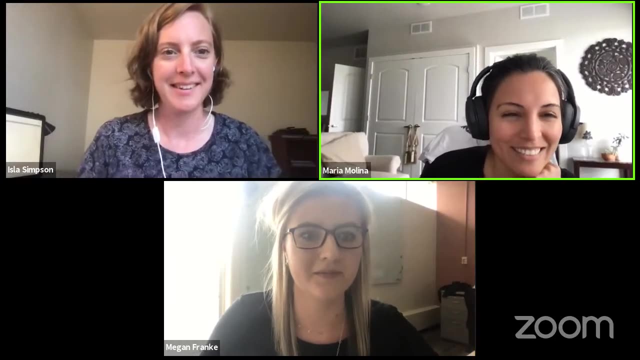 southeast US. So any of the the water that was included in that analysis in that southeast US region was masked, So I didn't actually include it in the correlations of SSTs and Cape SO6.. Thank you, Yeah, sorry for taking over. Oh, that's all right. You have another question. 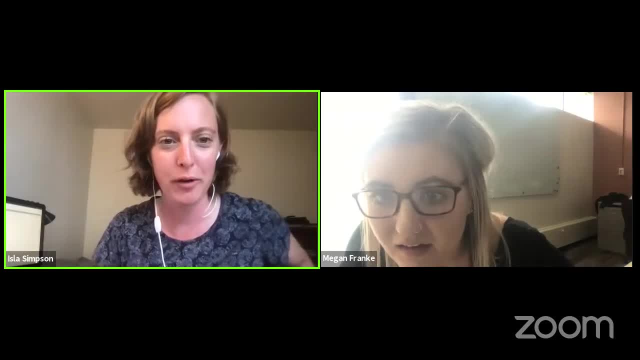 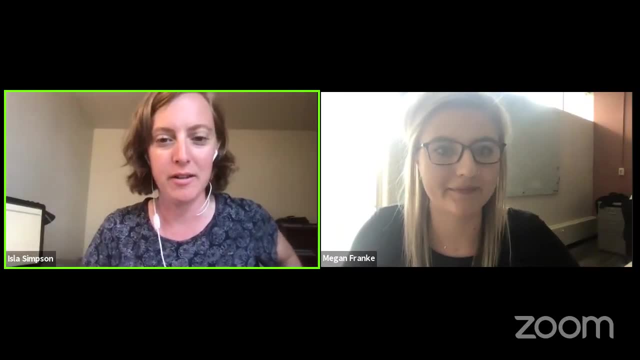 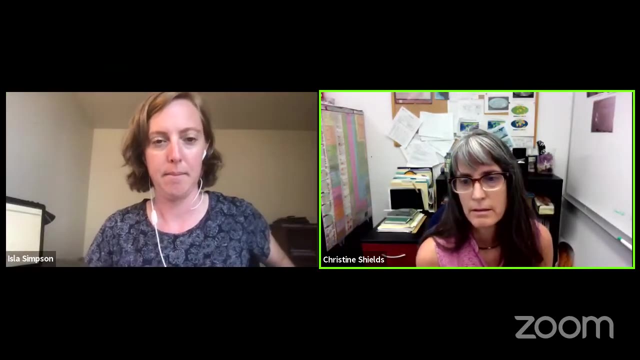 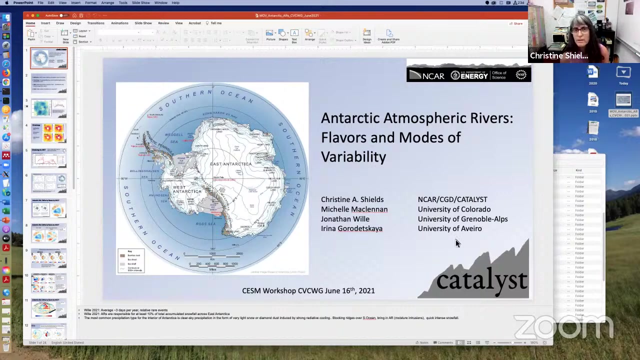 in the chat, so maybe you can just answer. answer that there and we'll move on to the next Speaker. So next speaker is Christine Shields telling us about atmospheric rivers in Antarctica. OK, so let me share my screen To start full presentation mode. 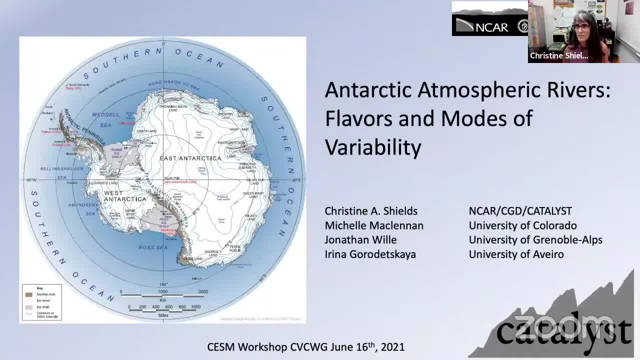 So is everyone seeing everything? OK, It's not full screen at this point. Oh, really, I see your whole screen. Oh, now it is OK. good, I guess it's just a second. OK, so now for something totally different. I'm going to transport everyone into the cool high. 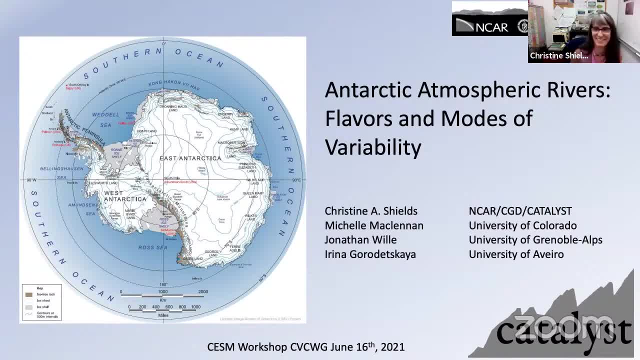 latitudes for those of us who are suffering in heat right now. So I'm going to talk about Antarctica and atmospheric rivers and a little bit about flavor, the different flavors of modes of variability. This presentation is in collaboration with a number of people: Michelle, 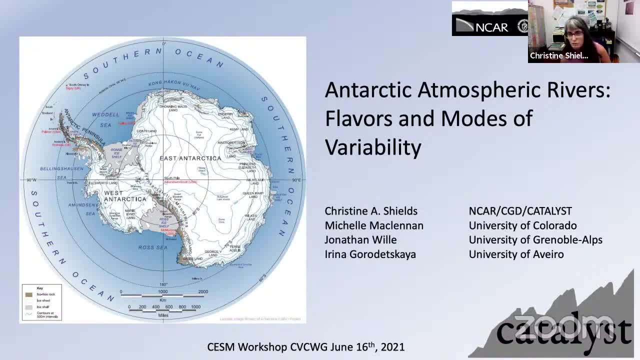 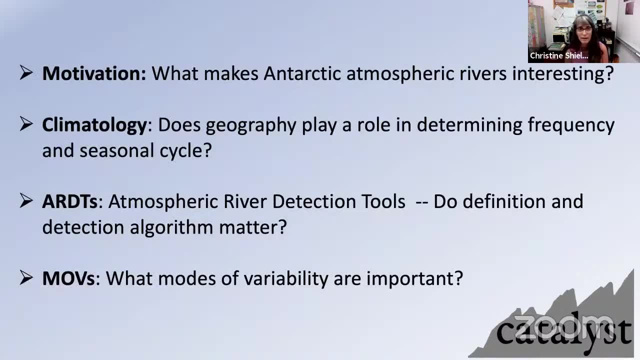 MacLennan at University of Colorado, Jonathan Weil University of Chernobyl and Irina Gordetskaya at University of Aveiro. OK, so just just a quick outline. First, I'm going to try to motivate you and tell you why Antarctic atmospheric rivers are so interesting. show you a little. 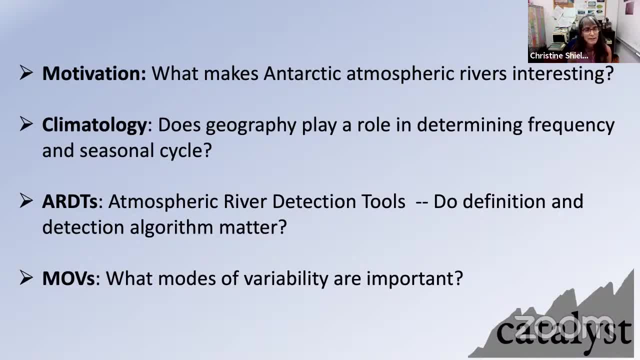 bit about the climatology of the region and we'll spend a little bit of time on atmospheric river detection tools, because this actually is quite important, especially for climate control in regional areas such as Antarctica- that the definition of how we define an atmospheric 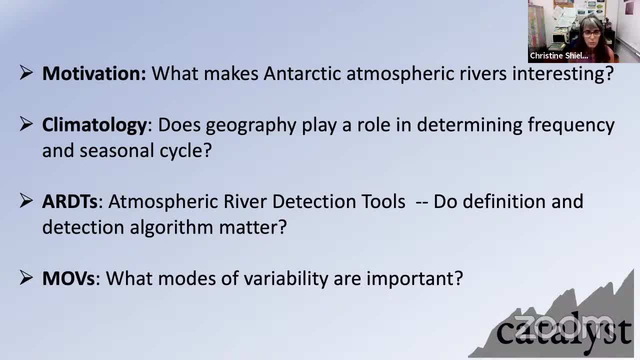 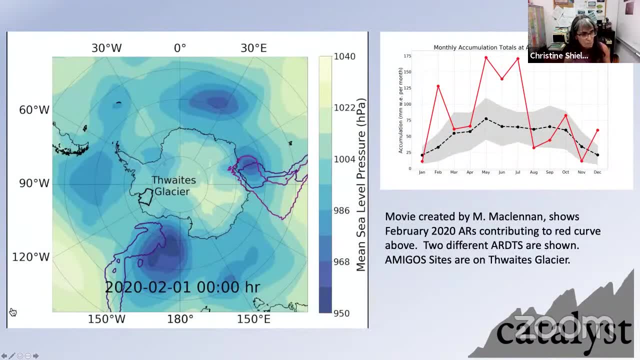 river matters And then finally just sort of launch into some of the results I've seen with different modes of variability and what's important for different regions of Antarctica. All right, so this is a nice little movie that Michelle put together. It shows atmospheric 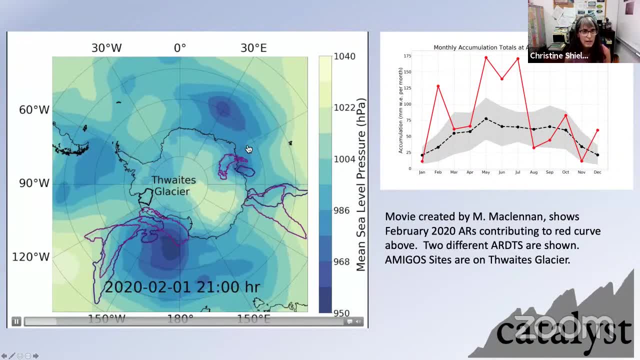 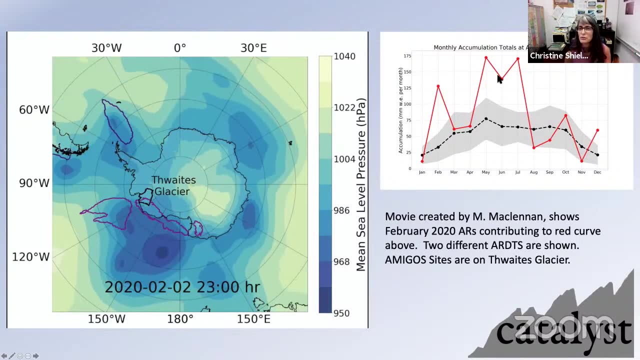 rivers making landfall over Antarctica. I've highlighted Powaites Glacier over here because I'm going to sort of transport you over here While that movie is going to this figure that shows snow accumulation totals over Powaites Glacier for the mean period of the ERA 5, which was 1979 to 2018.. And then what happened? 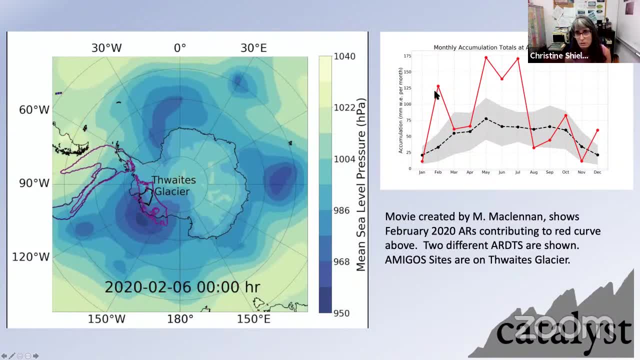 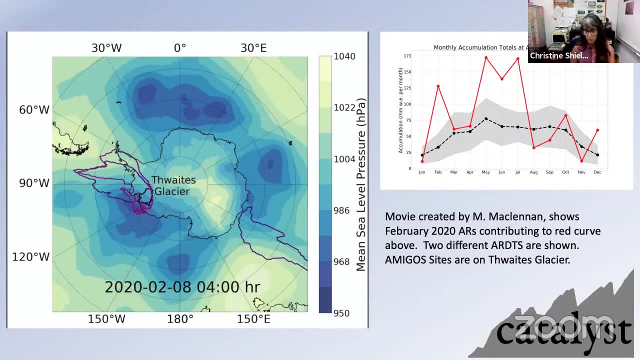 in 2020. last year we had three major atmospheric rivers making landfall over Powaites- one in February, one in May, one in July- And these were massive events that you could see. compared to them, The mean Really did increase, boost the snow accumulation totals at those regions. So hopefully this 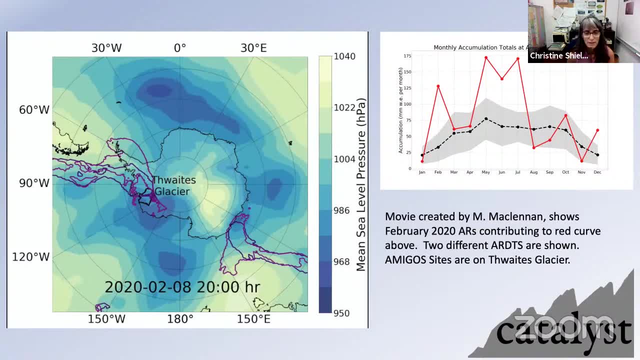 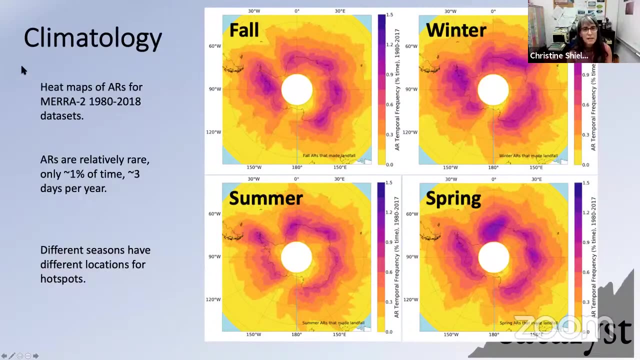 will help to convince you that atmospheric rivers over Antarctica actually are quite important. Trying to advance here, Okay, there we go. All right, so a little bit about the climatology. Here is some heat maps I call where we're looking at like the density of the ARs. So 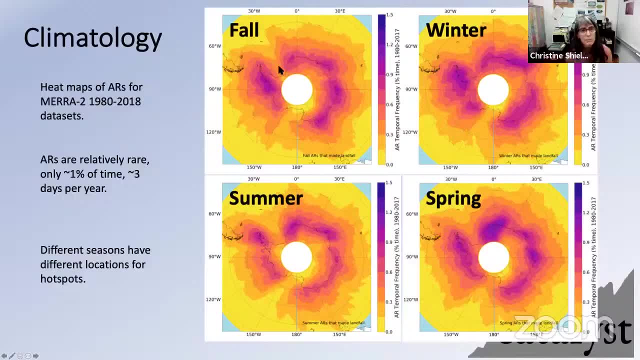 these are the density of the ARs as they've been detected, divided by season: fall, winter, spring and summer. If you notice the, the color bar and the actual range, the atmospheric rivers that make landfall over Antarctica are actually relatively rare events. we have, on average, three days of atmospheric 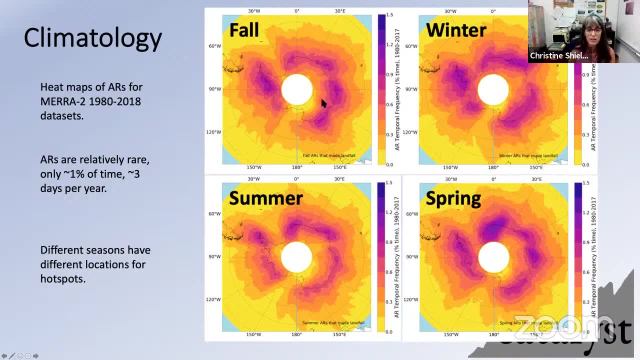 activity over Antarctica. So they're relatively rare events, But when they do occur they're actually quite impactful. And the other thing to sort of take away from this plot is: there's a lot of activity over Antarctica. You can see on the slide. there's actually three different events that are happening. 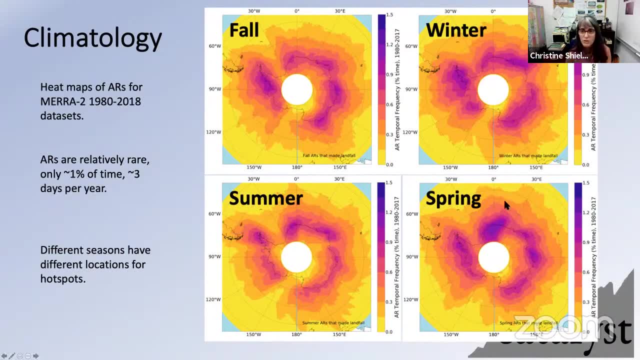 And the other thing to sort of take away from this plot is: you know, the amount of activity is that for the different seasons- fall, winter, spring and summer- you see different hotspots. So those deeper purple colors are changed, shipped, depending on what the season is. 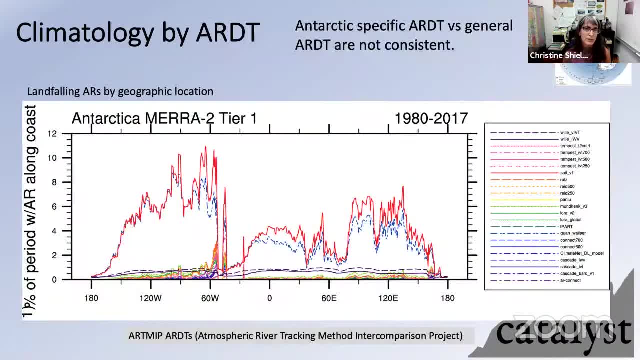 And this is actually quite important when we start looking at modes of variability. All right, So on to a little bit about what this geographical distribution looks like. here I'm actually plotting a whole bunch of different ARDTs. These are Atmosphere River Detection Tools from the Atmosphere River Tracking Method Intercomparison Project. 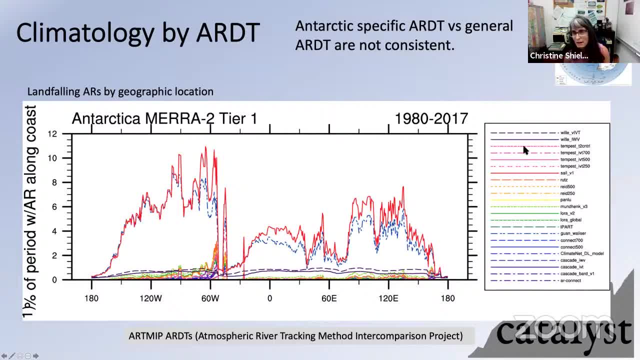 So there are quite a few different ones to look at. All these colors mostly are ones that are global and are general detection algorithms, And I have these darker purple ones, the YL-IWB and YL-VIBT. These are regional, specific and specific to Antarctica. 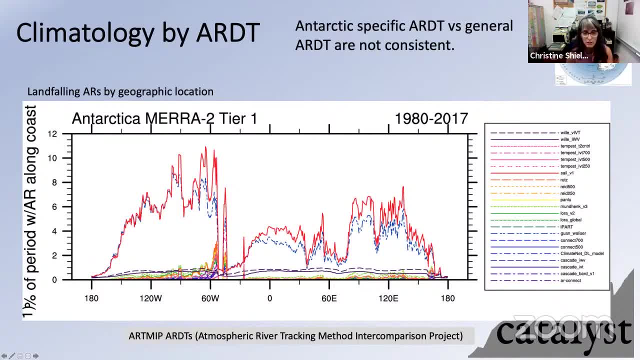 And so just by looking at this, as you can see, there's actually quite a dramatic difference between the two. So what does that mean? What a regional algorithm will tell you and what a global algorithm will tell you? And just for your perspective, here's Antarctica, over here, where this is zero. 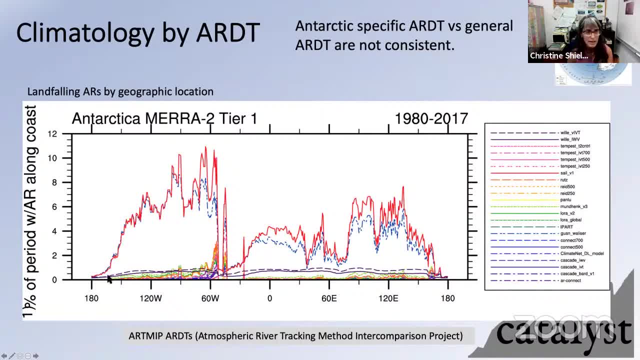 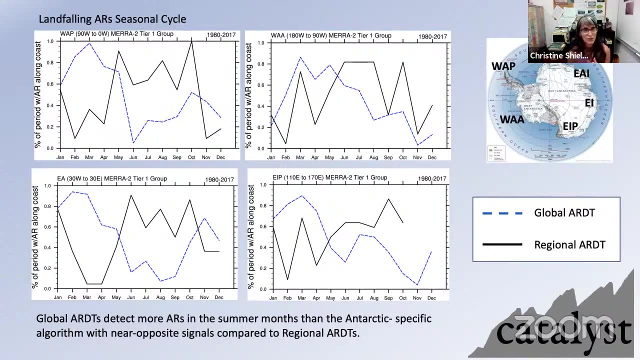 And we're actually looking at 180, around the horn to 180.. The only place where there's agreement across all the algorithms is actually the minimum, which is this frosty area. So sort of making this a little bit more digestible and understandable. 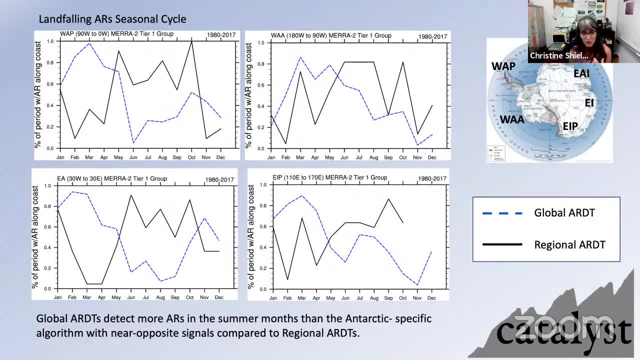 I've actually grouped all those together. So this is the global ARDTs compared to regional ARDTs, And now we're looking at specific regions around Antarctica in terms of the seasonal cycle. Here is again my little cheat sheet map of Antarctica. 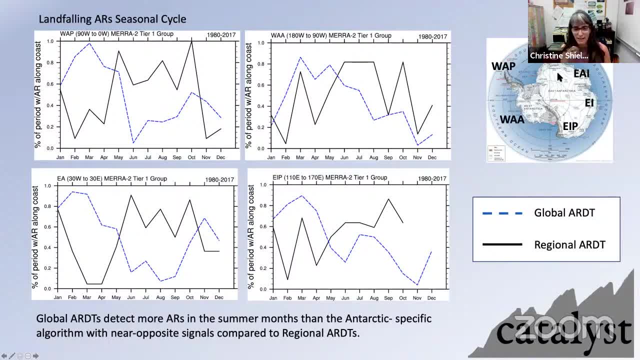 Instead of using the Antarctic land names and stuff, I've actually used the ocean that it backs into as a reference, because for me this is understandable. So apologies to all those Antarctic ice sheet people. So EA would just be the East Antarctica that backs into the Atlantic. 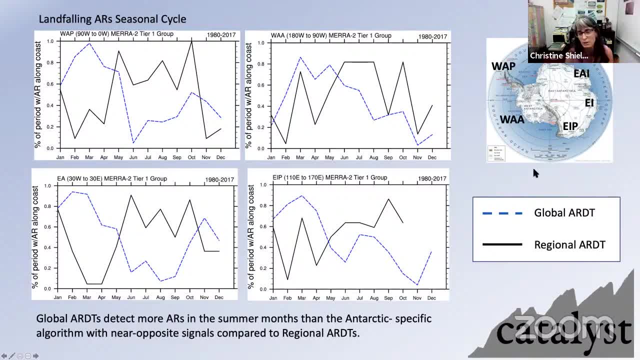 AI would be Atlantic India and so on and so forth. WAP is just essentially- I'm looking at this West Antarctic Peninsula area And WAA is just backing into this Edmonton Sea area. So I've done these for all these different regions, but I'm only sort of highlighting a few here. 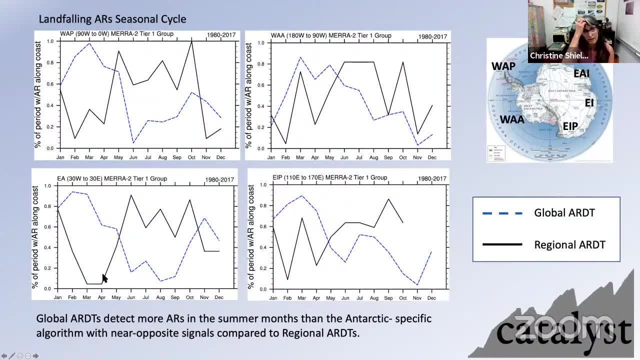 The West Antarctic Peninsula and the Edmonton Sea area versus a couple of the East Antarctic ones. And the couple of things to pull out of this is that you can see, especially for the WAP and the EA, it's absolutely opposite with the global zoo versus what the regionals do. 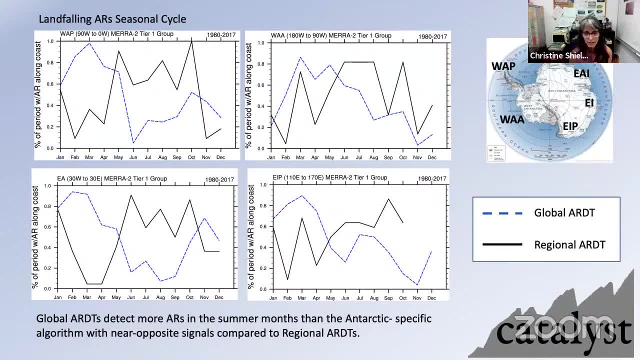 And the regional ones are a little bit more closer in line to what we might do if we were going to hand detect atmospheric rivers over Antarctica. So I personally view these, the regional ones, as a little bit more accurate than the global ones, And I can sort of explain that and what the global ones are doing and sort of picking up 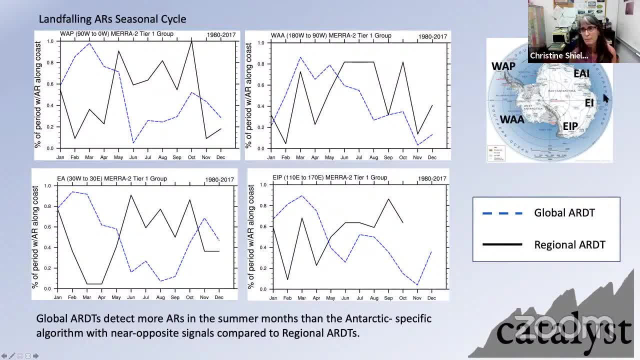 you know, basically the Southern Ocean storm track as opposed to atmospheric rivers that are actually extending into the continent. And then the other thing to sort of pull away: these globals tend to actually over detect ARs in the summer, for the reasons I just mentioned. 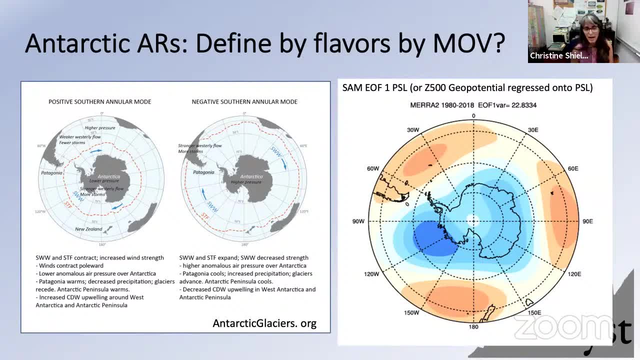 All right. So now I sort of wanted to spend the rest of my time sort of talking about modes of variability And just for the record I guess I should say I'm focused on these regional ARDTs. So I'm using the IWB and the VIBT from the wild Antarctic specific because I feel like that ARDT is superior for this type of analysis. 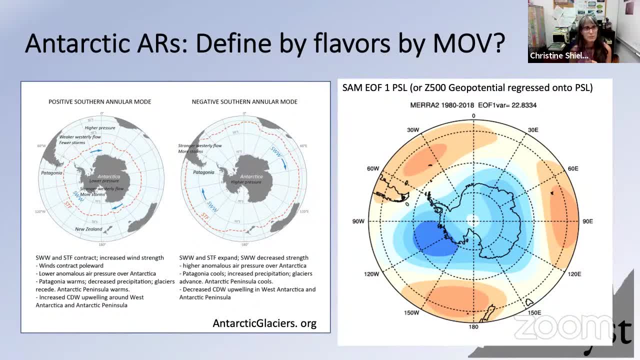 So so now on to the modes of variability. Clearly, the big one is the SAM. I don't really have to, I think, explain it to this group Here, So this is just sort of a nice little graphic I pulled pulled off to show what the SIP of the SAM is. 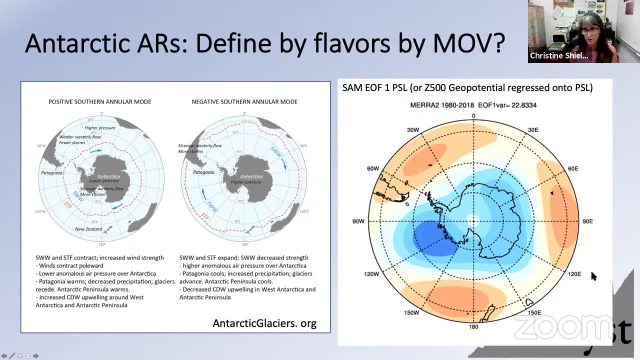 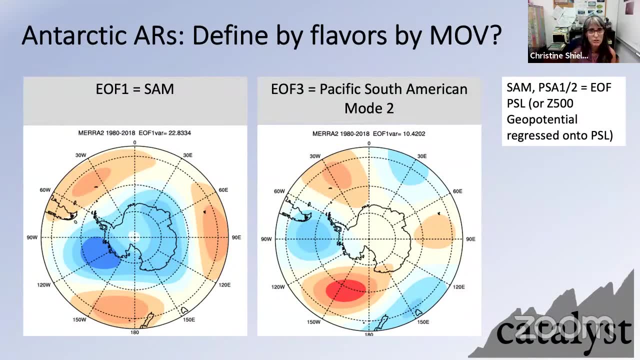 which is essentially the first EOF of sea level, of sea level pressure. Here's the spatial pattern. I'm actually going to also look at the different EOFs of sea level pressure, extending into EOF 1, 2 and 3.. It turns out that EOF 3 actually has some significance for this WAA area, where 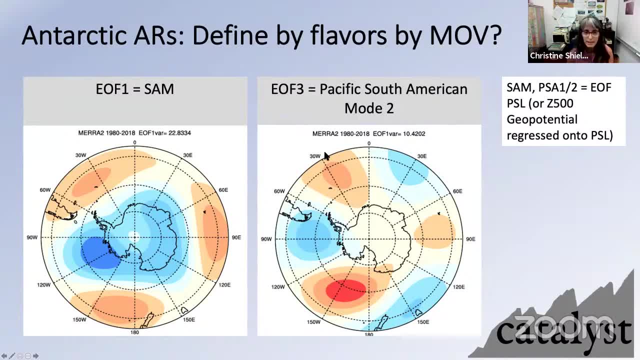 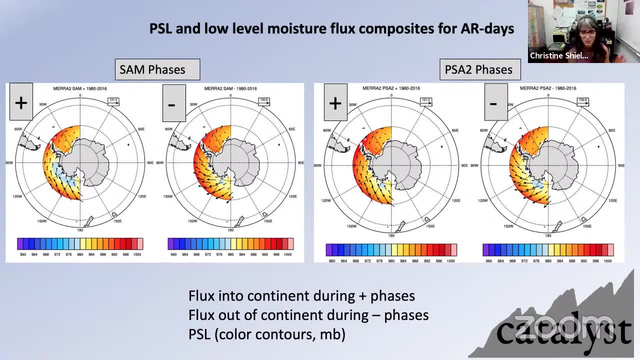 especially Ripley's Glacier. So I sort of also want to include that in what I show you next And also we'll give you the caveat- because of this, the time limitation- Sorry, trying to keep track of my timer- that I'm going to only just show you some results on West Antarctica. 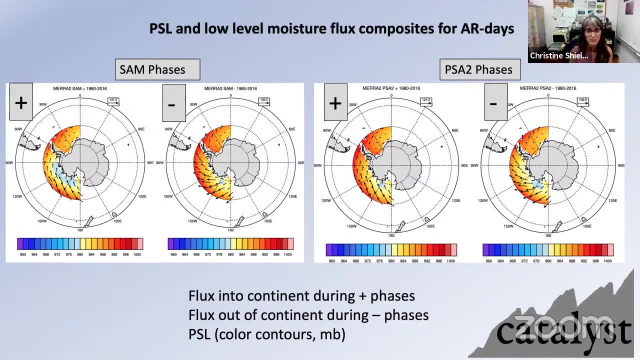 I do have them for East Antarctica but, and so I'm happy to talk to people about that later, But for now just sort of show you just some highlights from the West Antarctic piece. So this is looking at the SAM and the PSA2 phases. 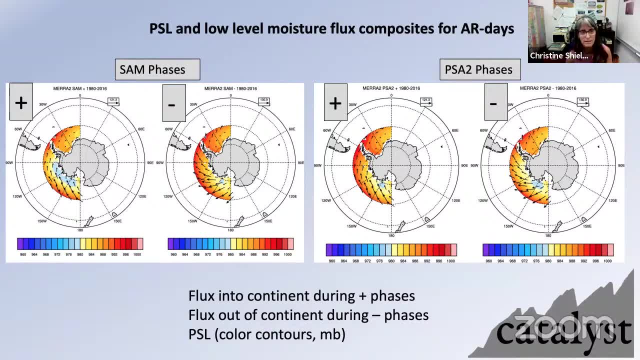 For positive phase and negative phase, And we're looking at the sea level pressure, which is the color contour, And then the vector arrows are the is the moisture, the low level moisture flux. So this is, this is UV and incorporated into reciprocal water. 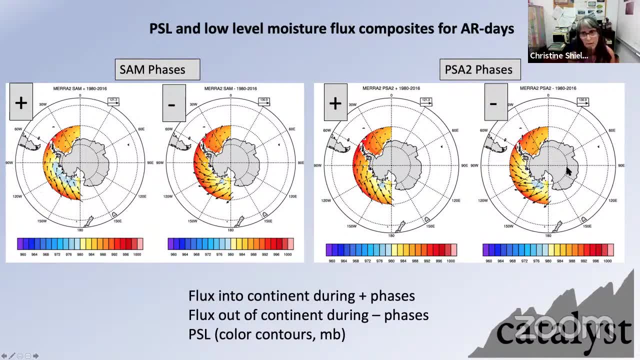 And you can see for both, for the positive phases, for both SAM and PSA2, you see this flux of moisture into this West Antarctic piece, So this is favorable for us. And for the negative phases, you see this outflow from the continent out into the oceans. 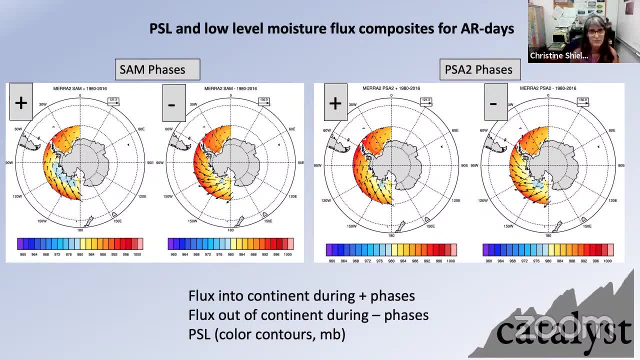 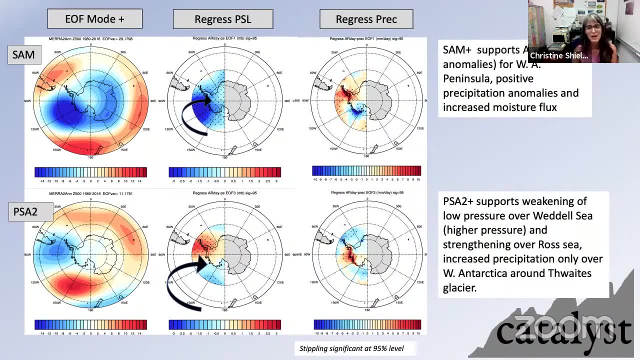 which is not supportive of atmospheric river activity. So this is sort of just like to give you some background. Two minutes, OK, thanks, And so so I guess we'll just jump to sort of the these different modes of variability regressed onto. 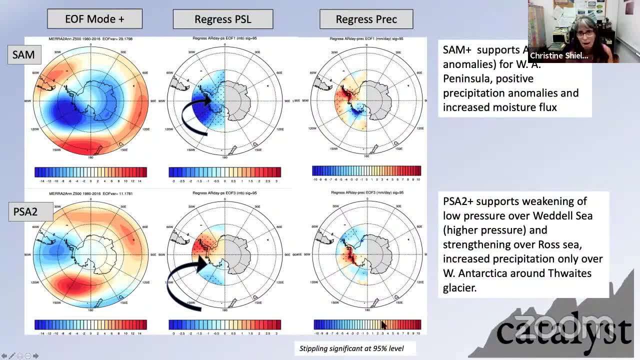 I did both a number of variables, but we'll just sort of highlight here The precipitation, because in this is precipitation attributable to AR. So now I'm only looking at AR days where it precipitates. So you can see there is for the SAM, positive phase. you have this, you know- lower pressures. 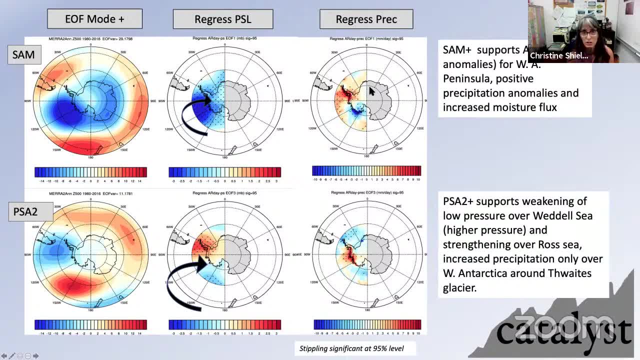 And it's positively correlated with precipitation in the Swiss Antarctica piece and negatively correlated closer to the Ross, the Ross Sea area For PSA2, you have these positive precipitation correlations In this WAA section of West Antarctica which is where Thwaites Glacier resides. 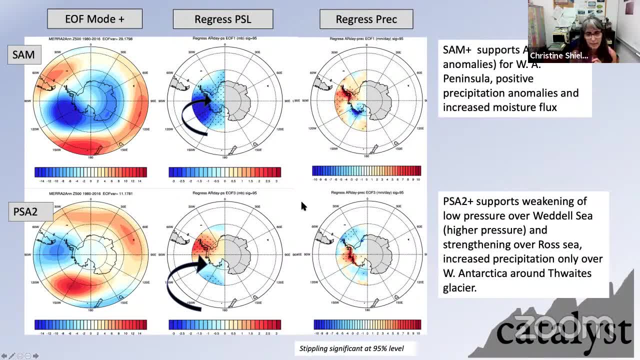 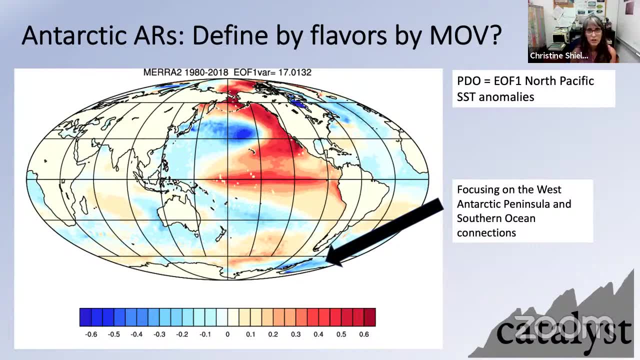 So these are in there and the dotted stippling that implies significance for these regressions. All right, So the last little bit here. I sort of started looking at the PDO, which is the first UF of SST anomalies, But instead of the typical thing of looking at over the western US, 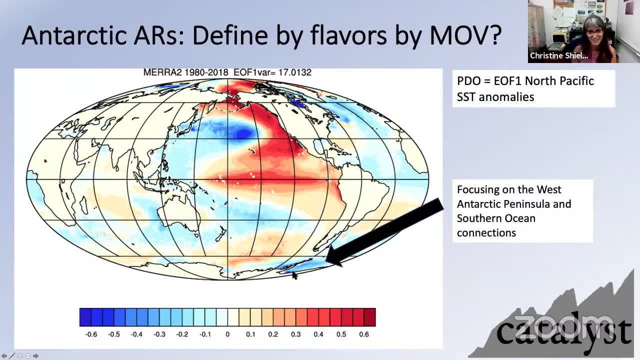 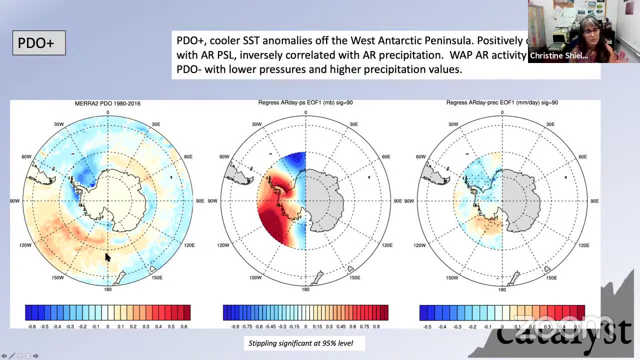 I'm actually going to draw your attention here to West Antarctica because there is some correlations with West Antarctica. So for this is the spatial pattern for P. for the PDO positive. Sorry, You know, this was sort of a quick plot. So we have negative SST anomalies here. for the PDO positive: 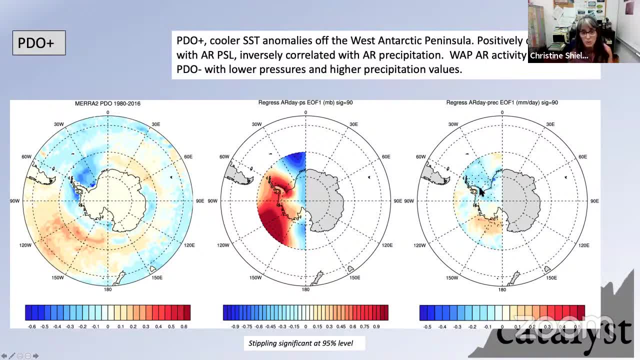 which correlates to negative correlations with precipitation over the West Antarctic piece here. So if you flip that, so PDO negative phase would actually be supportive of AR activity in the West Antarctica peninsula and over the West Antarctic ice sheet, And there is literature out there that has just come out that actually supports this. 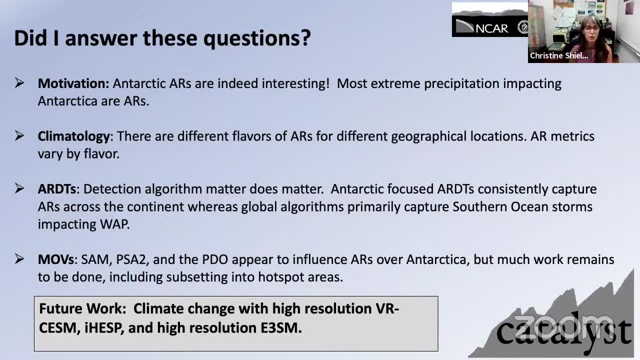 OK, so just quick in summary. hopefully I've convinced you that atmospheric Antarctic, atmospheric rivers are interesting. I certainly think they are. I've showed you a little bit about the climatology and hopefully convinced you that the regional ARDT that I'm using is the most appropriate. 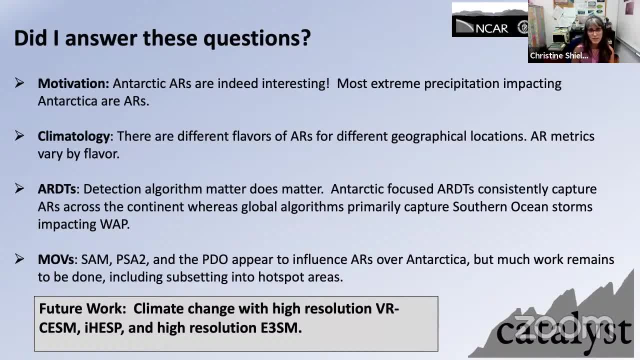 And then we've looked at different modes of variability thus far: SAM, PSA2 and the PDO and their influences over Antarctica. I've done a lot of subsetting and I'm continuing on this work and stuff with East Antarctica. I plan to move forward in this, looking at model resolution and the variable resolution, CSM, that Adam Harrington talked about a little bit earlier. 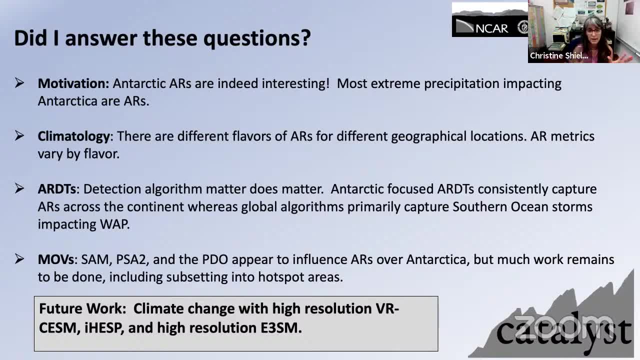 I think a number of other people may have been in the land ice. I'm thinking of the land ice working group, that high resolution piece over Antarctica and other high resolution simulations. So I'll stop there and take questions, Thanks, So there is one question in the chat from Alice. 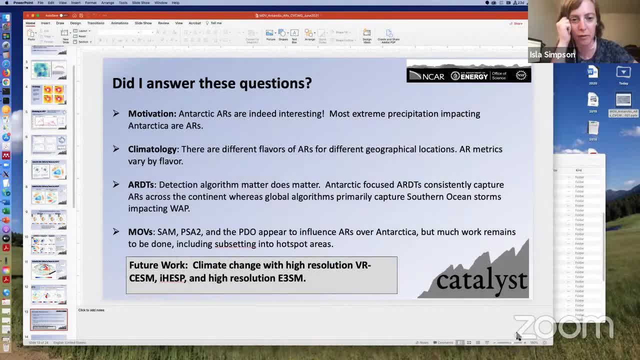 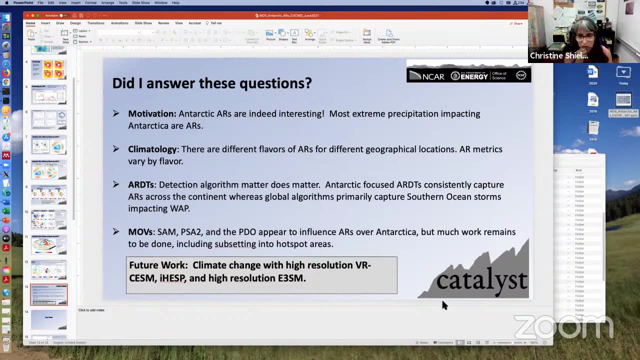 She's wondering how the magnitude of the atmospheric rivers versus frequency differ by season. It looked like more purple colors in winter, but do the is a total snowfall lower in these months. Have you looked at that? Yeah, So this is entirely sort of dependent on what region you're looking at. 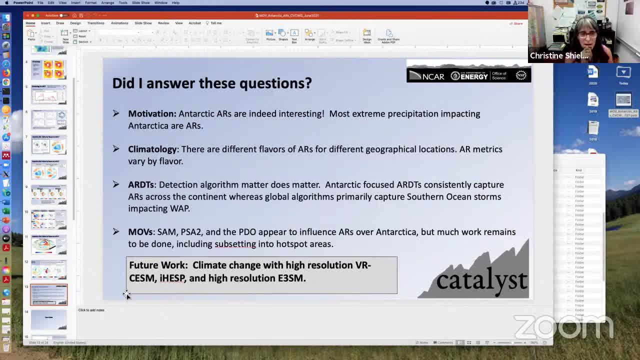 It's not like a one slice fits all sort of a thing. So, Alice, we can sit down and look at different maps and I can show you which pieces are better There's. there's some you know for for the most part, like you know, if it's well, I guess I shouldn't say for the most part- 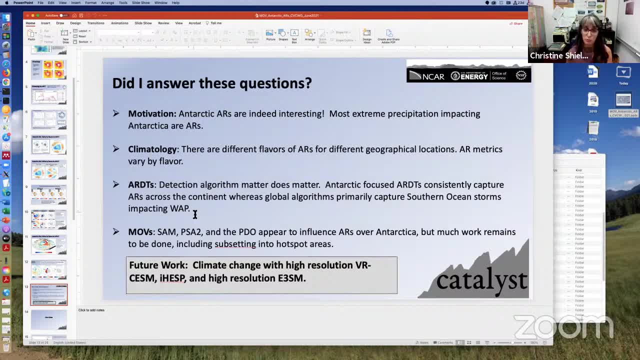 But there is evidence that there's, you know, both atmospheric rivers can contribute to these increases, Snow totals like we saw in Puig's Glacier in that beginning, but also in East Antarctica piece. There's evidence that for you know, say a negative you have- or it's warmer and not necessarily conducive to air activity. 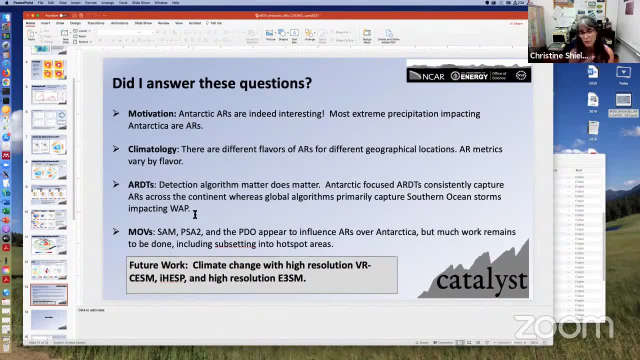 You get these warm air intrusion events would actually cause, And then you get you know something that may result look like an atmospheric river that would cause a melting event, because it's warm air That's doing this rain on snow. Yeah, So yeah, I don't. I'm not sure if that is your question. 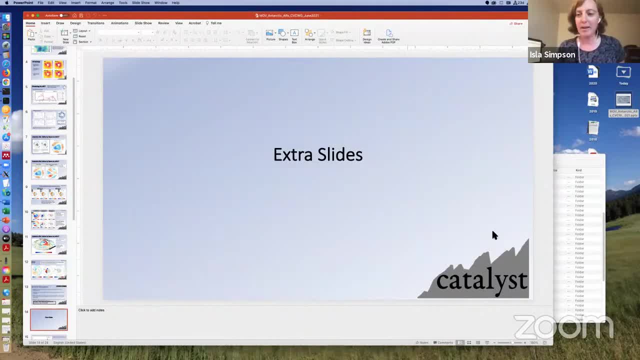 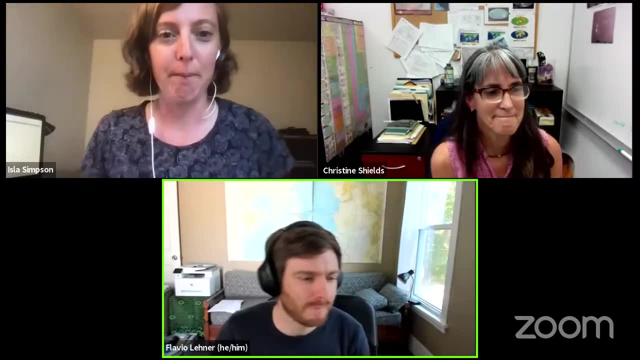 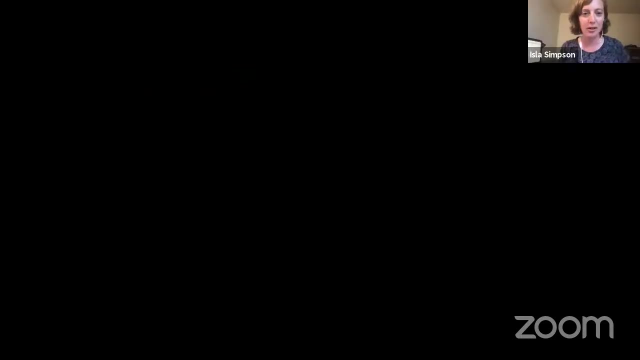 I hope so. OK, I think we probably best move on. Flavio, maybe you can type your question in the chat after you've given your talk. Sure Yep, OK. so next speaker is Flavio talking about the extreme 2020 Siberia temperatures. 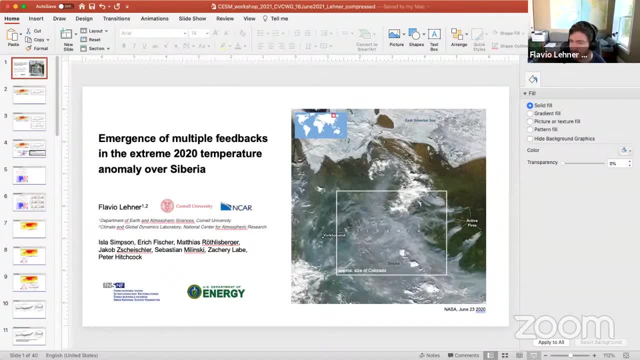 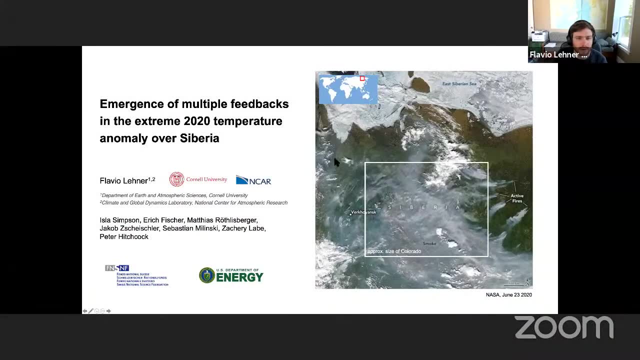 All right, Yeah, Thanks for organizing this nice session. Well, there are an issue. I hope you can see the screen. Yeah, So this is a- it's a bit work in progress with like a sort of a last year's team of people that started with a Twitter discussion last summer when there was this heat wave or sort of persistent temperature anomaly over Siberia that was in the news a little bit. 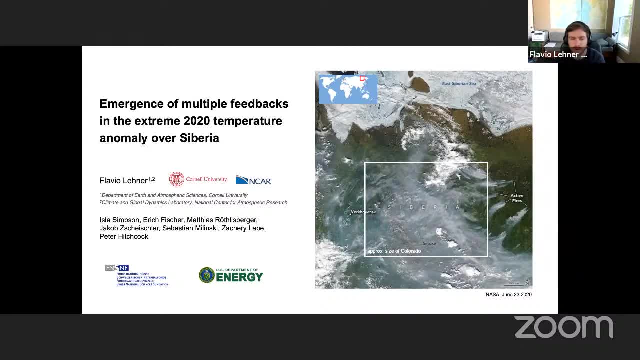 And I'll talk about a few more nuanced aspects In this presentation. the relevance in general was: it was quite interesting in the context that it was just a very strong temperature anomaly, But it's also coincided- not just last year but last year in particular- with widespread fires over Siberia as well as sort of worry about accelerated permafrost melts during these really persistent temperature anomalies. 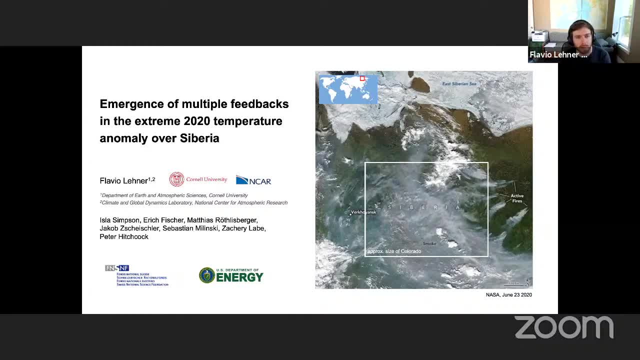 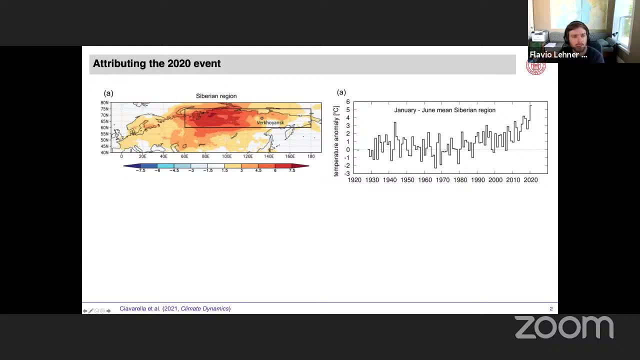 And so we're going to try to look at this a little bit In more detail. A couple of attribution studies have come out with quite quickly, especially focused on the first half of 2020,, which was sort of the one that grabbed the headlines. 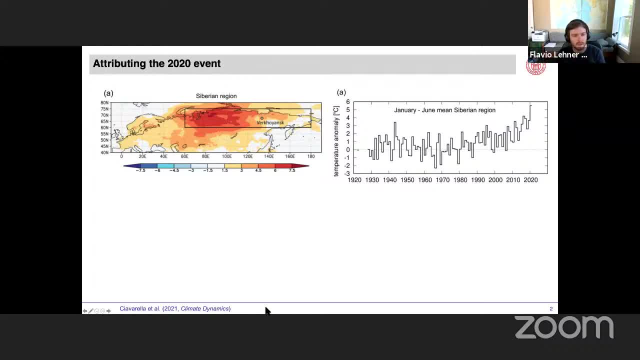 I was involved with one with this world weather attribution team where we looked on the one hand that sort of the half year, So January through June, temperature anomaly over Siberia- You see the map of this plotted here. But then The study also looked at the daily maximum temperature at a particular station which went over 100 degrees Fahrenheit, which was the first time in the Arctic Circle. 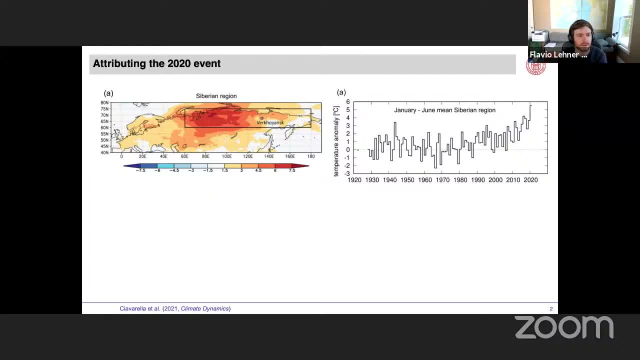 So that really grabbed the headlines but was maybe less interesting, at least from a scientific point of view. Yeah, here's the daily temperature time series. It was just very extreme, but it was an extreme event in general. Also, if you look at sort of the half year average and the attribution study, maybe unsurprisingly- 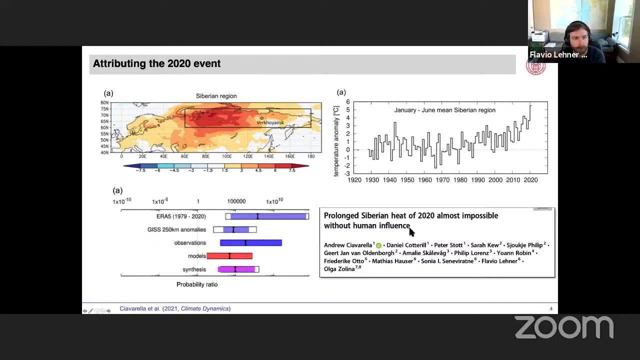 Then concluded that At least this first half year was effectively almost impossible without human influence. This derives from sort of this, Yeah, sort of expansive analysis of observations and different models, large ensembles, to come up with a probability that this event could occur in today's climate, comparing it to pre-industrial climate. And so the probability that this could occur was without climate change was extremely low. That led to this headline of almost impossible. People also looked at sort of the drivers again, in particular of the winter and the spring part of this event. A study by Overland and Wang pointed out that, yeah, the Arctic Oscillation was very positive during the winter 2019, 2020, which was like driven by a strong, very strong polar vortex. 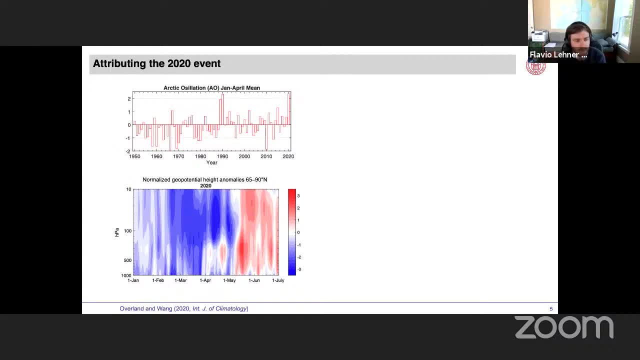 I think even record breaking ozone levels in the Arctic And then sort of a different pattern towards spring and summer. So these are two potential height anomalies. So you're seeing strong negative anomalies aloft in the early part and then more positive anomalies and more closer to the surface. 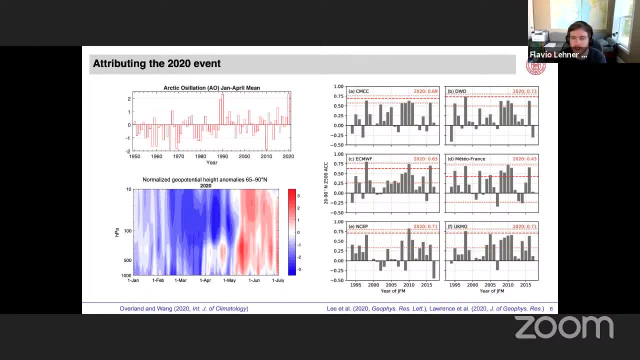 It's also exceptionally well forecasted event. I'm not going into that, But these are six different Sort of seasonal forecasting models And in several of them this event- which is the skill of the forecast is given with this dashed line compared to like sort of a hindcast, was very well among the best forecasted winter sort of- yeah, C500 anomaly correlations. 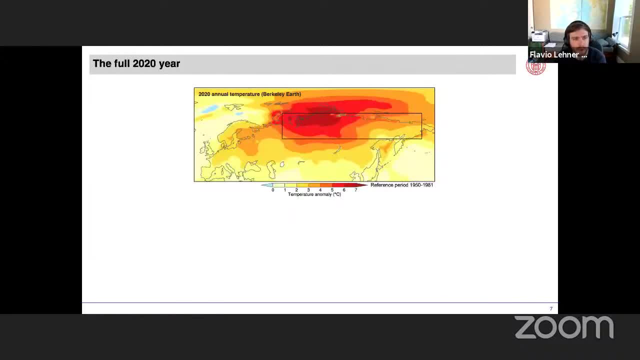 So it was like a strong event and well forecasted. So then there's a little bit of like sort of my personal story. I started looking into that together with a bunch of these people from the attribution group And then I started a new job at Cornell University in fall and really didn't get too much in the beginning. 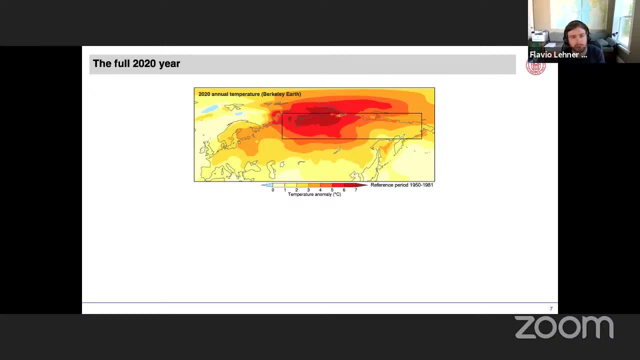 And so the whole year 2020 passed and it turned out that also the second half was relatively extreme. So I decided to pivot a little bit and focus on the whole year and look at what caused this very persistent temperature anomaly over the whole year. 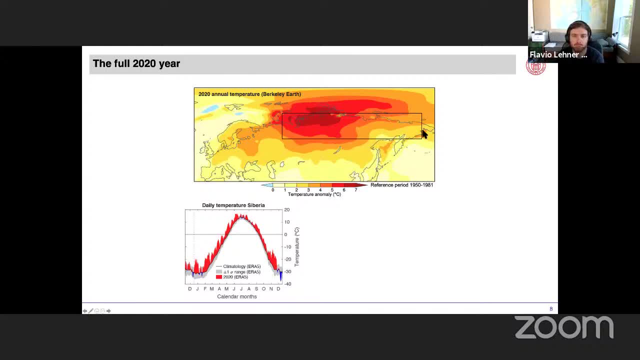 So here are daily temperatures over. This is the same box. I'm just looking at land in this box. The same boxes was used in the earlier attribution study And again you can see that this really compared to a climatology that is 1951 to 1980. 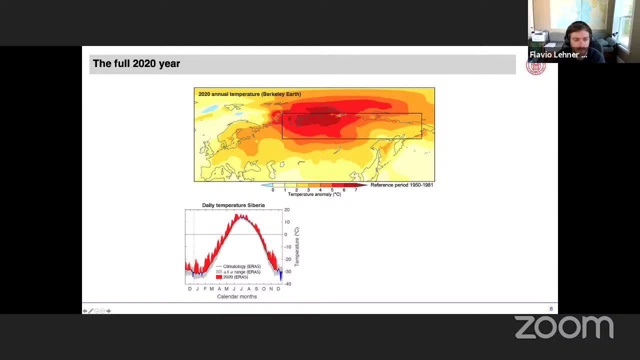 Almost every day was above normal. So very, very persistent temperature normally through the year, Then also leading to a four degree temperature anomaly, The annual mean, which is again sort of quite extreme but in generally consistent with long term trends. 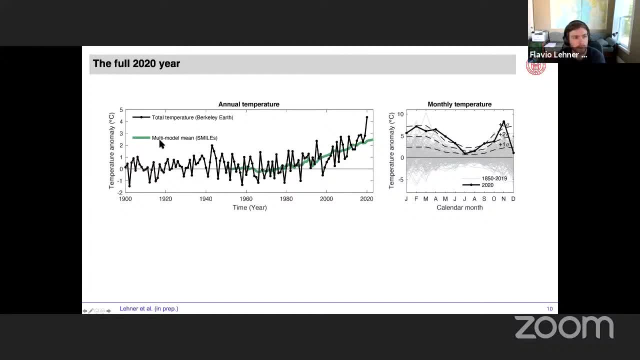 This is just plotted again here. Again, yeah, a multi-model mean doesn't really matter which ones seem at five to be this collection of large ensembles. whatever, It's generally consistent with that long term trend. What I want to point out here is, again, these are the monthly mean anomalies over the region of interest for 2020.. 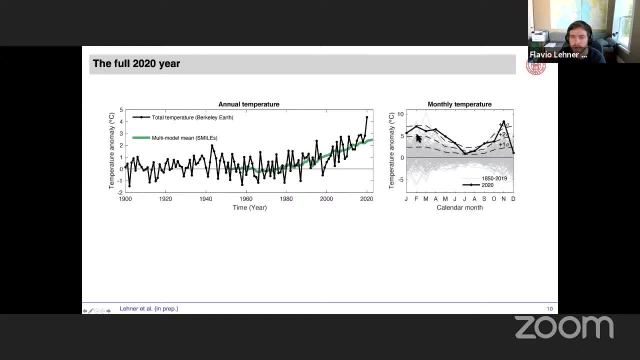 So really this consistent, positive anomaly throughout the year, at times three standard deviations over climatology And then in light gray. you see all the other years In the In the observational record. So we wanted to tease this apart a little bit more to understand how much of this anomaly was due to internal, mainly atmospheric circulation variability and how much might be driven by other factors and potentially feedbacks. 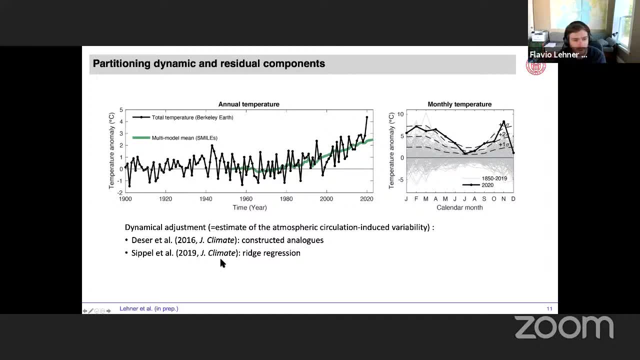 And we applied two dynamical adjustment methods. I'm not going to go into the details very much. In particular the first one I've used extensively and presented on earlier. That was coming out of work from Clara Desser and Laurent Théry. 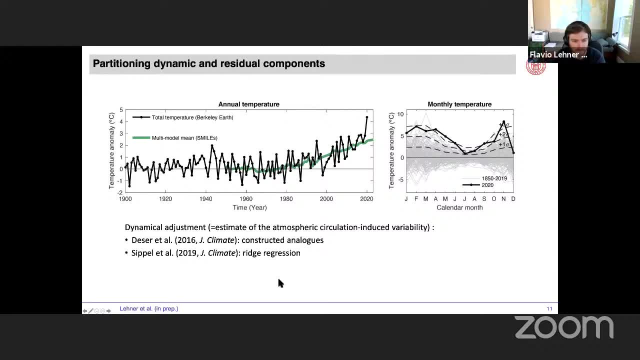 And then another one by Théry, And then another one by Sebastian Zippel. The point really here is to estimate with various methods the contribution of atmospheric circulation and its variability to, for example, temperature anomalies in this case, and try to separate that out. 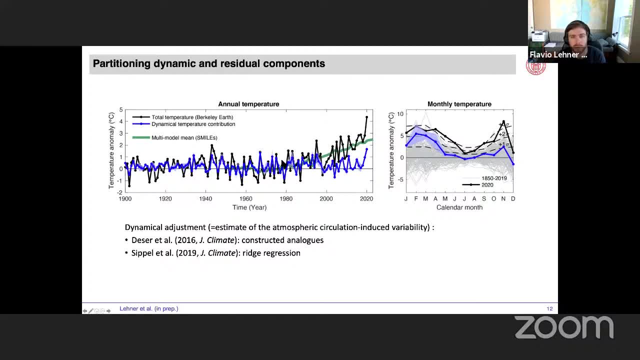 And so if we do that with both of these methods, we come up with an estimate of the contribution from atmospheric circulation variability to well the entire time series, but more specifically this particular year, And sort of consistent with our expectation that a strong arctic oscillation, a strong polar vortex influence this event. 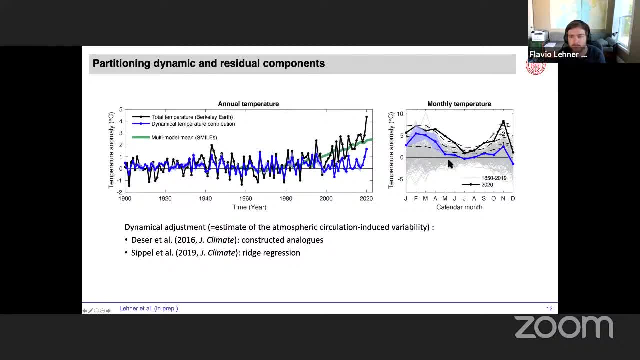 We see a large contribution from atmospheric circulation variability in the first half of the year and then less later on, And the residual effectively we can then use to interpret more as a thermodynamics driven component And we see that this was the one that dominated the temperature anomaly in the second half. 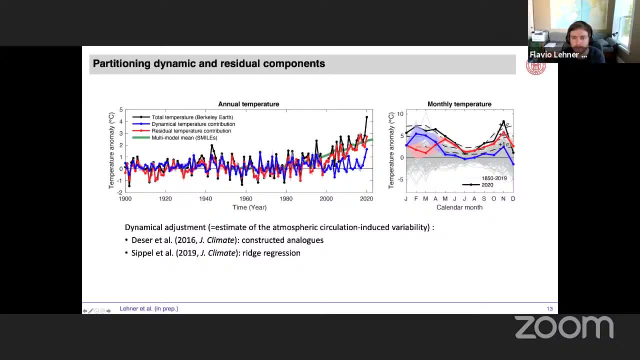 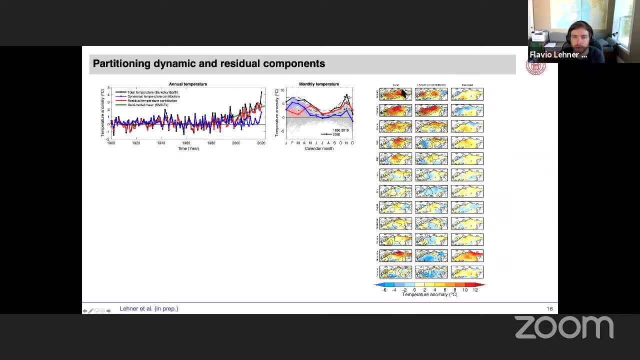 So somewhat contrasting about that Right evolution throughout the year. I'm not going to go into too much detail, but you can go in and look at the actual circulation anomaly and temperature anomaly in each month- January, February et cetera- and then the dynamical contribution. 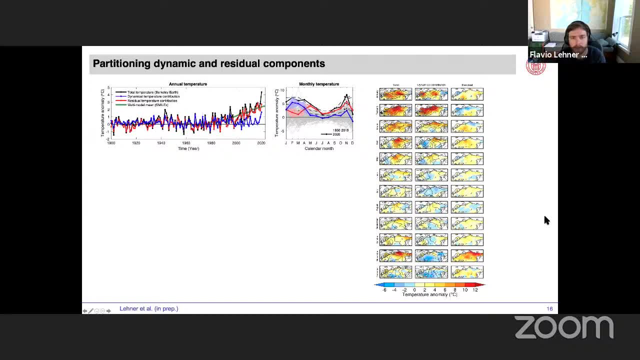 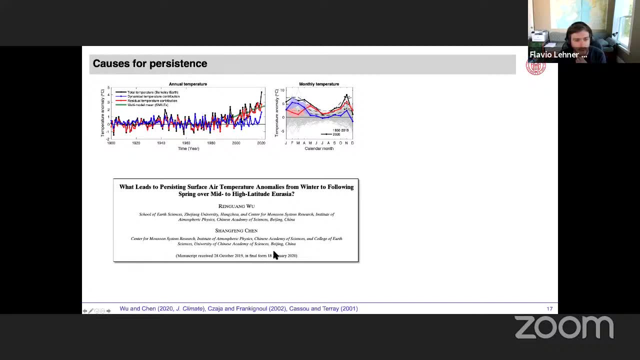 and the residual throughout the year. I'm not going to delve into that here, but that's something you can get out of these methods. And then it turned out that right around the time, so it was, I think, ultimately published in spring 2020,. 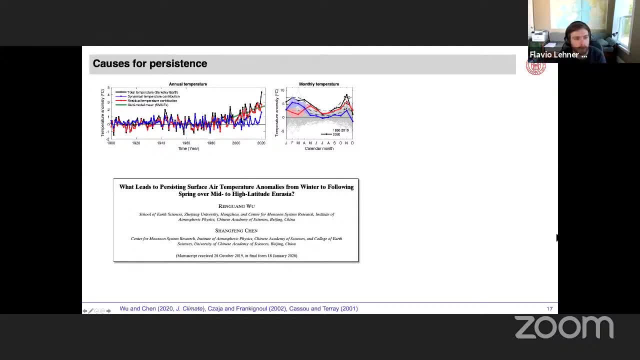 a paper by Wu and Chen looking at factors that lead to persistent air temperature anomalies. They were just focusing on going from winter to spring but over mid to high latitude Eurasia, And they sort of compiled a nice recipe, if you will, of some of the ingredients they think are important. 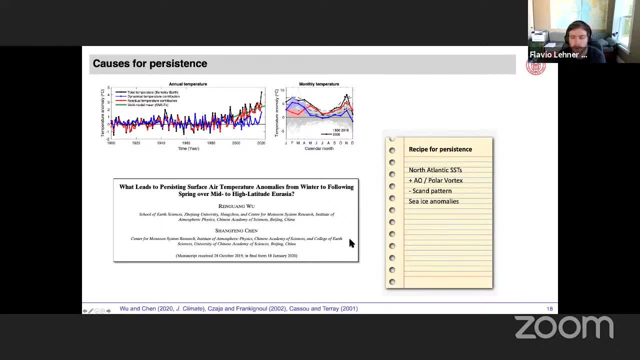 And they were hypothesizing, based on earlier work by others, that particular North Atlantic SSTs are favorable for a persistent Arctic oscillation. in this case It's not always clear that the strong polar vortex is driven by that, but we definitely had both of these patterns in place. 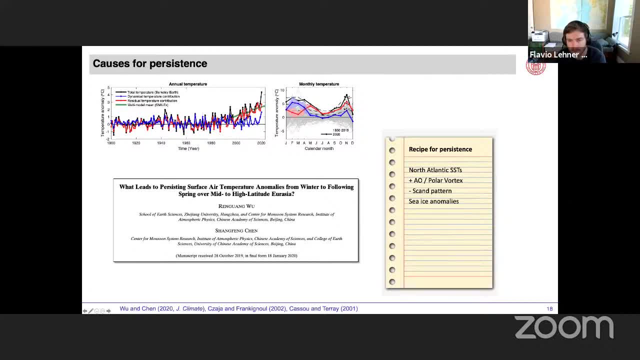 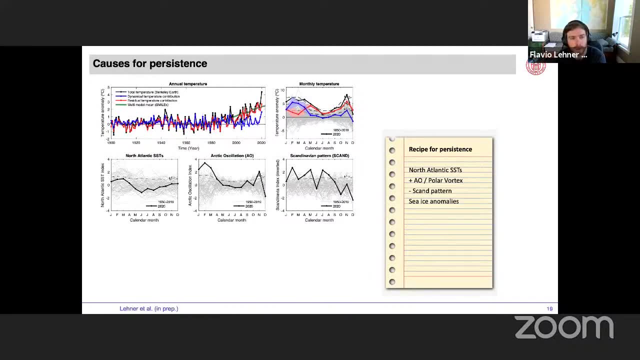 And then also the Scandinavian pattern as a circulation anomaly pattern becoming important in spring, And then also they touched upon the potential for CIS anomalies. But this was sort of like in the general sense but they had done this analysis on the historical record without looking at 2020 yet. 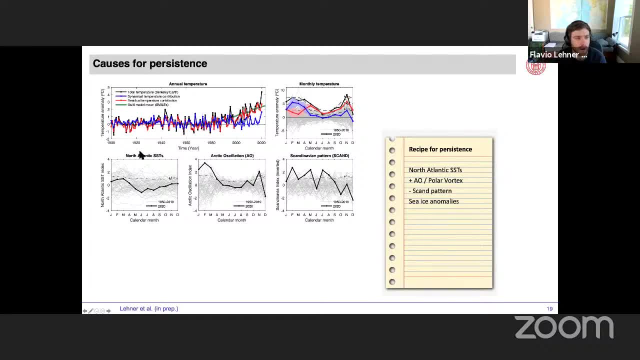 And so if you do look at these factors, the North Atlantic SST- I'm not going to show it here, but particular index- was slightly positive throughout winter. Here we see this very strong Arctic oscillation that I mentioned. that then goes back to normal values. 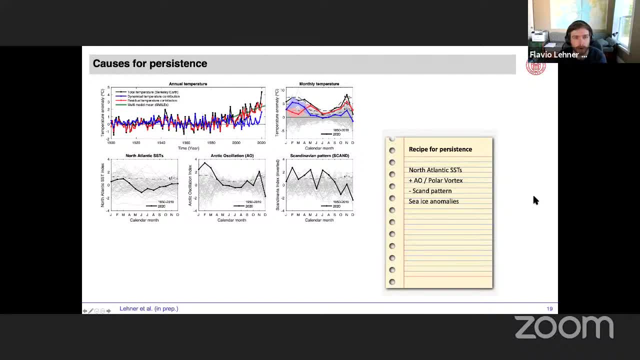 Scandinavian pattern also quite high in certain instances. So all of these ingredients were in place, And we also know that these ingredients are important for these linkages, And so here I'm showing the correlation for each month between atmospheric, the Arctic oscillation and temperature. 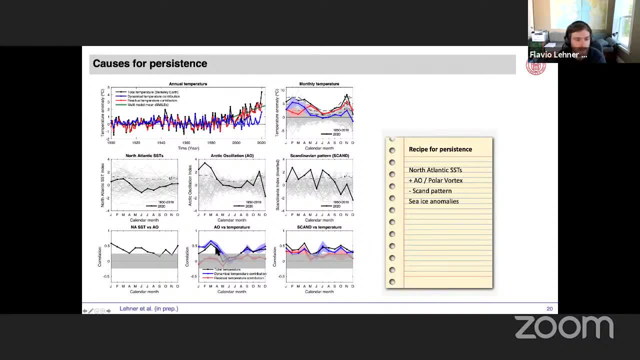 over the region of interest. And now what we can do. that's shown in black. Now what we can do. we can look at this also in the dynamical part, the blue part of the temperature, And we do see that this variability in generally, 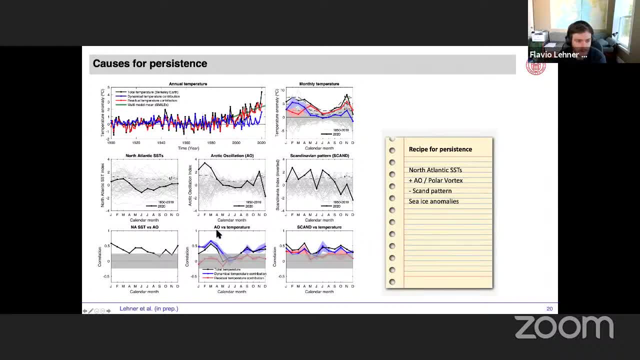 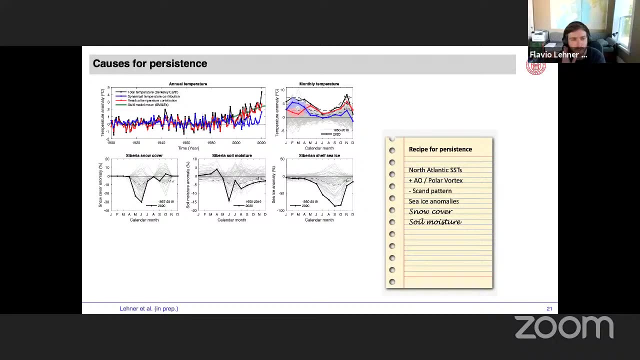 is very strongly correlated with the Arctic oscillation, while sort of the residual, this more thermodynamic part, isn't correlated, just as we'd expect. Slightly weaker correlations for the Scandinavian pattern- Two minutes, Yep, And then we looked at it. We had a few other patterns, sorry, other potential drivers. 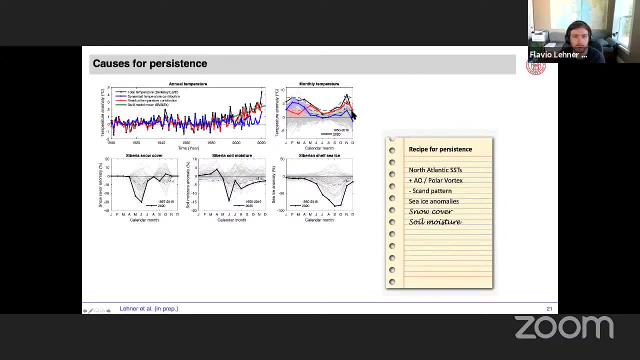 especially in context of this second half, where we think that the thermodynamic part is more important, like the Siberian snow cover, which was exceptionally low during 2020.. Then soil moisture, which also had almost a record minima in June, And then sea ice along the Siberian coast, which also 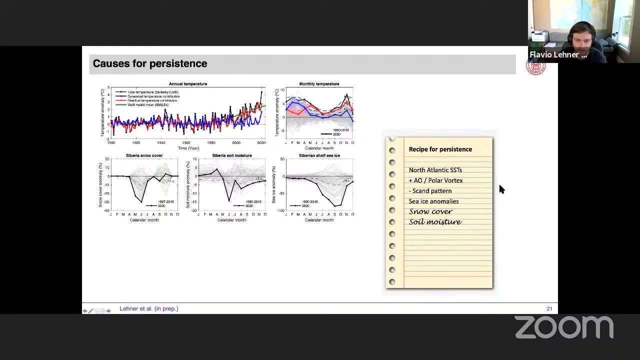 was record low in 2020.. And so those factors- Yeah, Yeah, Yeah- Are generally also correlated negatively with temperature in parts of the month, parts of the year, And again we see that this time around. if we do this dynamical adjustment. 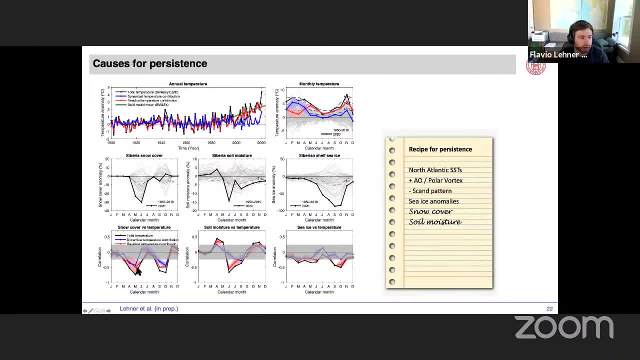 we see that the residual temperature- something that we might expect to be more thermodynamically driven- is more strongly correlated with snow cover, soil moisture and sea ice I forgot to mention. in all of these cases, temperature is detrended. 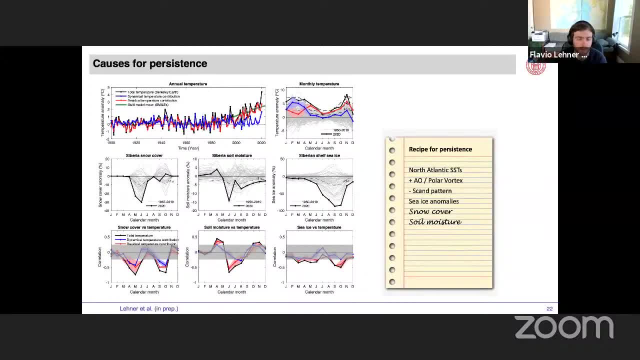 So we're like, We're like subtracting the long-term temperature effect, which would inflate some of these correlations a little bit. So those are significant in any case, And so then we can go in and try to reconstruct, especially this thermodynamic part of 2020, with a regression model that 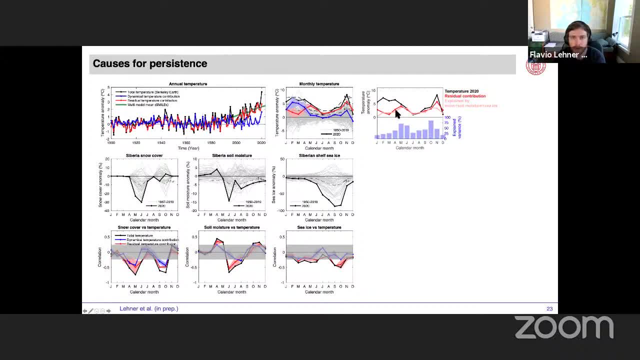 just uses snow, soil moisture and sea ice, And we can do a reasonably good job to reconstruct this red curve, except in November 2020, which still causes some headache Because The very strong thermodynamic contribution suggested by dynamical adjustment. 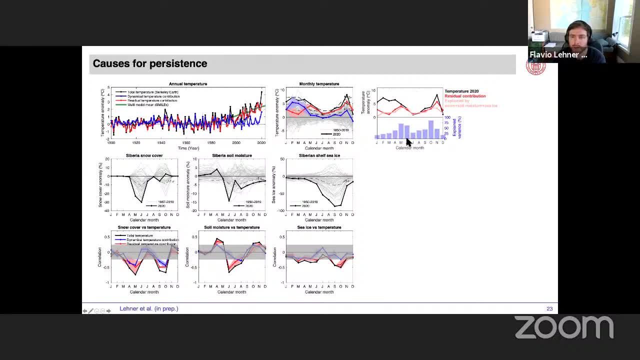 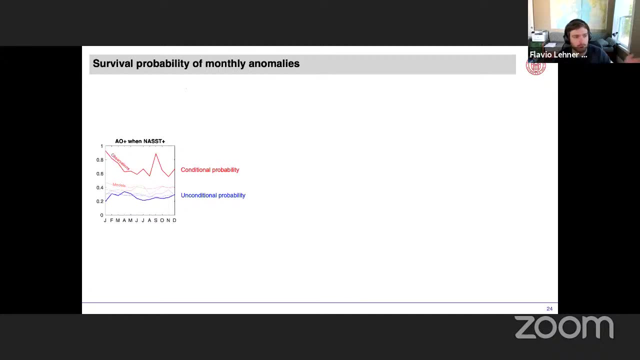 but it's not easily reconstructed. Here is the generally explained variance of this model. It's also not that high in November, So some questions remain in this part, And then I forgot to mention this. I have a whole bunch of slides because I'm 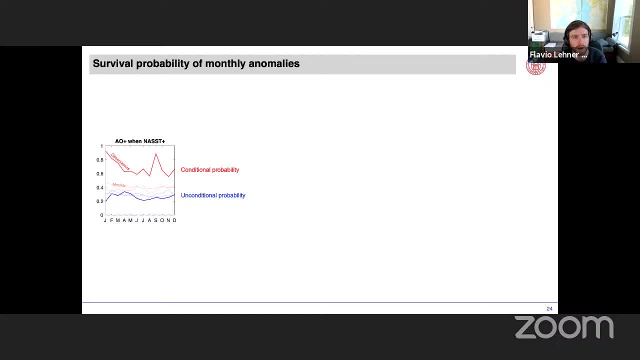 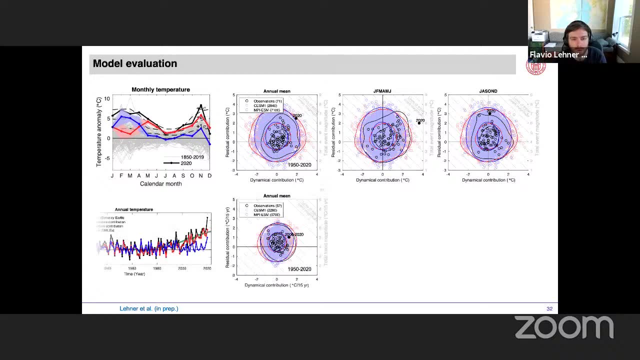 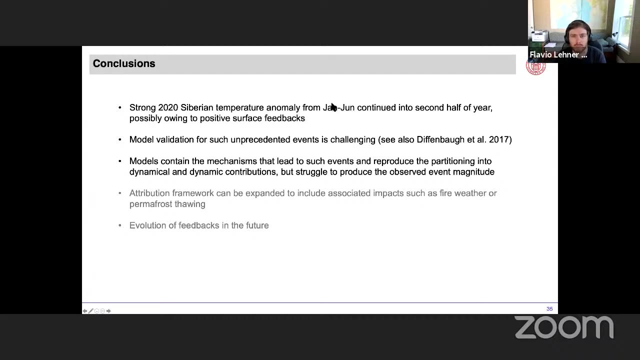 working on a larger, trying to get up to speed with this paper, I got to, unfortunately, skip over those for time reasons, So I'm going to go to the conclusions to summarize this. Yeah, we had these strong temperature anomalies that mainly grabbed the headline in the first half of the year. 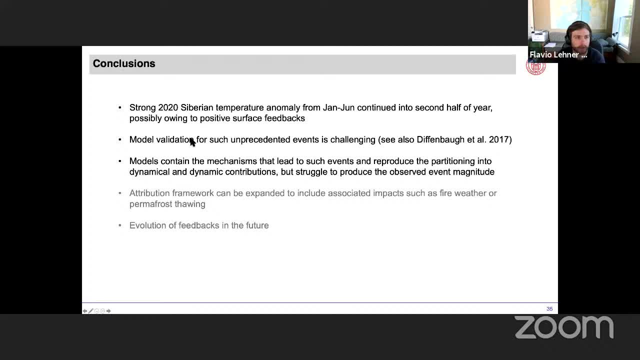 but continued on and are quite interesting. I didn't get to the part where we looked at the model validation, which is quite challenging because this is sort of an unprecedented event And to study the actual processes, which isn't usually done in classic attribution studies, it becomes quite tricky. 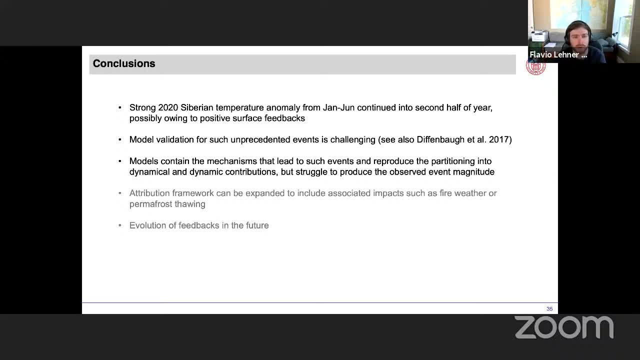 Because, Yeah, It's in any. in a lot of these observational metrics it's the most extreme event, But generally we do find the models to reproduce these mechanisms. We think this can be expanded to include other impacts such as fire or permafrost thawing. 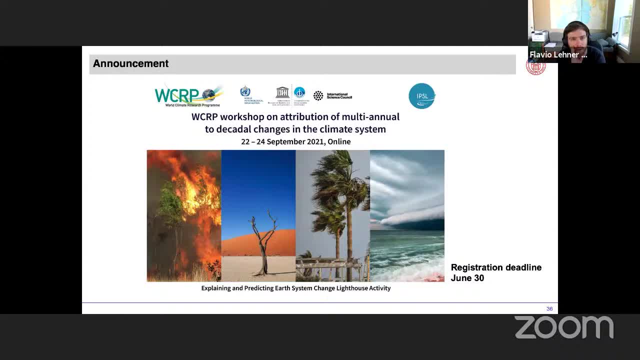 And I did want to plug this announcement- for a workshop that does look at attribution specifically of multi-annual to decadal changes, which is a bit of a new topic, and we're in particular looking for people who work with large ensembles and some of the tools that you've all presented on. 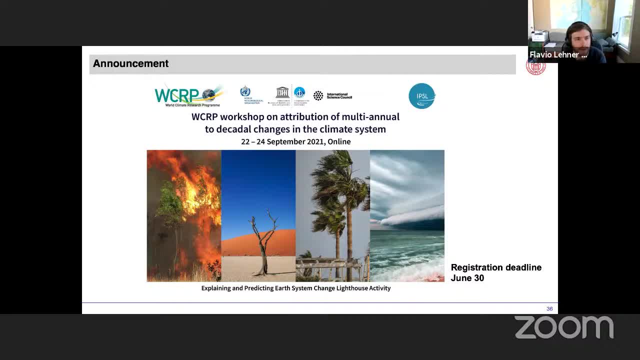 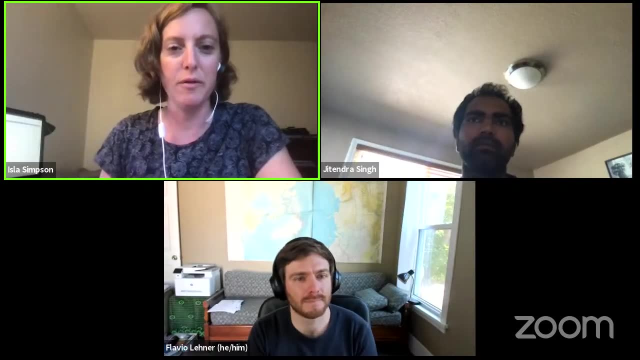 It's going to be virtual and free and registration deadline is coming up soon. Thanks, Thanks. Are there any questions for Flavio? I guess I was wondering. you mentioned that the first half year was very well forecast. Do you know how the forecasts were predicting things? 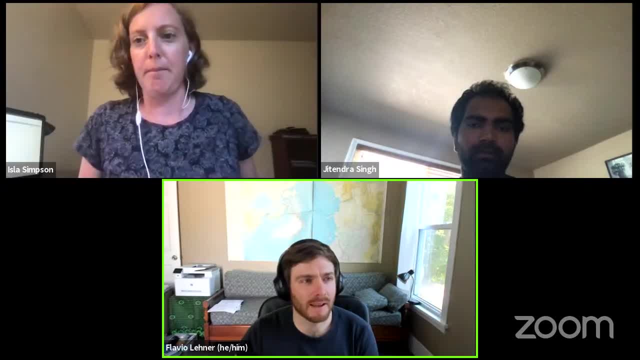 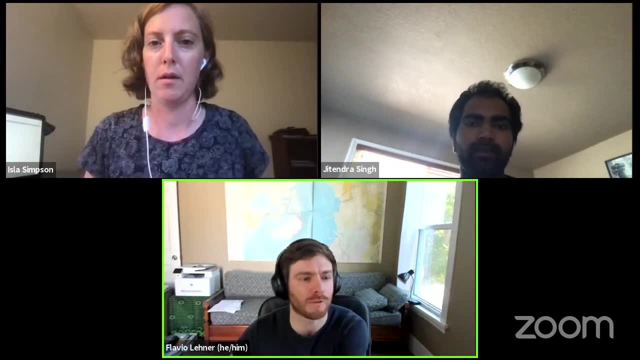 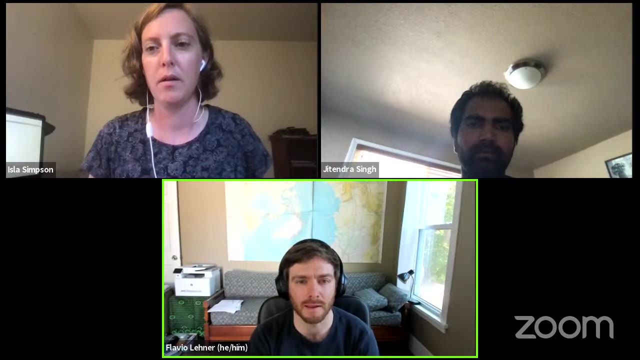 for the second half, I haven't looked yet and I should also say that this was mostly for the circulation. Hopefully that translated into good forecasts for surface temperature as well and other factors. But yeah, this was the classic sort of 500 hectopascal pattern. 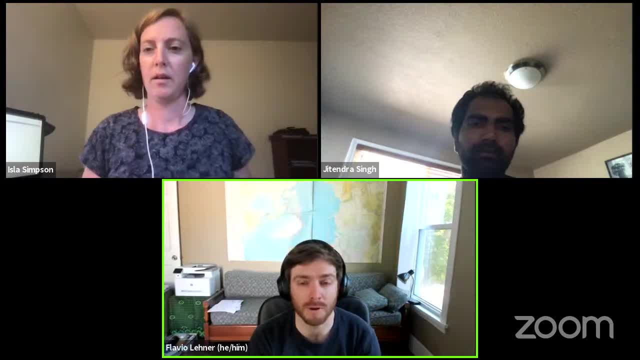 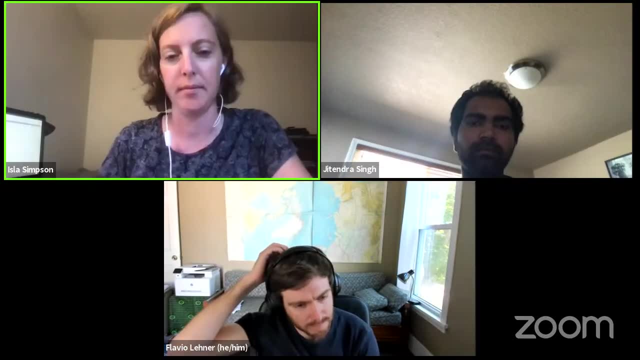 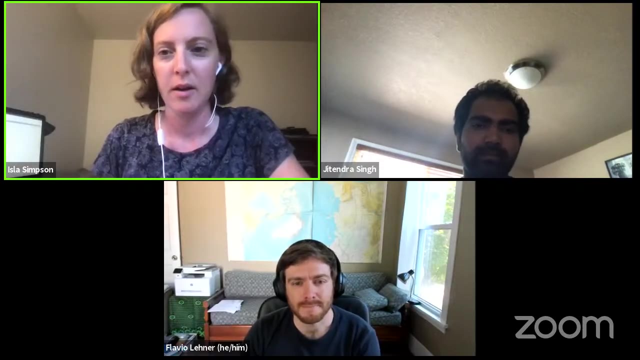 correlation. I think that is quite So. I'd have to look into that or, maybe easier, ask these authors. Yeah, I think that was Simon Lee and the other paper was by, I think, Sak Lawrence. Yeah, OK, All right. 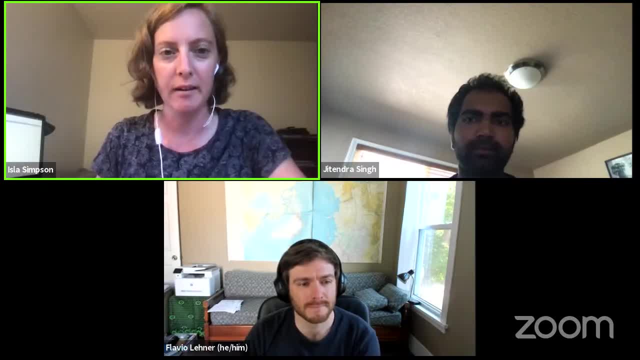 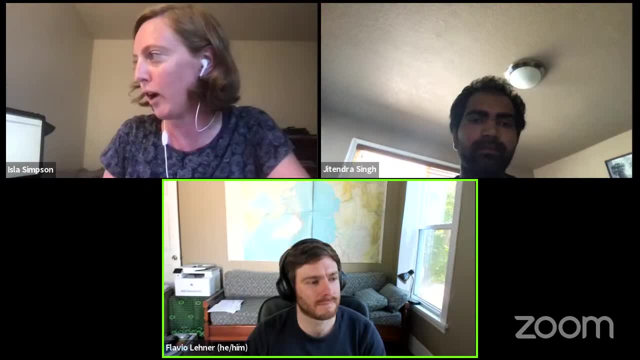 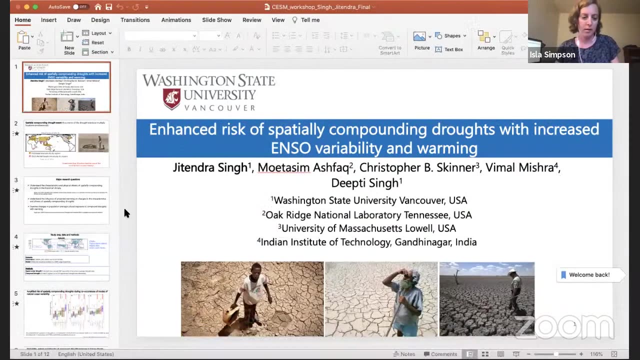 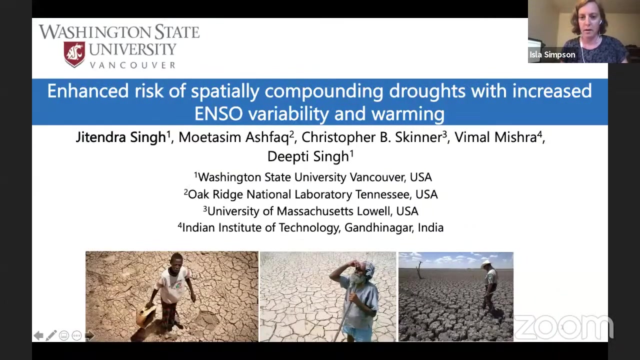 Well, if you have any more questions for Flavio, you can type them in the chat. Our next speaker is Jitendra Singh, talking about enhanced risk of concurrent regional drives with increased ENSO variability and warming. JITENDRA SINGHALA- Yeah, sorry, I just muted myself. 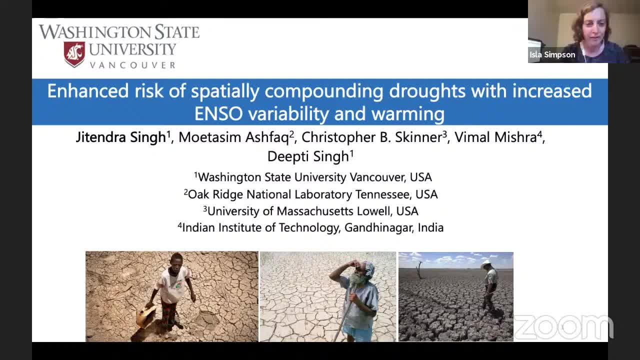 So my screen is visible to anyone, right? Yeah, that looks good. JITENDRA SINGHALA- Yeah, And so hi everyone. I'm a postdoctoral research fellow at Washington State University, Vancouver, So I will present some of my work. 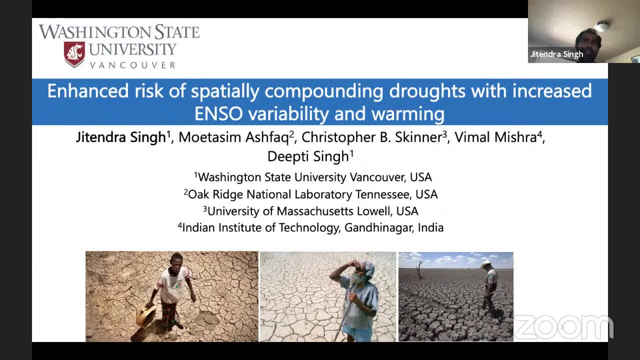 I have been doing in postdoc, So my presentation would broadly focus on understanding simultaneous droughts and their drivers and historical and future climates. So I'd like to acknowledge my collaborator listed here for their suggestions and feedbacks on this study. So the compound droughts events are: 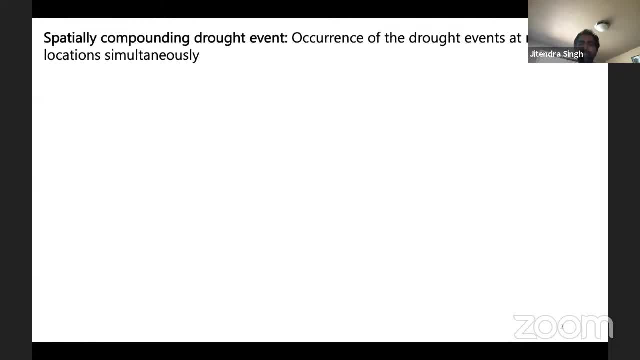 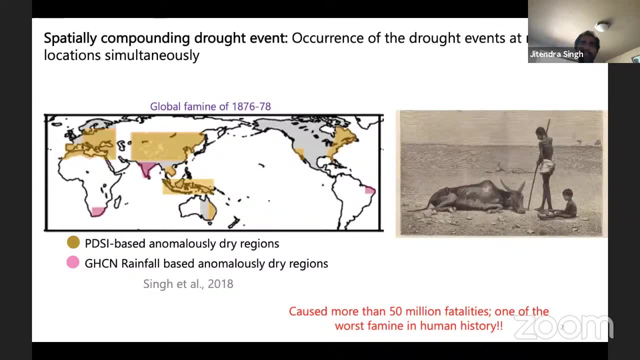 defined when multiple regions experience drought simultaneously. So the motivation of this work comes from a historical drought event which occurred during 1876 to 1878, when multiple regions, which are highlighted with yellow and pink color, experienced the drought simultaneously. So it was a multi-year drought which 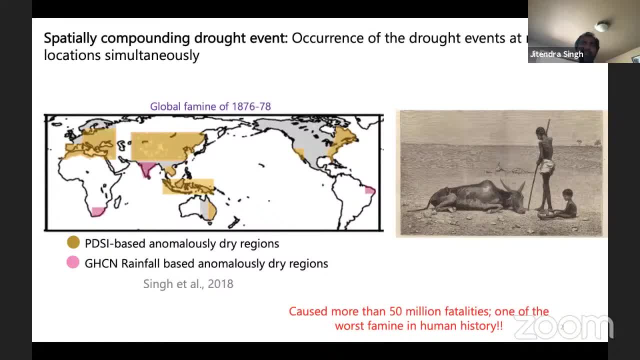 caused widespread crop failure and further catalyzed the global famine, which resulted in more than 50 million fatalities. So this event was considered one of the worst famine in human history. However, the impact from such event may not be same in today's world. 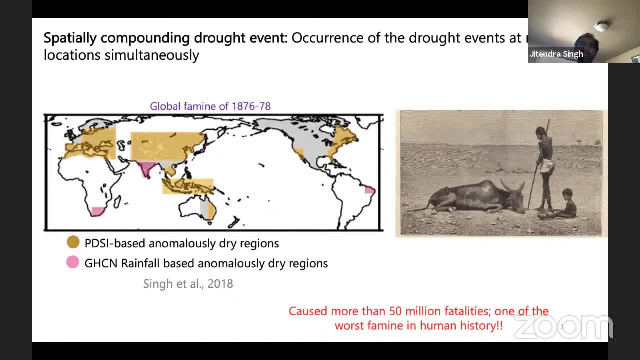 but still it may have a serious impact on global food system. For example, these kind of events may affect the food production, and which may increase the global food prices. So, from this point onward, I will give you a little bit of background. 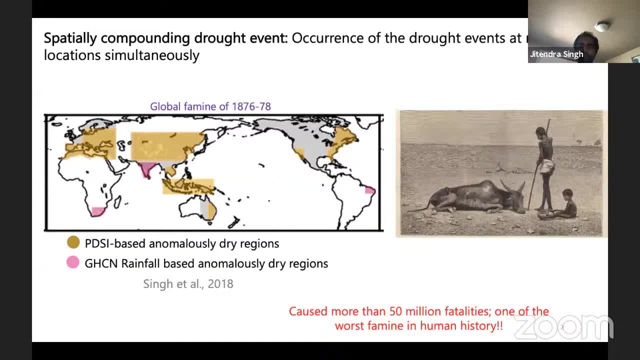 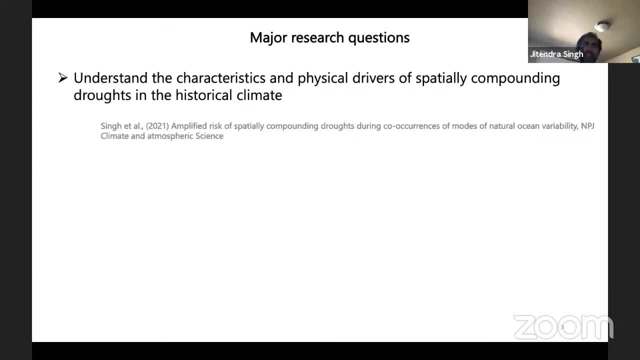 I will use the compound drought instead of saying spatially compound droughts. So this study explore broadly three major questions. So first, we focus on understanding the characteristics and physical drivers of compound drought in historical climate. Second, we understand the influence of projected warming on changes in characteristics. 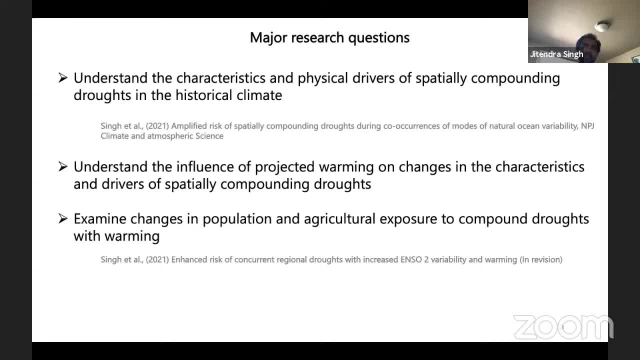 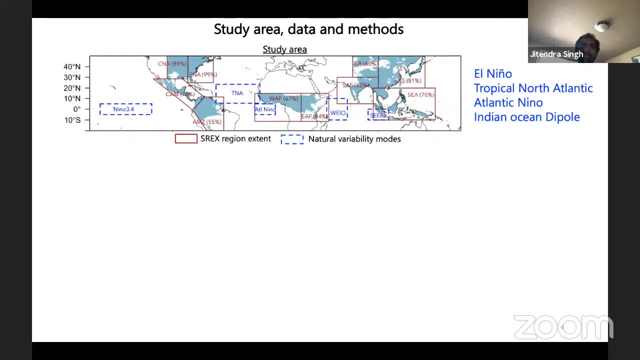 and driver of compound drought. And lastly, we focus on examining the changes in the population and agriculture exposure to compound droughts with warming. So we study the compound droughts over these 10 regions marked with red solid lines. So basically, several of these regions. 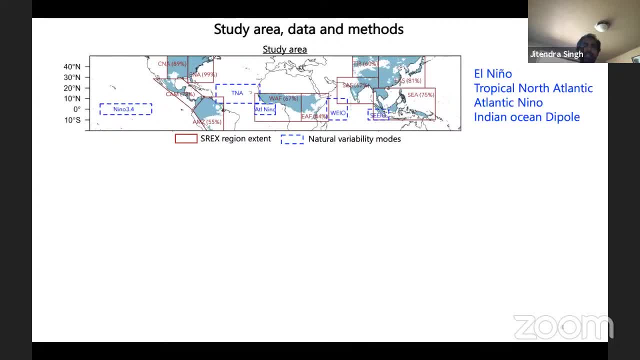 are influenced by global monsoon systems, And these regions includes important broad bed waskets and vulnerable populations that depend on land-fed agriculture for their livelihood. So within each region, we consider the only area which shows The variability during summer monsoon precipitation. 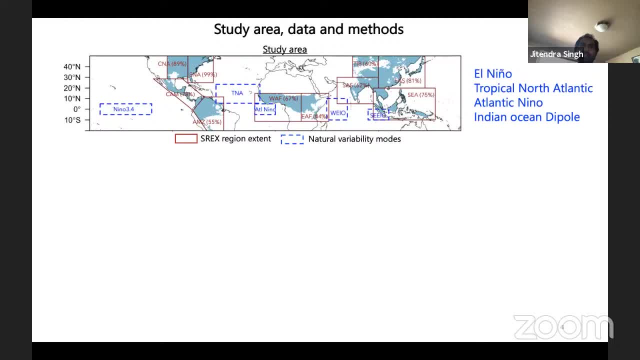 which is indicated with teal color Text and red color shows the fractional area with higher variability within each SX region. So we also consider sea surface temperature over various ocean areas marked with dashed blue line to define the modes of natural variability. So we examine the influence of these four variability modes. 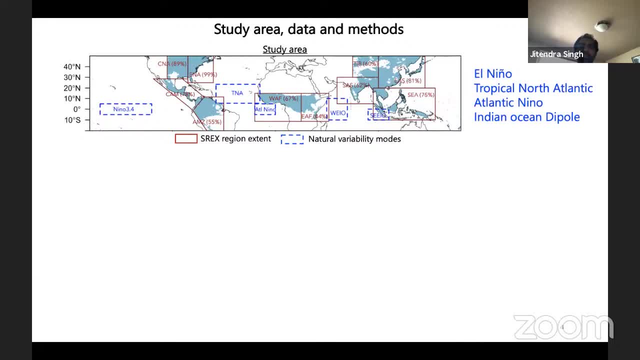 on compound drought characteristics. So these modes are Indian Nino, Tropical, North Atlantic Atlantic Nino and Indian Ocean Dipole. So these modes are known to have an influence over one or more regions we consider in this analysis. So we use observed precipitation from CHIRPS and CRU and the SHD. 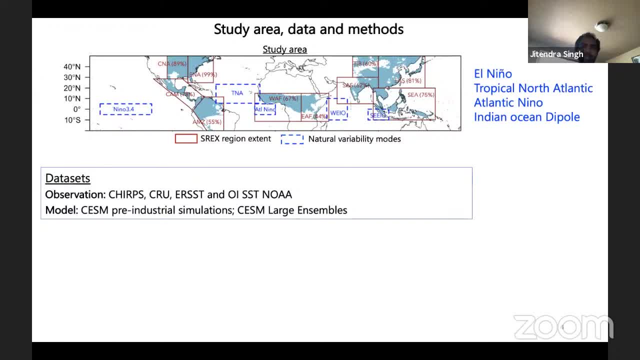 from the NOAA And we also use CSM- pre-industrial and large ensembles. So we define region under drought if drought affected area exceeds 80th percentile of long-term average drought area And we define the compound drought event if at least three regions out of 10 experience. 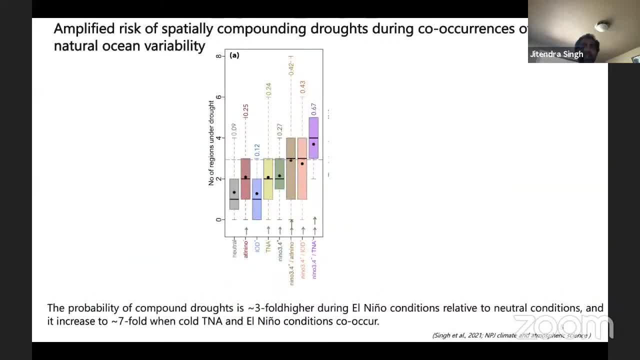 drought simultaneously. So we identify the specific phase of four variability modes relevant to compound drought based on the observational analysis And due to larger sample size. so we use the CSM pre-industrial simulation here to isolate the influence of each individual modes and their co-occurrences phase on compound droughts. 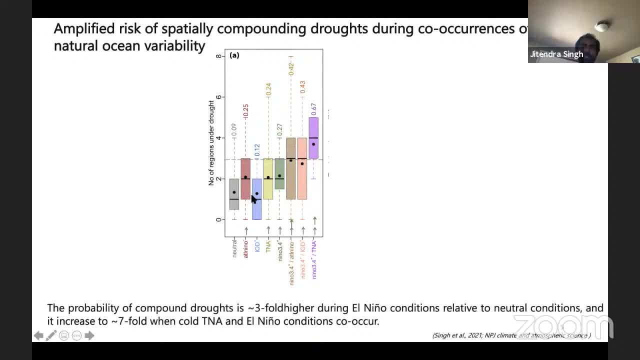 So this figure shows the distribution of number of regions experienced drought simultaneously during the occurrences of individual and combined variability mode, which is indicated on the x-axis. So the number on top of each box shows the probability of compound droughts during each condition. So we define the neutral year when the SHDs over TNA Nino 3.4,. 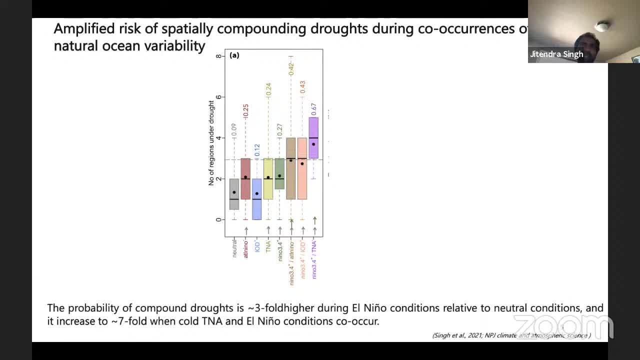 Atlantic, Nino and Indian Oceans are within a plus minus 0.5 HD. So the horizontal dashed line shows the threshold used to define the compound droughts. So the significant difference in the distribution is marked with arrows. So the distribution of drought region. 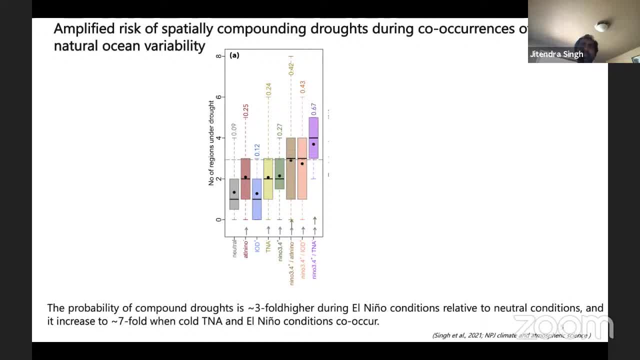 during negative phase of Atlantic Nino, so which is like a negative Atlantic and the negative TNA, and during El Nino conditions are significantly higher than that during the neutral condition. So, more specifically, the probability of compound drought increase more than two times during neutral conditions. 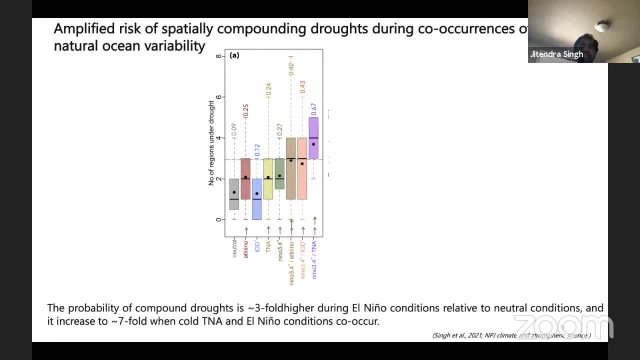 Negative Atlantic Nino and TNA conditions and around three times during El Nino, conditions related to the neutral conditions. So further, the co-occurrence of negative TNA conditions with El Nino increase the probability of compound droughts nearly seven times relative to neutral conditions. 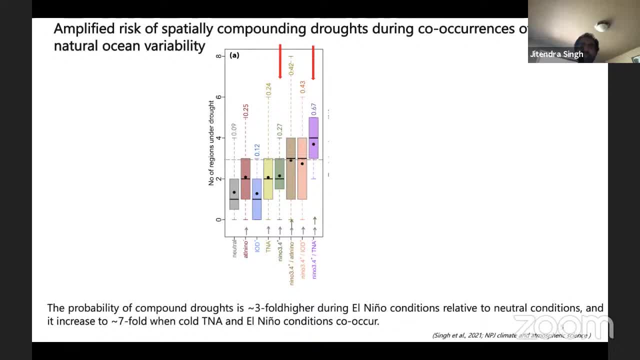 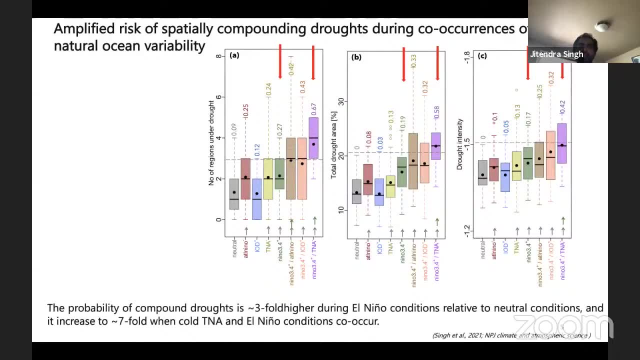 and more than two times relative to El Nino conditions alone. So we find a similar influence of individual and combined modes of variability on distribution of drought area and drought intensity. So overall we find that El Nino is the major driver of compound droughts and TNA negative conditions. 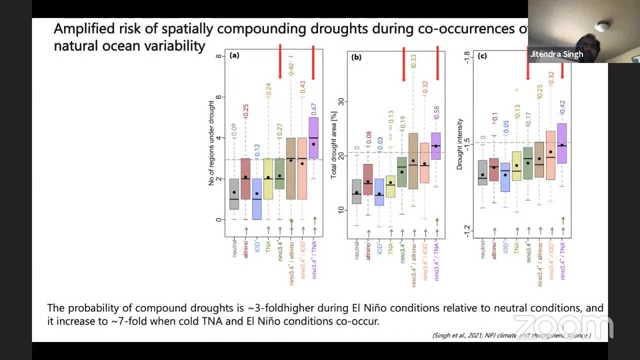 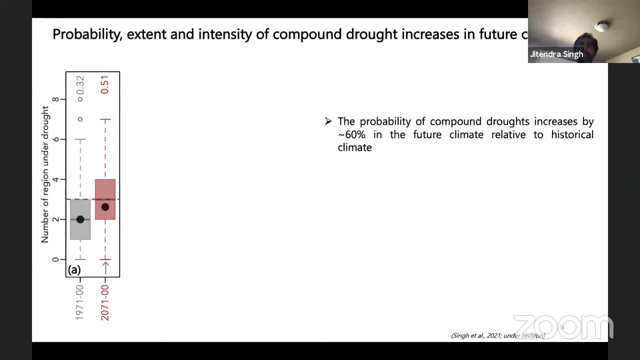 has a largest amplifying influence on the El Nino driven compound droughts. So next, now we have some understanding about the compound drought and its drivers, So we further extend this work to understand the compound droughts in future under business as usual scenario. 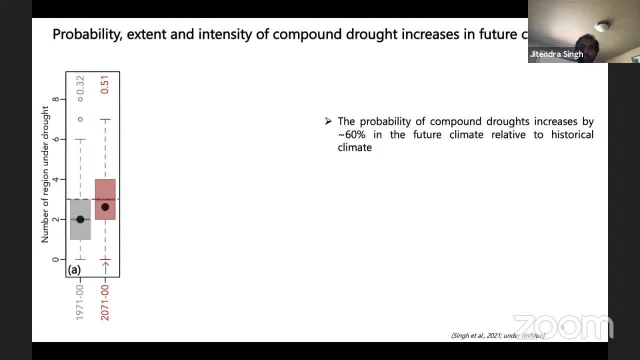 RCP 8.5.. So for that we use the CSM large ensemble for this analysis. So this figure shows the distribution of drought region in the historical climate, which is defined as 1971 to 2000, and the future climate. 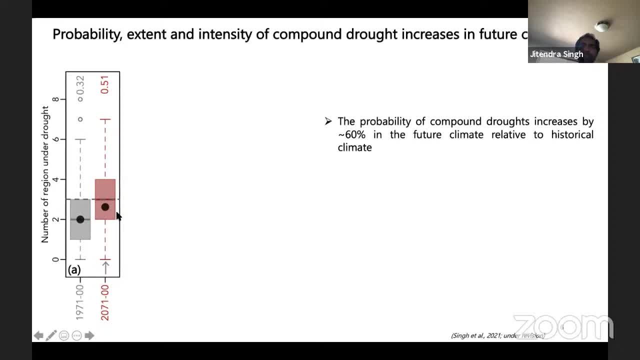 with the red color, which is defined over 2071 to 2100.. So the number of top of each box shows the probability of compound droughts and the horizontal line is same, which shows the threshold used to define the compound drought. 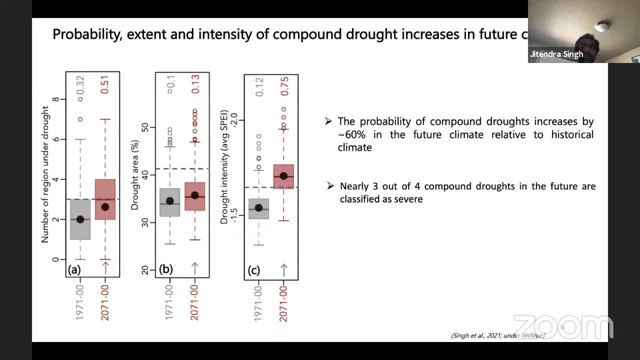 So overall we find a significant increase in the distribution of drought region in future relative to baseline period. that is the kind of historical period. So the probability of compound droughts increases by around 60% in the future. relative to historical period, We also find similar changes in extent and severity. 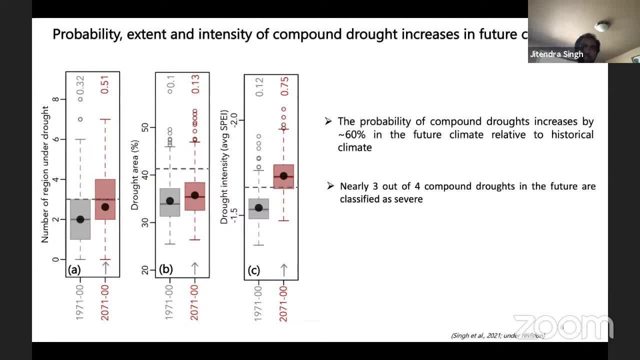 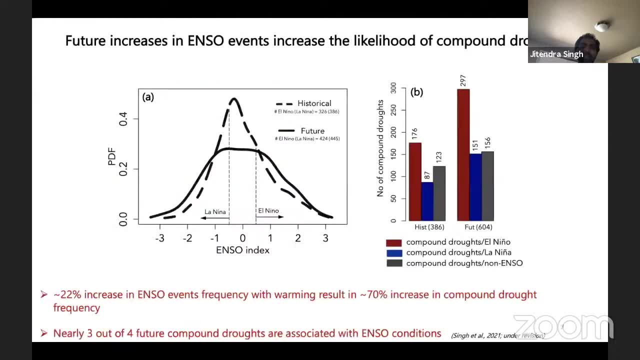 of compound droughts in future relative to historical climate. So specifically, nearly three out of four compound droughts in the future are classified as severe, And we also find a significant increase in the distribution of compound droughts in the future relative to the previous analysis. 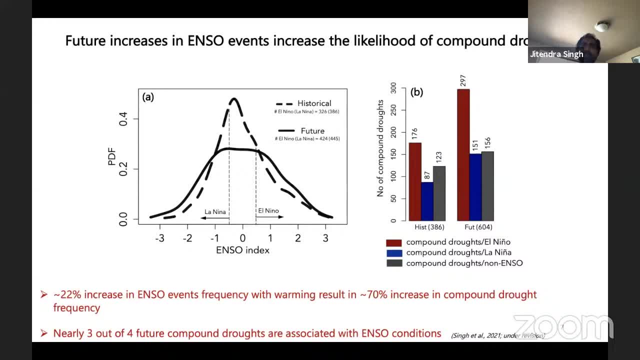 So we examine the historical and future characteristics of the Enso Index and their association with the compound droughts. So in the panel A shows the PDF of the Enso Index which shows almost 22% increase in the frequency of L-linear and La-linear conditions, which is consistent. 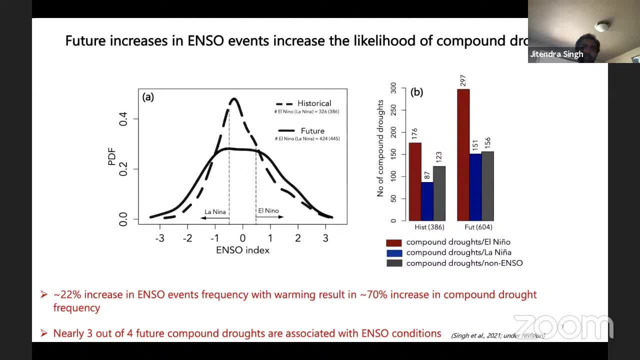 with the previous studies, such as CHI et al 2014 and 15.. So that shows that. So the panel B indicates the distribution of compound droughts associated with L-linear and La-linear conditions and non-Enso drivers. So the number on each bar shows the count. 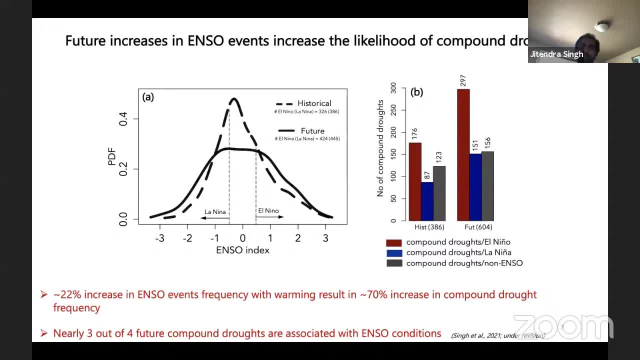 of compound droughts associated with the L-linear and La-linear and non-Enso drivers. So, although L-linear is associated with the major fraction of the compound drought, La-linear are also associated with a significant fraction of compound droughts in the historical climate. 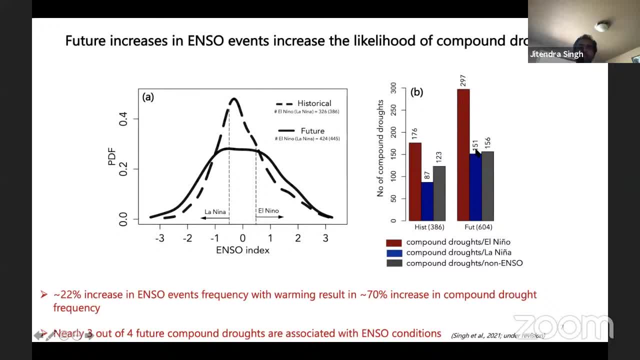 and it further increases in the future. However, the regions they affect may differ, So the panel B indicates the distribution of compound droughts in the historical climate. there are three main droughts associated with the L-linear and La-linear conditions and non-Enso drivers. 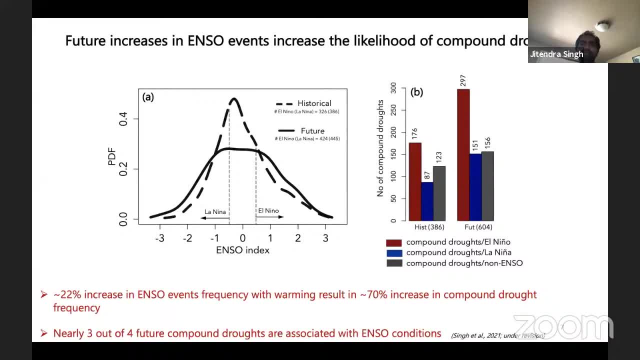 So overall the frequency of compound droughts associated with the L-linear and La-linear conditions increases by 70% in the future, in response to just 22% increase in the frequency of Enso conditions and future warming. So in the future nearly three out of four compound droughts. 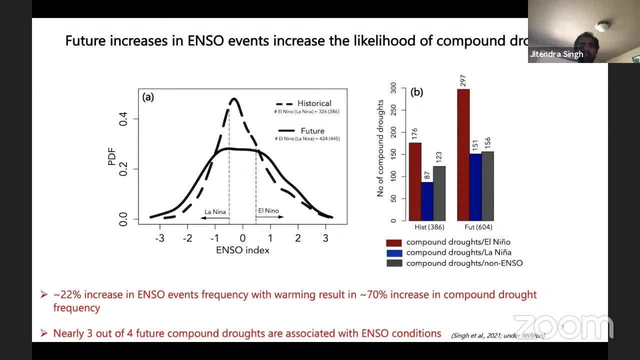 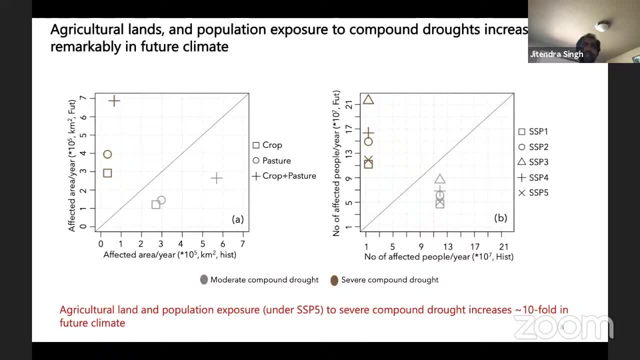 are associated with the Enso conditions. So we further estimate the population and agricultural and exposure to compound droughts to panel A. So the panel C indicates that total shows the comparison of agricultural land exposure to moderate and severe compound drought between historical and future climates. So the x-axis shows the agricultural land exposure. 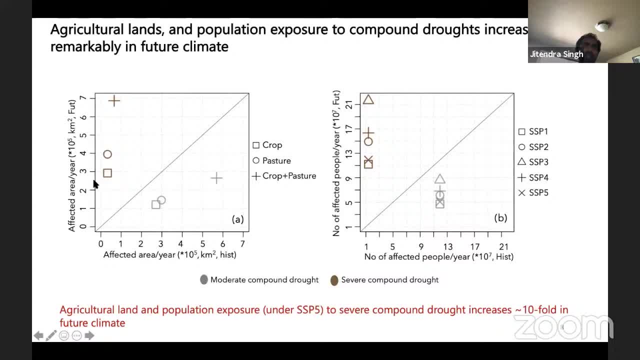 to moderate and severe compound drought in historical and y-axis shows for the future climate. So, however, I will just focus on the exposure to the severe compound droughts. So the agricultural land exposure to severe compound droughts increase almost tenfold in the future climate relative to historical climate if we compare with the one ratio one. 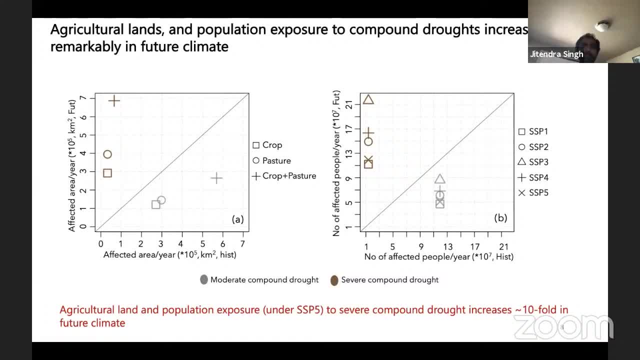 line. So similarly we see a remarkable increase in the population exposure to severe compound drought. So we consider the population Exposure under all SSPs to highlight the difference. in the projected population scenario, However, SSP 5 is the largely consistent with the RCP 8.5.. So under SSP 5 scenario we find 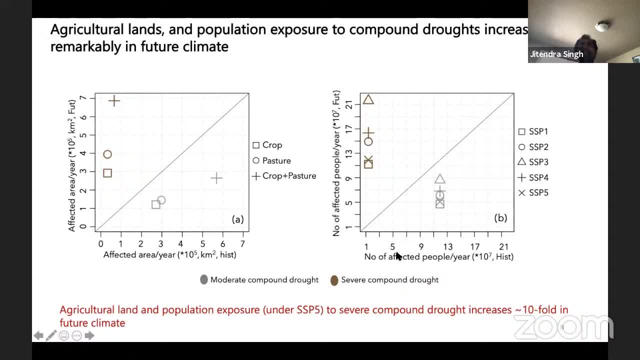 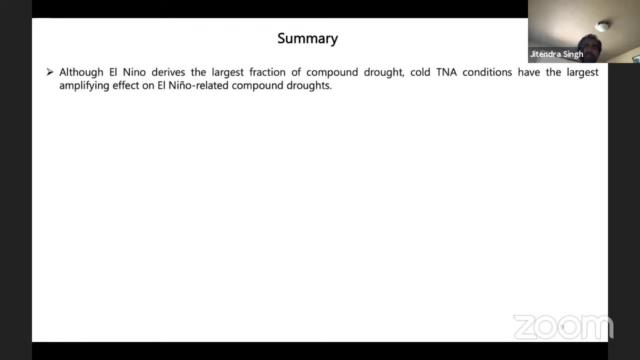 that, on an average, 10 million people per year are exposed to severe compound drought, where this number increased to 120 million, like around 120 million per year in the future climate. Okay, thank you, So I will quickly summarize the results. So we find that L-lino is the major driver. 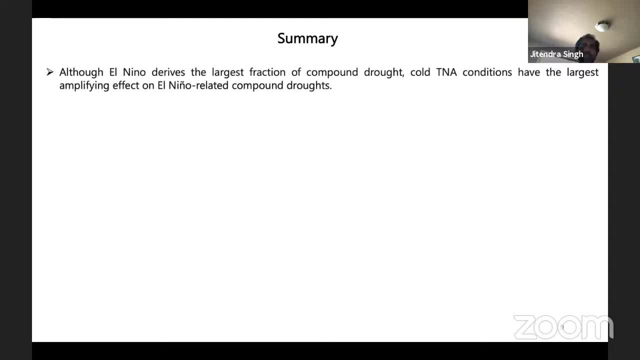 which control the largest fraction of historical compound drought. However, the co-occurrence of cold SSTs over DNA has largest amplifying influence on L-lino-turbine compound drought, So the probability of compound droughts increases by 60% in the future climate relative to historical. 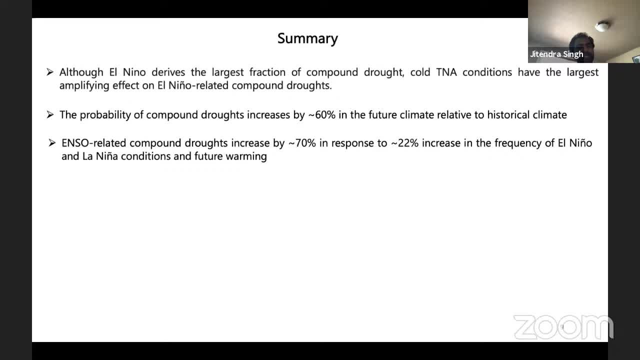 period And ENSO-related compound droughts increases by 70% in response to just 22% increase in the frequency of ENSO conditions and future warming. So the increase in future compound drought characteristics result in up to almost tenfold increase in agriculture and land population exposure. So these results have several implications. 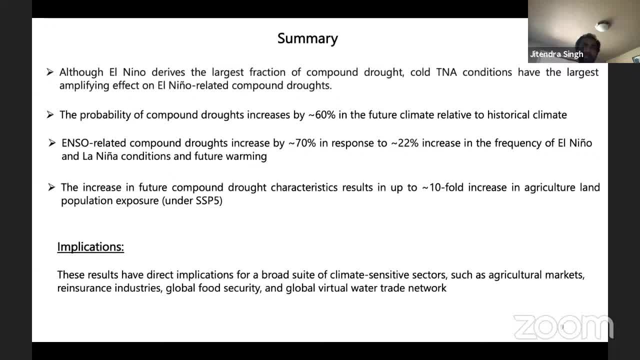 for a wide range of climate sensitive sectors, such as global food security reinsurance industry, and also these results have a broad implication in the global virtual water trade network which involve water intensive goods. Thank you, I'm happy to take answer And also we are revising the second manuscript. 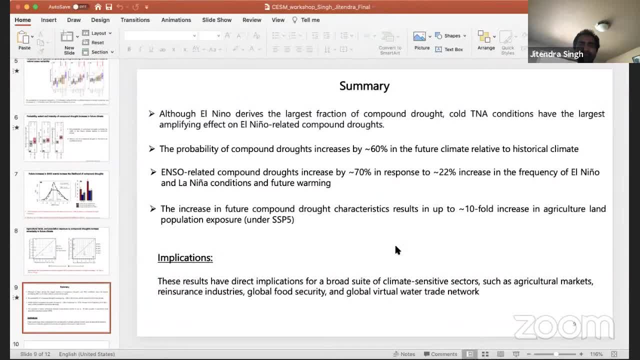 so I would appreciate any feedback, Thanks. So there was one question in the chat from Sanjeev asking why you didn't include the US Southwest in your analysis. Yeah, so initially we considered the US Southwest analysis, but we consider only region which. 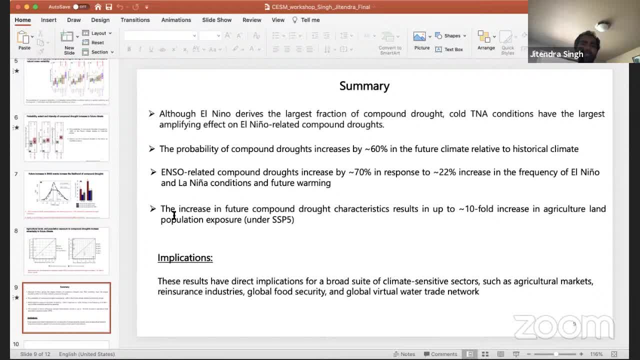 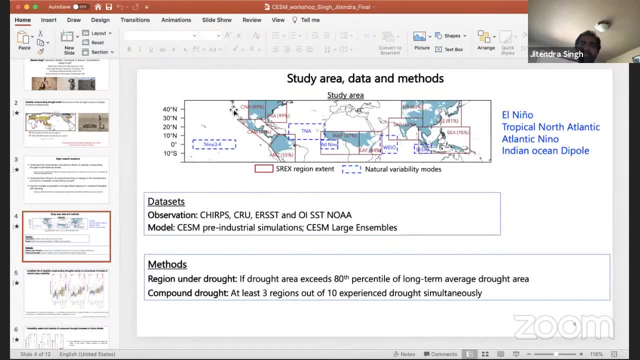 shows the high variability in the boreal summer precipitation. So we found that there was a really small fraction of area which shows the high variability over these regions And we used the criteria when at least 30% of that region shows the high precipitation variability. So that's why we excluded 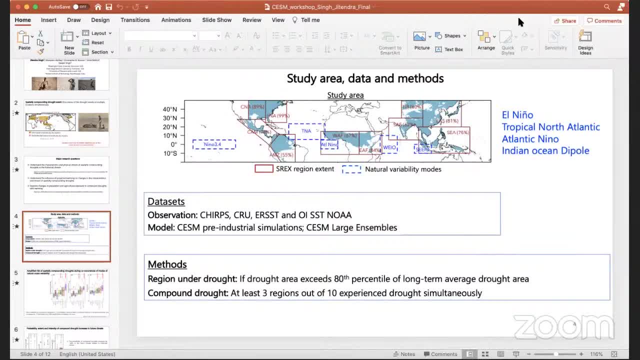 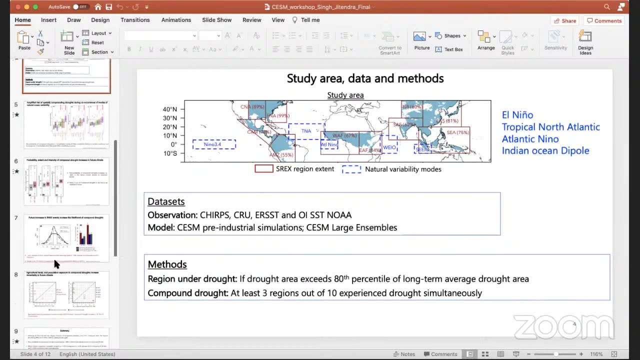 And Nicola Hi, Thanks for the interesting talk. I was wondering if you can comment on how model dependent the results are. If you look at different large ensembles, you get quite different future projections of ENSOs. Yeah, So I was wondering how that would affect this study. 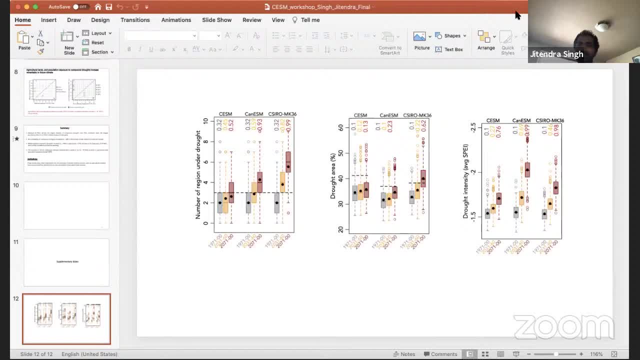 Yeah, So I'm revising that paper and we got the same comment from the reviewer So I'm working on that. So I smile a couple of more model from the smile And so we found like a quite good consistency in terms of compound drought characteristics across the model. 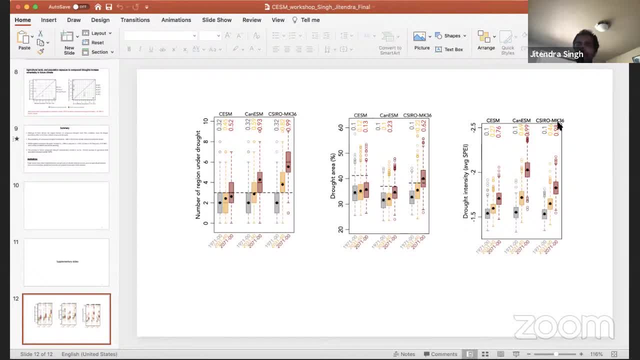 But definitely there are some differences in the ENSO response in different models. So we are still working on that. Yeah, So this figure is showing like a same distribution of number of drought region, drought area and drought intensity, And so this is the first three box plots for CSM. 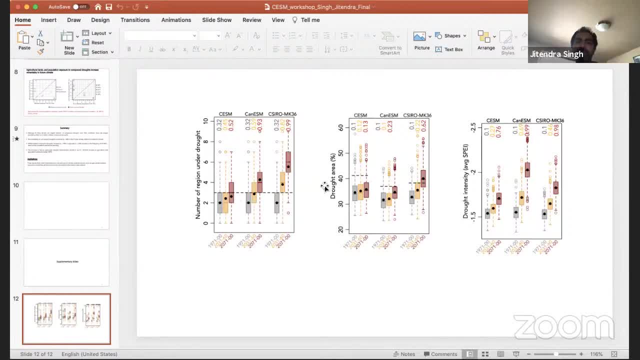 and the middle one is for the CAN-ESM and last three ones. So we see a strong consistency between these models in terms of drought characteristics. Okay, Thank you. So we'll move on to the last speaker of the session, Xiaoxin Ban, And he's. going to talk a little bit more about this. Okay, Thank you, So we'll move on to the last speaker of the session, Xiaoxin Ban. Okay, Thank you, So we'll move on to the last speaker of the session, Xiaoxin Ban, And he's. 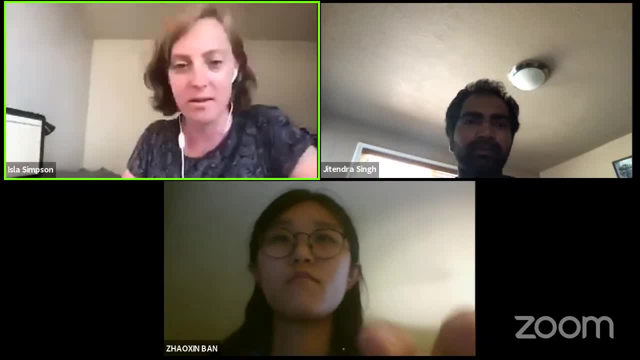 going to talk a little bit more about this. Okay, Thank you. So we will open at 16.. Okay, Thank you. So we'll move on to the last speaker of the session, Xiaoxin Ban, And he's going to talk a little bit more about this. 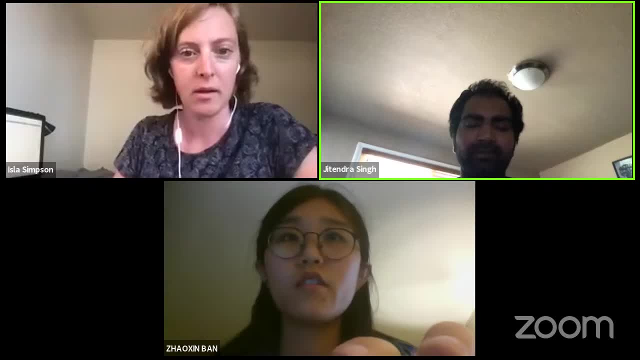 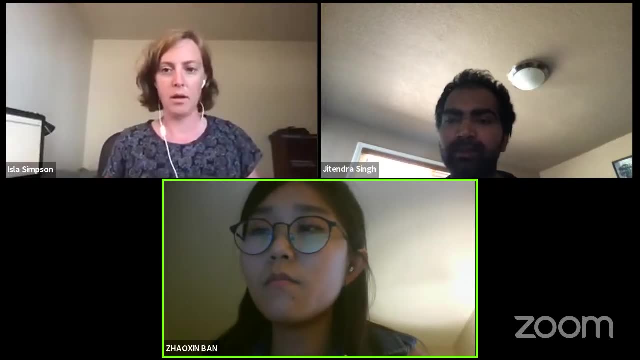 Okay, Thank you. So we lost our audience, so we are going to able to speech to Johann, who is going to talk a little bit more about this. Hi everyone, How are you doing? Of course Sounds good, Okay. Yeah, we can hear you again. 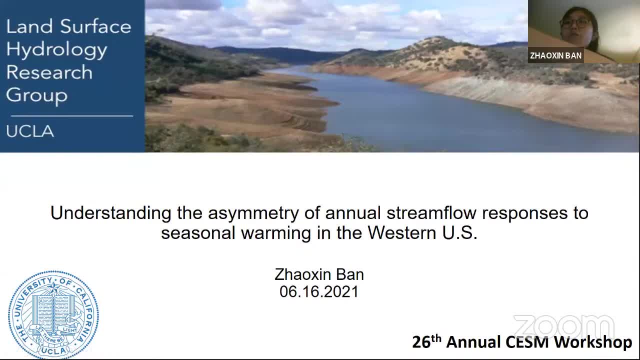 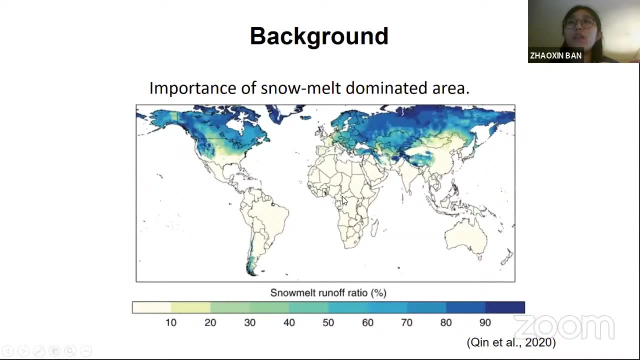 We don't hear anymore. Okay, Okay, Yeah, Yeah. Let me just briefly repeat the names: Okay, Okay, Yeah, Yeah, Yeah, Okay, Yeah, Yeah, Okay, All right, Yeah, Yeah, US. More than 26% of the global land area depend on snowmelt as their dominant water resource. 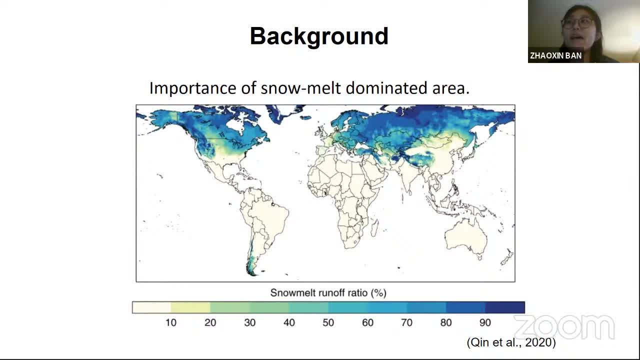 Western US is a typical snow-dominated region which snowpack has experienced a significant decrease in their climate warming, leading to a significant decrease in snowmelt-generated runoff. These changes are challenging to the region's social-economical safety. Therefore it is 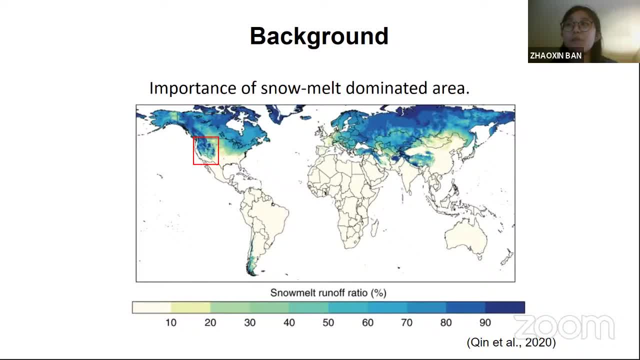 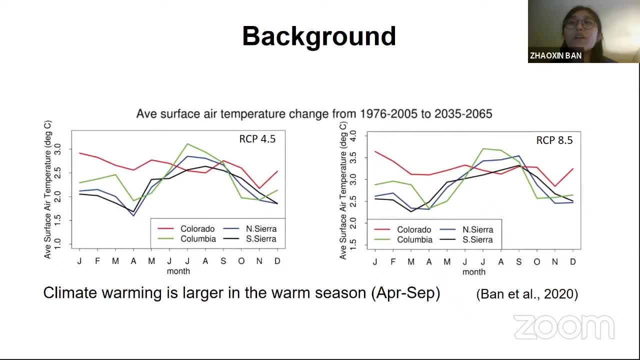 important to understand how and why the streamflow changes under climate warming. The climate warming signal in the Western US is not evenly distributed on a sub-annual scale. The warming in the warm season from April to September is substantially larger than the warming in the cool season from October to March across most of the regions, As shown by the two. 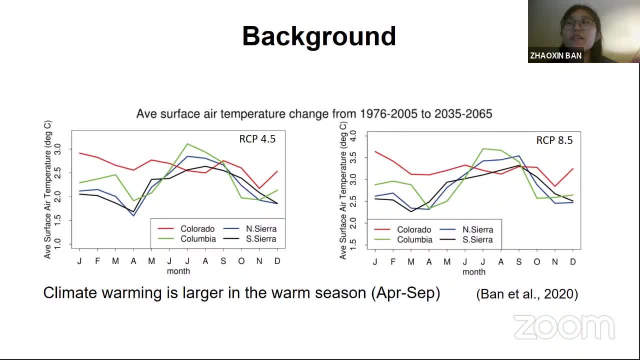 figures. three out of four regionally important basins in the Western US have warming peaks in the warm season under two RCP warming scenarios as projected by CMAP5.. Considering the projected asymmetrical warming pattern, understanding how the seasonal warming impact the annual 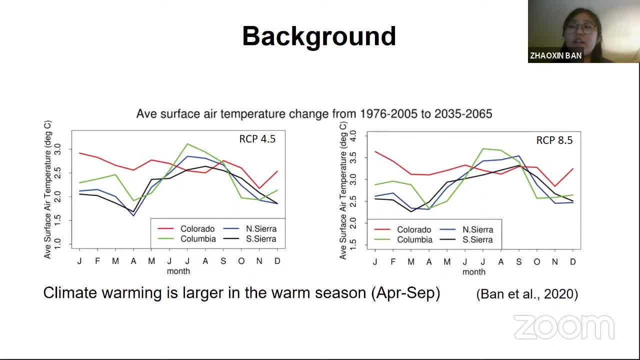 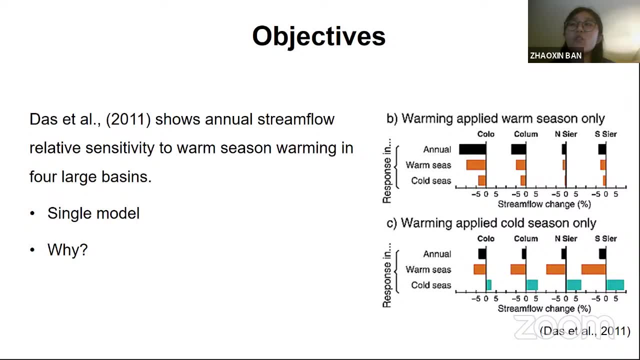 streamflow would be important for understanding future streamflow change. In 2011,, Bass et al discovered that the four basins above generally have stronger streamflow response to warm season warming than to cool season warming, especially the Colorado and the Columbia River Basin. 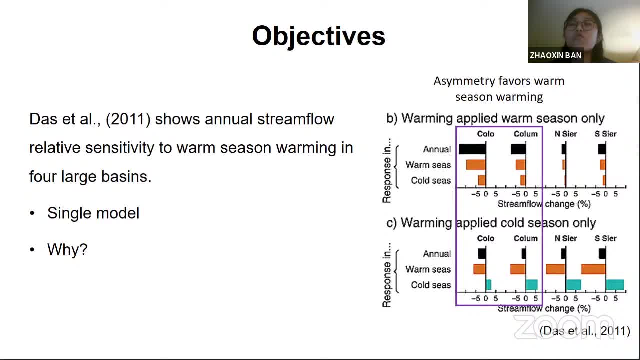 However, the other two basins, North and South Sierra Nevada, does not show such asymmetry. Bass et al did not explicitly explain why the asymmetry differs, and their results are from only one hydrological model, so whether this result is correct or not is not yet known. 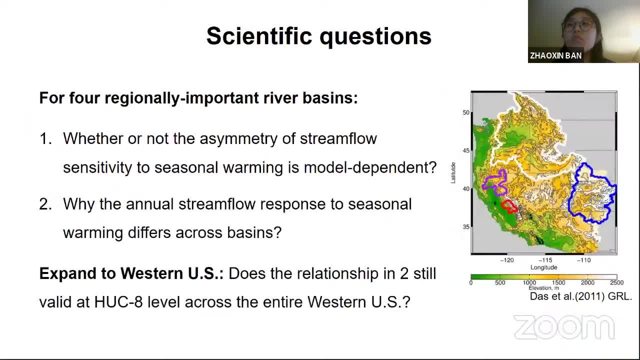 The question is: is the consistent across models still a question Motivated by these gaps? we ask two questions: First, why there are not the asymmetry of streamflow response to seasonal warming as model-dependent. Second, why the annual streamflow responses to 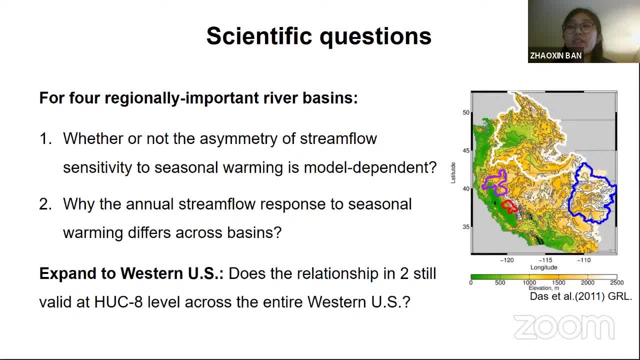 seasonal warming differ across basins. We have a new draft and a review at WRR. We also expand analysis to the entire Western US at a much finer granularity, and I will use some of its results in this presentation too, To answer your questions. we use four land surface models. 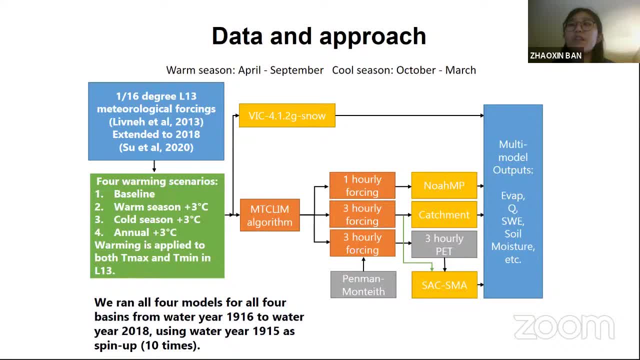 including variable infiltration capacity model NOAMP, Cashman and SACSMA. at advanced 16th degree resolution We fix precipitation and perturb the daily maximum and minimum temperature and the four warming scenarios to isolate the effect of temperature on streamflow. 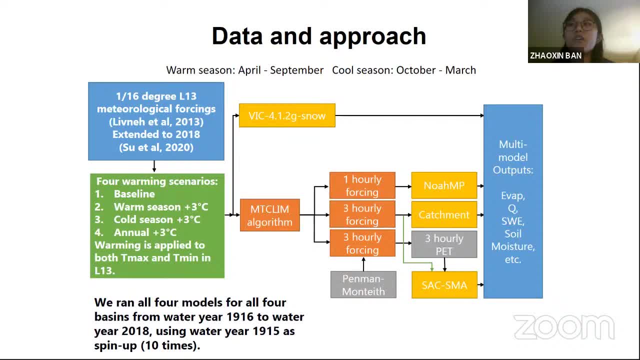 The first scenario is baseline. The second is three-degree warming in a warm season only. The third one only warms the cool season and the fourth one is annual warming. All models are run from water year 1916 to 2018.. 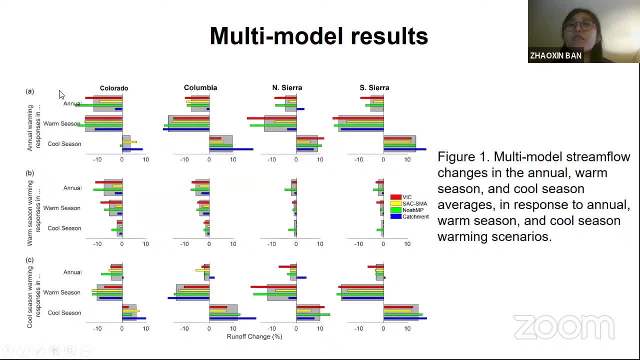 Here are the multi-modal results of streamflow response. From the first to the third rows are streamflow responses to annual warm season and cool season warming. Within each subplot, from top to down, are responses at annual warm season and cool season timescale. 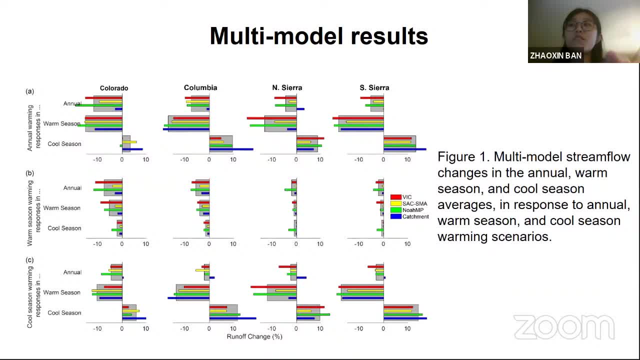 The gray bars are multi-modal mean and color bars are for different models. We can see that, despite the absolute values differ, the models share similar relative magnitude and sign And the multi-modal mean also shows stronger responses to warm season warming in Colorado. 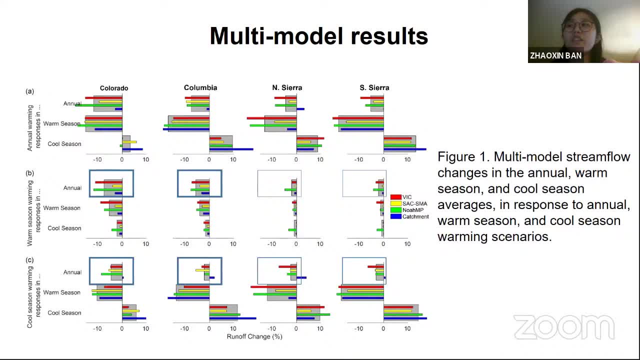 The streamflow response has a very weak or even reverse asymmetry. So here we answered the first question: The streamflow response asymmetries are consistent across different land surface models. Now we answer the second question: Why does asymmetry differ across basins? 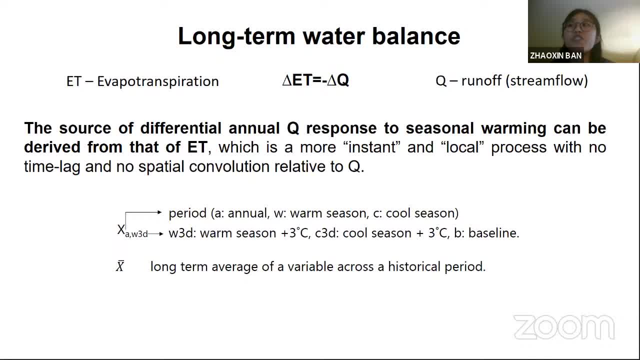 We apply a long-term water balance framework where the annual evapotranspiration change equals the annual runoff change. Therefore, we can explain the annual runoff change by explaining the annual evapotranspiration change, And this makes it easier than directly analyzing runoff, since the evapotranspiration is a more 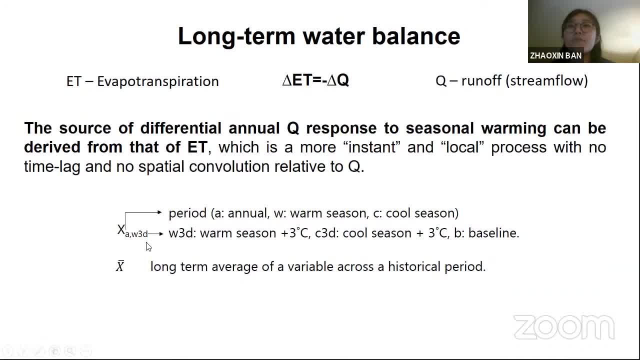 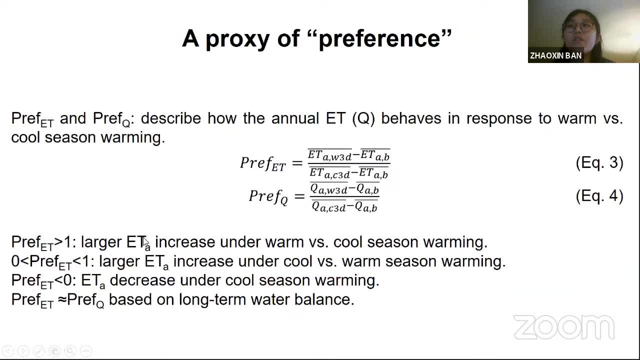 instant and local process than runoff. In the following slides you will see some subscripts. The first subscript indicates the season and the second subscript indicates the warming scenario. With the above framework we can get a proxy of asymmetry, which we call PReF. 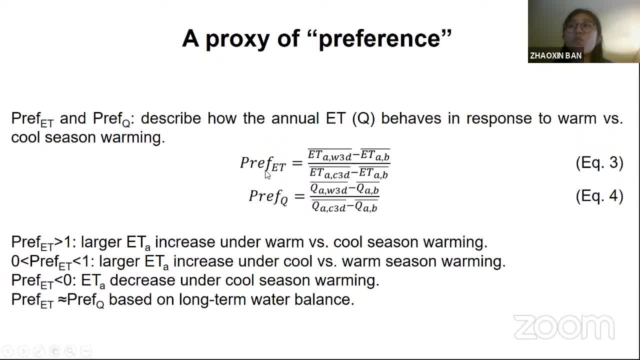 PReFet is calculated as the annual ET change under warm season warming divided by annual ET and cool season warming, And prefq is calculated seen as the change similarly using streamflow. If PREF is larger than one, it means other response happens. 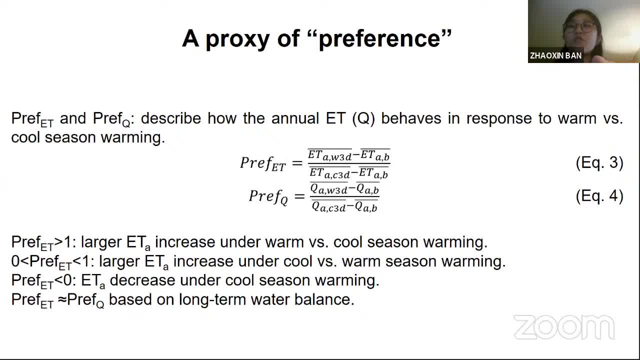 under warm-season warming. If it is smaller than one, it means a larger response happens under cool-season warming. If PREF is smaller than zero, it means the response is under the two warming scenarios. in our experiment to show the different opposite signs in streamflow: 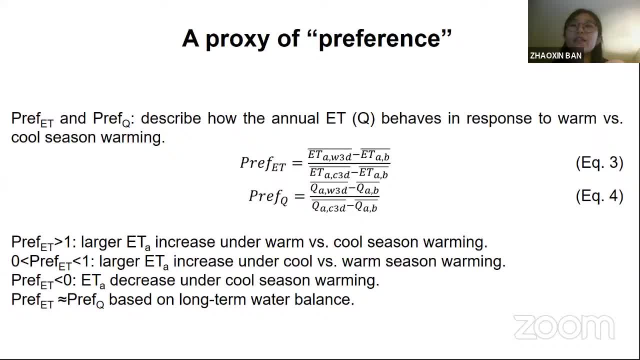 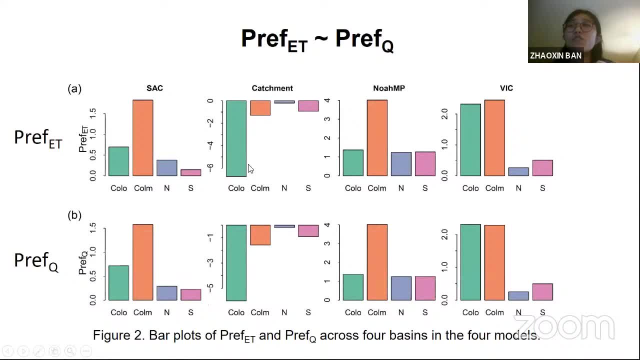 response Based on the long-term water balance, I would expect the PREF-ET to be close to PREF-Q. in any event, And this is confirmed by this bar plot, The first row is PREF-ET and the second row is PREF-Q. We can see that they are very similar. This ensures that we. 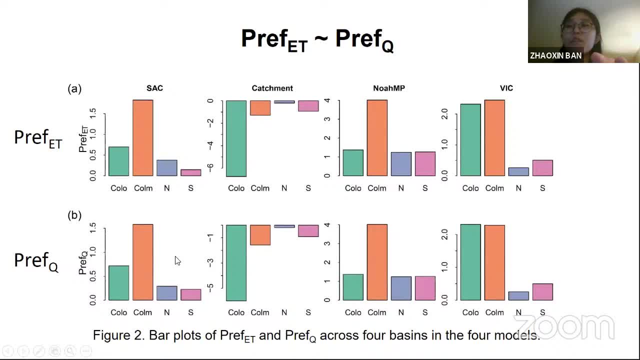 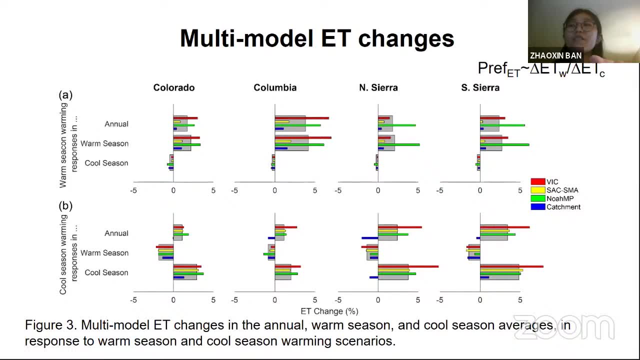 can shift our focus to the variation of PREF-ET, Because the annual ET change is the combined effect of both water and energy supply change. I want to identify if there is a season that dominates the annual ET change. This is the plot showing the ET response to seasonal warming. The first row is ET response to warm-season. 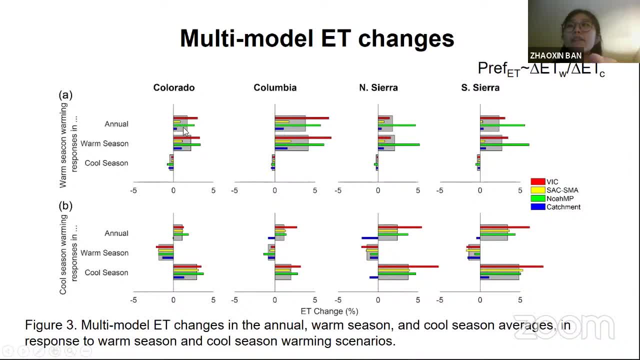 warming, and the second row is ET response to the cool-season warming. We can see that under warm-season warming, annual ET change is dominated by warm-season ET change, And under cool-season warming the annual ET change is dominated by cool-season ET change. Both 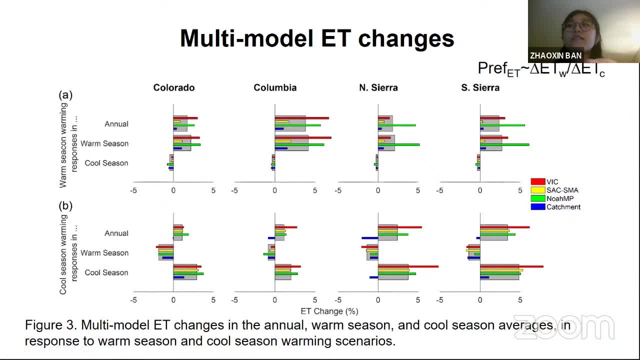 two seasonal ET changes are mostly caused by the season's temperature warming instead of water, because the water availability at the beginning of those warming seasons hardly changes. in our experiment. So we hypothesize that the relative rank of PREF-ET across basins can be approximately equal to the temperature of the water. 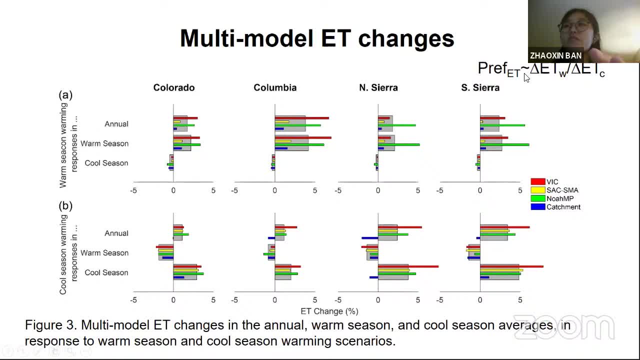 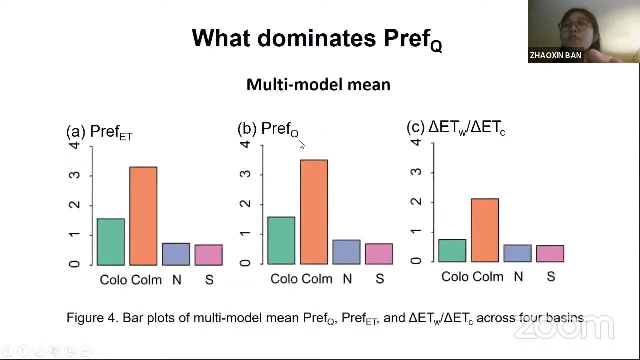 To test this hypothesis, we compare the PREF values under the ETT sensitivity ratio here across the four basins, using multimodal mean. We can see that the three proxies share very similar relative rank. They also confirmed it across the western US at HAC-ET level. 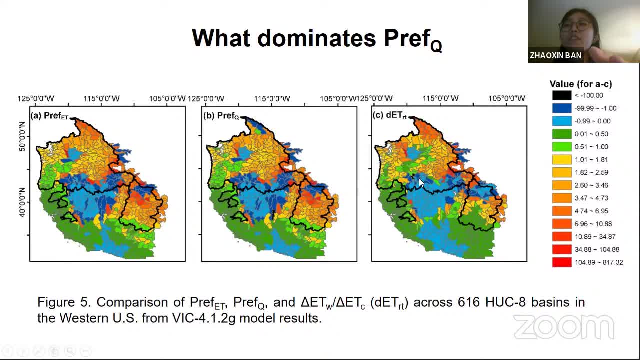 not only in terms of the relative rank, but also in the absolute magnitude. They are also similar, suggesting that the relationship is quite robust. Therefore, if we find what controls the basins' seasonal ET to temperature sensitivities, we can explain why the PREF- and hence PREF-Q- differs across basins. To do this, we choose. 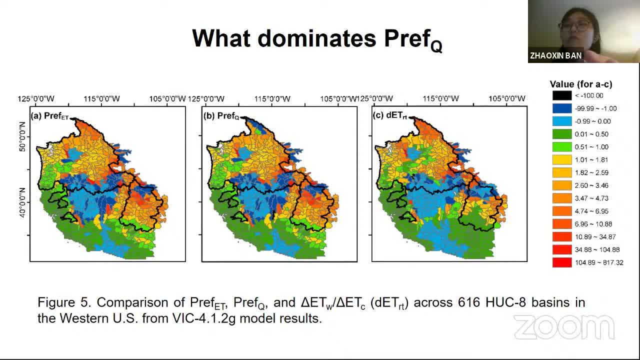 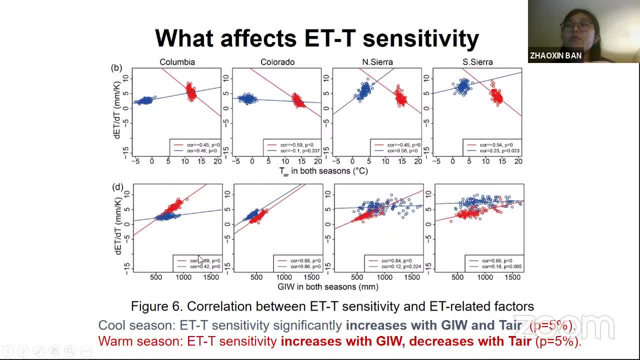 a series of variables related to ET and selected two most representative variables here, namely temperature and GIW. The GIW is gross incoming water defined as a season's precipitation and snow water storage at the beginning of the season. The red points denote the warm. 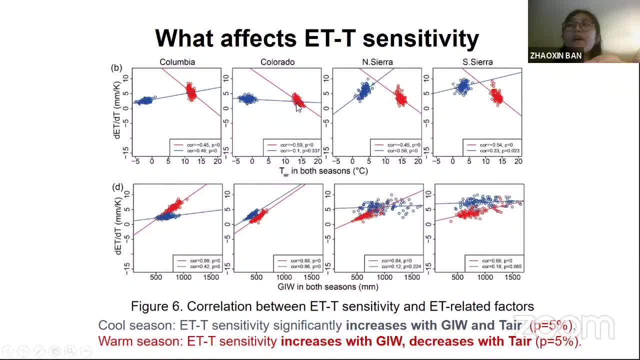 season value and the warm season warming for each year and the blue points are for cool season warming. We can see that for both seasons, the ET to temperature sensitivity and the GIW show both positive relationships, which is as expected, but the ET to temperature. 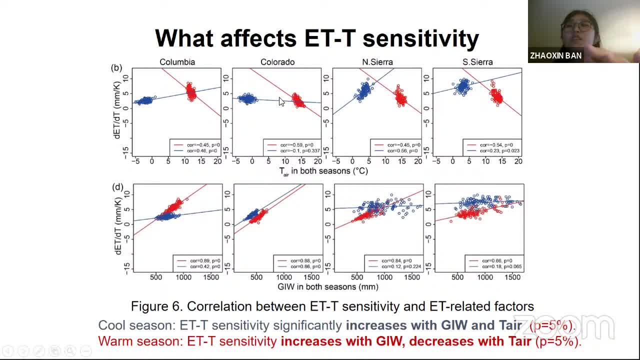 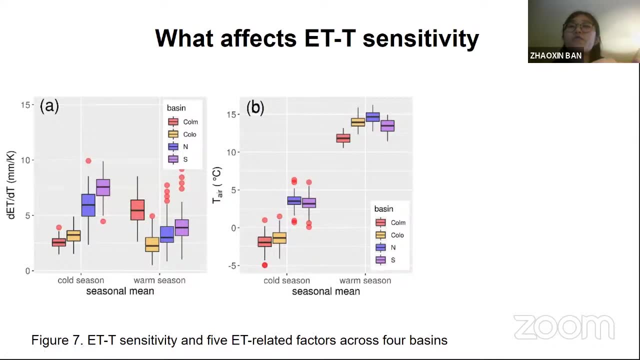 sensitivity with temperature shifts from positive relationship to negative relationship in most cases, which will be further explained in the next few slides. The previous slide showed the relationship within each basin across different years and this slide compares the relationship between the variables across different basins Under cooler temperature. 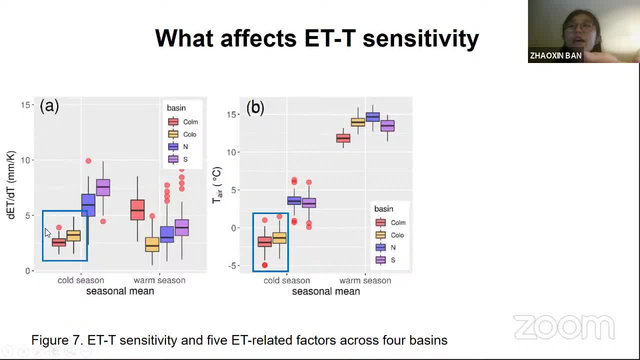 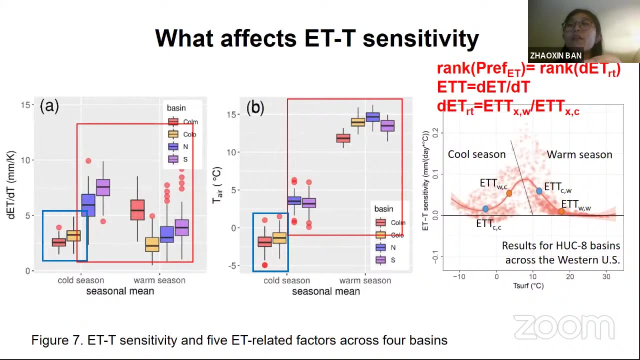 in the cool season the ET to temperature sensitivity increases at basins with higher temperature, while under a warmer temperature the two variables show opposite variation. Another look at this relationship across the entire Western ULSS also shows the first increasing then decreasing pattern. This pattern has an important indication, For example. 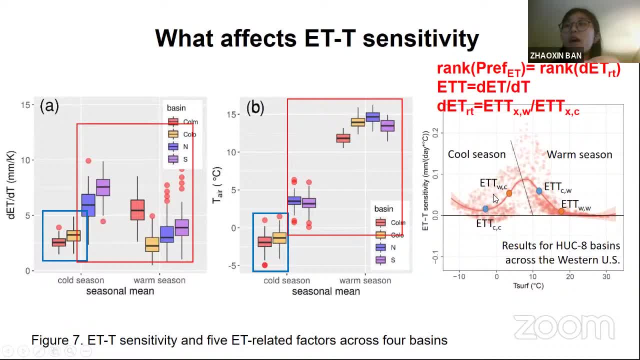 in the red figure. the blue points represent the cooler basin and the red points denote the warmer basin. The cooler basin has generally cooler temperature, so it has higher ET to temperature sensitivity in the warm season and lower ET to temperature sensitivity in the cool season. Therefore, the warm to cool season ET to temperature sensitivity ratio. 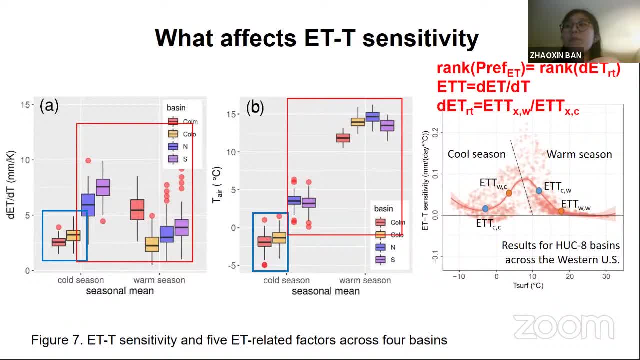 for the cooler basin is larger, since this ratio is describing the response symmetry. higher ratio also means that the cooler basin responses have a stronger preference for the warm season warming. Such cool basins are exactly the Columbia and Colorado among the fours. answering the second question, Before I explain the ET to temperature sensitivity, 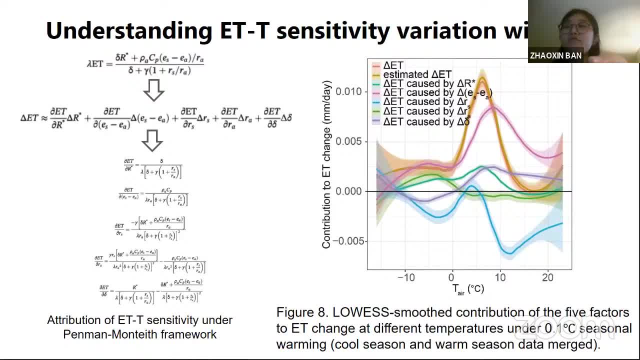 thank you. variation with temperature. by attributing the seasonal ET change to five processes using the permanent taste framework as shown in the red figure, the red curve is model simulated ET change and the brown curve is the sum of the five individual processes. contribution, We can see the increasing part of ET. sensitivity to temperature is mostly. 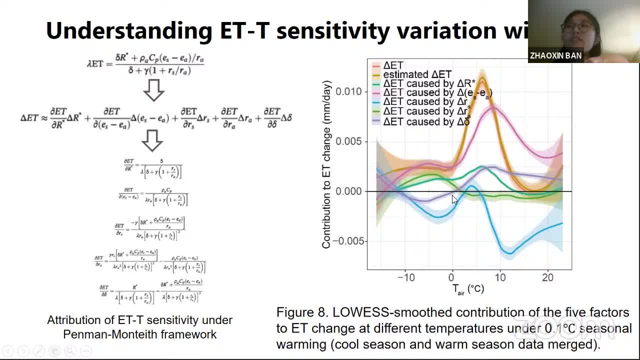 contributed by the pink and the purple curves, which are reflecting enhanced the rate of water vapor holding capacity increase And the decreasing part is due to mainly the blue and the ZN curves. One is the increase in surface resistance and a higher rapid pressure deficit. Another is the 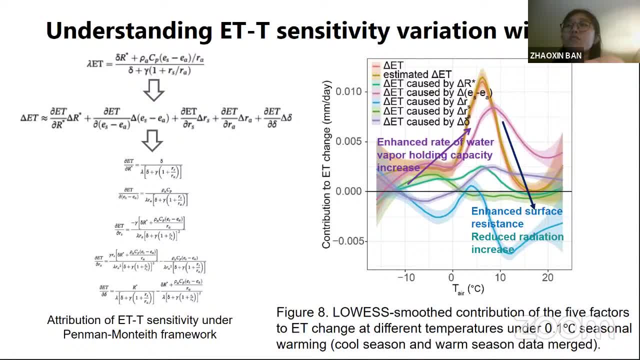 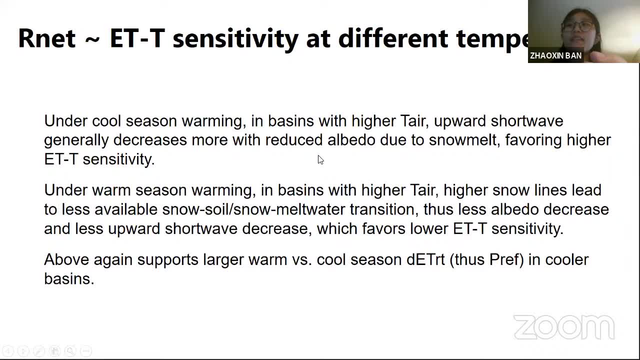 snowmelt albedo feedback, which causes less radiation increase when there remains less snowpack. Some other complex reasons. please see our paper at the end of presentation. We also discussed the effect of radiation on ET to temperature sensitivity. I only show the main conclusion here due to time limit. 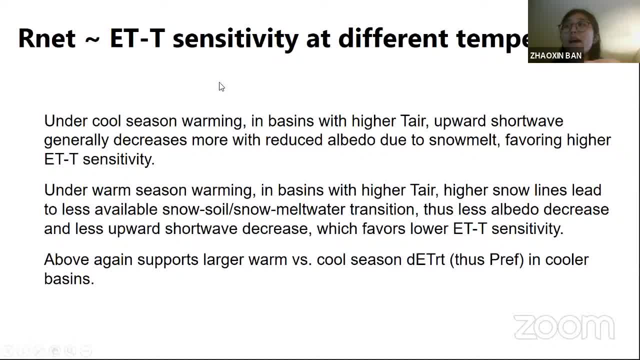 Under cool season warming the warmer basin tends to melt more snow and has larger albedo decrease and radiation increase, leading to a larger ET to temperature sensitivity. Under warm season warming a warmer basin generally have less snowpack remain, so less albedo decrease occur under warming, leading to a smaller ET to temperature sensitivity. 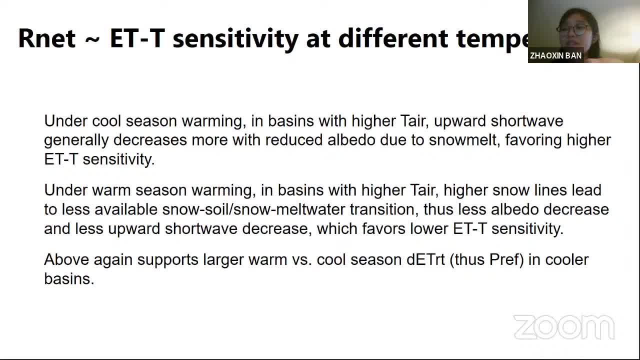 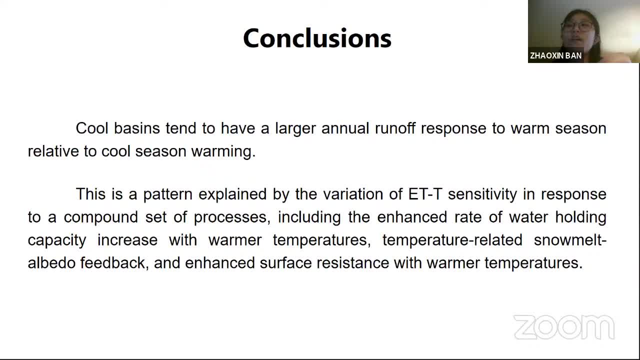 than a cooler basin. These results are consistent with our findings in previous several slides. In summary, we find cooler basins tend to have a larger annual runoff response to warm season relative to cool season warming. This explains why the Colorado and Columbia River basin has a stronger streamflow decrease under warm season. 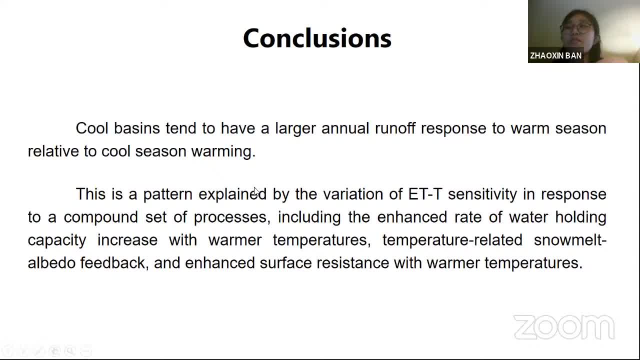 warming. This pattern is explained by the variation of ET to temperature sensitivity in response to a compound set of Lansan first stasis, And it has implications for better understanding the future streamflow change under an asymmetrical warming future. Here are my selected references And that's all. for details, Please see. 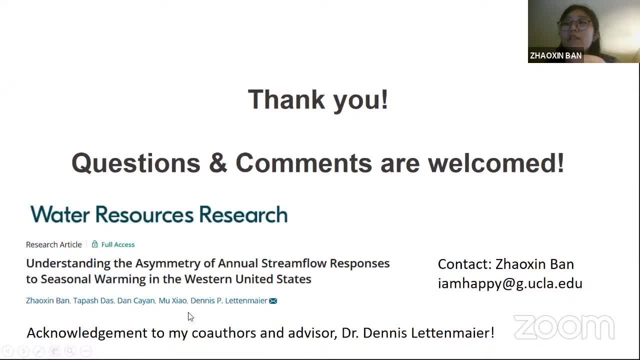 this paper or contact me directly at this email, And I want to thank my co-authors and my advisor, Dr LeTang Mayer, And finally, thank you. all. Questions and comments are very welcome, Thank you. Thank you, Any questions for Xiaoxin? 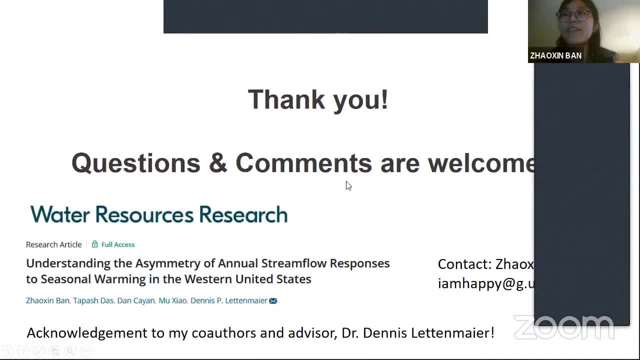 Do you have a question, Flavio, or you're just clapping? Sorry, Sorry, Sorry, Thank you, Thank you. Yeah, I wanted to both clap and raise my hand. Yeah, Very nice presentation, Thank you. Yeah, It's really convincing, I think. the only question I had like: do you have these? 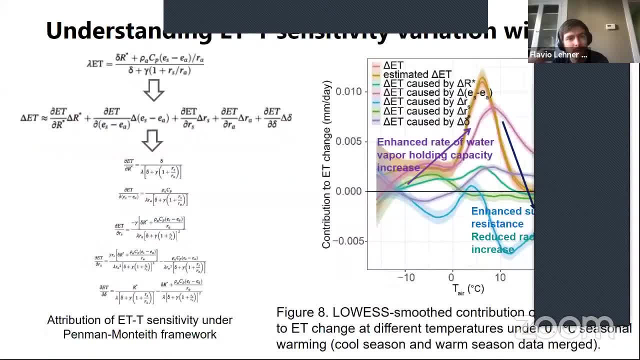 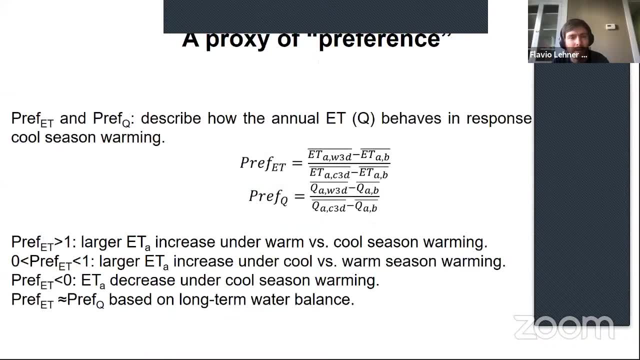 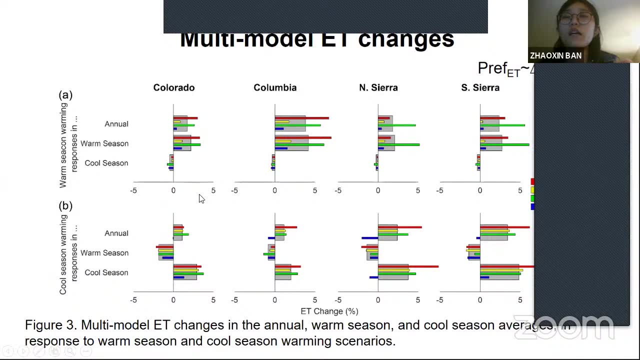 sensitivities. I know a little bit about them from trying to estimate them from observations, and it seems very difficult. Do you feel like the models are more or less in the right ballpark And like, how would you conclude that? Do you mean the uncertainty, or how should I? 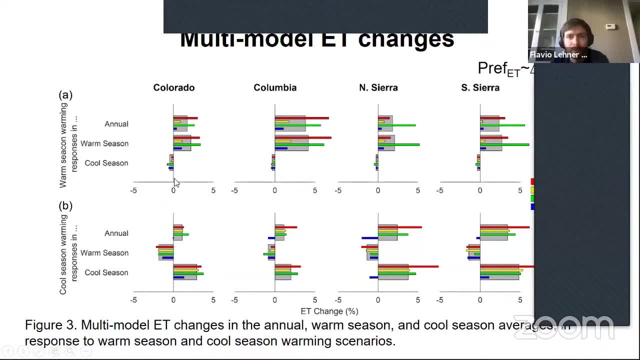 Yeah, Basically, yeah, Like what's the real sensitivity, Like from the real world? Okay, Okay, I know it's hard, Yeah, So, yeah, I'm using the model. Yeah, I'm using the model in this paper And we can see. 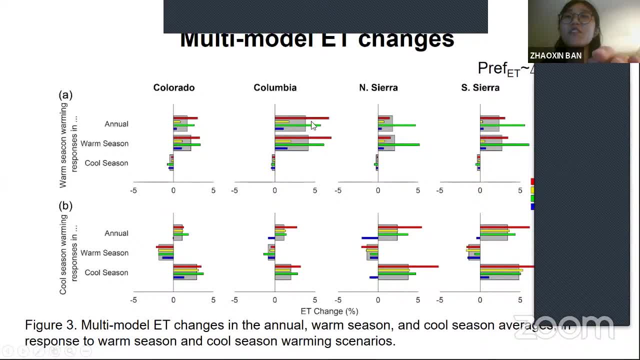 they, this model, have some uncertainty in their absolute magnitude, And the thing for my work is those models are calibrated in stream flow and the precipitation comes from the, from the stream flow, because we want to generate about or create some kind of 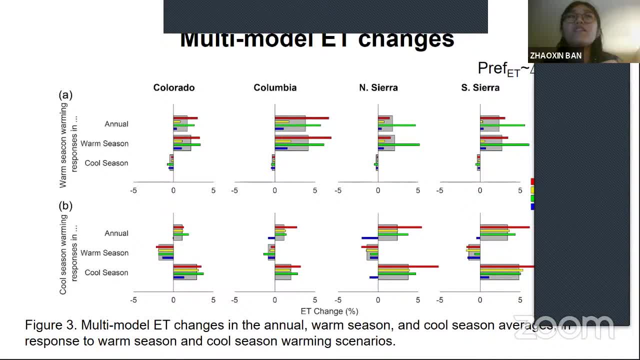 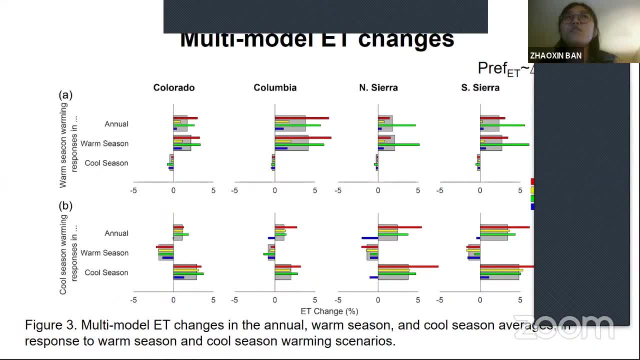 There are some water balance closure, budget error, and it is also hard to explain whether the evapotranspiration measurement is correct or not. The only thing we can kind of use may be the flux towers that can measure the evapotranspiration, and we can use the temperature measurement too and the precipitation and so on. 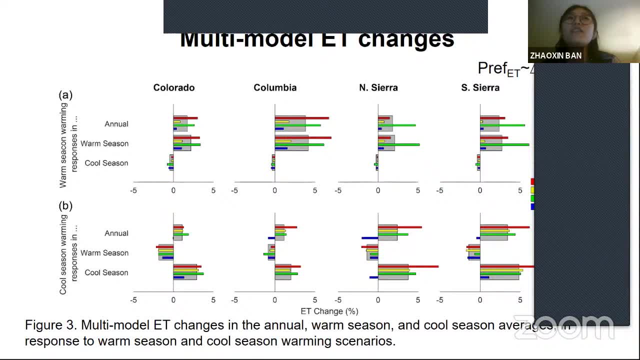 But I'm not quite familiar in that field. but to constrain the variability, I believe there are many methods that can combine with different models, For example the observation constraint sensitivity analysis. if we can find the evapotranspiration to temperature sensitivity is having a good linear regression relationship with another variable that is observable in the different observations. 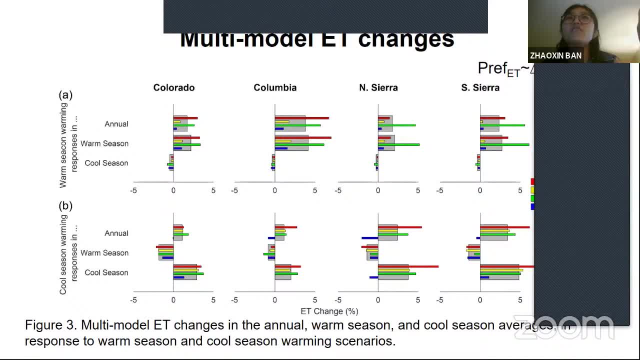 and this relationship is maintained across different electrons. So we can constrain the distribution of model-simulated sensitivities using the observed variables to see a more realistic estimation of the evapotranspiration. Cool thanks, Thank you. Okay, thanks, So we just have 10 minutes left of the actual session, so we'll use this for some discussion now. 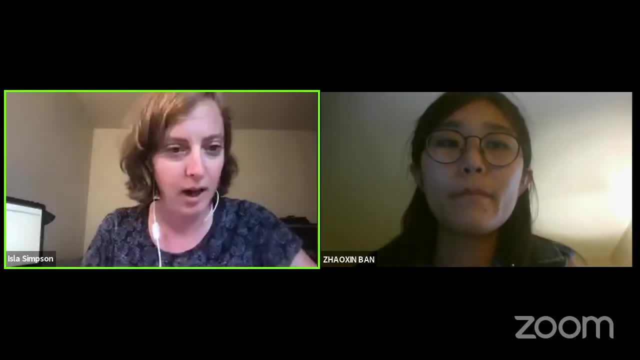 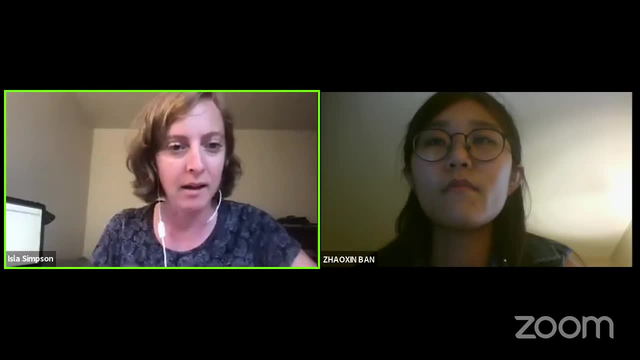 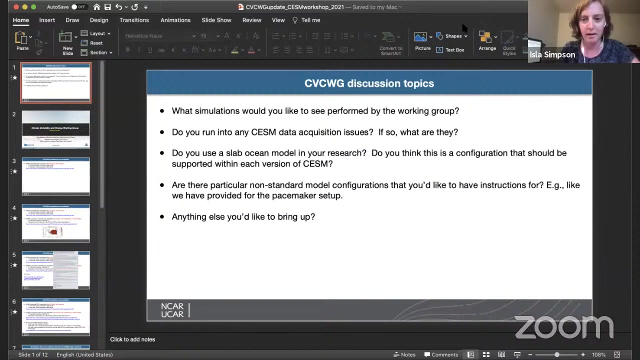 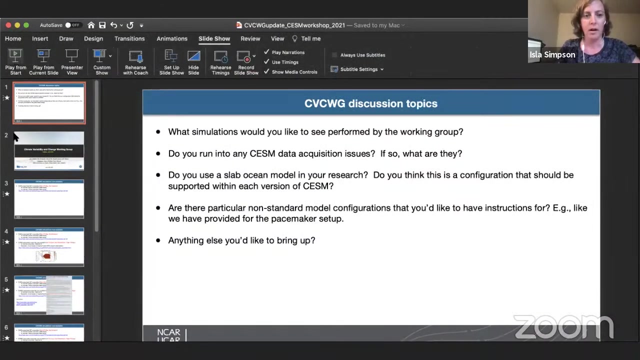 Okay, So we have. we can really talk about anything. now I won't go through kind of an update because we already did that on Monday, But I have these discussion points, But we can talk about anything if anyone wants to say anything. 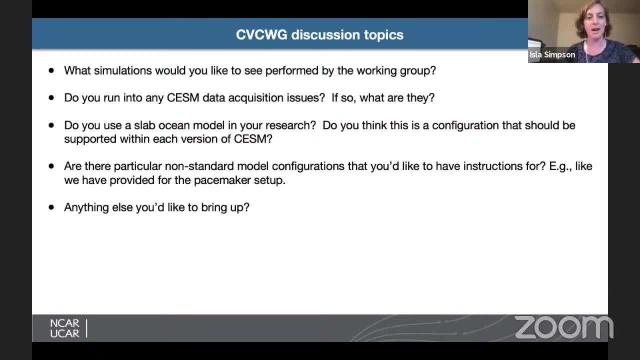 So some questions, though. that we thought Might be interesting to discuss is the usual one of what simulations would you like to see performed by the working group? At this point. we're kind of in the middle of the allocation cycle, so we don't need to write our proposal this year. 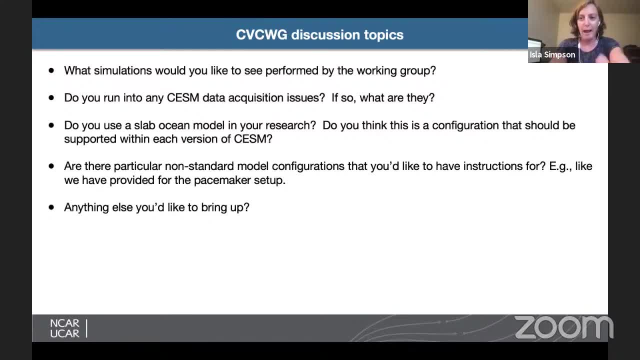 So next year will really be when we'll need to think of new plans, But it's always good to keep ideas coming in case we have extra computing time. If you have any issues that you run into in getting CSM2 data or CSM data. 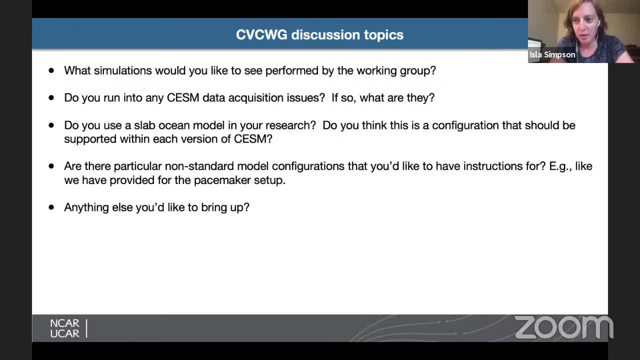 you can please bring them up. One question we thought maybe needs to be addressed- because a number of people, I guess, have asked me about this, And I know Sarah as well- is we currently don't have a slab ocean that is supported for CSM2.. 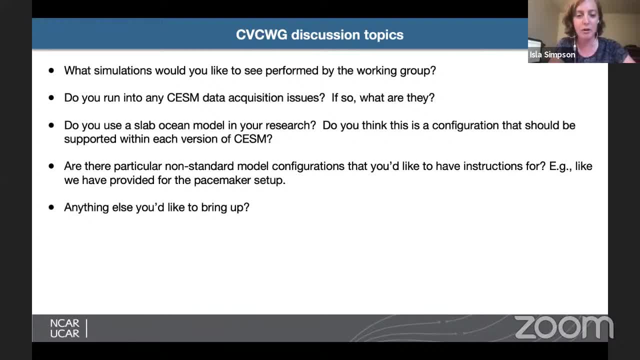 And the working group is going to perform, instead of the slab ocean, pre-industrial control where the plan is, as Yangu Kwan is running, a pre-industrial control with this new pencil model, which is basically a mixed layer physics at every grid point. 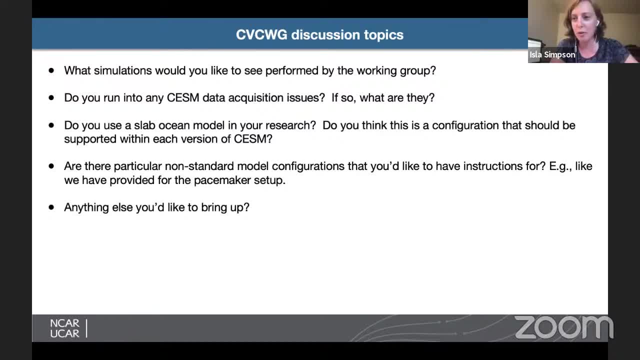 So one question is: do you think we should- all we should, should people be continuing to use slab oceans, And do you think this is something that should be supported for each CSM version? Are there any particular kinds of experiments that you'd like, that you've seen people do that you'd like to know how to do them? 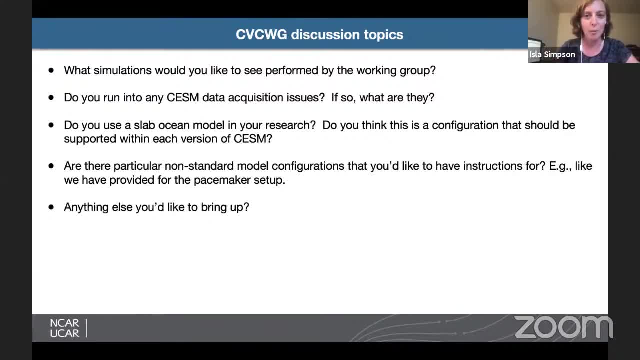 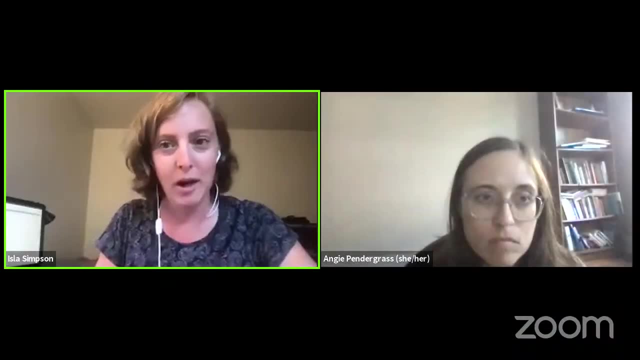 And is there anything else that you'd like to bring up? So I'm going to stop sharing, just so I can See everything. so hopefully you can remember these thoughts. Does anyone have anything they'd like to say? If not Daphne, I don't know. if you feel confident about the poll, we could give it a go. 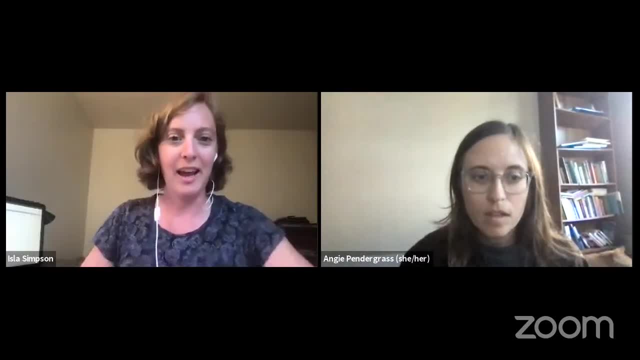 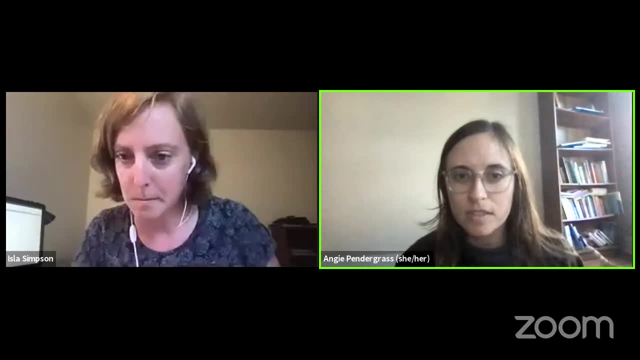 I can try to set it up while you guys talk. OK, Hi, this is Angie. I was just going to say I was just saying in the chat that I'm using some aqua planet slab ocean version of something similar to CESM2.. 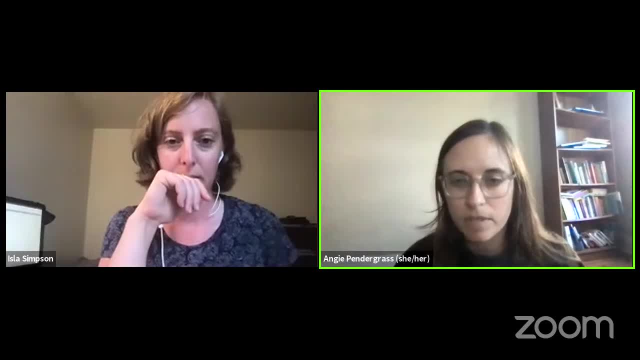 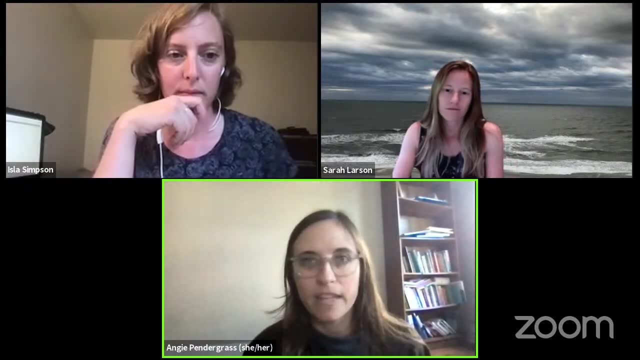 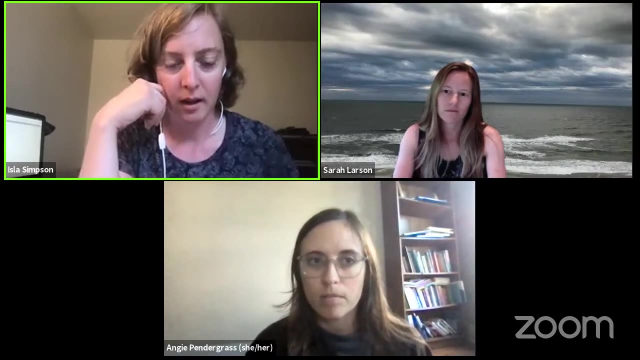 It might be CAM6 beta, the beta release of something that I got from Brian Medeiros, But I'm using that for these ITC ZMIP simulations And I think it's really valuable to have the slab ocean configuration, So I would be in favor of keeping that around. 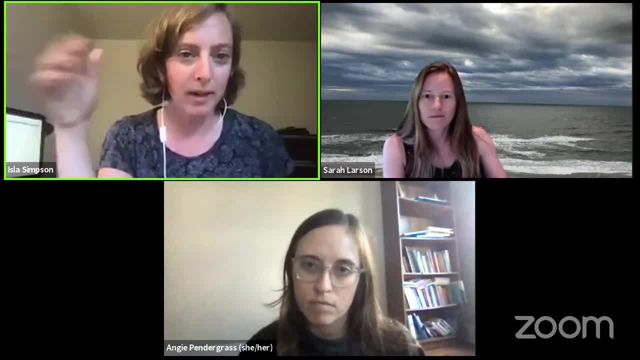 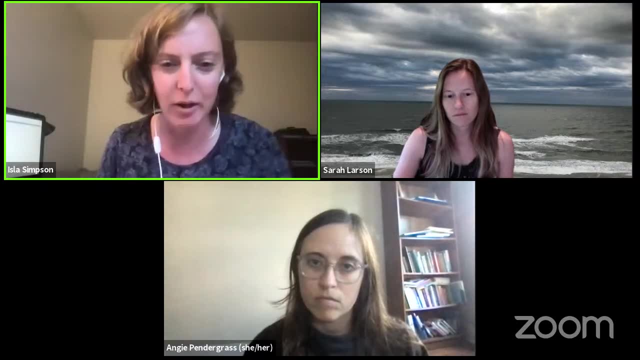 Yeah, I think it's the getting the Q fluxes for the more realistic version. I know that Cecile knows how to do it And I know that it's not totally straightforward. I don't think she's here because she was in the other session. 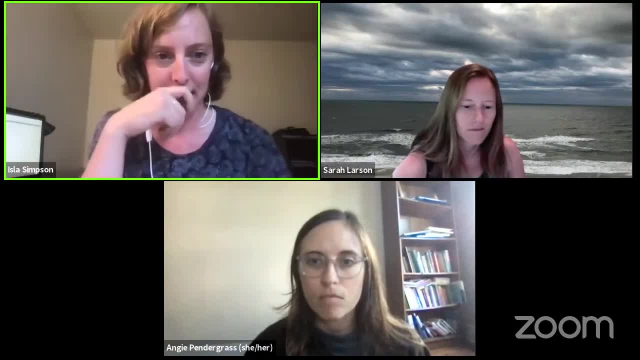 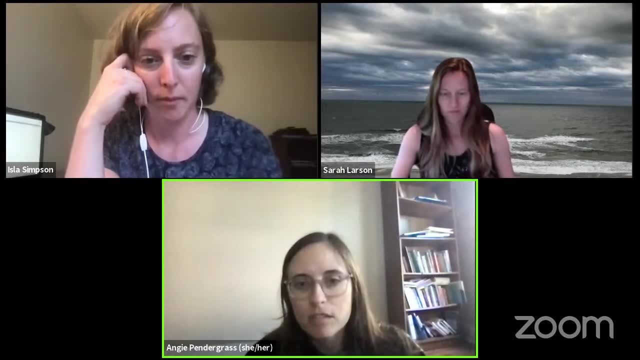 But it sounds like something that could be done and provided if there was a demand for it, for the kind of real world situation. I mean, I just generated Q fluxes. You start with the prescribed sea surface temperature simulation and then you generate Q fluxes. 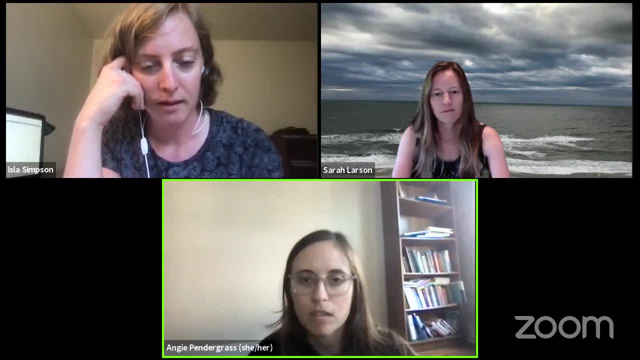 And it's not. I don't think it's that hard And it's also something that could be. I mean, I think I got Jim Benedict had a script for it. I think I got Jim Benedict had a script for it. I think I got Jim Benedict had a script for generating those that I use. 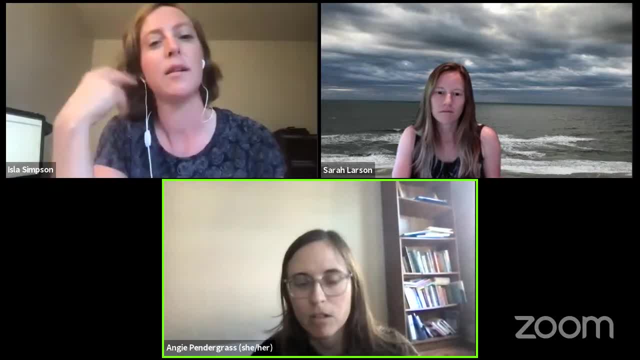 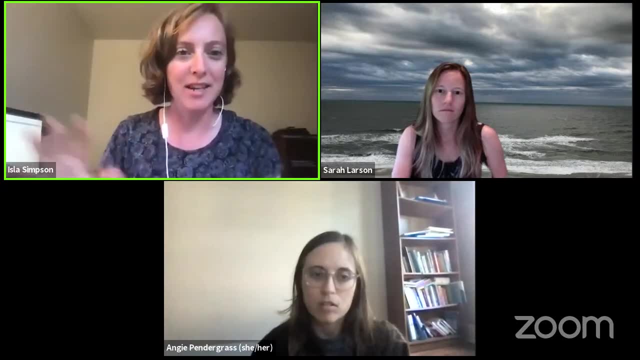 But yeah, I mean I think that that should be feasible for realistic configurations too. I don't know if other people find it valuable. I think it would be a case of like coming up with kind of the default Q fluxes, and then the tools may be more documented so that people can make their own. 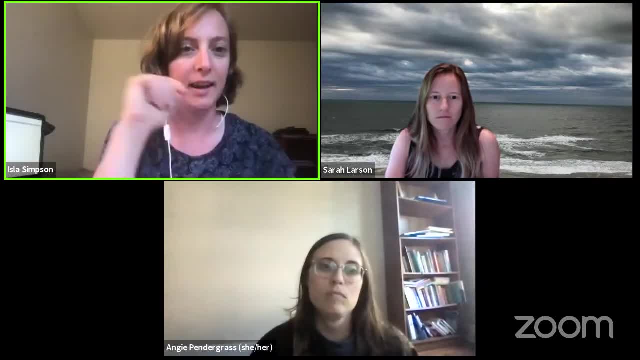 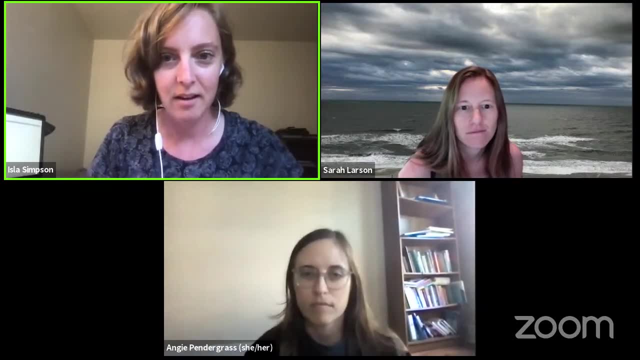 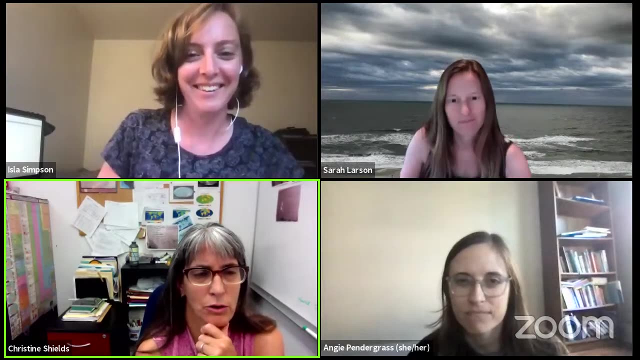 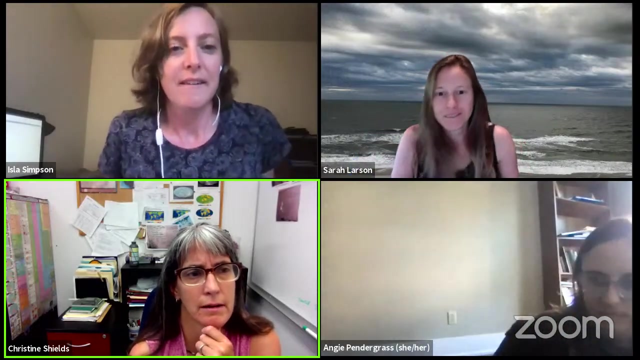 Ayla, I can launch the poll whenever you're ready. Okay, yeah, go for it. Not surprising, I'll add, about the aqua plant and computing Q fluxes. I've done this for a paleo configurations and there is supported tools for that. 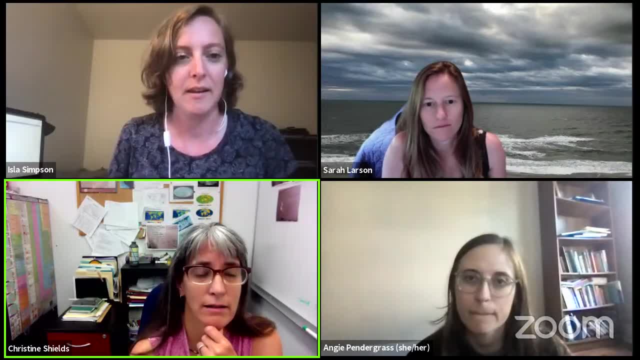 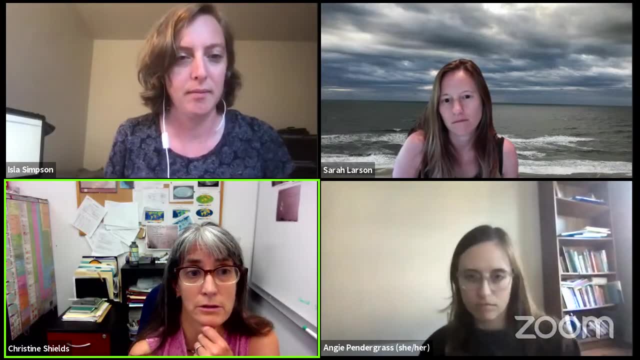 Yeah, I agree with Angie that I it's not. I mean it's. it takes a little work, but it's definitely something for people who want to use it. it's a valuable tool to keep around, And the tools I think are there. 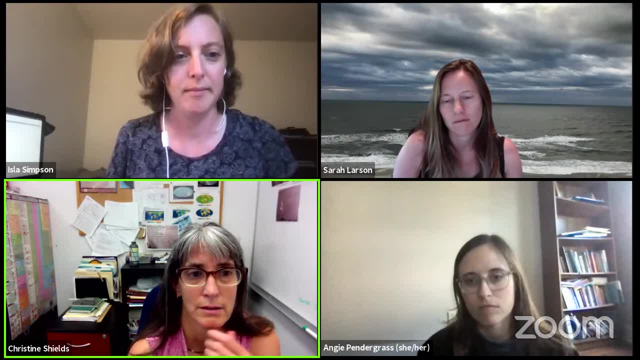 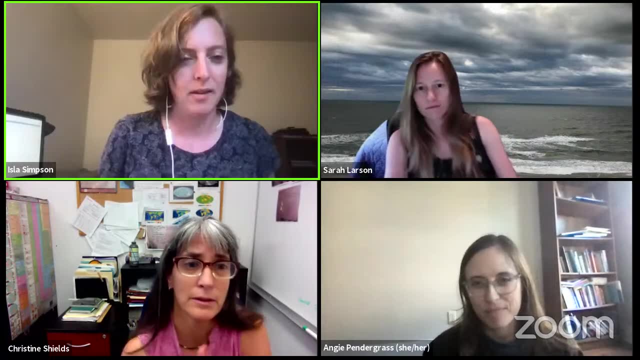 And if they're not perfect for sea surface, And if they're not perfect for sea surface And if they're not perfect for sea surface, Okay, I guess I'll add to that, like if I can't see them, like if they're not, if they're not, Ihave any resources into. 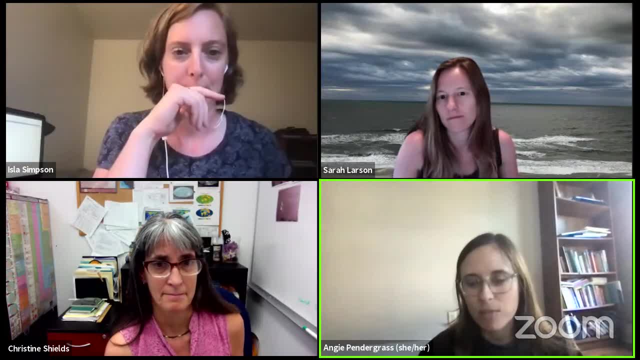 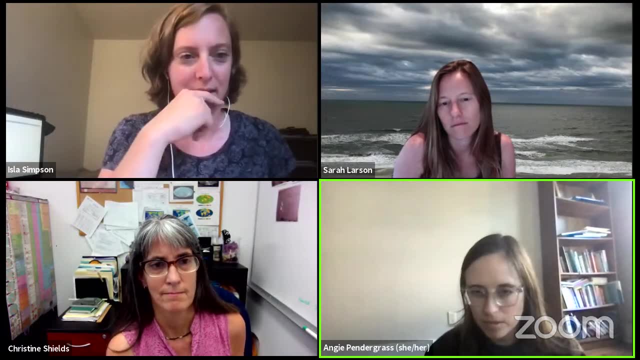 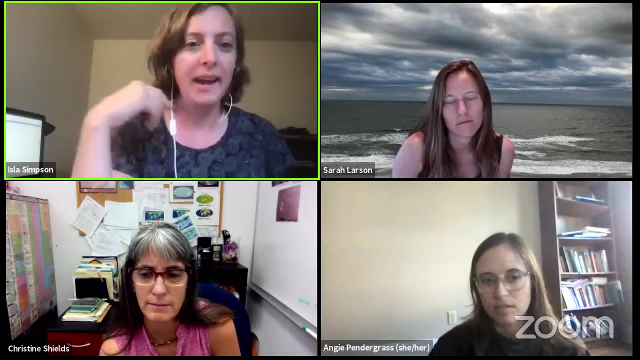 You know, I don't see why they could not be made. you know, with software and generic help. It might be useful to place it in the context of, like: what are the competing priorities that were, with those resources be dedicated? if they weren't, would they be dedicated to the pencil model configuration, because that would be new and cool and so something different. 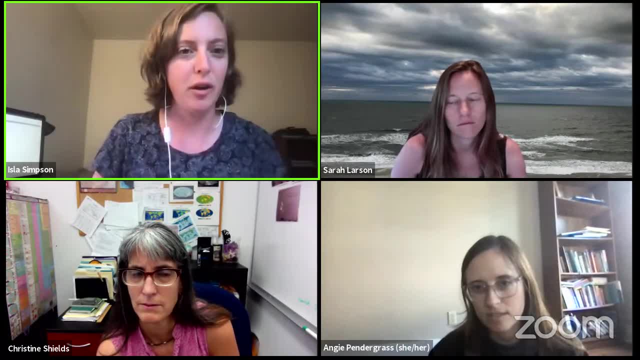 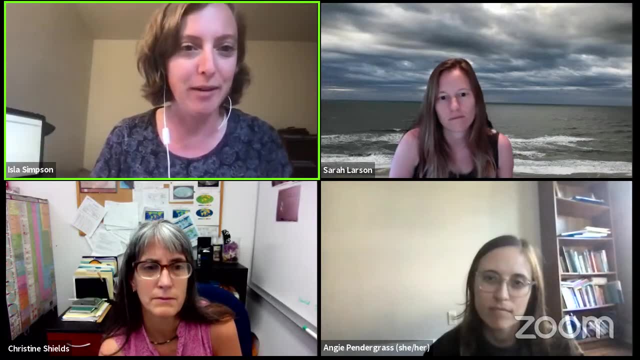 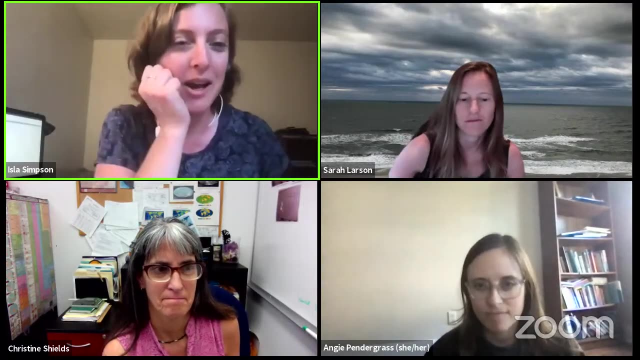 this is more. yeah, resources are already dedicated to the pencil model. i guess this- this would maybe be me talking to cecile and trying to write a website that would, um, yeah, set it up. but so if there's, if there's a lot of interest in it, maybe 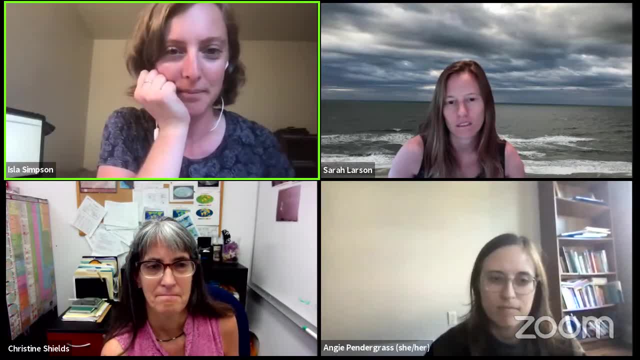 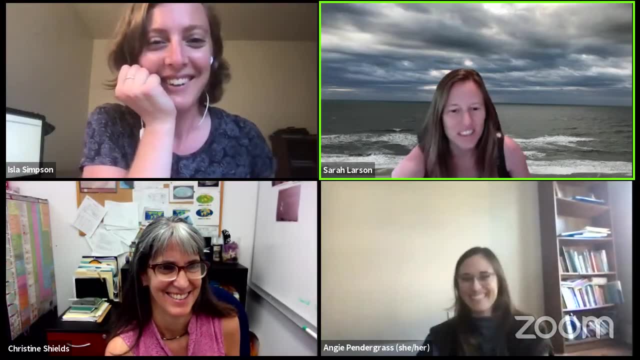 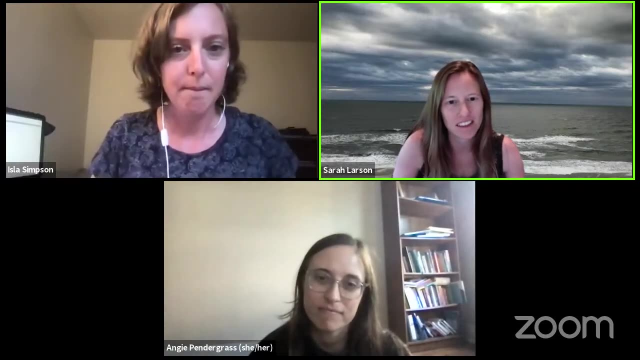 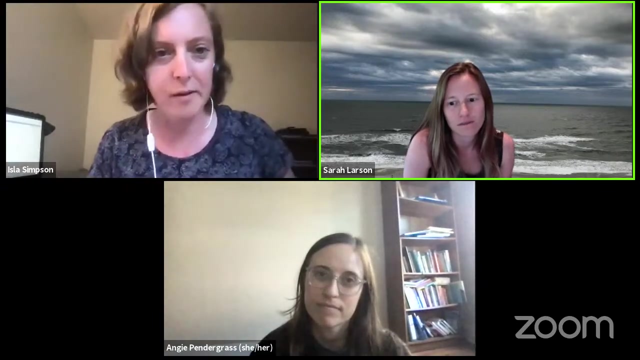 yeah, it wouldn't be too difficult because i also like isla's papers. i love to have an idea of the um, the timeline for the pencil model output. i know there was a question in the winter meeting but it sounds like it's moving forward now. so i don't know if youngo is on this, but i think last i heard i emailed him a couple of weeks ago. 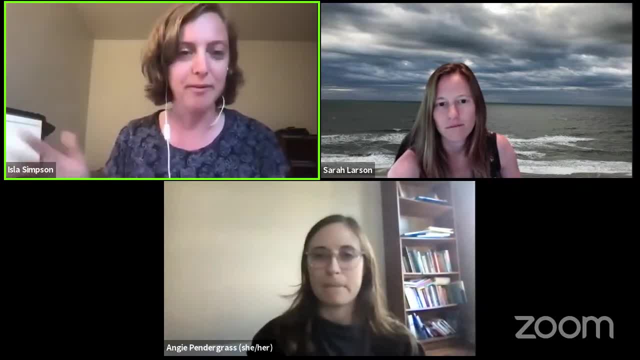 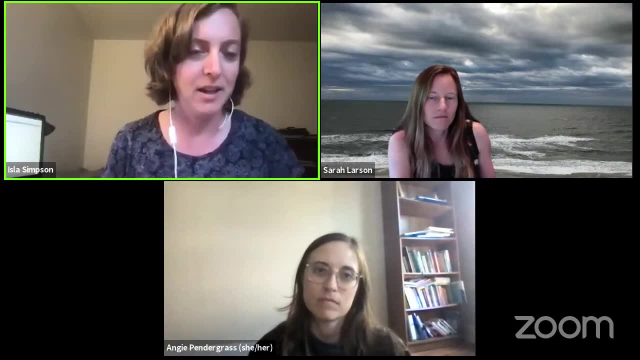 and they were just kind of seeing if the pre-industrial control was stable. and so i emailed him a couple of weeks ago and he was like i don't know if it's stable, it's. he signed it positive that he would use up the computing time that was allocated before the 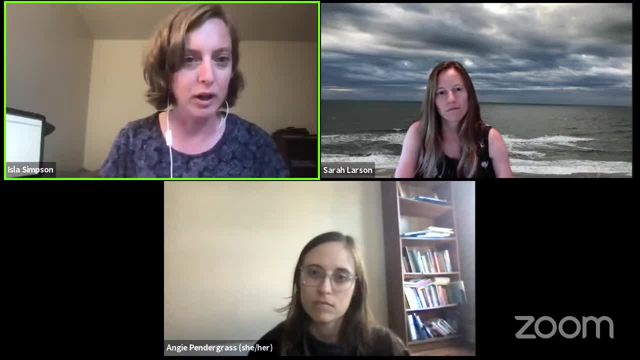 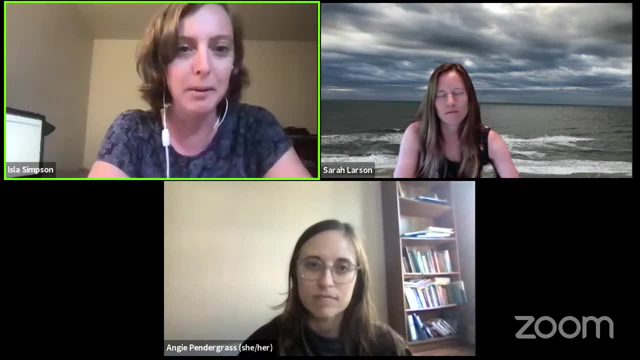 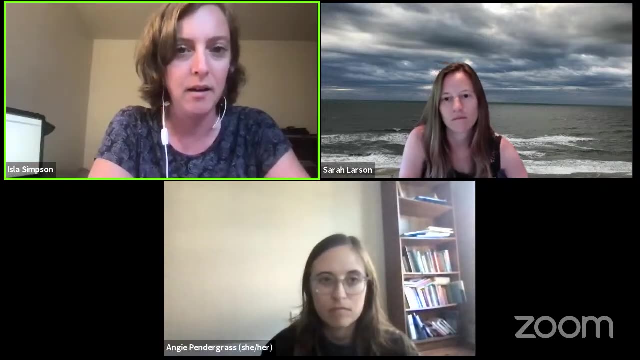 fall. so that would be for the pre-industrial control. and then i don't know if they have plans to um write a paper first, but i think it probably expects sometime later this year- or early next year would be my guess, if everything goes to plan. okay. so it seems like no one does not want. 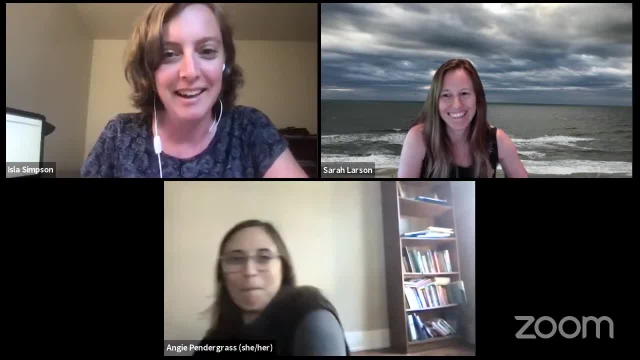 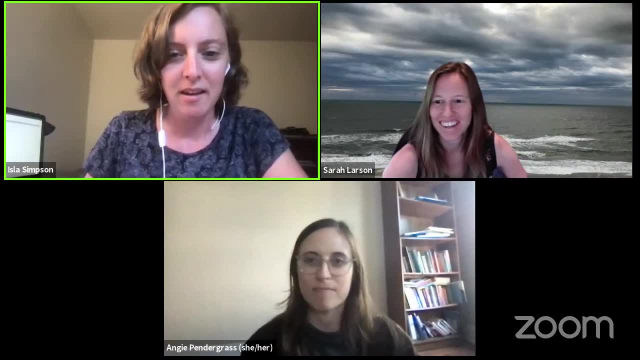 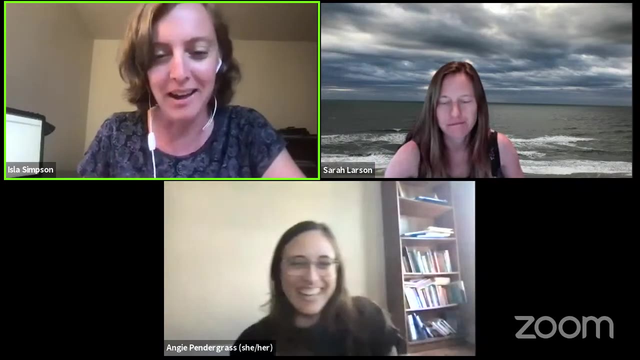 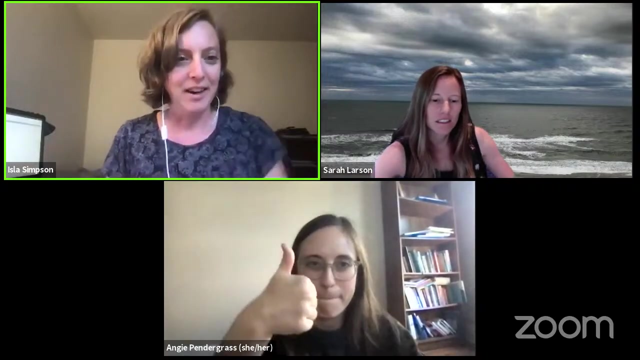 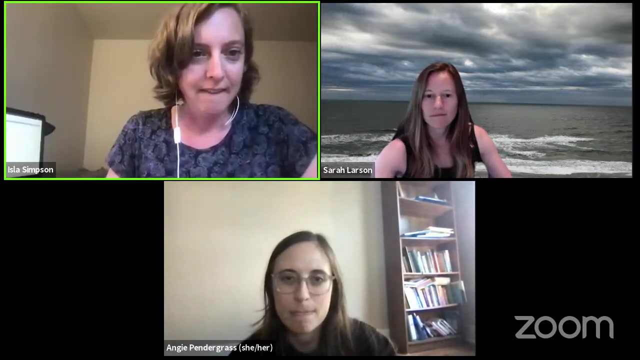 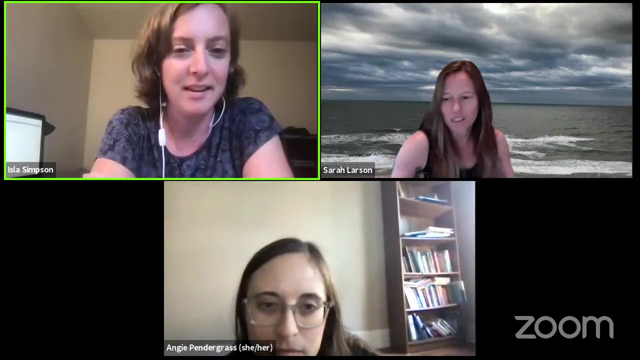 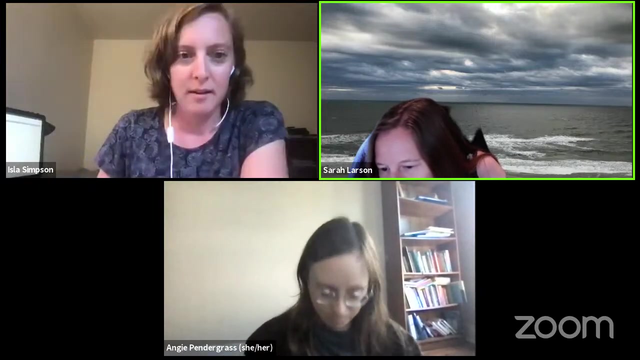 a slab ocean model. okay, 71% do so. that's. that's pretty clear. i don't know. yeah, i feel that did something. i just shared the results. okay, let's stop. all right, does anyone else have anything you'd like to say? there's a question in the chat is: is the gray radiation model implemented in the new cesm? 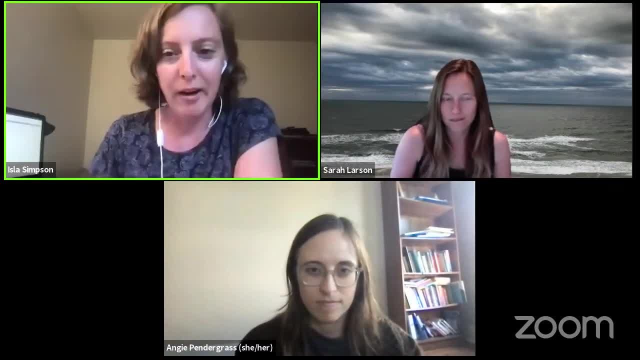 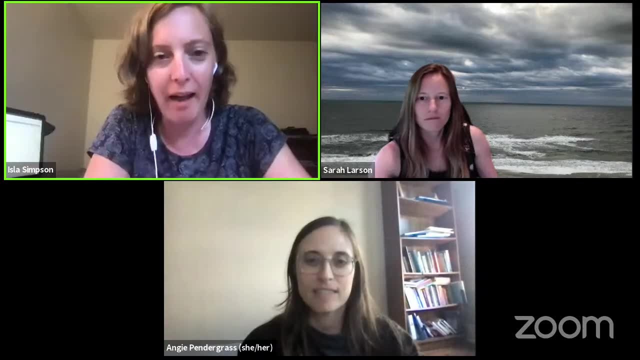 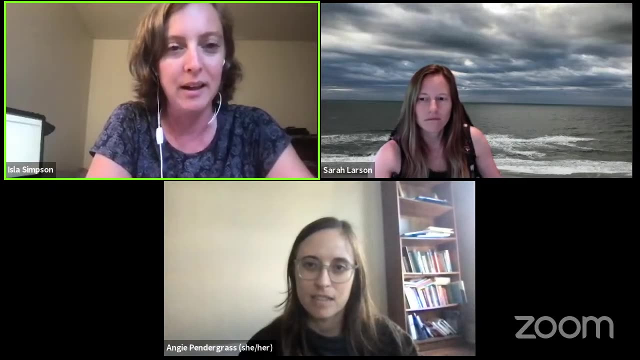 release um kind of it's. if you want it, you can definitely get it. um. so yeah, patrick callahan has implemented it. it just it hasn't been engineered into a release for the new cesm branch fully at this point and the software engineer who is going to do that is busy with 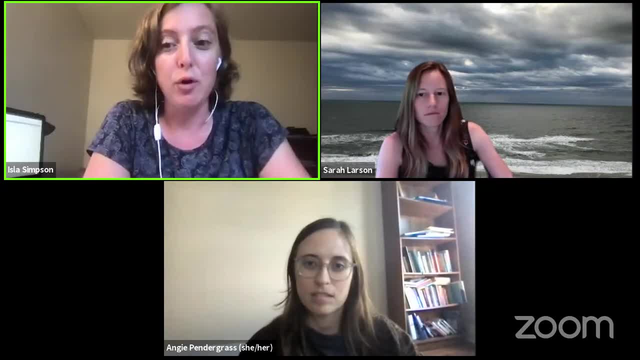 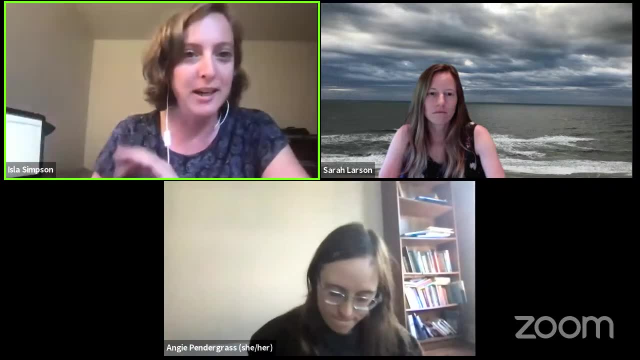 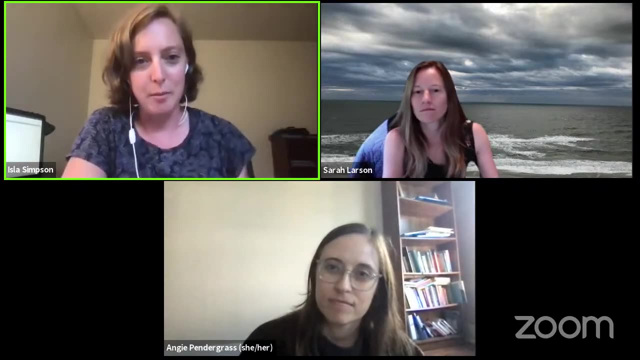 other things. so, um, if you want to use it, you can get in touch with me and i can find out what version on github you you need to download to be able to use it, but it should be coming at some point. it's not in csm2 at this point though. 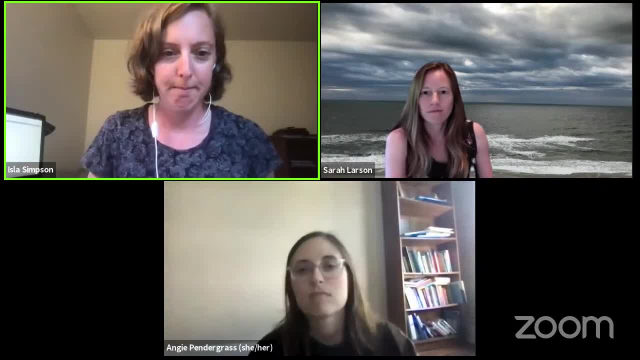 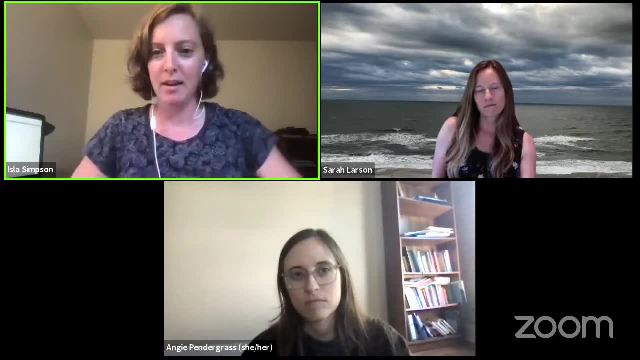 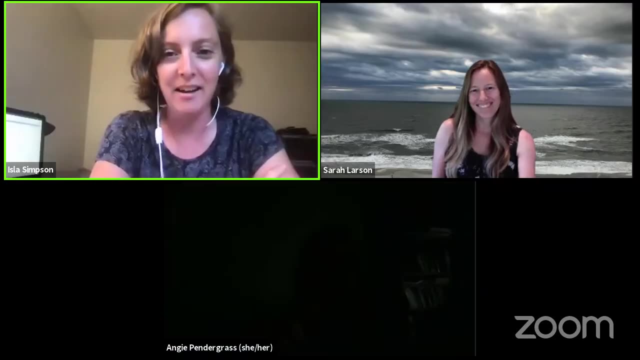 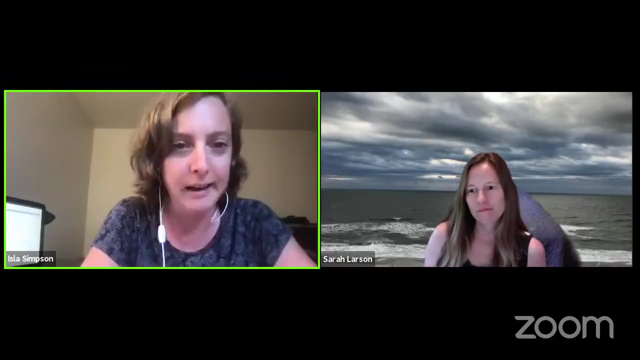 i hope everyone's going to go away and analyze the csm2 large ensemble now. lots of data and yeah, in case anyone missed it, there's. the working group is producing a single forcing large ensemble as well, and the ssp245 ensemble is there too. um. 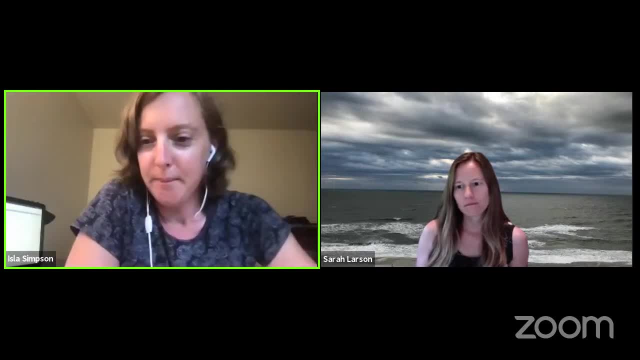 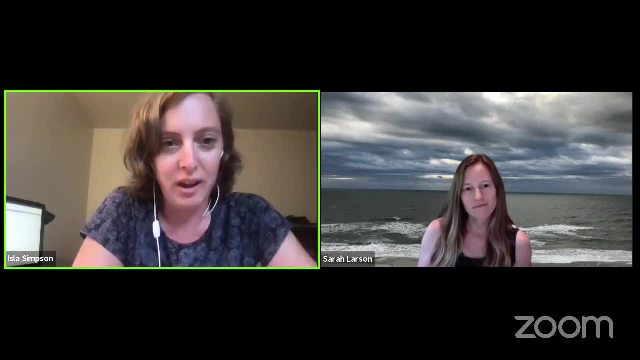 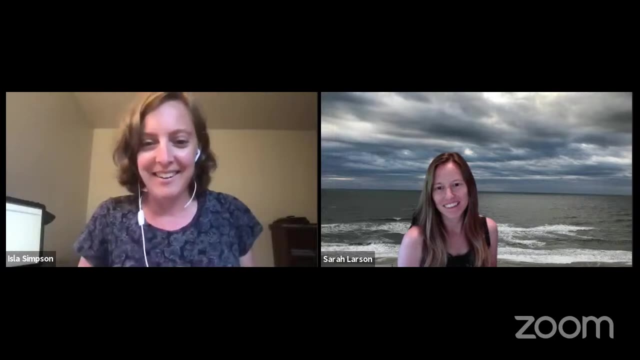